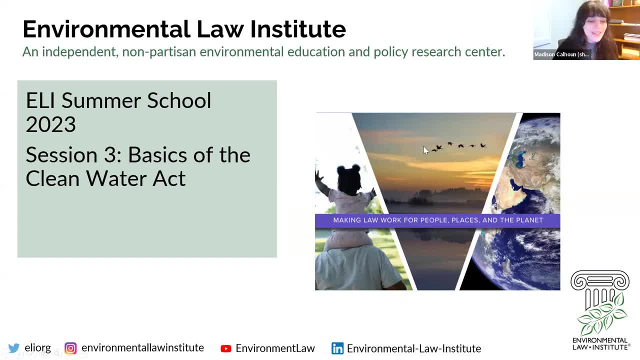 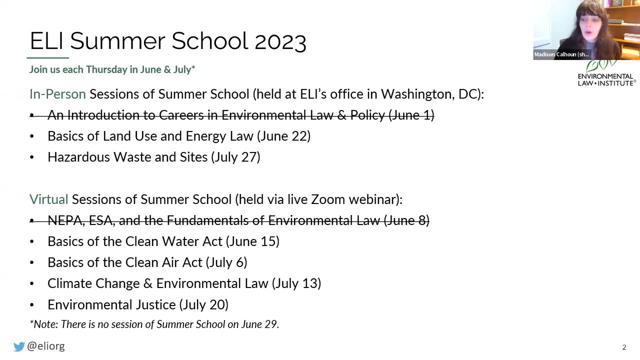 It's an introductory course into the basics and foundational elements of environmental law. No matter your background, you're welcome to attend all of our sessions. We'll have a session of summer school every Thursday in June and July at this time, from 12 to 2 pm Eastern time, except for June 29th. 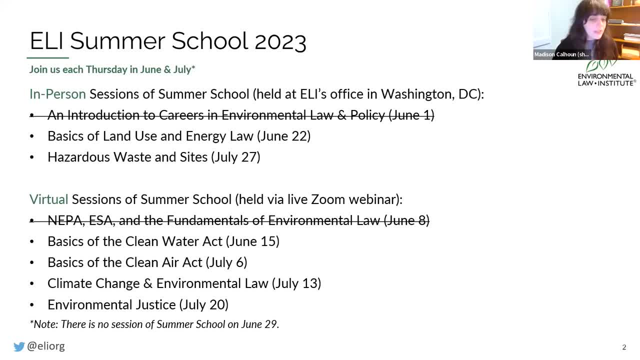 You can see on our PowerPoints the sessions that we've already held and all of our upcoming sessions as well. We will have two more sessions of summer school this year that will be hosted at our Washington DC office: Land Use and Energy Law Next Week and Hazardous Waste Insights at the end of July. 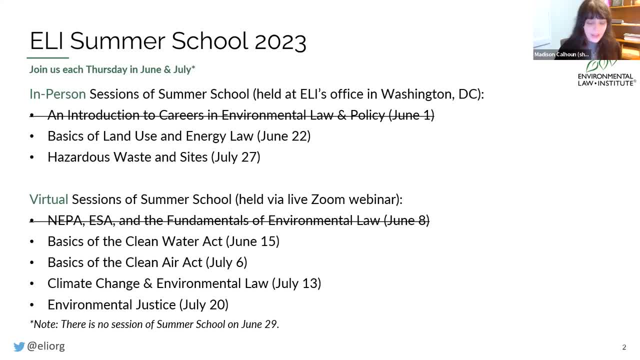 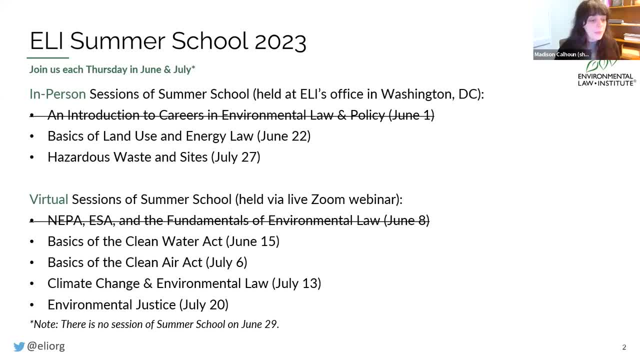 Each session will also be recorded and posted to ELI's website within a few business days of the event, so if you're unable to attend the in-person sessions, please feel free to watch them online a few days later. Please reach out to me or events at ELIorg if you have any questions at all. 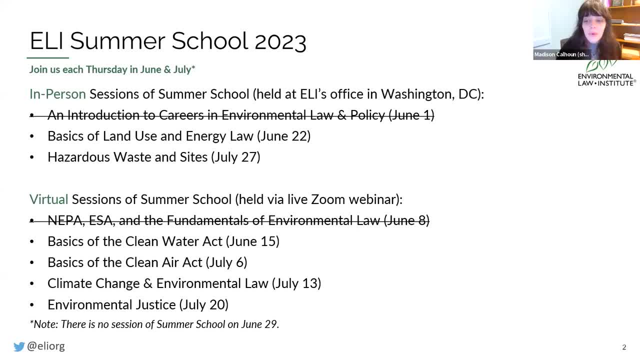 My email address is Calhoun at ELIorg. Now we will go ahead and kick things off for today, for today's session. Today's session is an introduction into the foundations of the Clean Water Act. In a moment I'll hand things over to our wonderful moderator. She will give some opening. 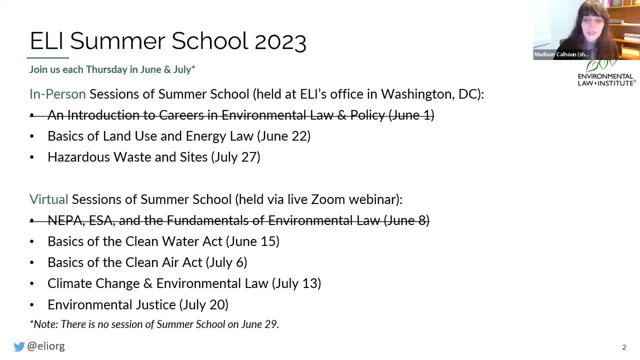 remarks and then our two panelists will present. After their presentation we'll have a roundtable discussion followed by time to answer audience questions. Please submit your questions throughout the webinar in Zoom's Q&A box, not in the chat. The chat is welcome or is open, so you are welcome. 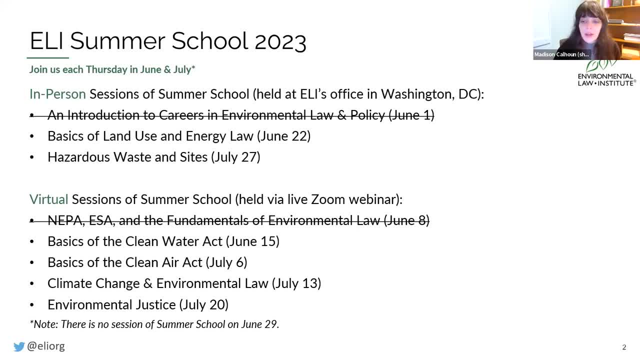 to use it to engage with one another and to post observations, but please post your questions in the Q&A box so that we can track them a little bit easier. You can also post your questions as soon as you think of them. There's no need to wait until the end of the webinar. With that, let's. 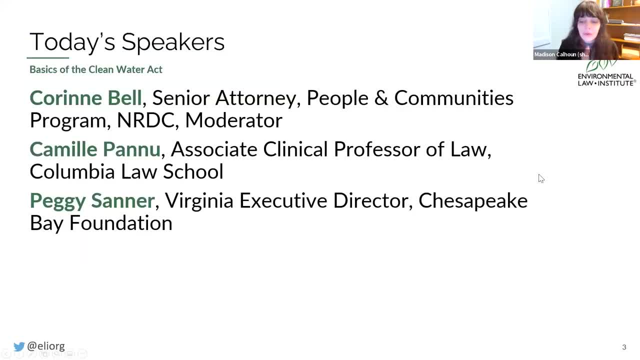 begin. I'm now going to introduce our moderator, Corinne Bell. Corinne Bell is a senior attorney in NRDC's People and Communities Program. Cori focuses on drinking water and surface water pollution in several states, as well as the water-related impacts of climate change. Cori's work includes: 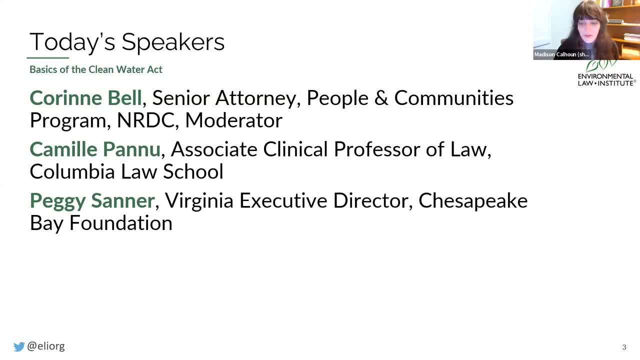 PFAS and lead contamination, environmental, environmental rights, urban runoff and green infrastructure. Before joining NRDC, Cori worked as a staff attorney at the Delaware Riverkeeper Network. She's a graduate of the Elizabeth Hobbs School of Law at Pace University, the Yale School of Forestry and Environmental Studies and Drexel University. She's 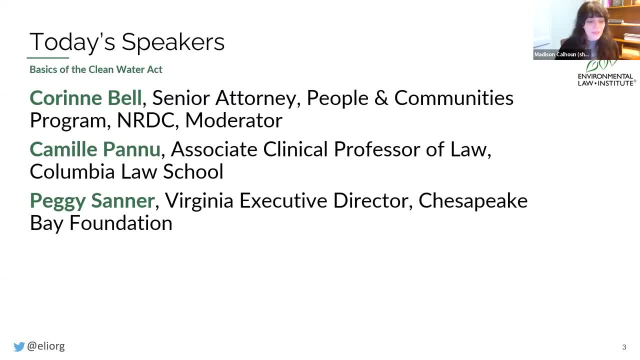 based in NRDC's Santa Monica office, And so all hand things over to you, Cori. Thank you so much to all of our speakers for being here. We're so excited to have you. Thank you for that introduction, Madison, And I'm excited to introduce you all to our excellent panelists today: Camille Panu and Peggy Saner. But first I do want to give a little bit of a roadmap. Peggy is first going to talk to us about the history of water pollution laws, starting with the Rivers and Harbors Act to the Clean Water Act. Then Camille will present on the regulatory framework for limiting water pollution in the United States. After that, Peggy is going to take us through how the Clean Water Act regulates both point and non-point sources of pollution. 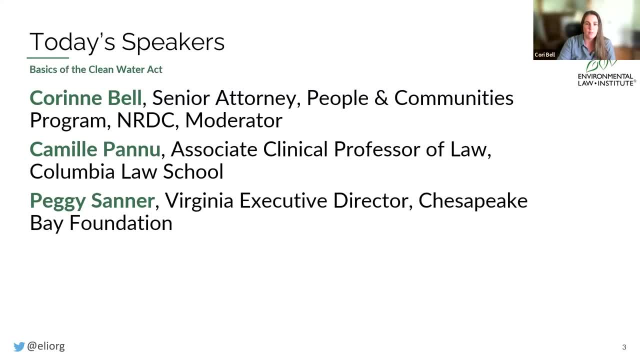 Thank you. And then we'll finish up with the three of us discussing what is covered by waters of the United States, which is a pretty hot topic lately. And, like Madison said, I'm going to keep an eye on the questions that are coming in in the Q&A session And if there are any quick clarifying questions, I'll ask them to the panelists at the end of that section. Otherwise I'm going to hold them until the end of the presentations. 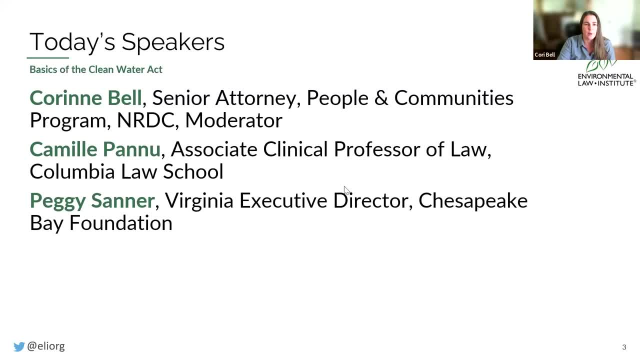 And, yes, this is being recorded, So if you have to step away for a little bit, you can come back and hear what you may have missed out on. So with that, I'd like to introduce you to Camille Panu. Camille joined Columbia Law as an associate clinical professor last year. 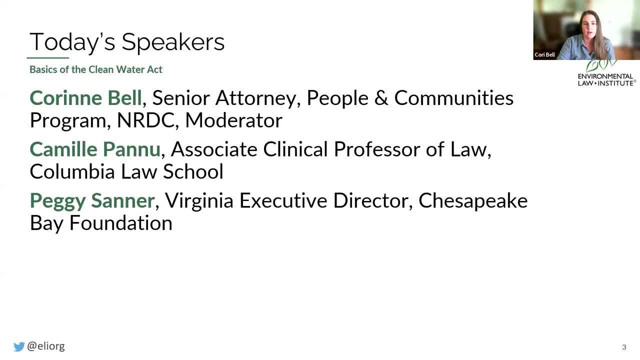 Camille founded and directs the Just Transition Clinic there, which focuses on addressing the disproportionate impacts of climate change on low-income communities of color, with particular attention to workers and shifting to more sustainable production. Before joining the Columbia Law faculty, Camille taught law clinics at UC Irvine and UC Davis. 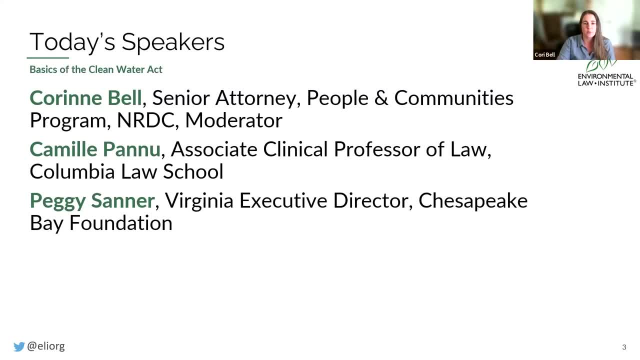 At the latter, she founded the Aoki Water Justice Clinic, which focused on providing safe and affordable water to low-income rural communities. Camille was also an Equal Justice Works fellow and a clerk for the US Court of Appeals, for the Ninth Circuit and US District Court for the District of Connecticut. She received both her undergraduate and law degrees from UC Berkeley. 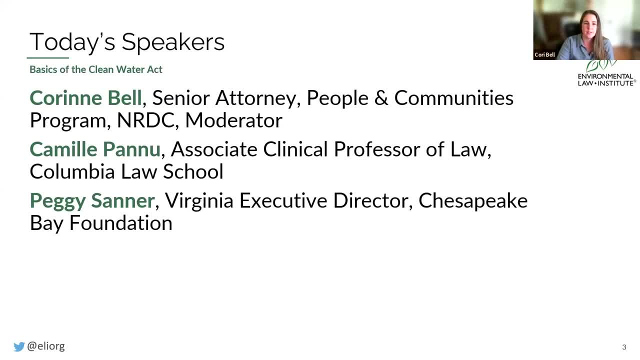 Peggy Sanner is going to start us off today, and Peggy has been with the Chesapeake Bay Foundation since 2010,, serving first to CBF's Virginia staff at the US Department of Justice, Peggy has been a law attorney and, since 2020, as the executive director of the Foundation's Virginia office, where she oversees 25 employees who work throughout the state. 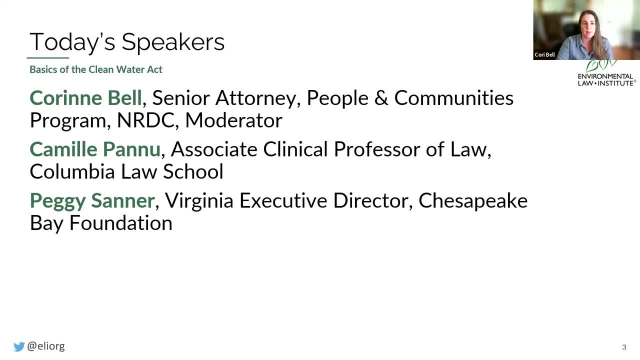 Prior to 2010,, Peggy worked as a litigator at several law firms. Peggy leads the Foundation's efforts to use science, law and advocacy to restore the Chesapeake Bay through implementation of the Chesapeake Clean Water Blueprint, the Total Maximum Daily Load Pollution Reduction Plan that you'll learn a little bit more about today. that was developed by the seven Bay jurisdictions and EPA. 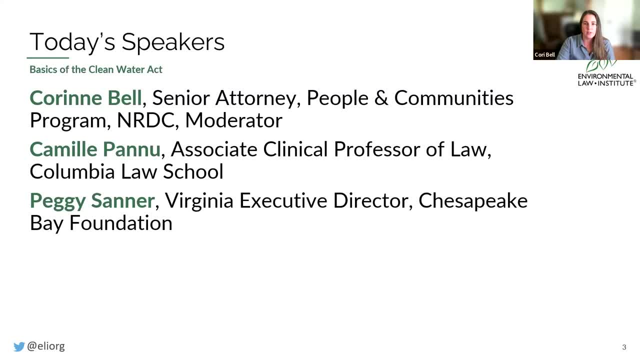 Peggy guides CBF's legal and advocacy work in Virginia, which includes working with the Virginia administration, members of the Virginia General Assembly, environmental agencies and numerous environmental partners. Peggy received her Bachelor of Arts degree from Swarthmore College, a Master's degree from the University of Pennsylvania and her law degree from Rutgers University. 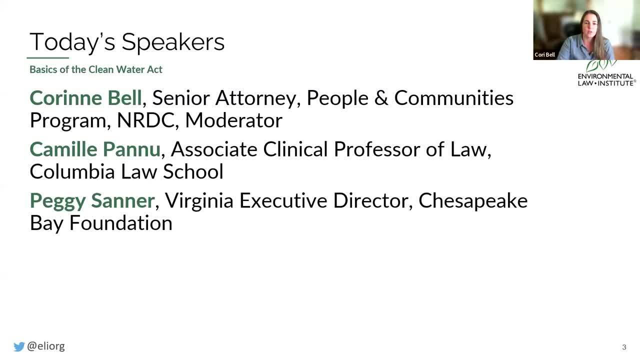 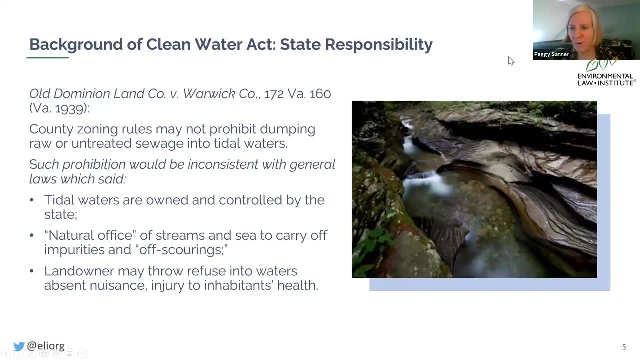 And with that, I will now turn it over to Peggy to give us an overview of water pollution control laws in the United States. Peggy, I think you're muted, Peggy. Good afternoon everyone. I'm very happy to be here to talk about, really, the foundation of the work that we do at the Chesapeake Bay Foundation and the foundation of clean water efforts throughout the United States. 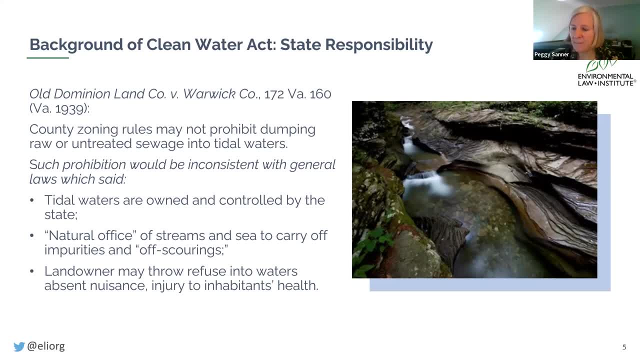 It makes sense to start off a little bit before the Clean Water Act, however, to think about the background and influences that may have on where we are today, And to do that I wanted to bring to your attention a case that was brought in Virginia in the first half of the 20th century, brought by a landowner, Old Dominion Land Company, against a county. 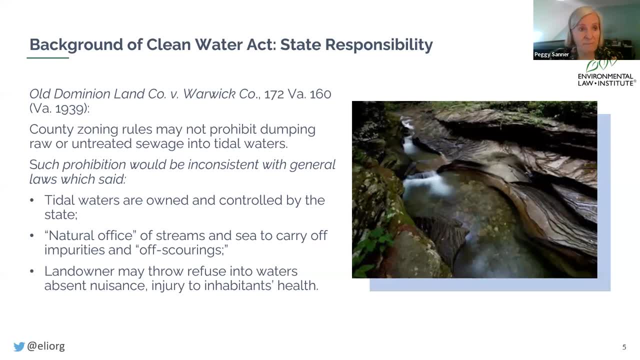 The circumstance was that that landowner had had been held in violation of the county's zoning laws because he dumped raw sewage into a tidal river nearby. The landowner was not happy about that and took the matter to, ultimately, to the state Supreme Court. The court ruled with the landowner saying first of all: 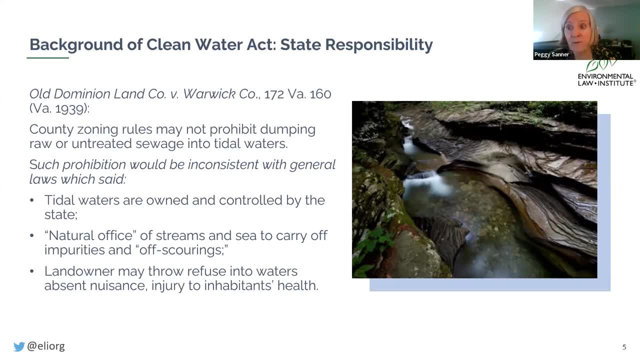 tidal waters are not something that the county has any control over, That's the jurisdiction of the state. But, more important, the very function of streams and rivers and indeed the ocean. the natural office, it said, is to carry off the impurities and the off-scourings of the land, getting rid of them so that the people can do what they want to do. 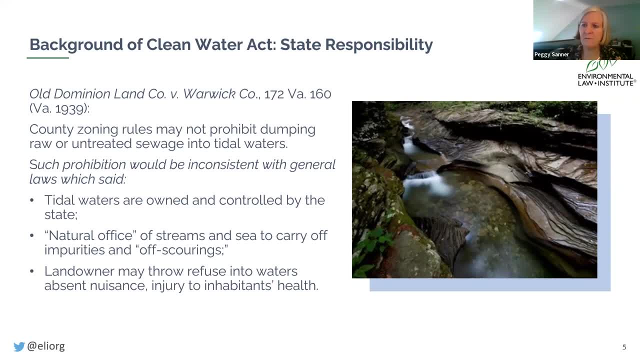 So pretty striking opinion, at least insofar as looking back on it almost 70 years later is concerned. but it wasn't alone. That was not a single opinion. That is a perspective that held sway across the country in a variety of different contexts from the state's level. 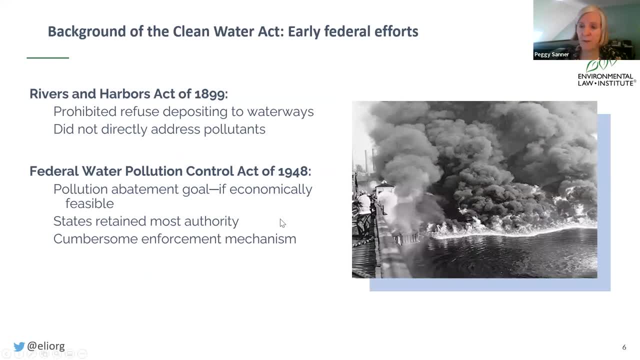 It was also in the background to early efforts by the federal government to take care of interstate waters. The first action that we've seen by Congress is the Rivers and Harbors Act of 1899, a law still enforced And though it did include some quasi environmental protections, largely it was directed to ensure that waterways- interstate waterways- did not have refuse dumped in it in a manner that would hinder or impair commerce on this waterways. 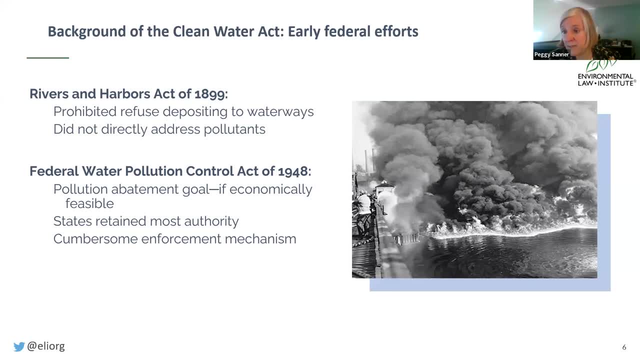 And so there was a permitting process in place. If someone disposed of refuse dumped in the waterways without securing a permit, There was no direct effect on pollution dumping per se. So some 50 years passed, during which various efforts were made to update that law. 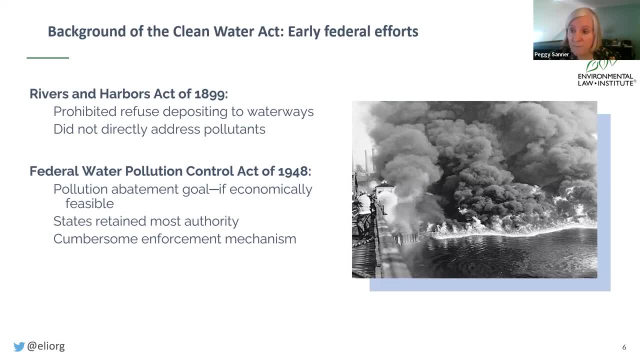 but they did not really come to fruition on a federal legislative level until 1948, when Congress was able to pass what became known as the Federal Water Pollution Control Act of 1948.. As you would imagine by its title, this one was focused, at least to some extent. 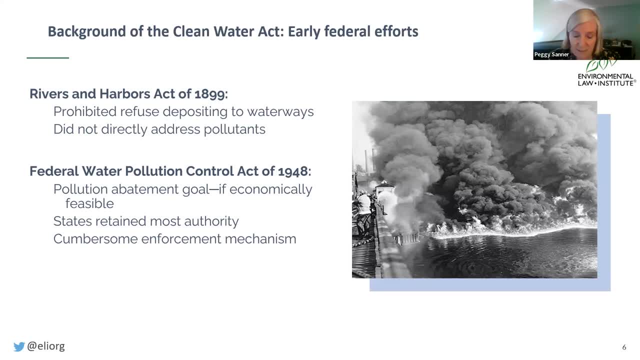 on controlling pollution, but it was quite limited. It applied only to interstate waters, not to any waterway that was entirely bounded within state borders. It allowed the federal government to, you know, give assistance to the states, maybe to provide some help in research related to. 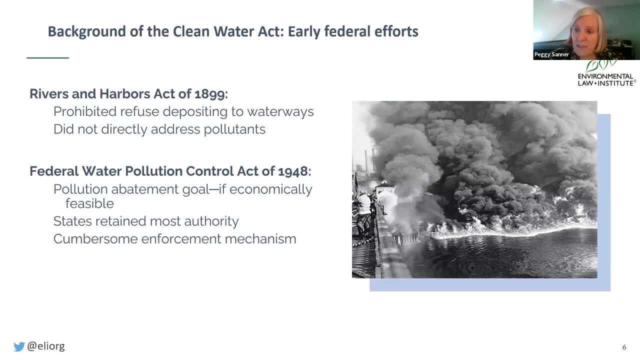 treatment facilities. but the states really retained most authority and you can see that in its very cumbersome enforcement mechanism. Really, the only enforcement mechanism that was included of any note is that if a downstream effect on health, a negative health effect, was asserted. 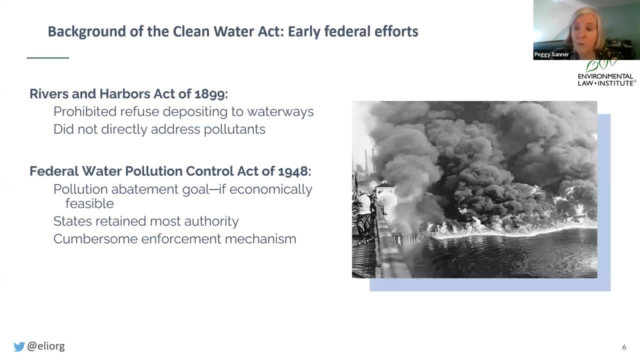 the US Surgeon General was theoretically empowered to bring an abatement action to stop that pollution, but only after some very cumbersome procedures and with the consent of the state where the pollution activity arose. That was so cumbersome and so awkward that in fact 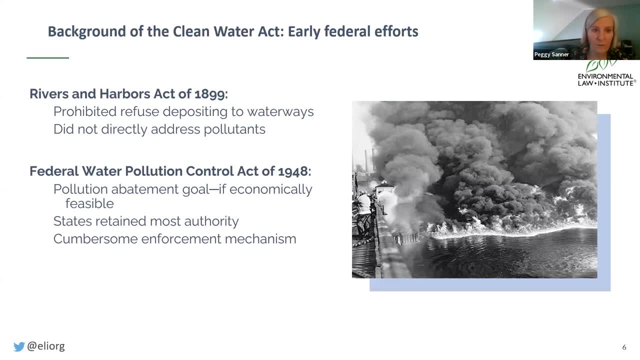 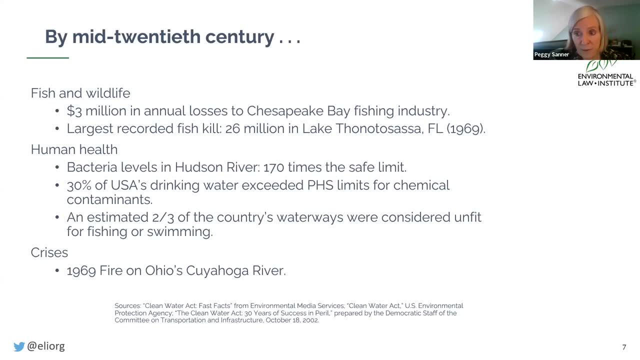 no enforcement efforts were undertaken for 20 years, And so we reached, frankly, the federal government in the middle of the 20th century with more than 100 years of industrial activity along our waterways, development activities that lined the waterways with cities, towns and other. 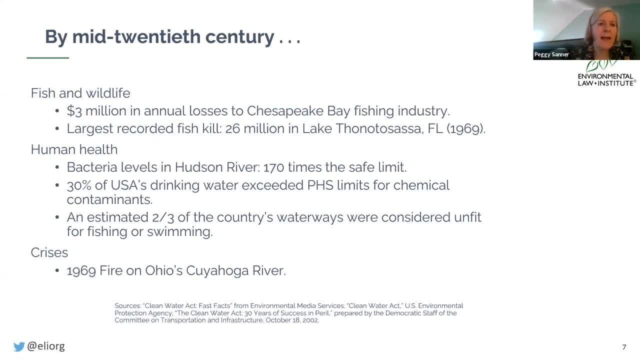 development, building activities and you could see the direct results of the historic treatment of our waterways, primarily as conduits to get rid of pollution or to facilitate commerce. We saw that in effects on our fish and wildlife. I've noted here a $3 million loss in 1969. dollars that's huge. 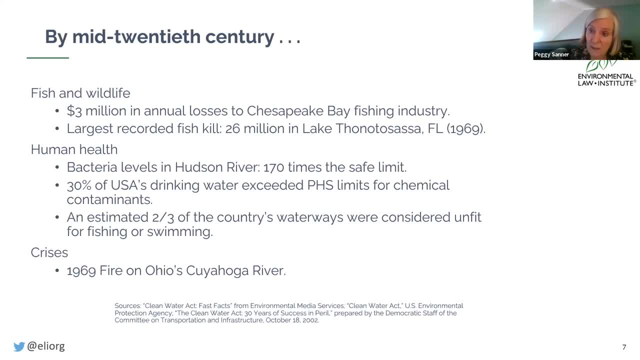 to the fishing industry. in the Chesapeake Bay, one of the historically richest fisheries in the nation, We saw the largest recorded fish kill in a lake in Florida: 26 million fish. those were not isolated instances. We had human health effects, bacterial levels in rivers. look at the one for Hudson River: 170 times what was considered the. 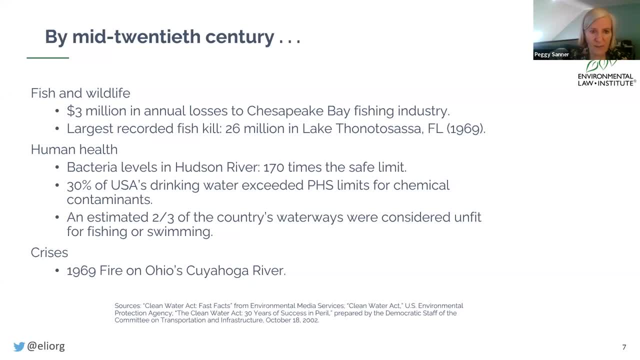 safe limit. 30 percent of drinking water in the United States exceeded public health standards for chemical contaminants and an estimated two-thirds of the nation's waterways were unfit for swimming or fishing- Obviously a terrible situation That could only be tolerated to the extent people turned their back to waterways. 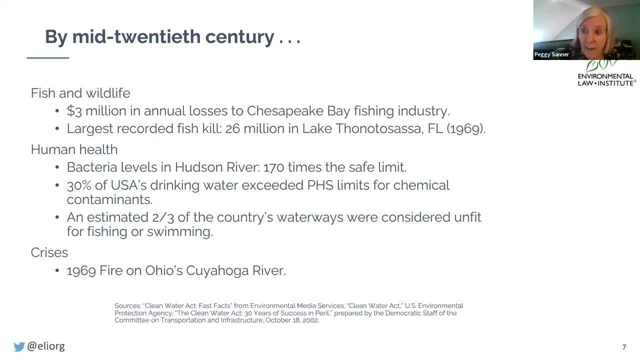 But then in that year- 1969, we had an event which many of you may have heard of, which was a major fire on the Cuyahoga River in Cleveland, Ohio. Now, it's important to note this wasn't the only fire that was ignited from the chemicals in the 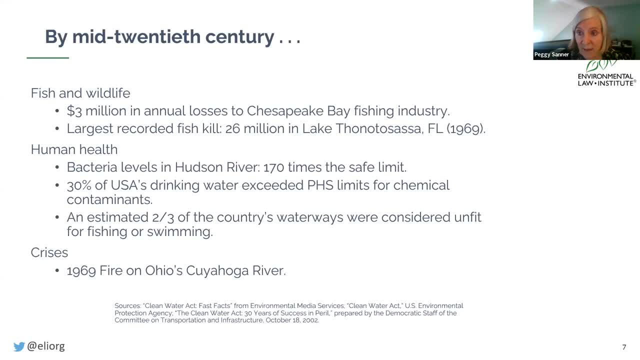 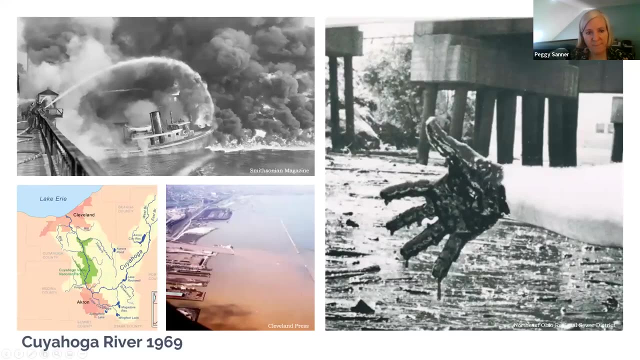 river. There were at least a dozen or so preceding that on that river. There were fires on other rivers across the country. It was not an uncommon occurrence, but it was a striking occurrence. You can see we're going to move ahead here. It was an occurrence that caught the horror. 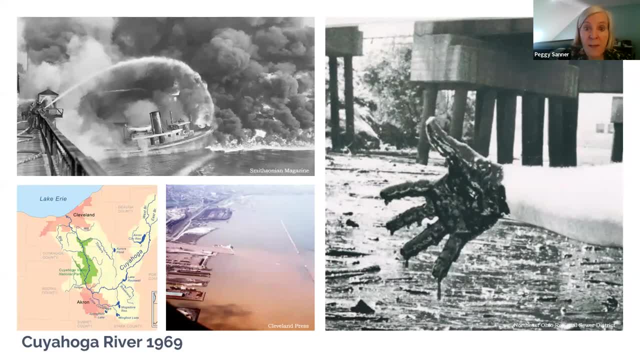 and, if you will, the imagination of our some very important media outlets in that era, certainly the local press Time Magazine, and you can see the images that the nation was treated to, which were, in a word, horrifying. 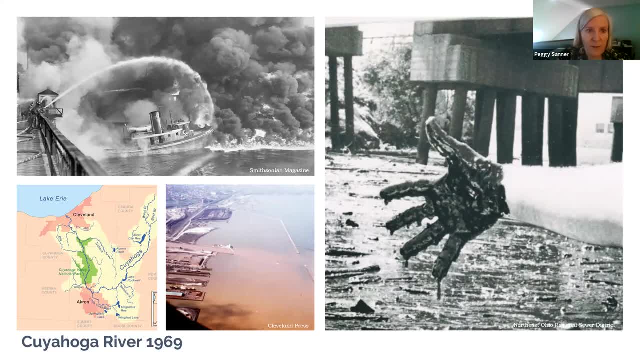 both in terms of the actual- if you will sludge in the river to the explosion type of fire that we saw in that picture. It was shocking to the nation and it generated an enormous public awareness and galvanized action. It is no mistake that it was the following year, 1970,. 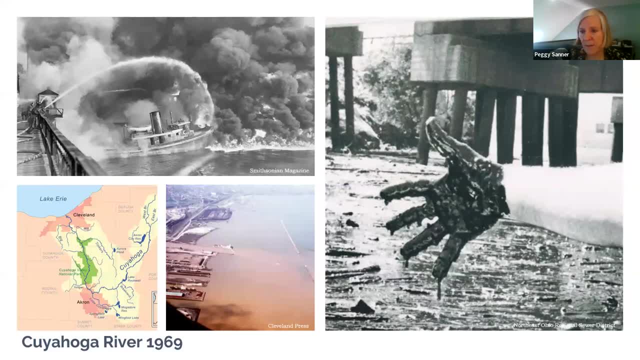 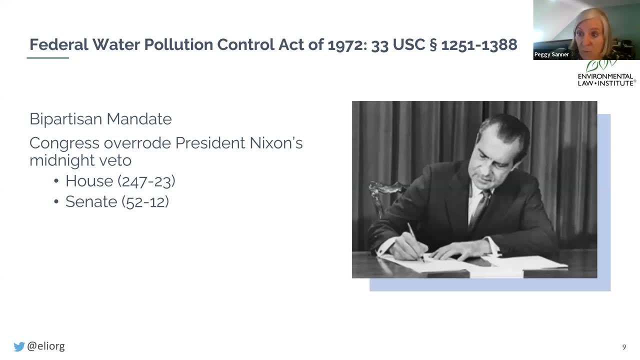 when we saw the first Earth Day across the nation. It's also no accident that shortly thereafter- shortly, that is in congressional terms- that we saw the major proposed announcement amendments to the Federal Water Pollution Control Act, which were enacted into law in 1972.. 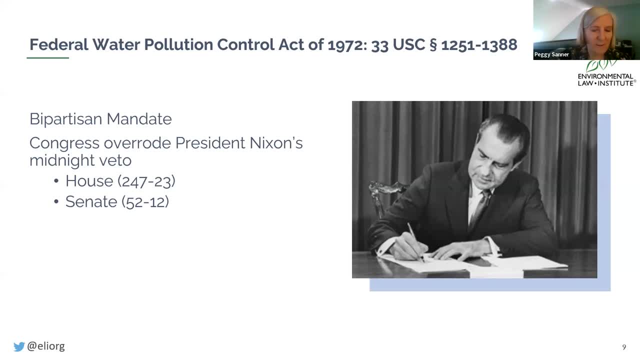 The law, as amended, was a mere what it shared with its predecessor of the same name is in fact the name that overhauled the framework in a dramatic way, as Camille will describe in great detail. But first I want to mention this was a bipartisan mandate. It was passed by both houses of Congress on a bipartisan way. The then president, Richard Nixon, vetoed it And in a stunning development, that veto was overridden in massive numbers by both parties, both houses. A remarkable statement of a unified national purpose. 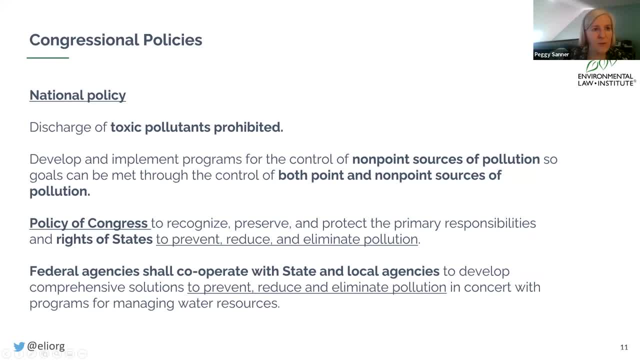 Let's see if I can get So. I just wanted to spend a minute or two on how that act articulated the national purpose. It reported to, in a specific way, schedule the elimination of toxic polluters. It talked about the different kinds of pollution. 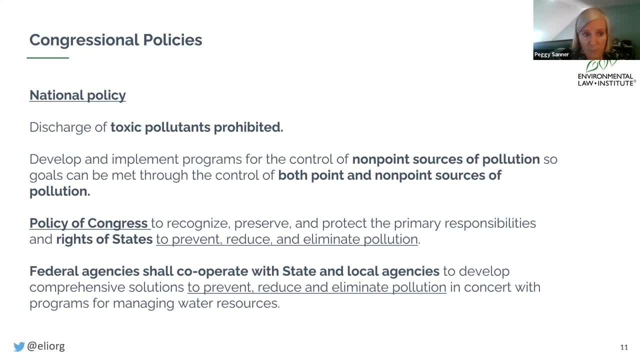 that would be regulated- And we'll get into more of that later- point sources and non-point sources. But it stated a policy that was important for the development of and ultimately the passage of, the act, And that is, it did not trample on. 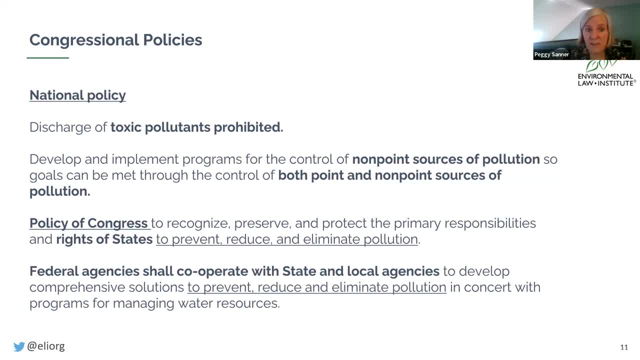 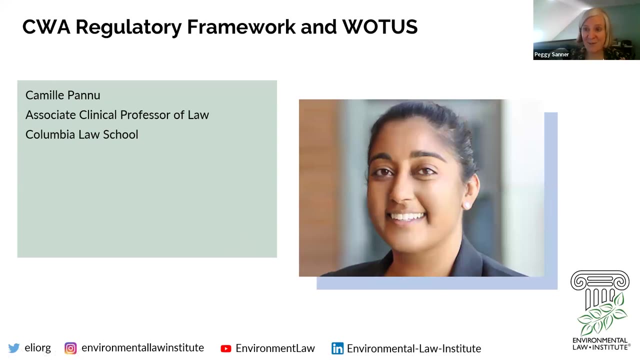 but it supplemented the historic rights of the states to prevent, reduce and eliminate pollution. Federal agencies were tasked with cooperating with the state, And that was a key part of helping it to pass. So I'll now be delighted to pass the baton. 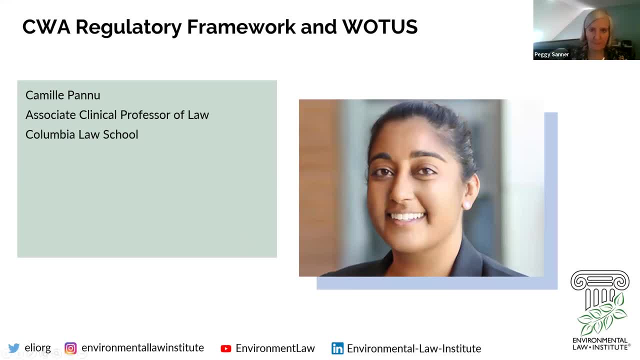 to my colleague, Camille Pannou. Thank you, Sorry. one sec, All right. so let's talk a little bit about the nitty gritty of the Clean Water Act. Thanks for giving me the opportunity to talk about it. If you could take a second to ask a couple more questions. 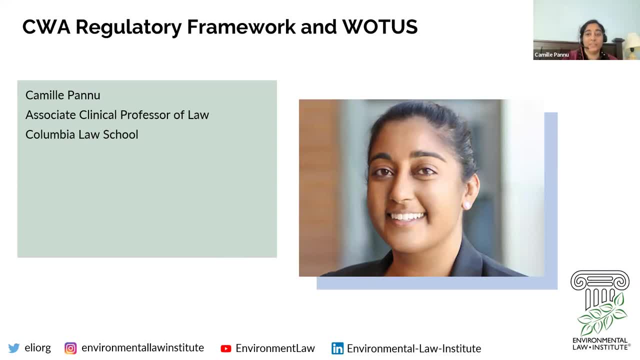 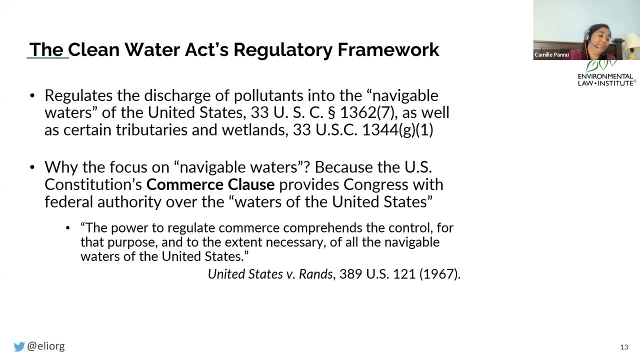 Sorry, I went off. I'm sorry, I don't mean to interrupt you. I can't hear you. now I know it's mostly us, but Sorry, I'm having a little bit of trouble with the slide movement. There we go. All, right, now we're cooking with fire. So, to take a step back, it helps to know kind of where the Clean Water Act gets its authority from, Because it kind of helps set up what we'll talk about a little bit later in this session on the waters of the United States. 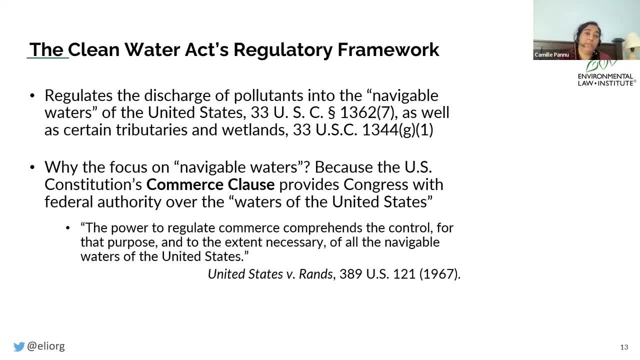 And that's a new event for us. we're doing a lot of work, So I'll talk about that in a little bit later in this session on the waters of the United States states. But I wanted to kind of set up the geographic scope a little bit. So the mandate: 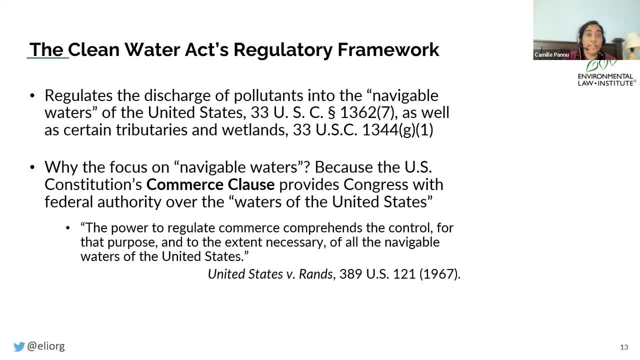 of the Clean Water Act is written fairly broadly, and that's intentional. As Peggy said, there was really powerful bipartisan support for the Clean Water Act and for its subsequent amendments, And so part of that was to ensure that it wasn't just the navigable waters of the United States. 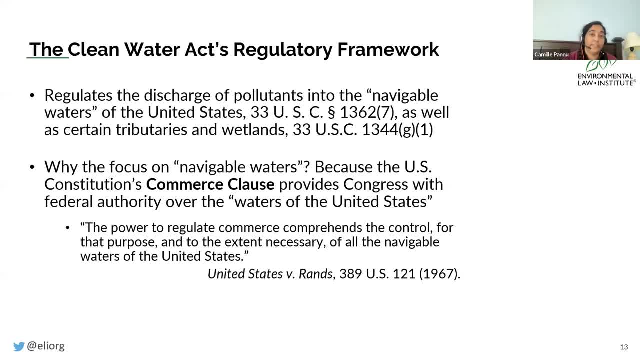 that were protected from pollution and that the navigable waters ends up being a term of art. But it was also important that we think about water systems as connected. So a lake doesn't exist on its own right, A river doesn't exist on its own. Anyone who has exposure to water systems. 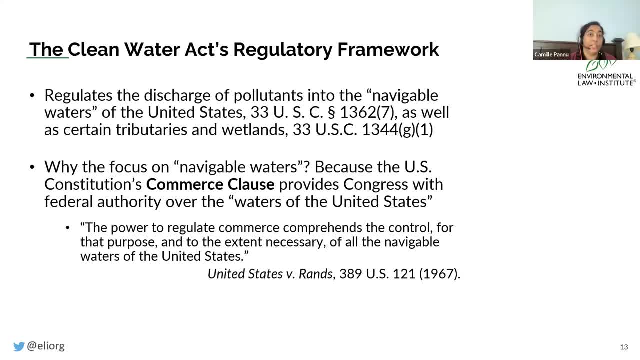 understands that there's watersheds, there's interactions between wetlands and streams and creeks and other tributaries. there's runoff. So the built environment and the natural environment are complex And are not limited. You can't separate a river from all of the different tributary streams. that 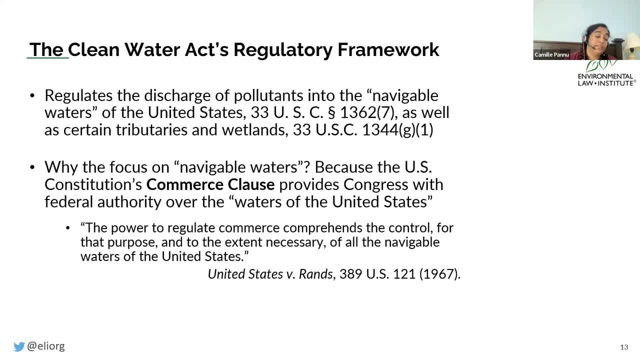 go to the river And because the federal government understood that the Clean Water Act tries to focus very directly on how to manage the flow of those kinds of potential sources of pollution into water And pollutants can be written kind of large. Originally we were thinking about 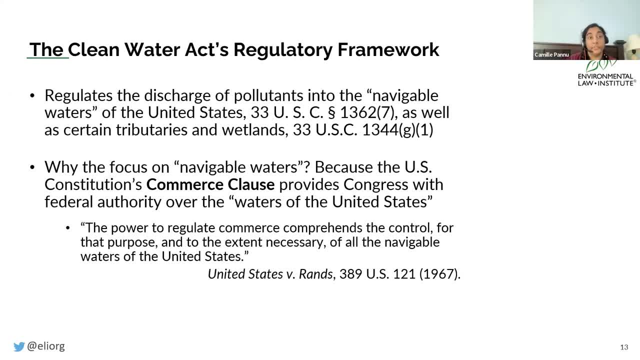 or when the Clean Water Act was passed, there was a great focus on industrial pollutants in particular. But examples, other common examples of pollutants can be: you know, raw sewage that's like dumped out into the water. that was kind of common at the time. 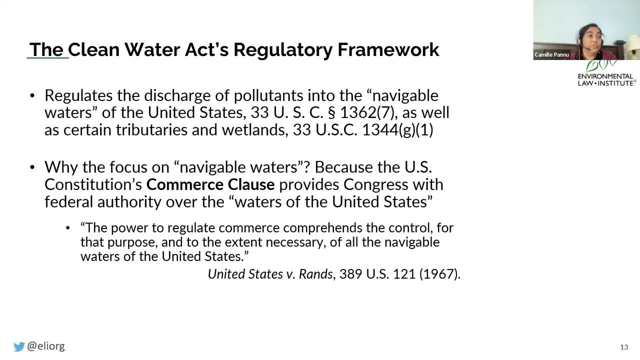 It can also include runoff from stormwater surge or from stormwater kind of flowing out into gutters, And it can also include things that we might not think of intuitively, like changing the temperature of the water. So it's not just chemical pollutants. there's a pretty wide array of things that can be considered a pollutant into. 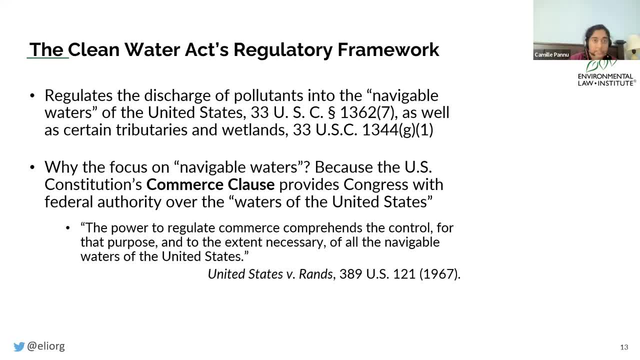 the water. The reason that we focus on these navigable waters is because the federal authority for regulating pollution and regulating the quality of our nation's waters comes from what's called the Commerce Clause within the Constitution. The Commerce Clause is how Congress does a lot of. 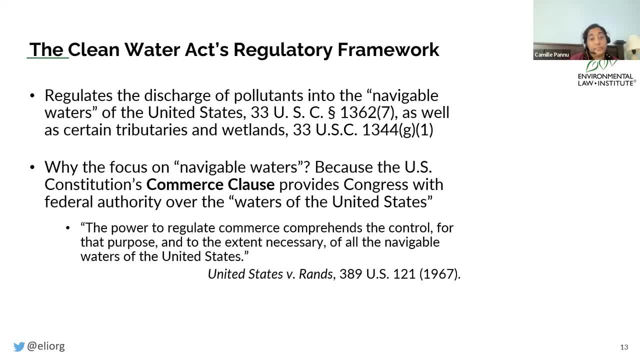 regulatory work That becomes really important. It's based on the idea that Congress has the right to regulate interstate commerce, meaning any kind of trade or activity that's related to economic processes, and that that can include maintenance of waterways- This term, waters of the United. 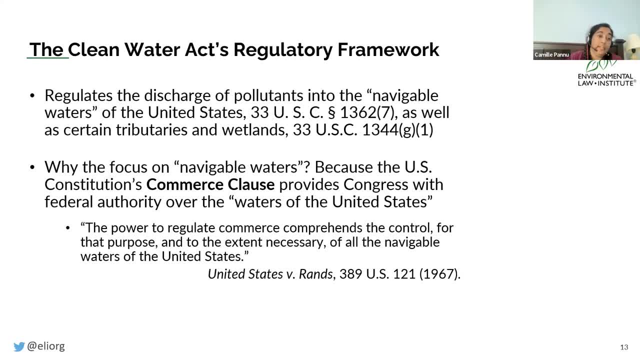 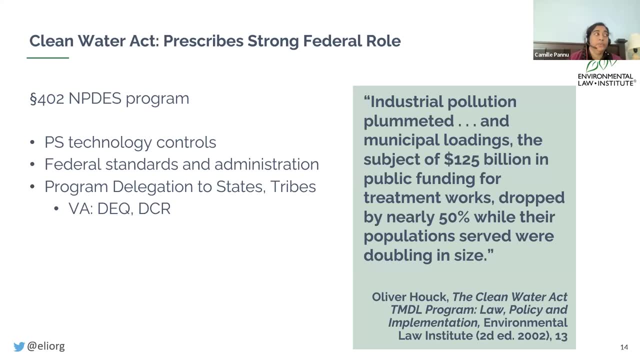 States and navigable waters, which we'll talk about at length, comes up pretty in-depth throughout the Clean Water Act. That is, the framework for the geographic scope. The Clean Water Act interceded in part because we weren't getting the same level of regulation that we needed at the state level and also 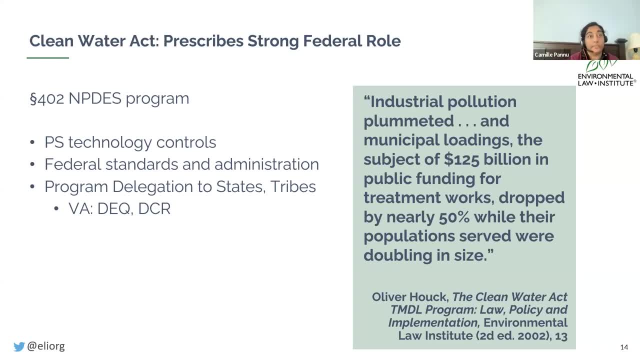 because anything that's an interstate water system is going to be difficult to manage, especially when you have a water system that's banned states that are politically very disparate. The federal government created a water system that's going to be difficult to manage and the federal government created a series of permitting systems and different permission. 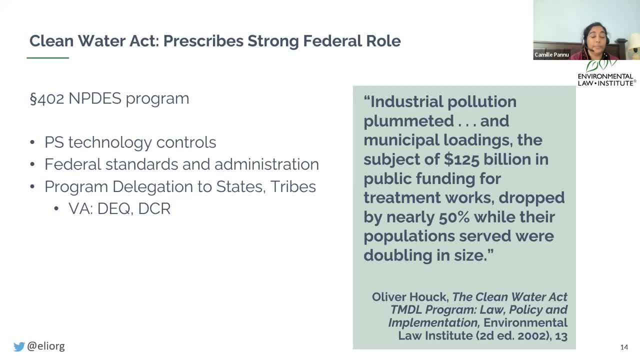 systems to deal with different elements of the Clean Water Act. The system that we'll talk about the most is the National Pollution Discharge Elimination System Program, or the MPDES permit. These are permits that are given to point sources, which Peggy will talk about in a little bit. but 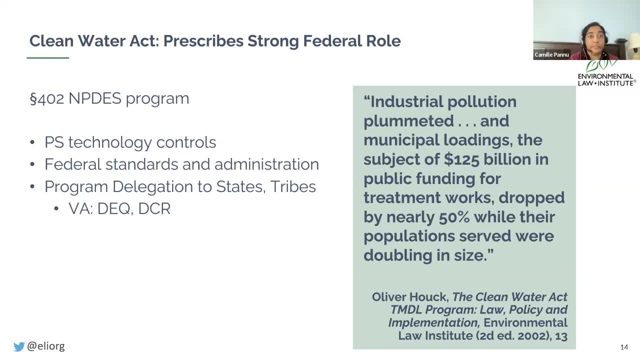 they are essentially concrete sources of water pollution. We know that this thing is going to be releasing things that will pollute the water on an ongoing basis, and so we are going to ask you to get a permit. The permit is going to do things like set the total maximum daily load, which is 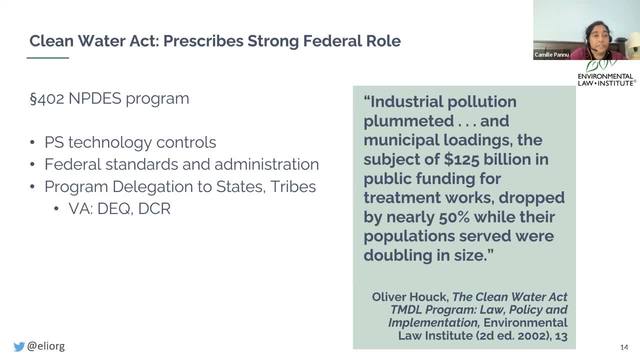 another term of art. So what is the most that this ecosystem and this water system can handle of any given pollutant? And so the permitting system is trying to help balance the inflow of different kinds of pollutants into our waters. It imposes certain technology standards. 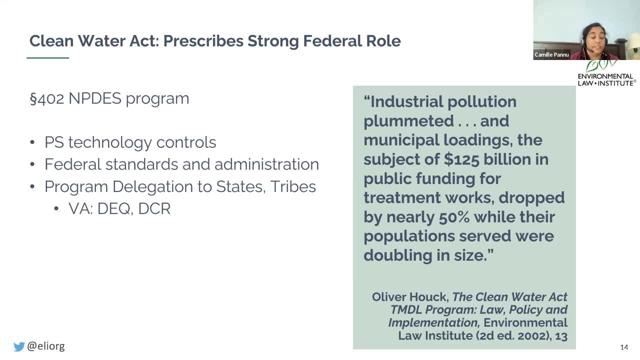 depending on what kind of pollution it is, and asks essentially the polluter to be responsible for a portion of ensuring that certain pollutants are not released at all and that other pollutants are treated before they're released into the water. And the way that this works is through. 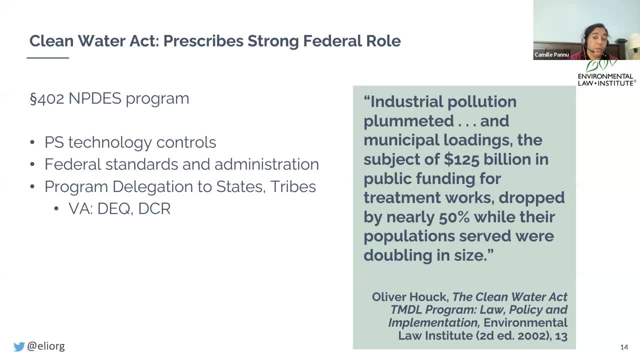 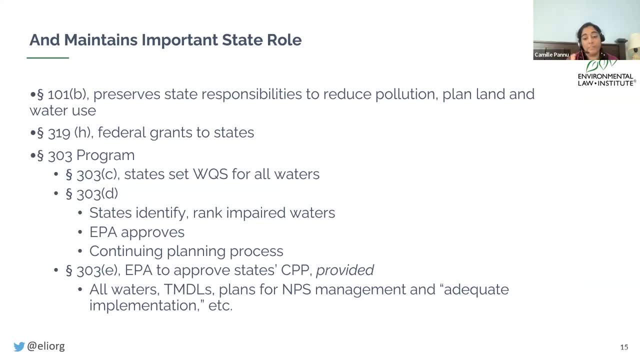 a pretty complex system of what we call cooperative federalism. So here we go. So the way that this works- and this is true also in the drinking water system- is that the federal government sets the standards based on science best available science at the 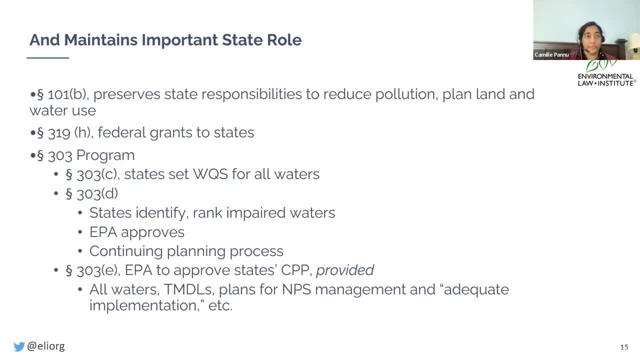 time. And so there's this iterative process where the EPA and other regulatory agencies are working together to generate as much public health and scientific data as possible to help support figuring out what each water system can survive or sustain, And they set the standards and then they delegate the authority to tribal governments and to the states. 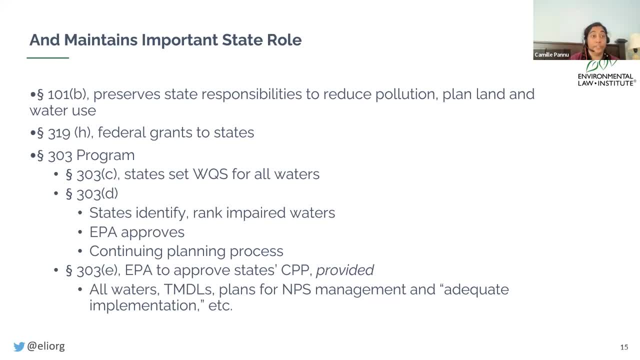 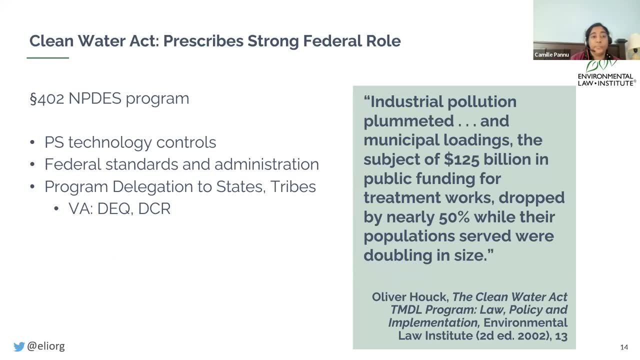 to issue the standards, And so they set the standards and then they delegate the authority to the states to issue the permits. So different states have different issuing agencies. So for example, if we go to the previous slide, in Virginia this is the Department of Environmental. 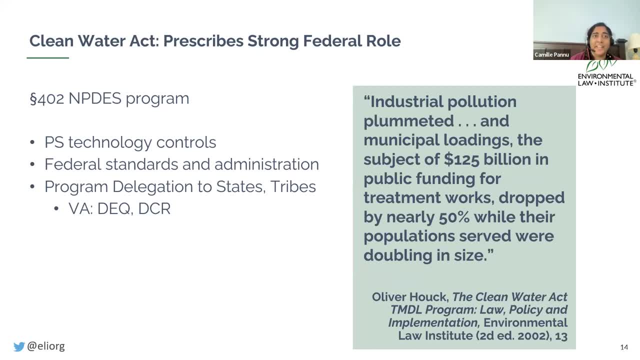 Quality. And then, Peggy, what's DCR? the Department of Conservation and Recreation. Conservation and Recreation: There we go. In California, this is the State Water Resources Control Board, which is a very long name. In New York, this is the Department of Environmental. 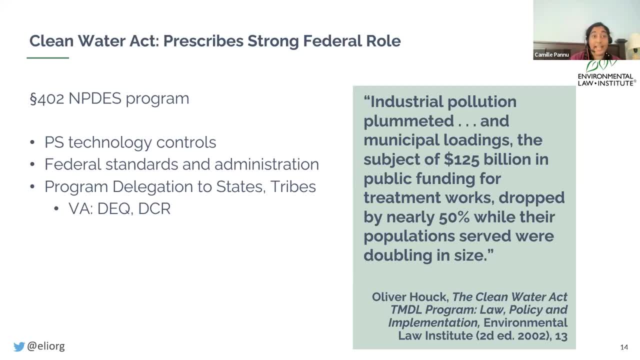 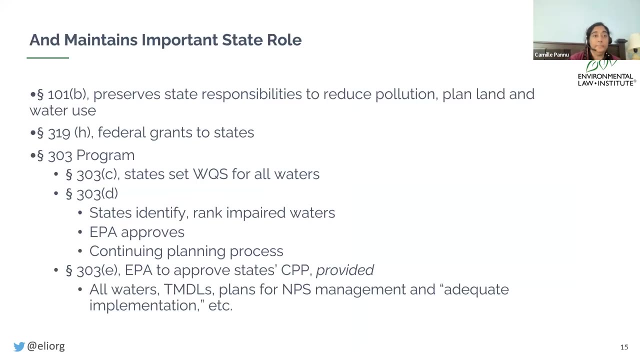 Conservation. So each state has an agency and is supposed to designate an agency that is in charge of managing the permitting system. So they're accepting the applications, issuing the permits and ensuring that folks are in compliance with these federal standards. It's important to note. 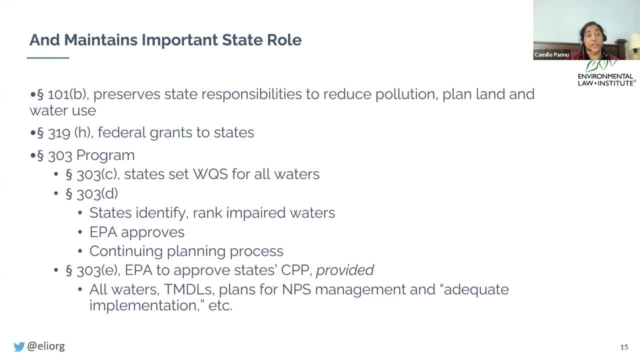 that the Clean Water Act really contemplated that states should retain their ability to manage their water systems, And so they're doing that, And so they're doing that, And so they're doing that as well. So it sets kind of what I would call the floor. So it's a federal floor on. 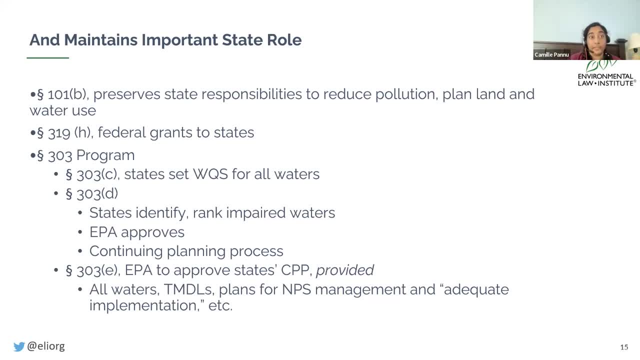 here's what we need, at a bare minimum, for our water systems to be healthy. States can then go above and beyond, And there are about- I think we were going to say in the context of wetlands- there's 19 states- is that right- that also have additional protections, that 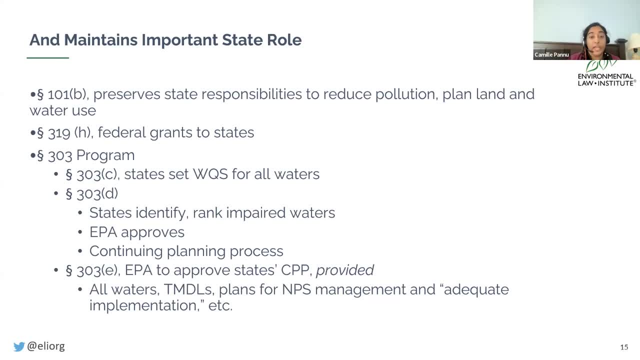 they've adopted at the state level that go beyond the federal protections And those work together to ensure that there's adequate protection in the clean water system. And so there's a lot of beasting and plenty of talk around the Clean Water Act, above all the other standards that the protection wants. 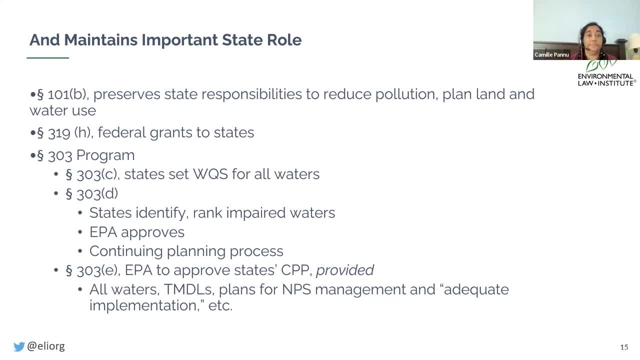 And so Cleカンタones says explicitly that, you know, the act does not supersede or preempt state regulation of its own standards if those standards are above what the Clean Water Act provides. So you can't go below, but you can go above. And so, in order to help facilitate this, the Clean Water 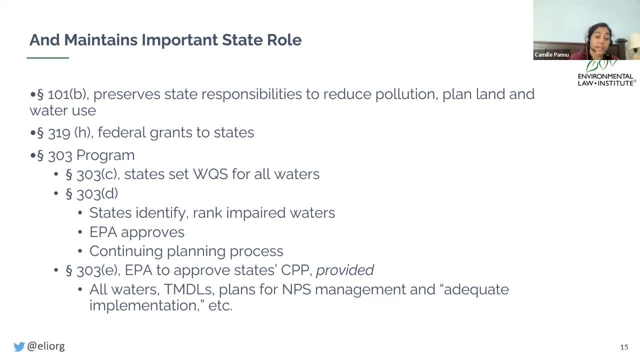 So state revolving funds, which are a partnership between the state and each state and federal governments to create, essentially, a pot of money that people can apply to to try to build projects or to try to implement systems that will decrease water pollution, particularly from sewage and stormwater systems. 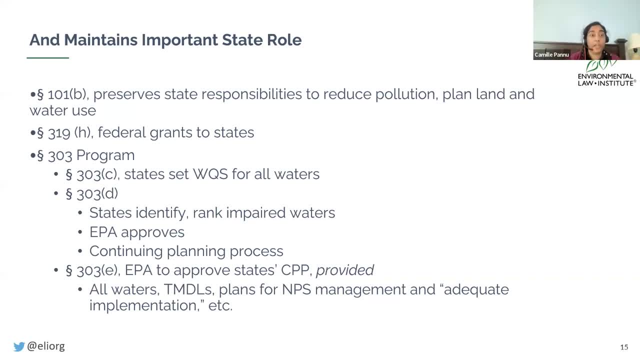 But the Clean Water Act covers more than that. There's a number of grant programs as well to states And you know the Clean Water Act kind of sets a standard for water quality standards and then also ask states to be involved in ranking how impaired each of their water systems is. meaning how far are you from your ecosystem being healthy? what's your most at risk system? 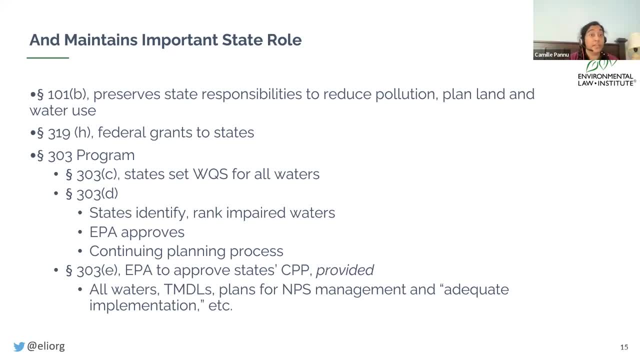 So, for example, I live now in New York City For the longest time. the goal Canal was very high on that list. the Hudson River was high on the list as well. So which water systems are impaired and require some kind of remediation and help can vary from state to state, and the Clean Water Act allows each state to essentially 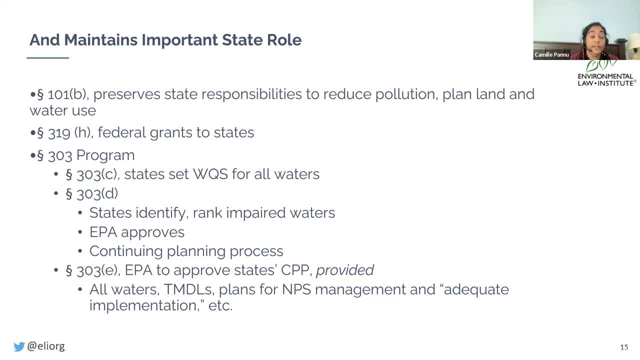 set its goals for what its highest priority water systems are, while requiring all of all of this process to kind of come up. states come up with plans for how they'll address this and then the federal government or the EPA approves that plan. That's very similar. 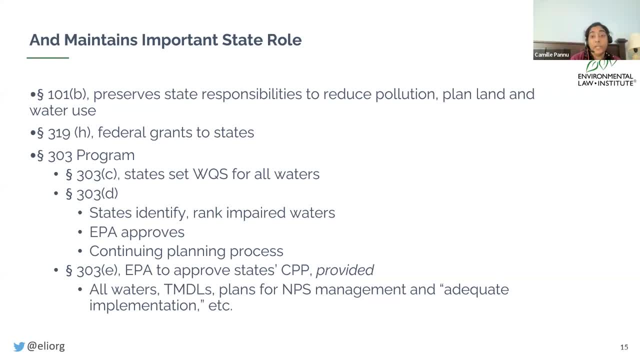 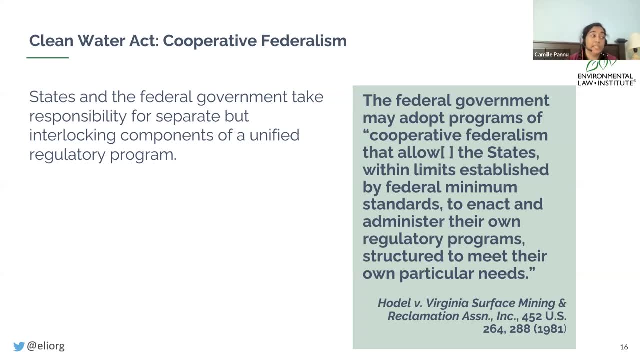 That's very similar to how we regulate air pollution as well, for example. So um So we talked about cooperative federalism. This is the idea that the state and the federal government or partners, and that there can be overlapping regulatory systems, but that they're working. together to meet the needs of of, whatever the local conditions are. there's this idea that there's innovation when you allow states to have that kind of flexibility so we don't have to pay it directly off to tenants or anything. And if that isn't the case, I'm going to tell you that any will or will not be a thing when, in November, there are grants. 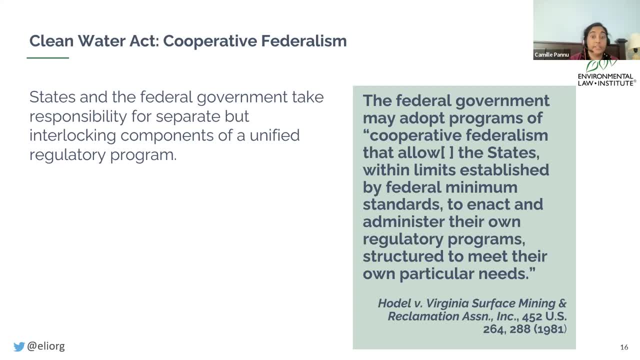 the needs of whatever the local conditions are. There's this idea that there's innovation when you allow states to have that kind of flexibility, so we don't have the federal government mandating and then being so rigid that states can't be creative with how they try to get programs off. 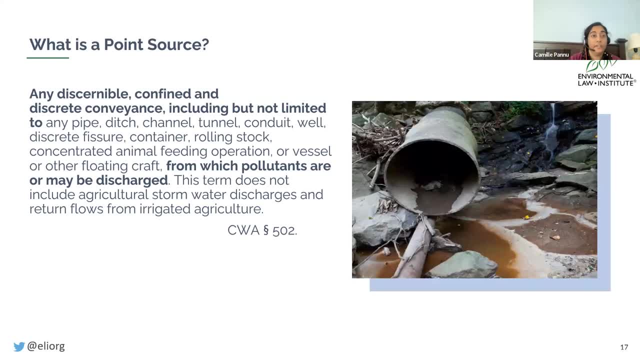 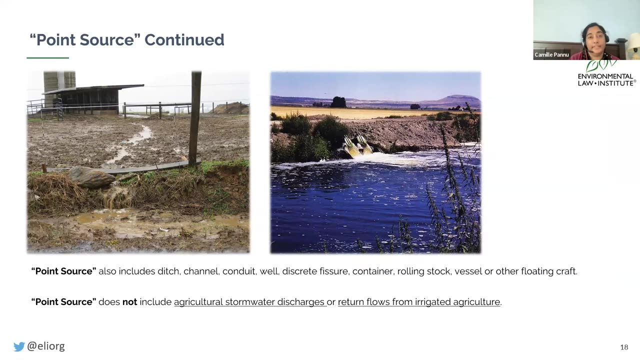 the ground or what they pilot. And now I'm going to turn it back to Peggy to talk about point sources versus non-point sources which, as I mentioned, are really important in the context of the distribution and permitting system that happens through the MPDES system. 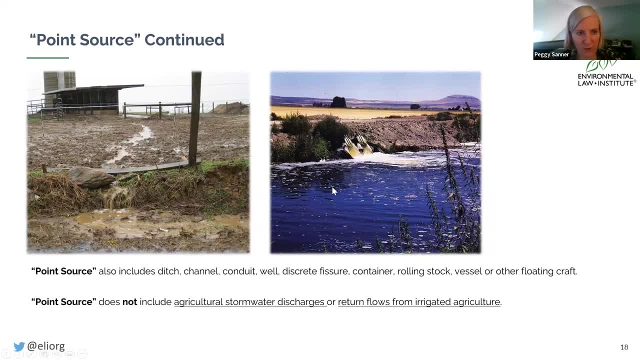 So I just wanted to state at the outset one characteristic of lawmaking, and in particular federal lawmaking, of complicated programs like the Clean Water Act. You have to kind of figure out what they're talking about, but you need to look at all the definitions. 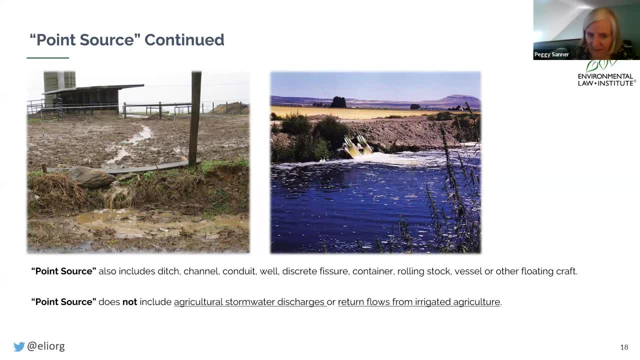 And the definition that I want to start off with is point sources. Camille has identified point sources as one of the group of sources of pollution that the Clean Water Act addresses. And so what is it? Well, it is classically a pipe, from which. 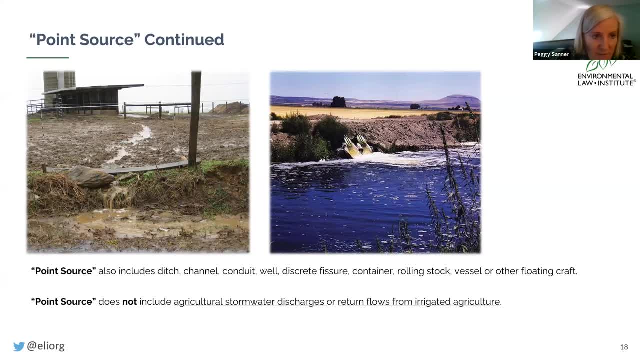 really nasty industrial stuff or wastewater stuff is poured out into a local waterway. That's what most people think of as the classic point source, But in fact it also includes a whole lot of other things: Ditches, channels, conduits, wells, discrete fissures, rolling stock vessels. 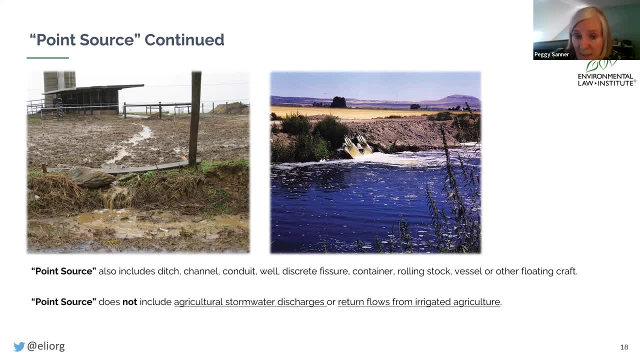 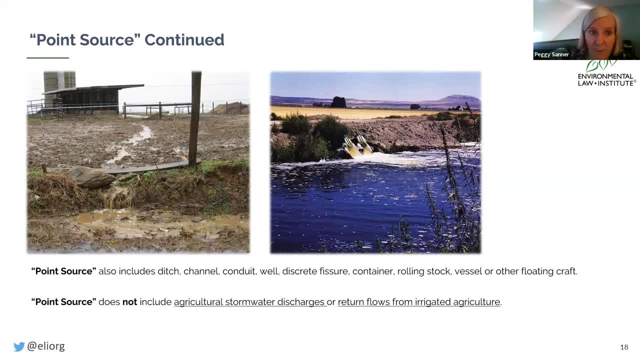 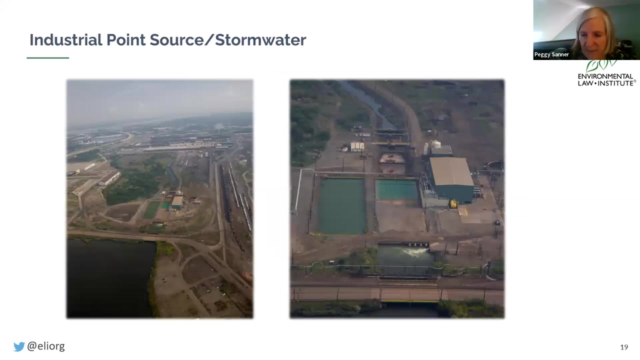 nonetheless. you may not think about that as a pipe, but you see the ditch which is pouring water into a larger ditch, potentially an irrigation ditch, and that is considered to be a point source. Moving this to the next slide, Here are two industrial facilities that I want. 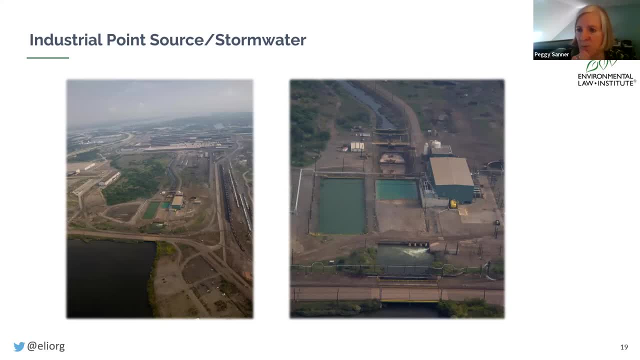 that allow us to talk about two different kinds of point sources. Under the Clean Water Act framework. there is the actual physical structure of an industrial facility, whether it's a wastewater treatment plant or another chemical producing, potentially a chemical producing, operation. Those facilities may have pipes that discharge local waterways. 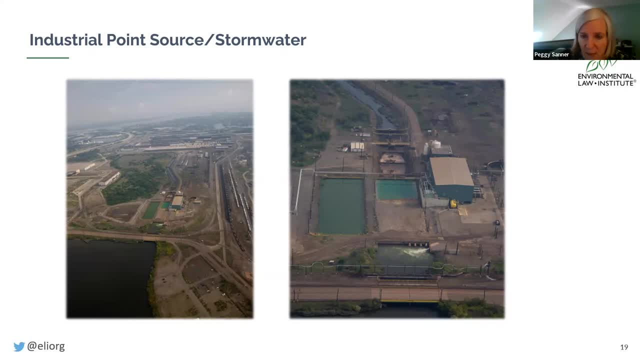 Those are plainly point sources. But you'll notice here, as we all know, these facilities, they sit on lands, and they sit on land which receives rain, and that rain can wash over the surface of the water, picking up pollutants, maybe dirt, maybe particles that come from the air that's been subjected to, for example. 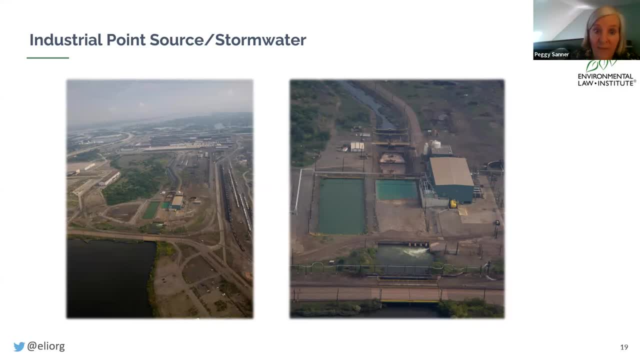 some air emissions, So it could be there are chemicals in that stormwater. So EPA regulates industrial industrial facilities, not just with the pipe leading it leads out that releases fluid discharges, but also stormwater discharges from industrial facilities. 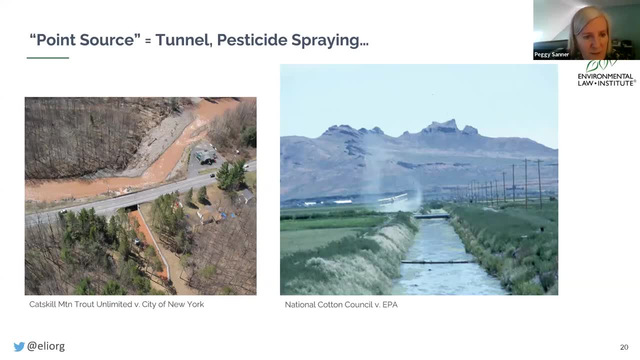 Here are more examples of industrial facilities that have been deemed to fall within the category and point sources. You see in the left this is that tunnel that connects wastewater from the city of New York, filled with sewers, to хそれ sediments. you can see by the color- with a waterway And the city first challenged. 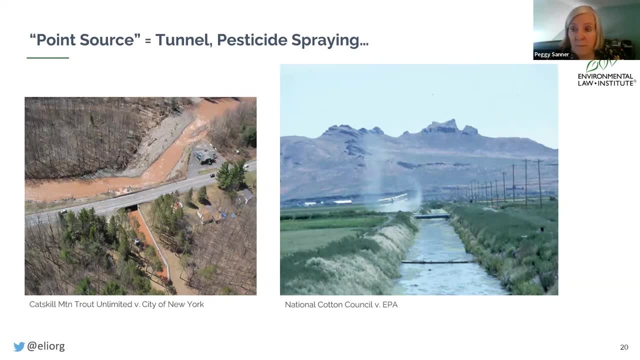 an enforcement action. They said the city had failed to get a Clean Water Act permit, a National Pollution Discharge Elimination System permit, and therefore was in violation. And the court held that there was a violation because this tunnel was a point source and it. 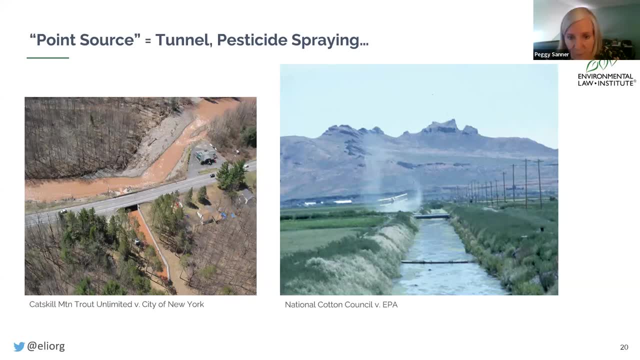 needed to be permitted. Another example: a fairly well-known case: the National Cotton Council versus EPA. What was at issue? there was a system which sprayed pesticides on agricultural lands, with some of the spray ultimately landing into what looks to be here, an irrigation ditch. 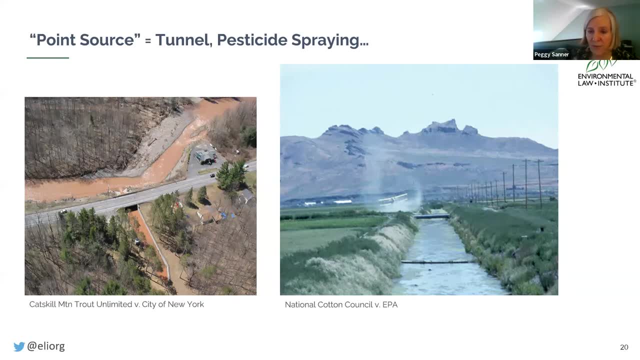 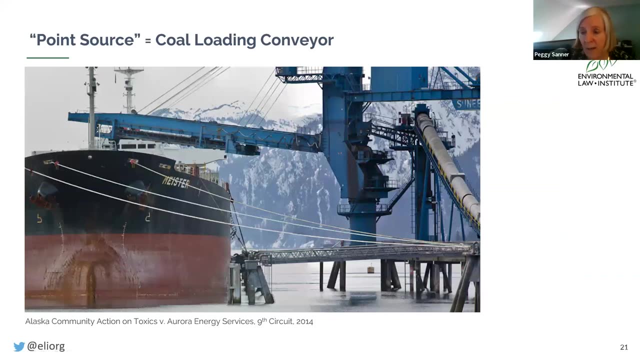 then connected to a waterway. The court held that that wasn't indeed a point source and needed to be permitted under the National Pollution Elimination, Discharge Elimination System permit. I'll call that a NPDES permit here on out, by way of habit. Another one here. this is a coal-loading conveyor which was under scrutiny by the. 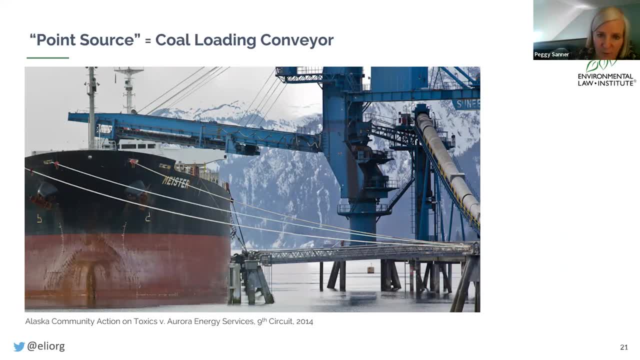 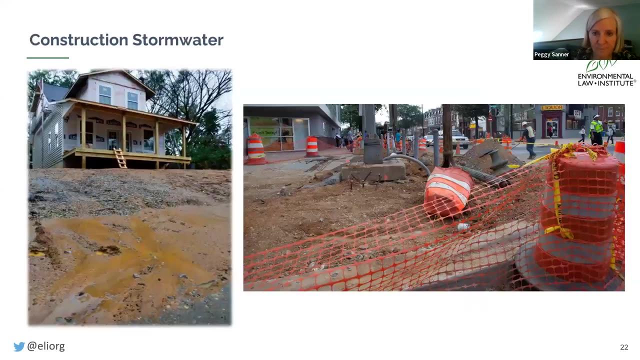 federal appellate court in the western part of the nation, the Ninth Circuit. The conveyor carried coal, of course, and some of which ended up in the waterway. It was a point source, according to the court, Another important kind of point source. 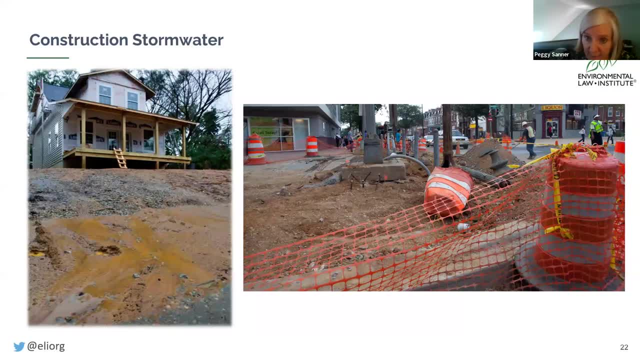 for land-disturbing activities, land-disturbing activities that disturb at least an acre, or when such activities are not carried out. This is a point source that is not carried out by the state. This is a point source that is not carried out by the state. 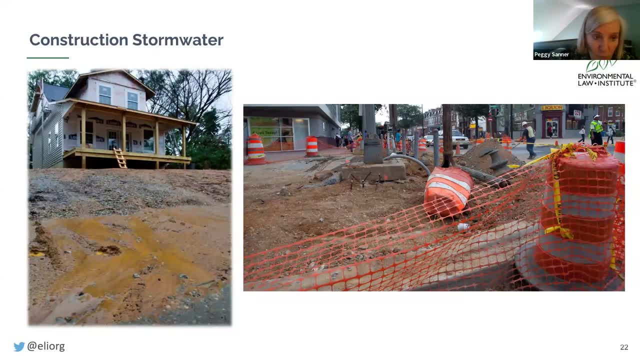 The construction activities were part of a common plan of development that, as taken as a whole, would be at least an acre in size, And so there was a permit that that's required for these construction activities to make sure that they were designed in such a way that once the permitting, once the 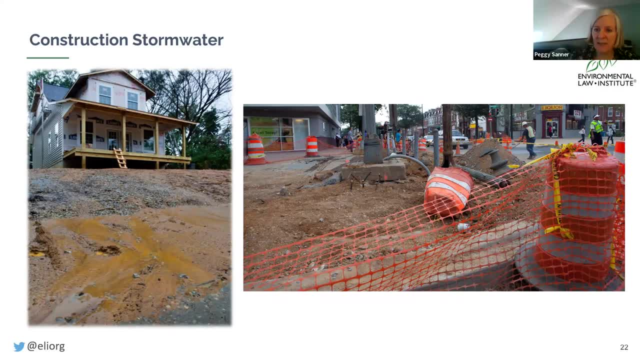 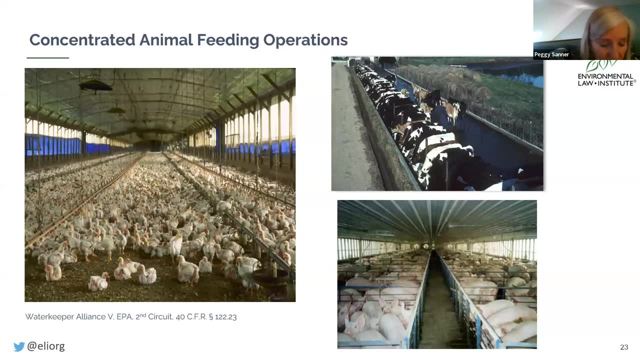 construction was done, the runoff would be as clean as possible. So that's also a point source. As many of you know, one of the largest sources of food in this country is our industrial agricultural operations- Poultry- this looks to be turkeys, I think. maybe chickens livestock in. 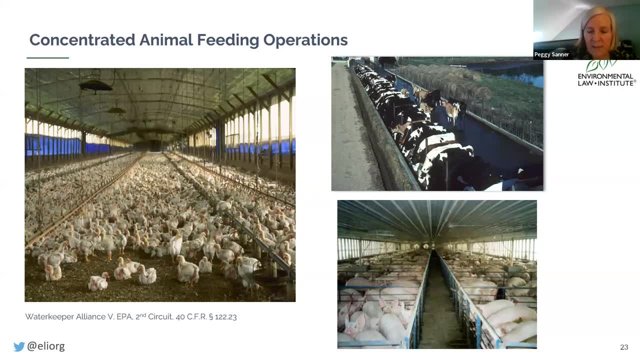 the top right and swine in the bottom right, All of those depending upon their size. if they reach a certain size, they can be used as a source of food, And so, as many of you know, one of the major producers is sweet potato. They are classified as confined animal feeding operations. 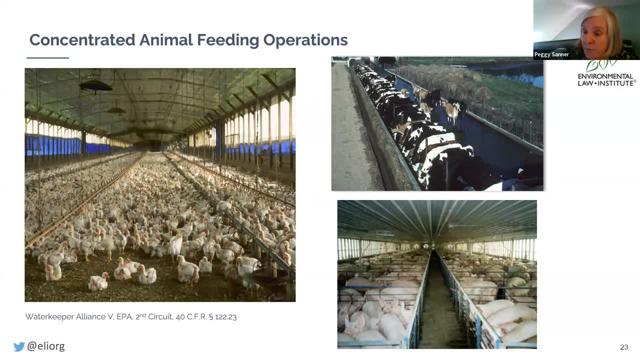 or CAFOs as we know them. These CAFOs can produce vast quantities of manure which is then used as fertilizer on ROCOP operations, And permits are required for those operations to ensure that the runoff from these fertilized- that will be, manure-fertilized- feed is great. 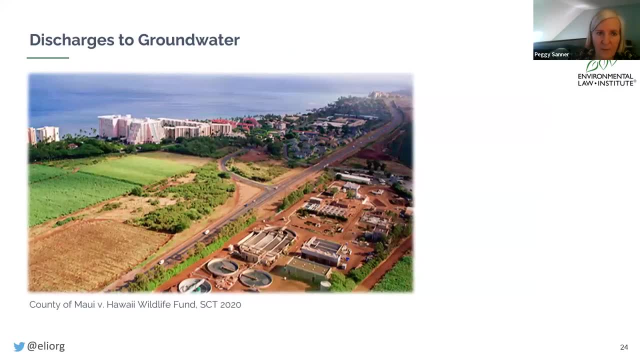 For example, this is a plant that we've called serine. We've changed the name to denso years are properly handled. Here's a one that honestly is pretty interesting and a relatively recent development: Discharges to groundwater. Under what circumstances can a discharge not? 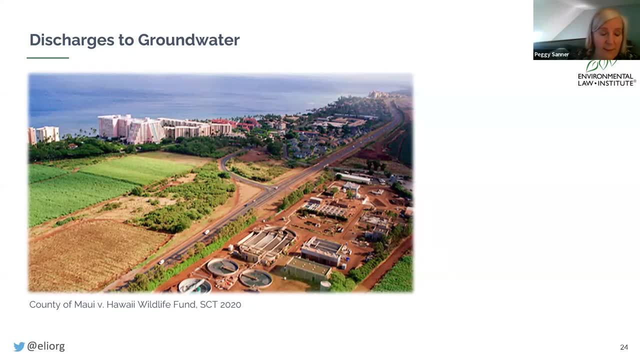 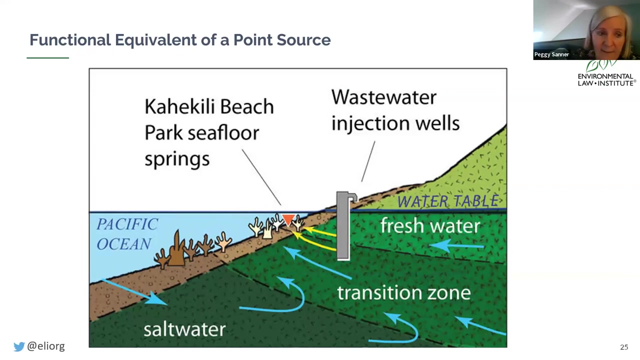 to surface water, but to groundwater be considered a point source. This arose in Hawaii. The county of Maui sued sorry reverse. ultimately, the Hawaii Wildlife Fund sued the county alleging that its system of disposing of partially treated wastewater was a point source and needed to be permitted. because the plaintiff said coral reefs were. 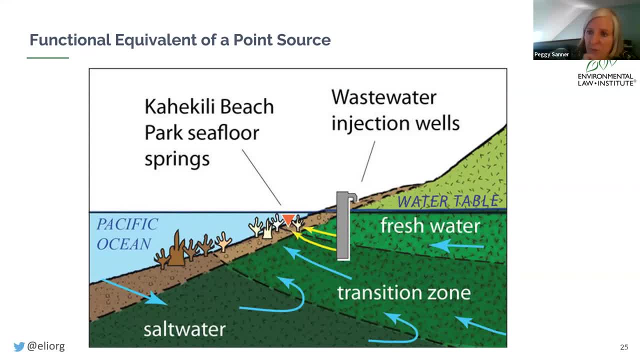 being hurt by discharge, And so, as the court evaluated it and ultimately this went to the spring court, the court studied what that process was. So we had partially treated wastewater that was injected into the groundwater by a series of injection wells that you can see in this slide, Deep in the 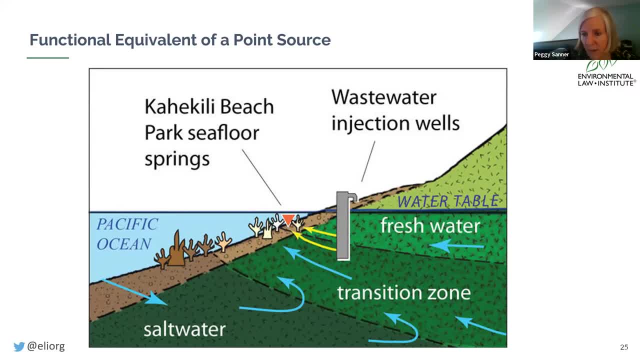 groundwater, that wastewater mixed with other freshwater and seawater that was found there, naturally And in a combined way. there's no doubt that the system of disposing of groundwater now contaminated with material from the wastewater injection reached the Pacific Ocean. The court found in what was a welcome decision. 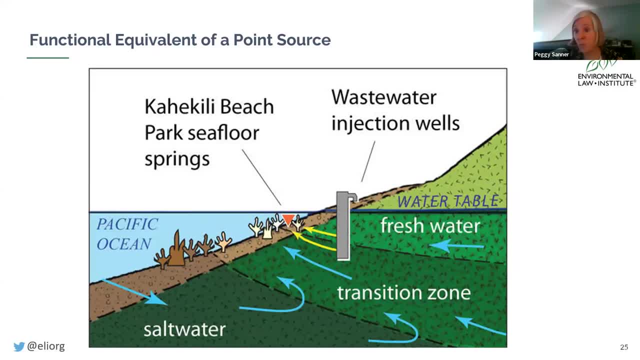 by many of us who care about waterways that this was a system that was the functional equivalent of a point source, because there was a conveyance that well, And the point source was a point source, So that led to the discharge of pollutants to surface waters in a way that made sense to the court. 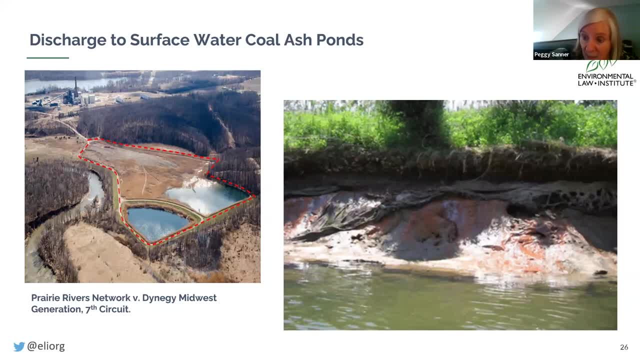 Now the court didn't say only this kind of injection system to the groundwater would be considered a point source. There are other situations where facilities do discharge a variety of kinds of wastewater to the groundwater and have claimed or are claiming to also be covered under this exception. 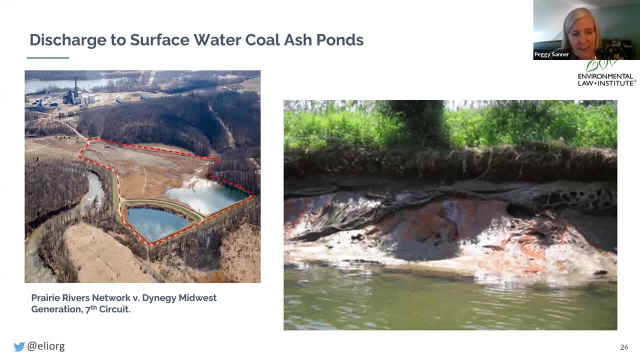 For instance, the arched ponds in the South Dakota- We see here pictures of a coal ash pond facility- and Midwest. This is a pond where an energy- coal fired- energy generation facility has coal ash as a waste And stored in ponds for a while, ultimately before dewatering and disposal. 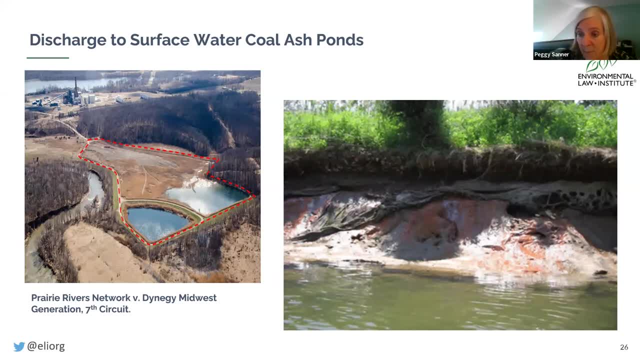 But the the liquid in the pond is filled with chemicals like arsenic, boron, etc. There are a number of sources of the information that i haven't taken any more words about- and selenium, all of which are deleterious chemicals and which can be found certainly. 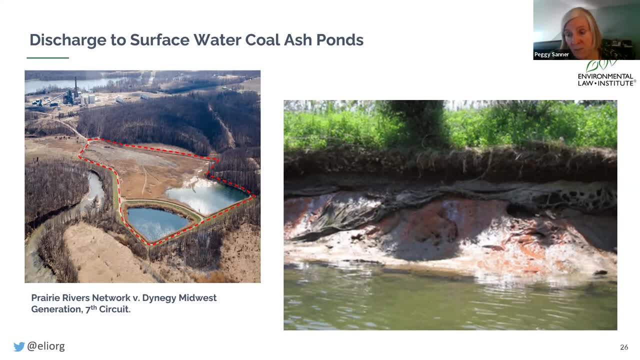 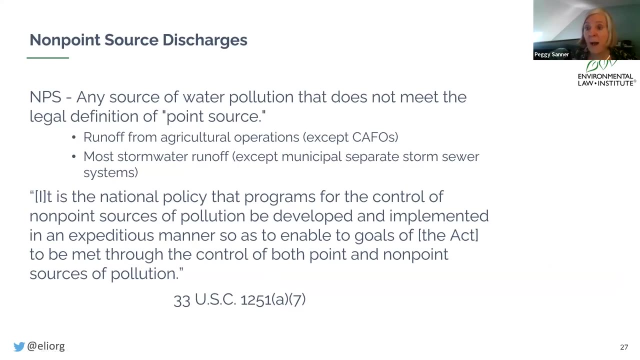 were alleged to be found in this case, And we know of other cases where the courts have found that those chemicals reach the surface water via this groundwater system. So certainly we'll raise the question whether or not they will be considered point sources. Okay, I have talked. 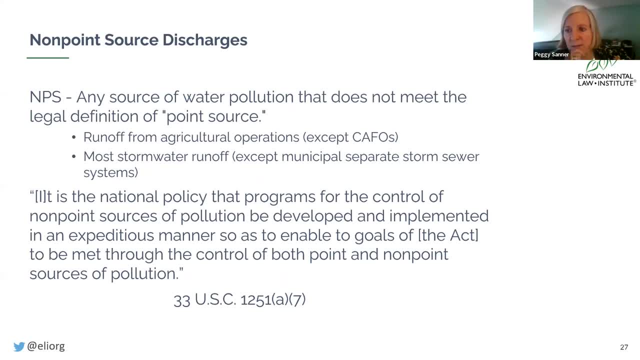 about a variety of point sources. There's- there are several, there's many others that we could talk about, but you see, it's a very large world of facilities and operations that require a federally authorized permit, the NPDES permit to control pollution discharges. But that's not all. 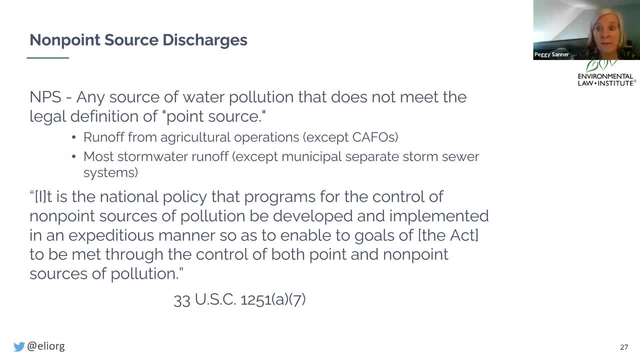 We have the world of non-point sources And in effect these are any source of water pollution that does not meet the legal definition of point source- Again, pretty, pretty broad, not too many boundaries there. but two non-point sources are the ones that receive most and very deserved attention. One is agricultural operations. 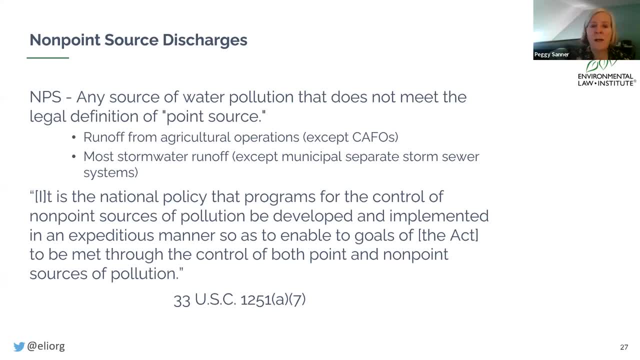 leaving aside the animal operations I mentioned And the closed water works, as I mentioned a moment ago, but also most storm water runoff, And they are. the Clean Water Act mentions them and notes that it is again the national policy that programs to develop and programs should be developed to control and reduce pollution. 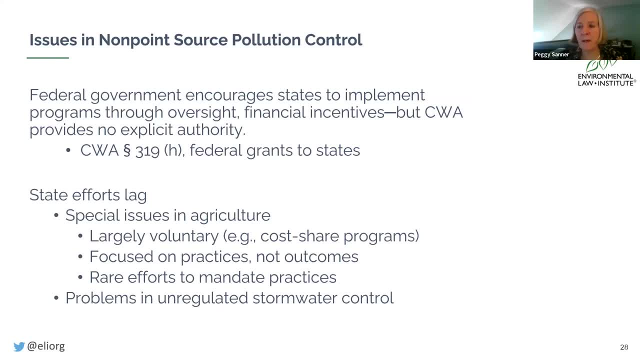 from these sources as well as point sources. So we have to think about what the states are doing, hopefully with and often with the assistance of the federal government, through the grant programs and other programs that Camille mentioned. So how are the states doing? I would say the answer is mixed And I'll just shine a light for a moment. 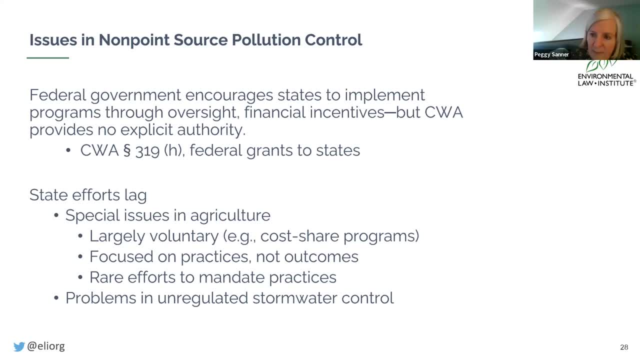 on agriculture. Probably many of you in this audience come from families who do agricultural work or know people who do agricultural work. A really important segment of the economy and, frankly, our ability to survive as a nation, as a race. Farmers are typically we have found in our 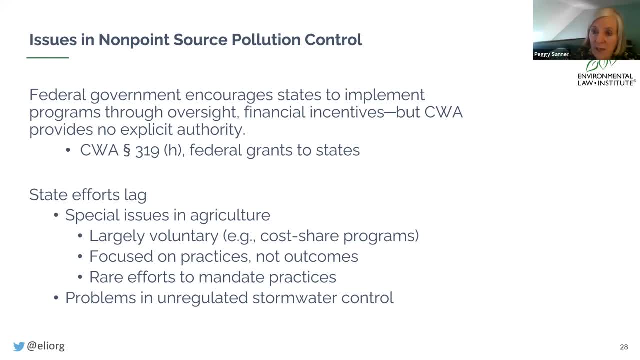 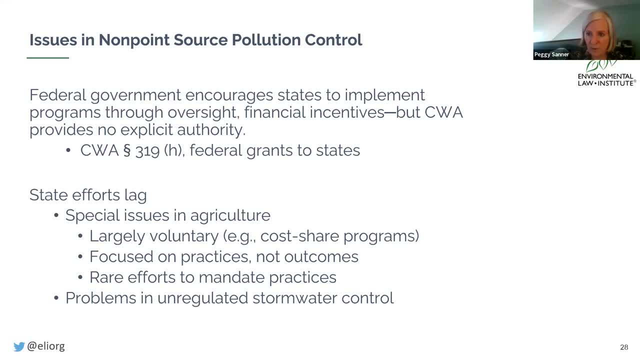 water, And so state programs addressing agriculture by and large are voluntary in nature. Farmers can sign up if they want. They can and do consist to a great extent of programs to provide money, either a percentage or a, in some cases all the cost of putting a practices on the ground. 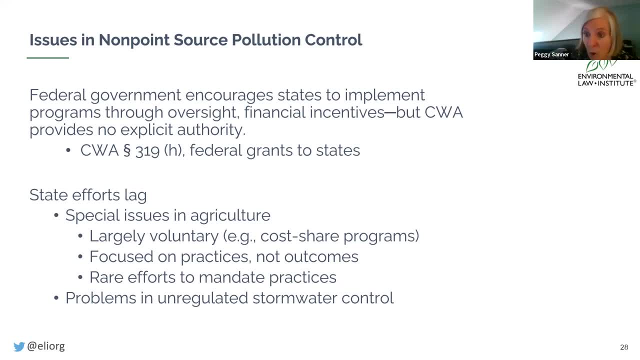 that stem, or are hoped to stem, the runoff of polluted water from agricultural fields, And these can be a wide range- I mean in Virginia more than a hundred- but they include fencing cattle out of streams to keep their feces on the land and useful for fertilizer purposes. 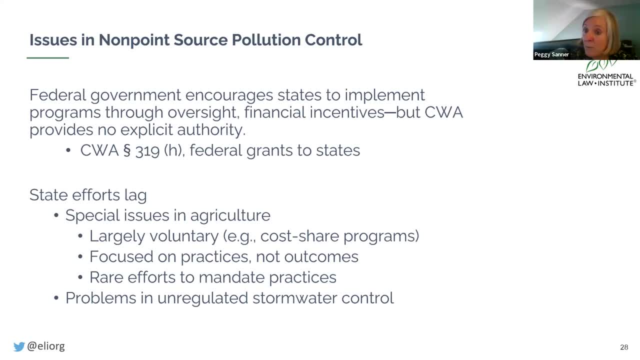 Planting riparian forested buffers, Planting cover crops so that you don't have a bare exposed soil Soil for many seasons of the year. The list goes on and on. What is characteristic of these programs to the present, however, is they focus on practices and not on measured outcomes, And so 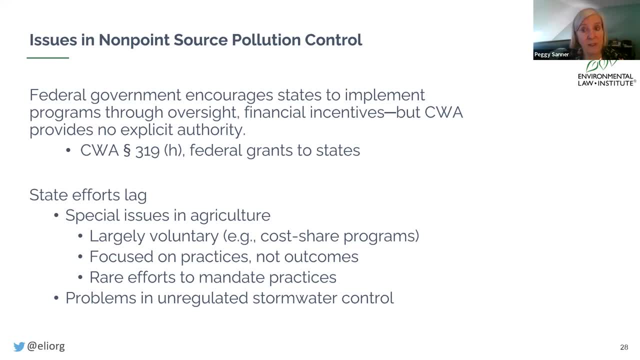 these practices, in effect, are very different from the point source. practices that are directed by the Clean Water Act, Agricultural programs, um, that are directed by the states, very rarely include any requirements, any mandates. I will just give you one example of one that we're familiar with in Virginia. There is 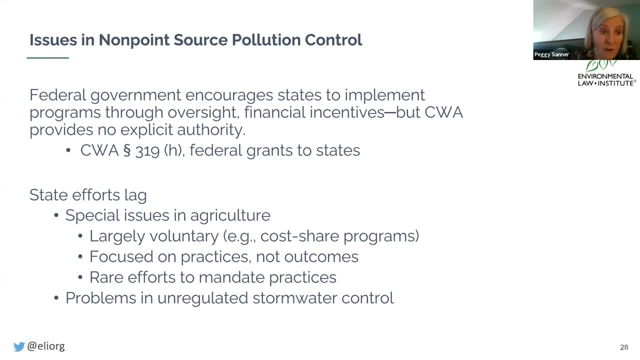 some legislation that requires farm operations with a cattle of a certain size to fence cattle out of streams, with an effective date of several years in the future, And I will just say that the date has just been postponed for a variety of reasons And I'm aware of another state. 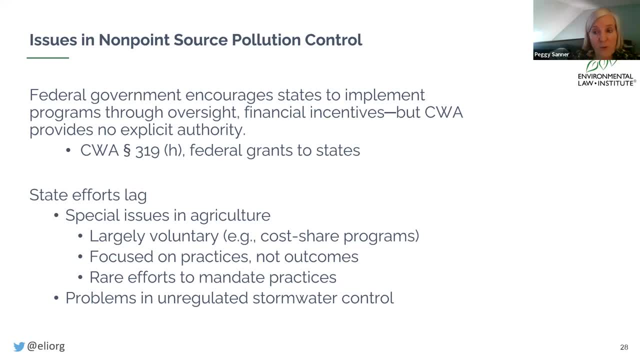 Pennsylvania, which has a specific law on the books which prohibits localities, municipalities, from requiring cattle to be fenced out of streams. So we have lots of experimentation going on, lots of efforts, but we haven't made the same kind of progress as on the nine points. on the points, So, uh, we have lots of experimentation going on, lots of efforts, but we haven't made the same kind of progress as on the nine points on the points or side. So, uh, we have lots of experimentation going on, lots of efforts, but we haven't made the same kind of progress as on the nine points on the points or side. 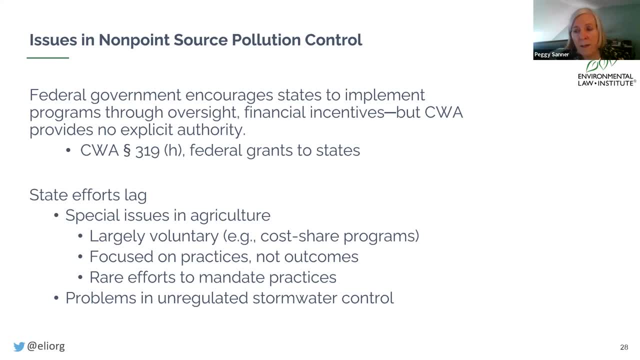 Unregulated stormwater. Think about this, Think about a suburban community, anyone that you might think of, where rain hits the roof goes, from the roof to the driveway, to the street or to the sidewalk. It picks up temperature, it picks up speed, it picks up pollution. 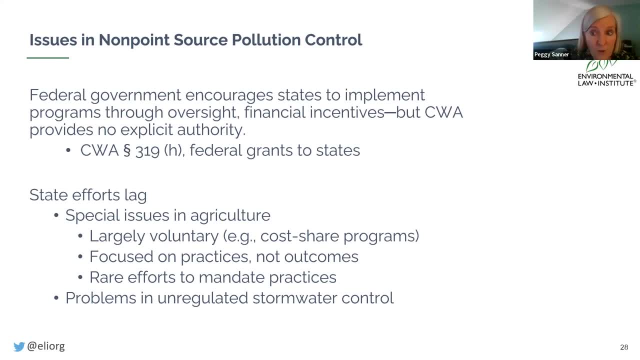 goes into our waterways. That is, largely speaking, unregulated stormwater, meaning very few controls. There's one exception: Municipal systems to collect stormwater usually are under a point source permit, but it's very difficult to control or to reduce pollution from unregulated stormwater. 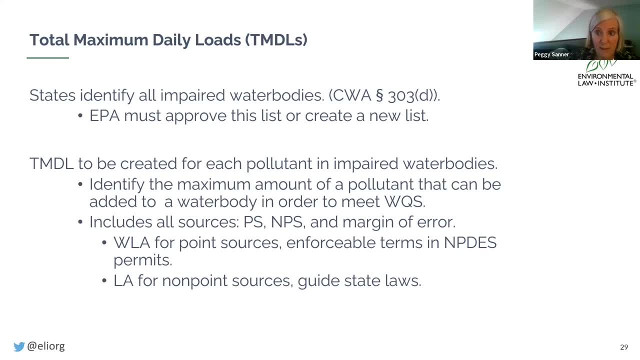 So now that you know all there is to know about point sources and non-point sources, the question arises: what happens? how do these programs work together? Camille mentioned that states are required under the Clean Water Act to identify all of their impaired streams, all the waterways that do not meet water quality standards. 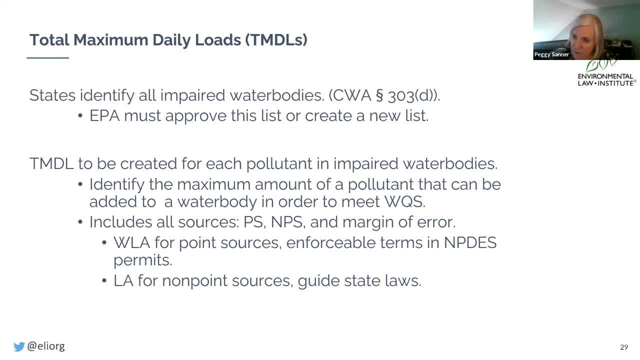 that are polluted, And so for each of those streams, the state is obligated to develop this terribly cumbersome term: total maximum daily load. we call it a blueprint. this blueprint is to be created for each pollutant that makes a waterway impaired. 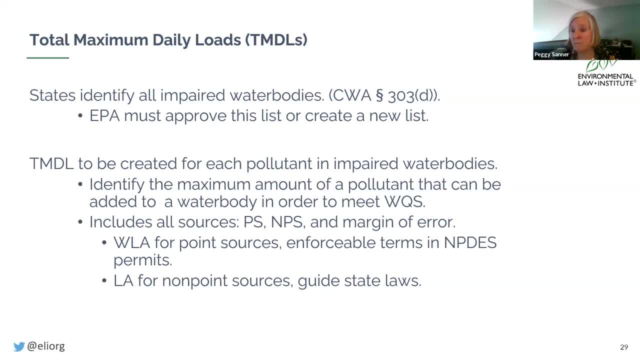 So it might be for nitrogen, it might be for phosphorus, it might be for sediment. you have a different TMDL for each of those, And the idea is it identifies what comes from the point sources, what comes from non-point sources, assigns responsibility to point. 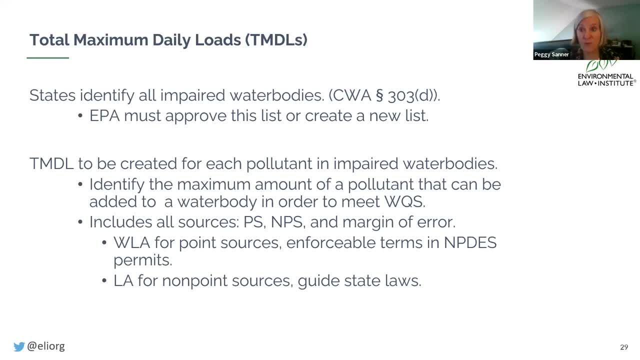 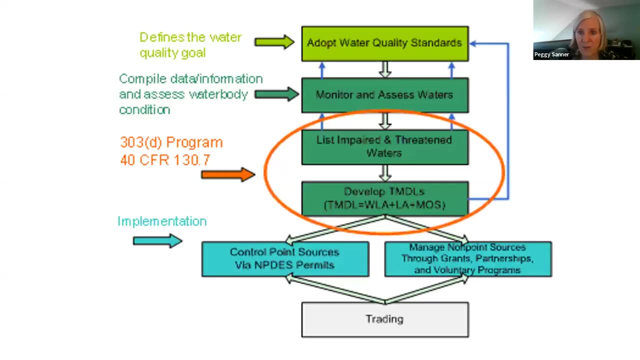 sources and to non-point sources to do things to reduce that pollution so that ideally, in the end the reductions are such that the water is returned to water quality standards. So that is the theory. just a little diagram to show the elements of this. 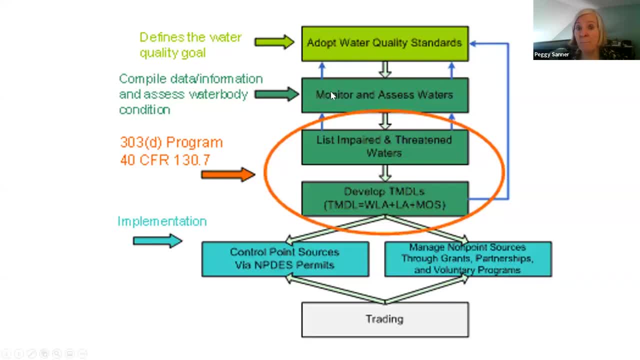 The state adopts the water quality standard. the state then monitors and assesses those waterways, which ones are polluted or impaired. They go on a list. EPA looks at the list, says it is or it isn't okay. If it is okay, the state is then charged to develop one of these TMDLs that takes. 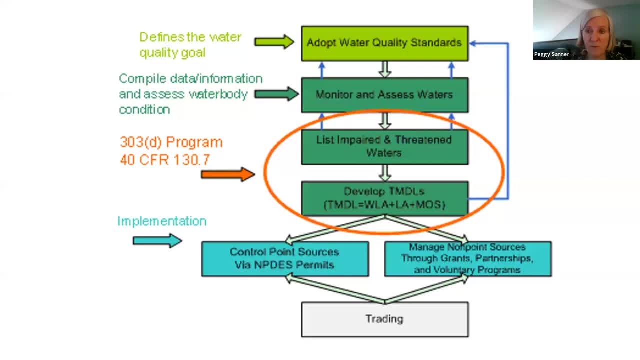 into account point source pollution, non-point source pollution, and that's a little bit of an extra piece just to make sure that everything is taken into account. So, theoretically, that is how we are taking account of what comes out of point sources and what comes off of the land. 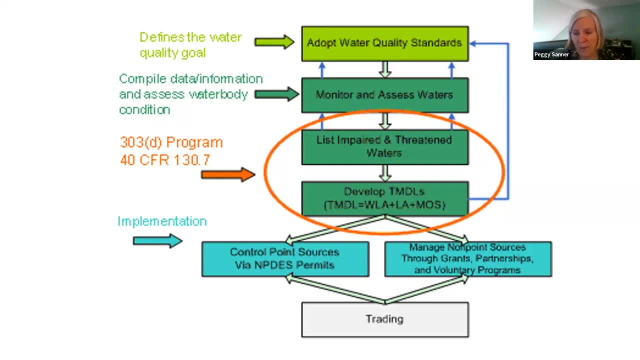 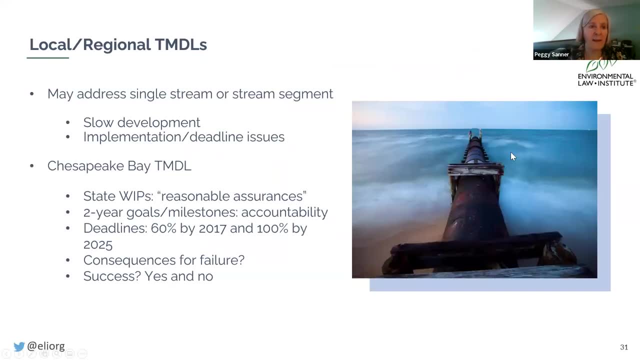 and non-point sources and we're going to end up with clean water. There are problems associated with this system. I'm sure you're not surprised at that. There are TMDLs, or blueprints that states across the country have been developing. hundreds of them, probably thousands of them. 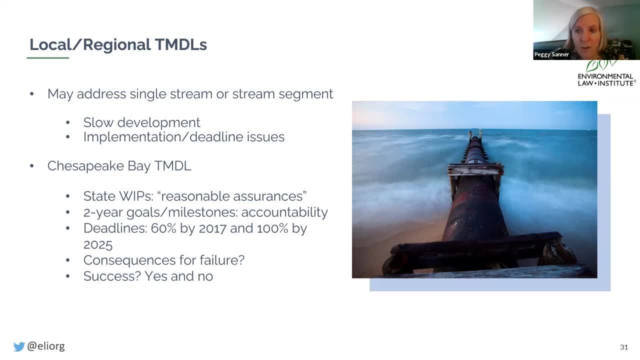 To my knowledge, virtually all of them address not all, but many of them, most of them, address a single stream at a time or a stream segment, even a part of the Potomac River, for example. They largely do not have a deadline for any of these activities. 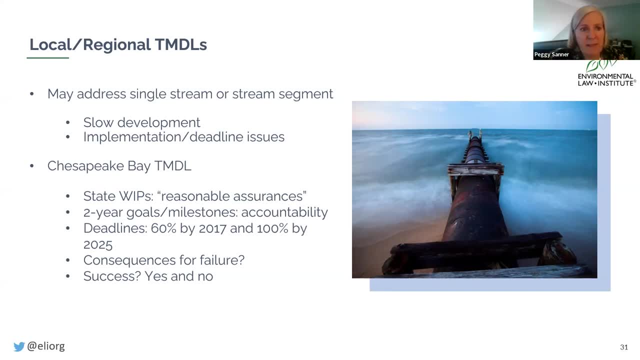 They take a long time to develop and the enforcement mechanisms, particularly on the non-point side, are pretty limited, if they exist at all, And so the examples of success, a successful completion of returning a waterway to a restored condition, are very, very welcome, and they're certainly not as numerous as we would all hope. 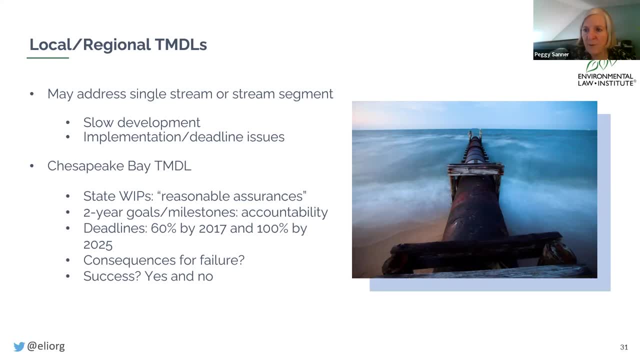 I just wanted to turn your attention for a minute or two to a regional TMDL that we've been working on for a number of years. I'm going to turn it over to you. I'm going to turn it over to you. I just wanted to turn your attention for a minute or two to a regional TMDL that we've been working on for a number of years. 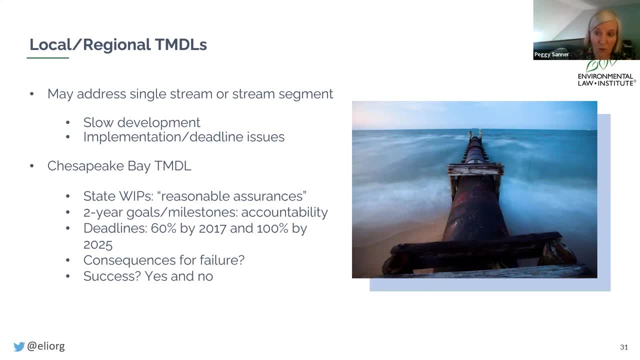 And that addresses the Chesapeake Bay as a whole. As Camille mentioned, there's seven jurisdictions, six states and the Washington DC area. Those seven jurisdictions partnered with the EPA to develop a new TMDL to address the whole region And they did that after. 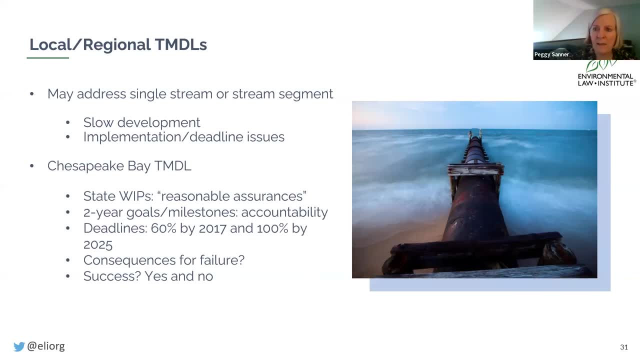 years of efforts, singly and in collaborative efforts. that did not work. So they agreed to put together this TMDL that addressed three pollutants- nitrogen, phosphorus and sediment- And it told each state each one had to reduce its levels of pollution to the Bay by a certain 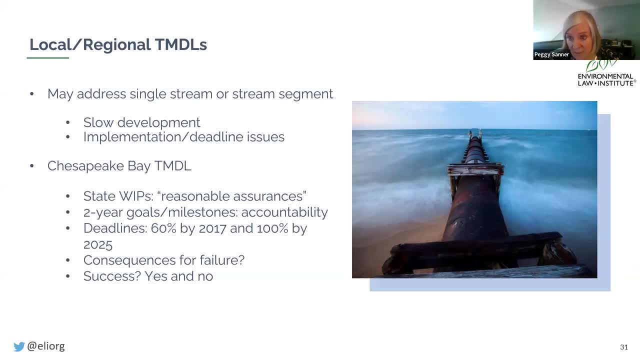 percentage States had to develop plans to achieve that goal. There were milestones involved, There were deadlines- one of them- the big one- coming right up in 2025. And there were some consequences if the goals are not achieved, And I would say we have now. 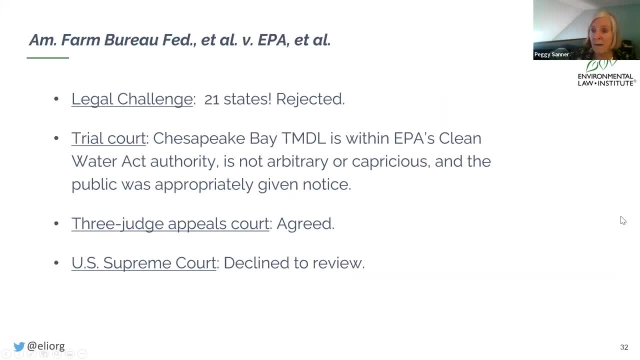 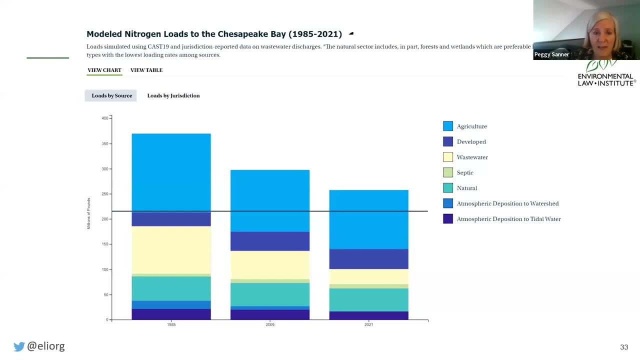 as we're nearing 2025, some great successes from this program, particularly on the land side. I need to skip ahead here. This is one of many charts, graphs that you can see that point out both its successes and its failures, And I'm going to turn it over to you, Camille. 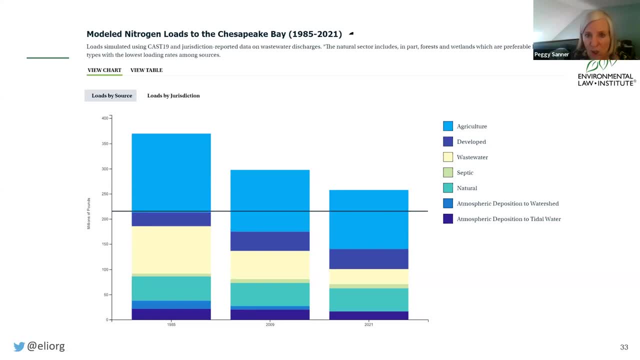 And it's big challenges. The large light blue block in each column is agriculture, In other words, the chunk of the pollution load to the Bay. it comes from agriculture And the yellow is the chunk of pollution to the Bay coming from all the wastewater facilities. 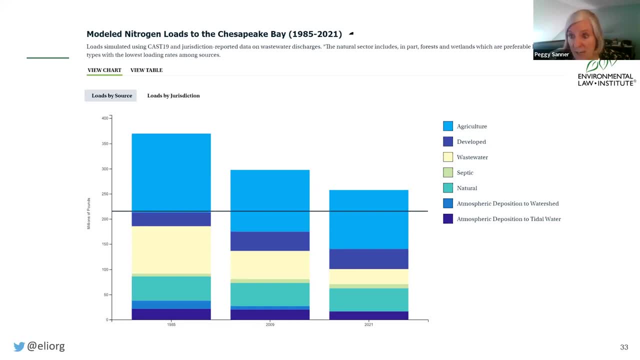 And if you look at the middle bar, that's 2009, when our program basically started, And on the right-hand column is 2021.. You look closely you can see that the block representing wastewater diminished considerably And that's certainly an accurate representation. 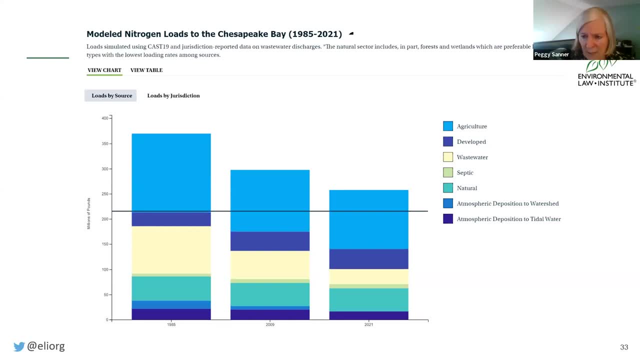 of what we have seen. We see some, really. I mean, the Potomac River, for example, was kind of like the Cuyahoga River when some of this process started, And it's seeing a remarkable renaissance right now. 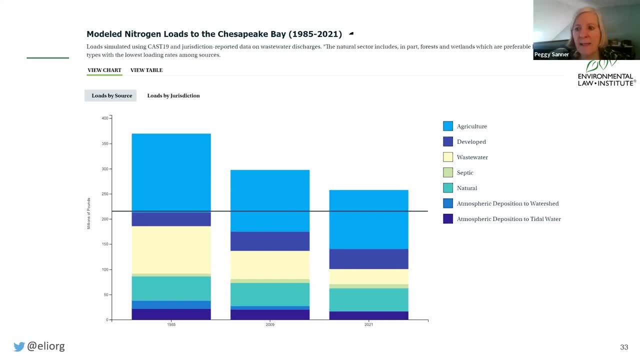 The blue area very stubborn, It continues to provide a very large chunk of the pollution. Lest you be disheartened by this, keep in mind that the region at issue, the 64,000 square mile area of the Bay, has seen a dramatic increase in population. 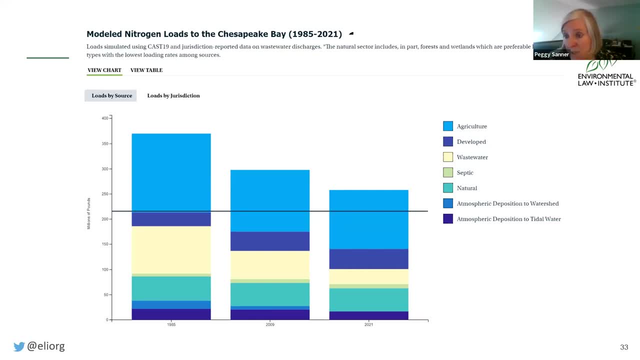 in the same timeframe And we have not increased pollution from our agricultural sections. So there's success, just not as fast as we would like. And I just one last point that I mentioned before I turn this back over to Camille, and that is: 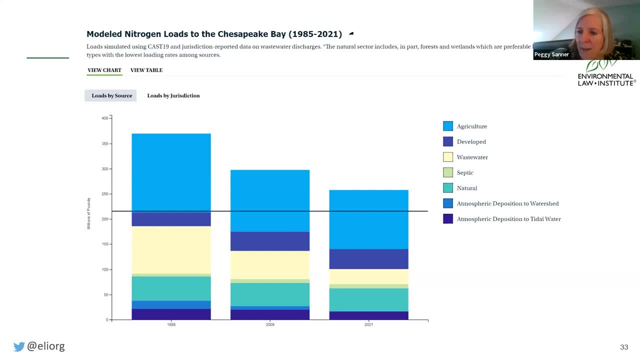 it is helpful, I think, to all of us working in the environmental area that this particular regional TMDL was upheld by the federal courts as being consistent with law and well within the authority, And so what I would like to ask you to do is 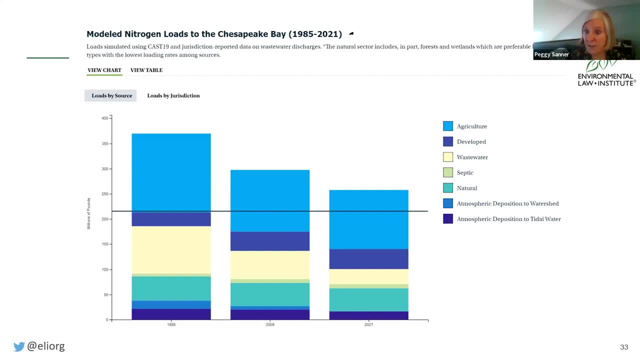 as we look at the historic area and the areas we just touched on, is to give the opportunity to discuss about the individuals- the individuals who are living in the community- granted to a VPA to participate in. So I'll leave it at that and hand it back over to Camille. Thank, 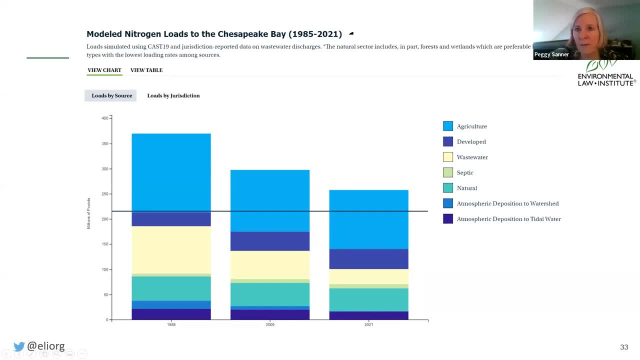 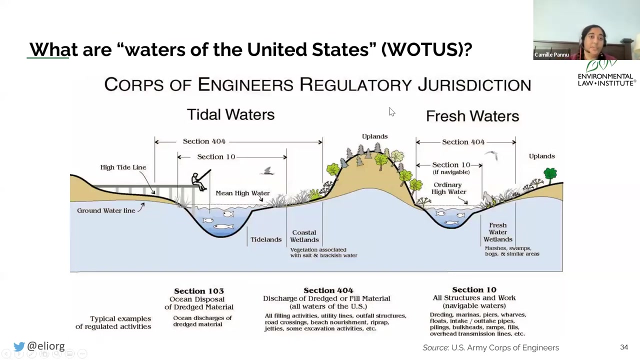 you. I was on mute, Thank you. So we're going to keep rolling, There we go. So there was a question a little bit on the chat on this where it asked if navigable waters also covers It advanced. without me wanting you to, Here we go, Navigable waters, or if the Clean. 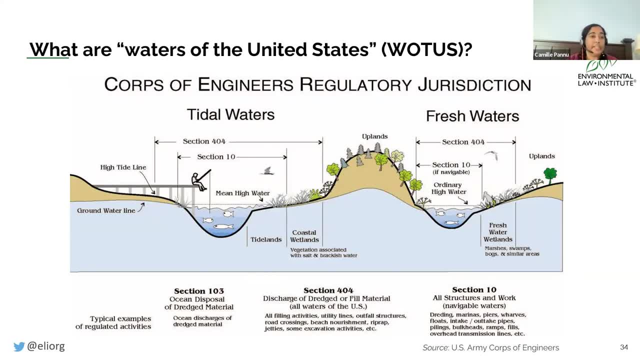 Water Act covers waters that are not navigable, I guess, is a better way to frame it, And so the answer is yes-ish. This is a bit of a moving target because of the Sackett case that just came down, But I thought that this visual is very helpful. This is specifically: 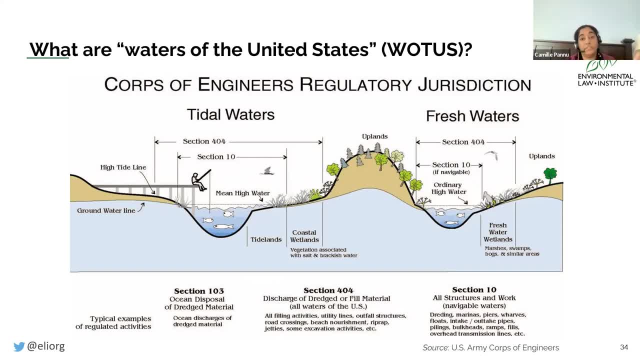 about the Section 404 program, which is generally for the Army Corps of Engineers. So EPA has kind of lead authority, or is the lead agency, on things like TMDLs, the MPDES permit system etc. But another critical part of the Clean Water Act is focused on infill and dredging. So are you sucking? 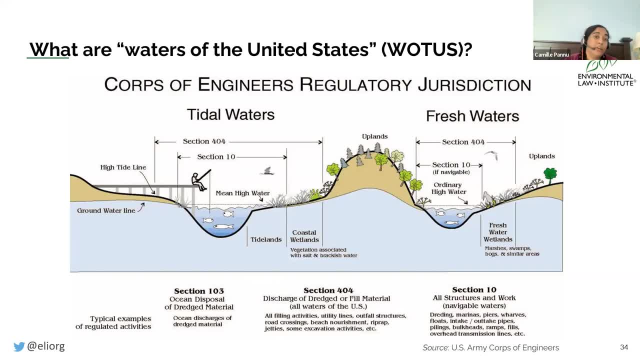 stuff up from the bottom of a water body or are you infilling by putting rocks and other kind of dirt into an area, Or perhaps other items? And so this is how the Act- this is a visualization of how the Act- talks about jurisdiction over waters. So, generally, the Clean Water Act, in addition to covering 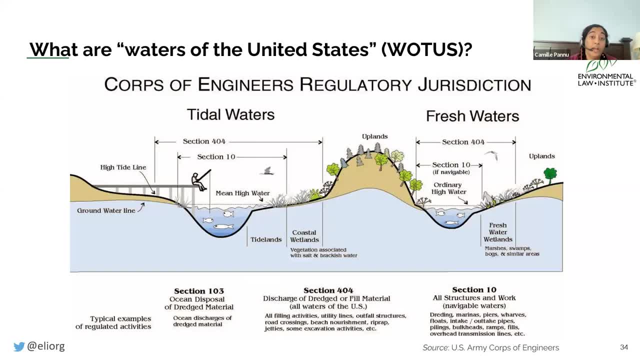 navigable waters also covers coastal wetlands. It goes up to the high water line, the ordinary high water line and the average high tide water line, And it includes tidelands. for sure, If you are not a navigable, you might be covered under the Clean Water Act if you are part of a navigable. 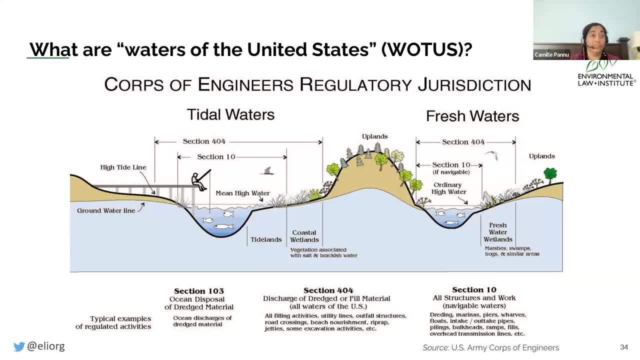 water system. So County of Maui, I think, was actually a really good example of that. right, You had discharges to groundwater but groundwater is, by definition, not navigable. You cannot like run a canoe down a groundwater system, But it was connecting with a navigable water source. that was. 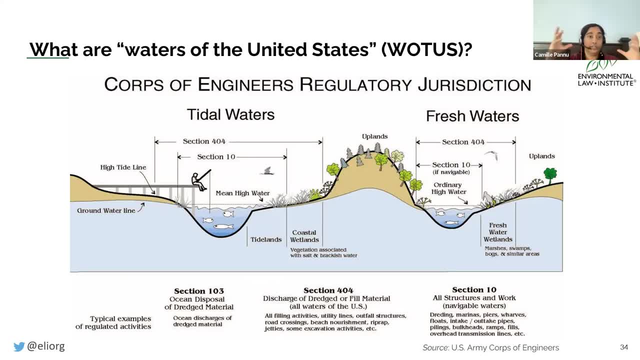 part of the waters of the United States. So waters of the United States has been interpreted to include water systems in a very different way than just navigable waters. The reason that folks use navigable waters in the Act and talk about that is because of the authority under the Commerce. 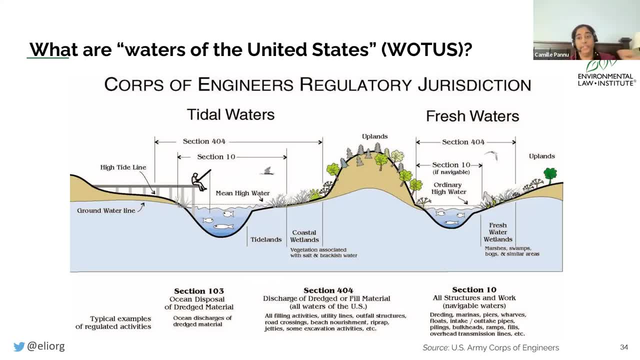 Clause of the Constitution. So they're kind of calling back or signaling to a line of cases that is talked about, specifically federal authority over navigable waters. But as a practical matter the courts have understood and Congress has established that when we have these water systems, 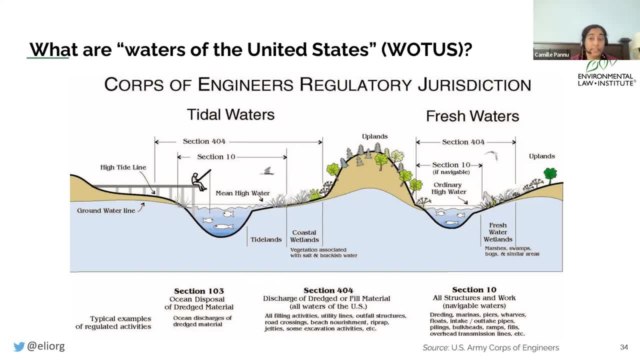 with tributaries, they're not going to be able to use navigable waters. They're going to have to be able to use them in a way that is not a water system, And so the point is, you can't just put a. 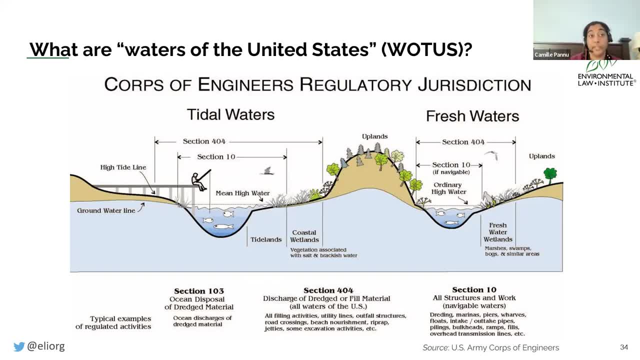 boat on a creek. you can't just put a boat on a stream or a creek- which you can't necessarily put a boat on necessarily, depending on its size, But it could still be a waterway that is subject to Clean Water Act regulation, particularly if it's going to fill into a navigable waterway. 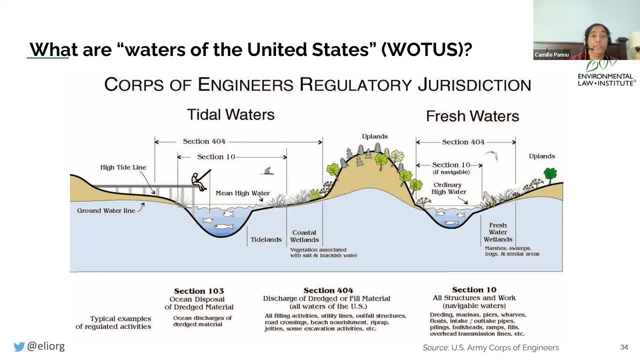 If it doesn't have that connection to a navigable waterway at the end of this process, then it would be a waterway that would require an additional or more technical explanation. So, as you can imagine, that requires a little bit of scientific work as well to kind of set up what. 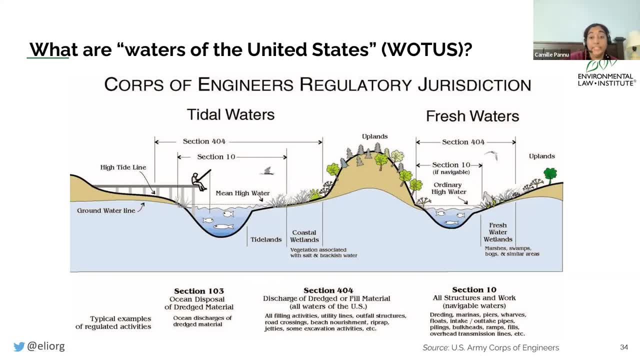 the hydrology systems are for each of these different waterways that are protected and how that works. So this becomes important because wetlands, which exist both on the coast and inland, are critical for the environment and are explicitly covered and explicitly mentioned several times in. 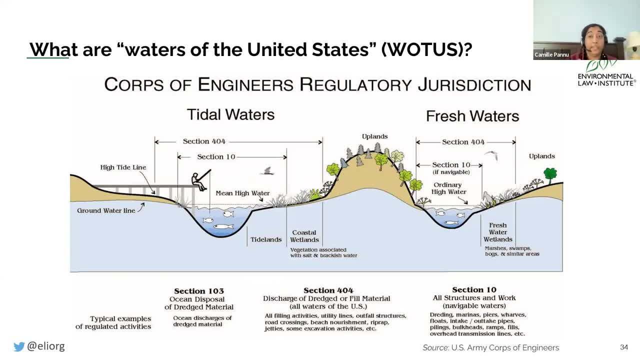 terms of the state's ability- the state meaning like state government's ability- to work with the federal government on these infill issues and other issues that might require special permitting. Wetlands are always kind of popular for development reasons, Depending on where you've. 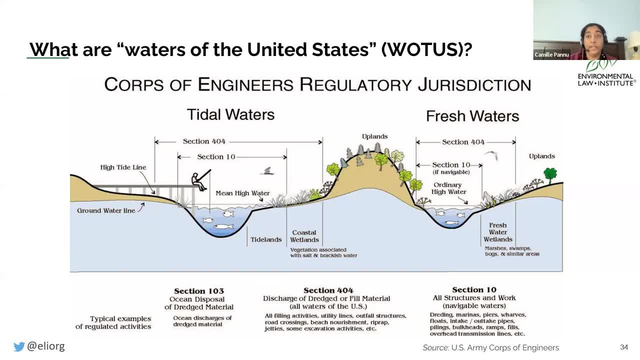 located. that could be because there's offshore drilling opportunities for oil. It could be an effort to expand or extend land so that it can be developed for like commercial or residential enterprises. A lot of parts of the country infilled their wetlands prior to the Clean Water. 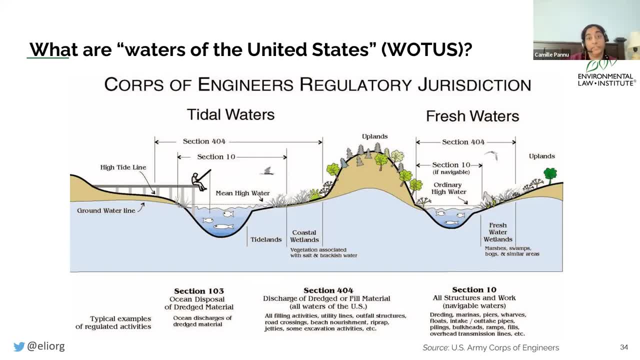 Act being put into place, And so this was an active effort to preserve our wetlands, which are really critical ecosystems that also are essential for flood control and water quality management, in addition to the biodiversity that they provide. So, Waters of the United States, or WOTUS. 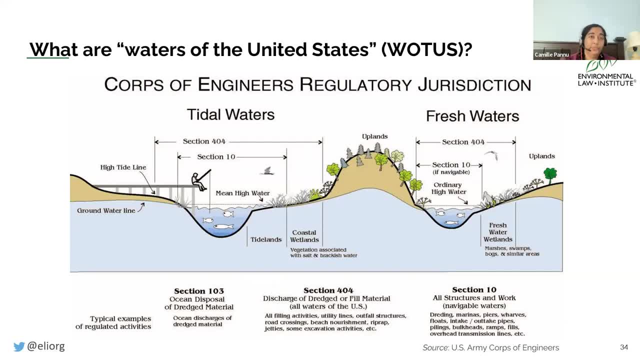 Technically, the phrase is relatively broad In the statute, which usually means that the agencies that are in charge of applying or implementing the statute get first shot at defining what that means. So EPA and the Army Corps of Engineers worked collectively to define WOTUS. There's been some back and forth, So 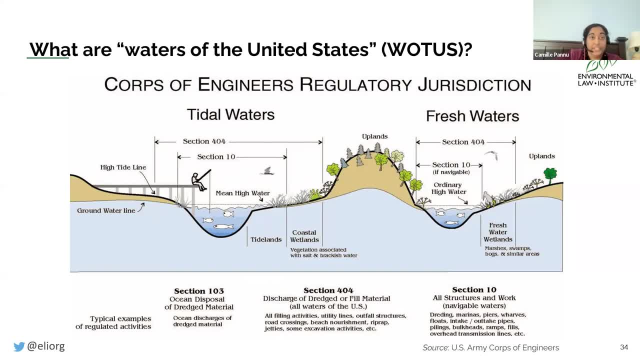 there was a WOTUS rule that came out under the Obama administration. It was not finalized, And then the Trump administration tried to redo it and scale it way back, And then the Biden administration came in and reestablished it, And then the Trump administration tried to. 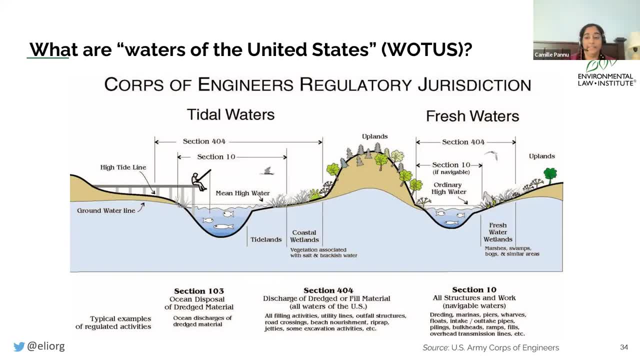 reestablish the broader definition. And then we had SAC-IT. So when we talk about waterways- I think one of the things I'm going to tee this up so we can talk about SAC-IT and a little bit- But one of the things to keep in mind is how we think about. 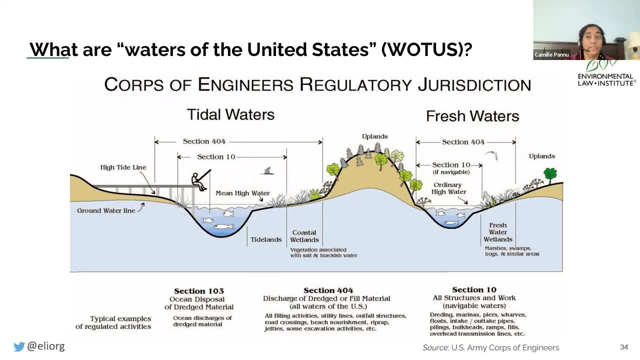 water in the east versus the west. So for the most part on the east coast rivers don't go dry. Rivers consistently flow, they may be diverted, they may have canals, they may have other infrastructure built on them, But areas that are wet and lakes that are wet tend to remain wet. That has changed recently with. 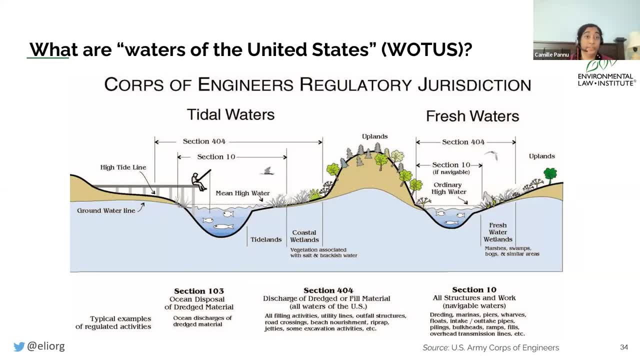 climate change, We saw like historic droughts in areas that are considered to be historically very wet, including parts of New York, the Great Lakes states, etc. But historically prior to like kind of the climate change moment we're seeing right now, the east has been wet and the west is very. 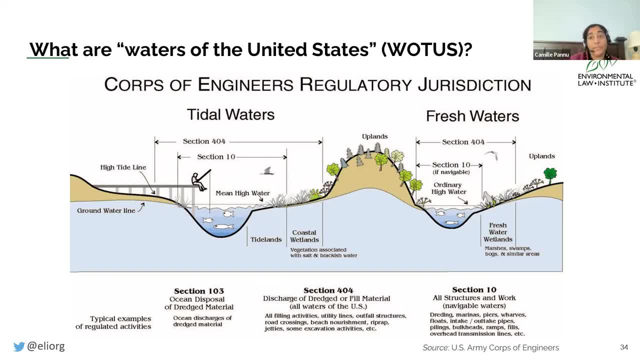 dry. So once you cross the Mississippi, groundwater becomes really critical, but also surface water becomes less reliable. So I wanted to show a couple of images to talk about, to show examples of waters of the United States that might not occur to us as waters of the United States. So 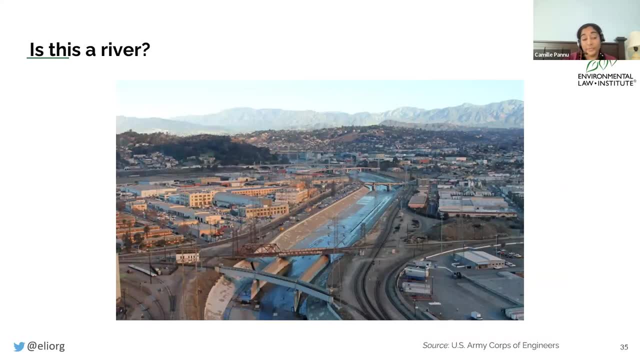 this is a photo from the Army Corps of Engineers, And so my question is: is this a river? So you may have seen this before. This is the Los Angeles River, which has been lined in concrete that Hollywood actors have filmed scenes there, And it's very rare to see water flowing through the. 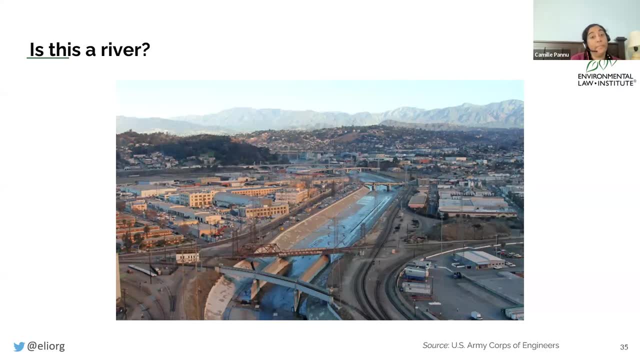 river anymore. There's a multi-year restoration project going, but this was a river that flowed naturally And it no longer like. you can't put a boat on the water ponds that you're seeing or the puddles you're seeing here in the like concrete bed. However, if you talk to any 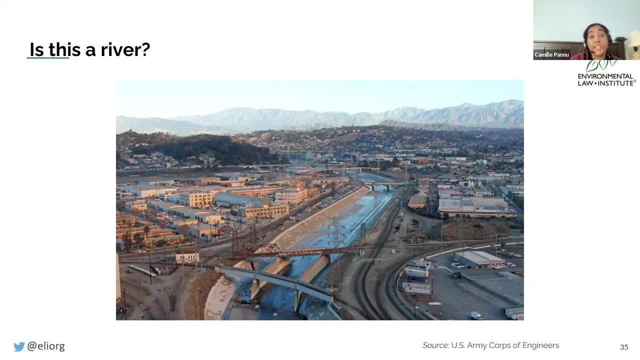 Californian, certainly any Angeleno- they would tell you that's a river And they would tell you that it's a river. And they would tell you that it's a river And they would tell you that it's an interstate river or connected to an interstate river system, And this is part of the waters of. 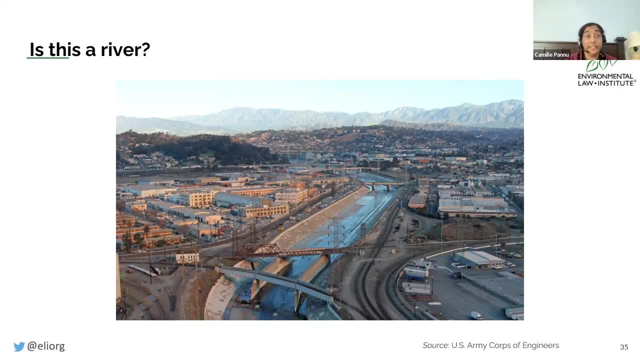 the United States, And it is. it's subject to the Clean Water Act And what we do with it- whether we fill it in or we don't fill it in, et cetera, whether we restore, it is covered by the Clean Water Act. But I think it's really interesting because it's really typical of the 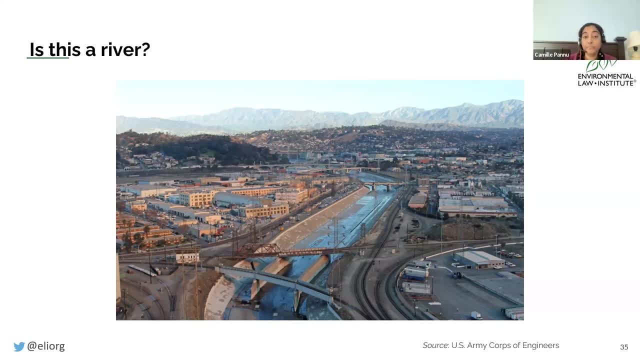 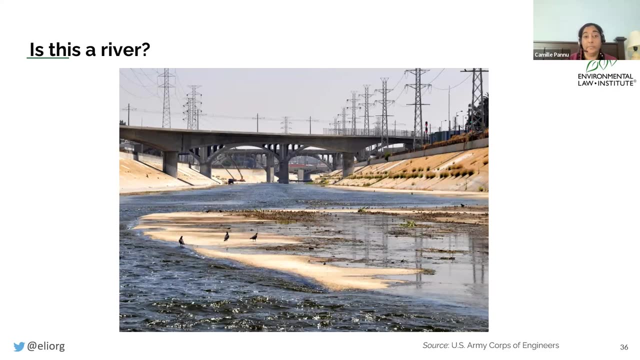 West, where you can have a river and the river might not flow. This is another example. This is also the LA River, So you can see just how shallow it is, even when there is water. Recently it's been flowing. I saw a video that showed like water in the LA River and I was 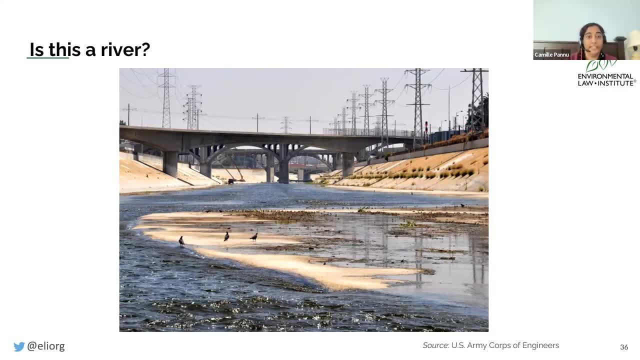 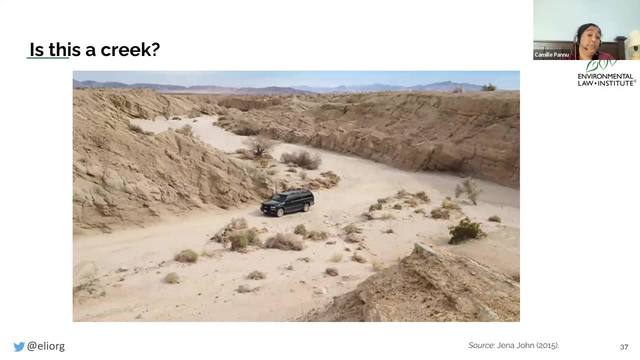 shocked. I've lived in California for over 35 years and I had never seen water flow in the river before. So my question with this photo is: is this a creek? So this is an arroyo, which is a Spanish word for a wash or a floodplain. It specifically refers to tributary creeks that are often dry. 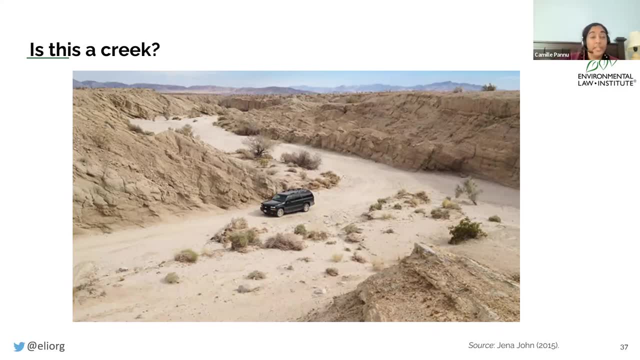 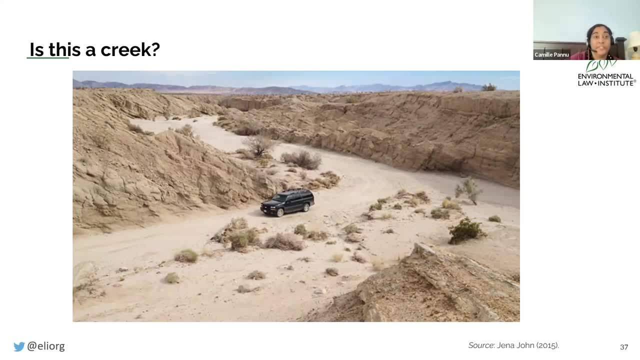 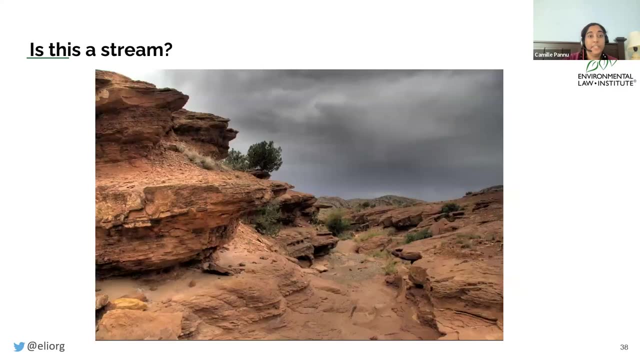 when there's rain. If you ask any person who lives in this region, they will tell you this is a creek, even though you can't see water, And they will say that it should be protected by the Clean Water Act. And this is another example. This is from Arizona. This is another arroyo. You can't. 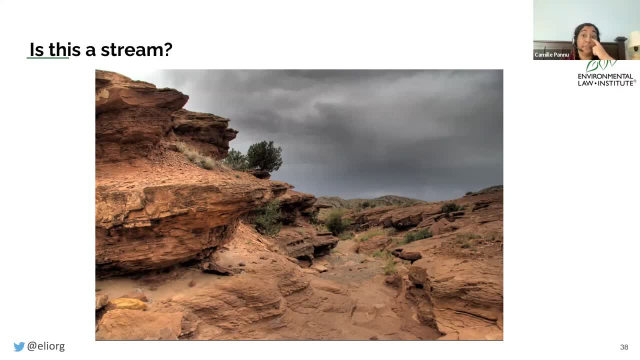 unless you know what you're looking for, you might not even see the bed where it flows, But this is a tributary river or stream to the Colorado River system And so, again, you know it's important for us to consider where the Clean Water Act is being applied and how it's. 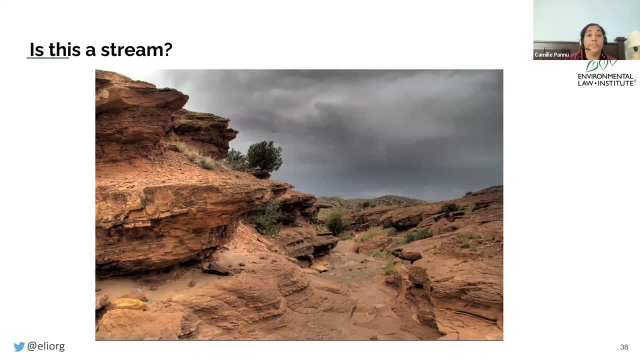 being applied and how we think of water flowing. Certainly, if you have water coming through the arroyo- which you will, as you can see from the storm clouds- it's about to flood any moment, Once you start getting water flowing, and flowing into these Western water systems in particular. 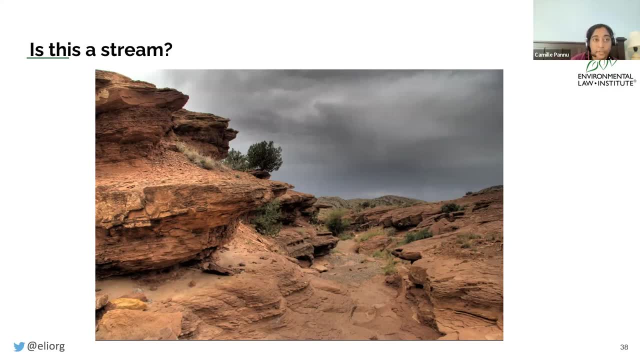 it's important for us to think about what's being put in the arroyo and how the arroyo is being used, Because it absolutely affects the water quality of the Colorado River for the other major rivers that flow out of that system, And in the Southwest a lot of surface water looks like this. There are 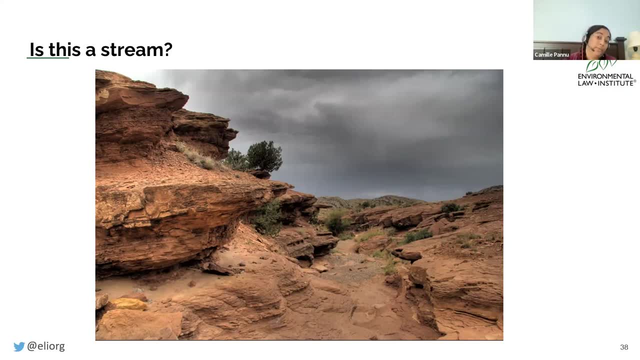 lakes that go dry and then you know they come back. So you know query whether that's a navigable water. Until SACET there was no real kind of majority opinion in the Supreme Court, And so states were kind of filling in the blanks and regulating a lot of this. Some of them will. 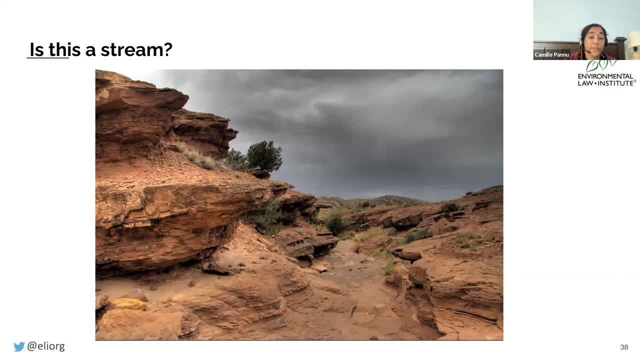 continue to regulate it, But I think there's going to be a lot of work to be done to make sure that there's going to be some fighting over whether the Clean Water Act covers these kind of- quote unquote- dry rivers or dry streams that are intermittent or that come in when there's major water events. But 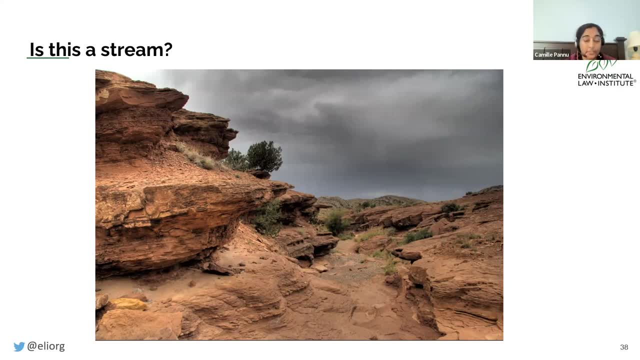 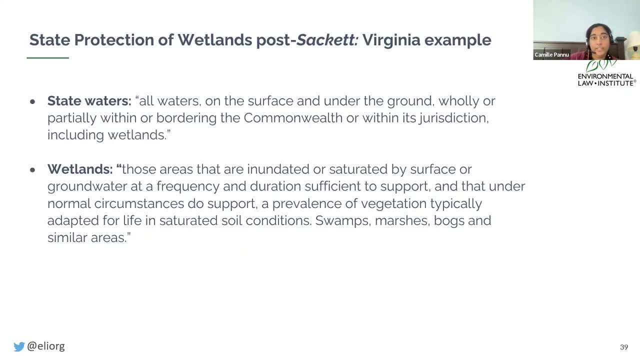 I would argue that the ecosystem of the desert is different than the ecosystem of the East, where it's much more lush and much more wet. All right, So I'm going to turn it back to Peggy to talk about, or to Corey, I think, to talk about. 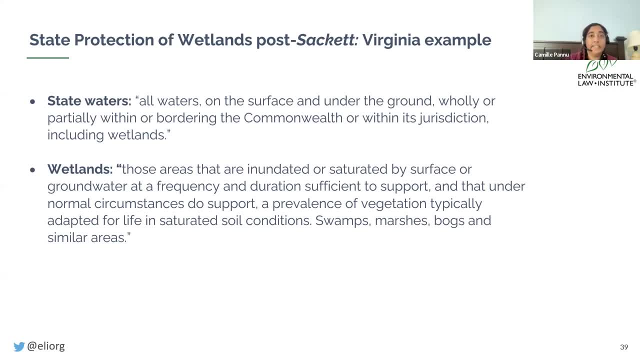 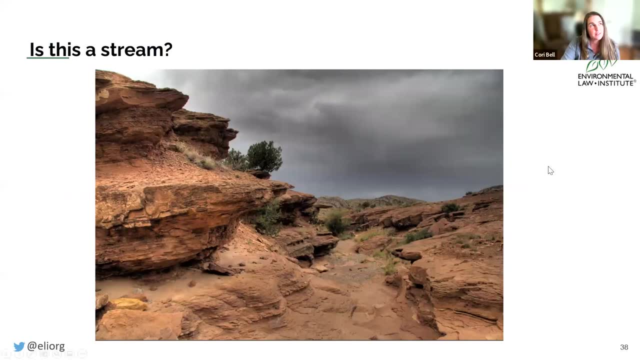 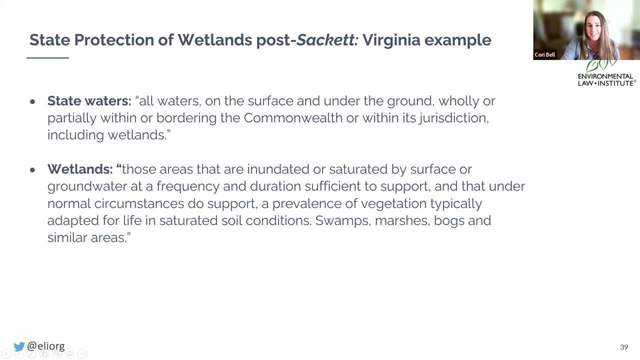 SACET first. Corey, do you want me to go back? Yeah, that would be great. Okay, Yeah, and I'll just say that as someone who worked on LA river issues for several years. it is a true river and you can kayak on it at times. So, yeah, we've been talking a little bit. 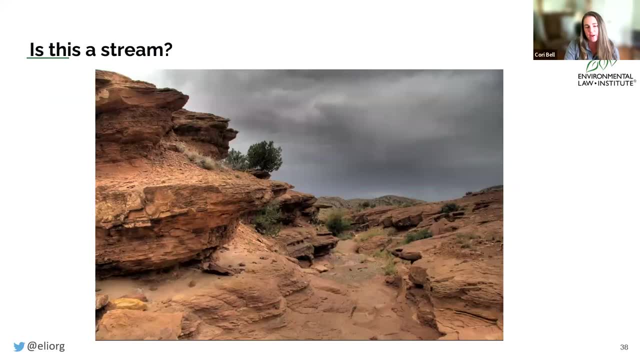 about SACET today And I'm going to give some background on that. And this case addresses exactly what I was talking about. So I'm going to give some background on that And I'm going to tell you exactly what Camille was just talking about. you know what is covered as a water of the? 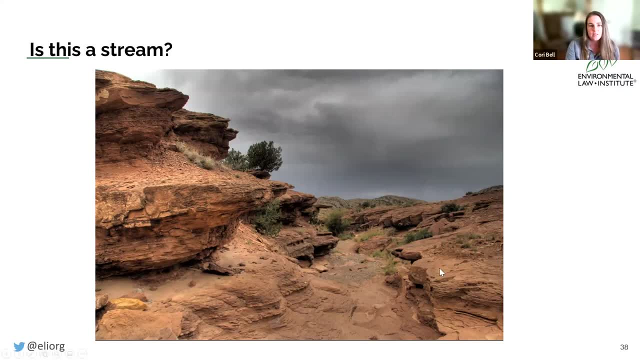 United States And unfortunately, the decision in SACET versus EPA drastically reduces the number of wetlands that are protected by the Clean Water Act. Just for a little background on why wetlands are important and should be protected: to begin with, wetlands themselves filter out pollution. 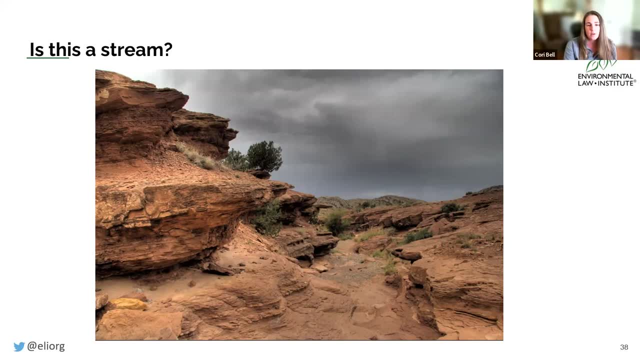 and help reduce pollution in water bodies. They're a critical habitat and they act as nurseries for all kinds of critters And they're a critical habitat for all kinds of critters. So they're a critical habitat for all kinds of critters And they're a critical habitat for all kinds of critters. 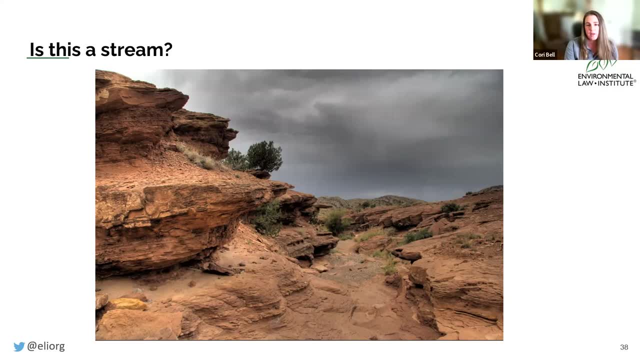 and wetlands also recharge groundwater supplies and are critical to reducing the effects of climate change because they absorb floodwaters, they protect against erosion and sedimentation, and they also store carbon, so they're a tremendous resource when it comes to climate change problems. in sackett, the court ruled that wetlands are not waters covered by. 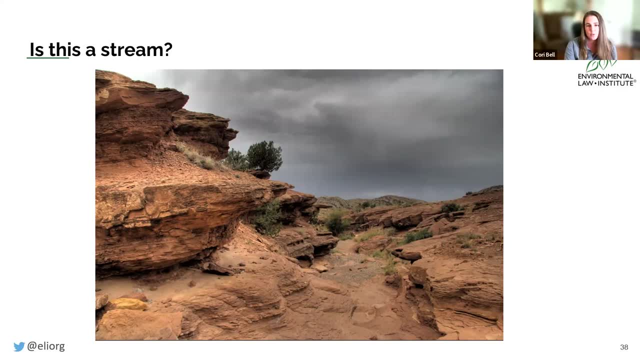 the clean water act unless they touch and are indistinguishable from other covered waters, things like lakes, rivers or streams, and this is a reversal of roughly 50 years of federal protections. um sackett also adopts a reading of the clean water act that five justices on the. 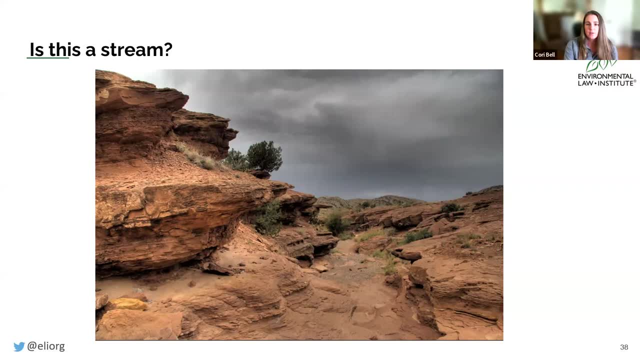 court rejected in a prior case almost 20 years ago, three justices, led by justice kagan, accused the majority in sackett of rewriting the law to fit their policy preferences. and just to provide some more context on on wetlands, there has been significant degradation of the clean water act. 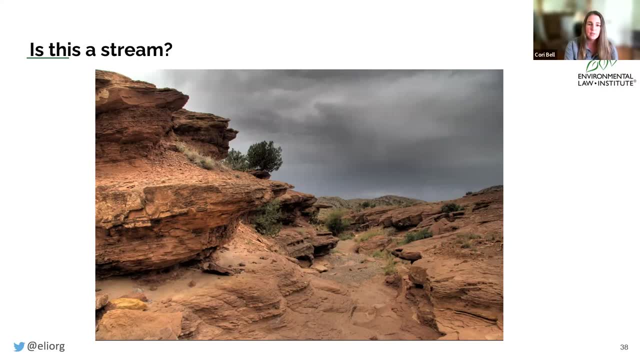 and destruction of us wetlands. between the time of european colonization in the 1980s, it's estimated that we lost about 53 percent of the wetlands in the continental us. they were destroyed and now, with sackett, we're estimating that at least 50 percent of those remaining wetlands in the lower 48 states. by our count, at least 19 000 wetlands at a minimum are no longer protected under the clean water act, so more of them are protected and the rest of the wetlands are not protected. they're going to be destroyed. this is really an unacceptable outcome and it's not what was. 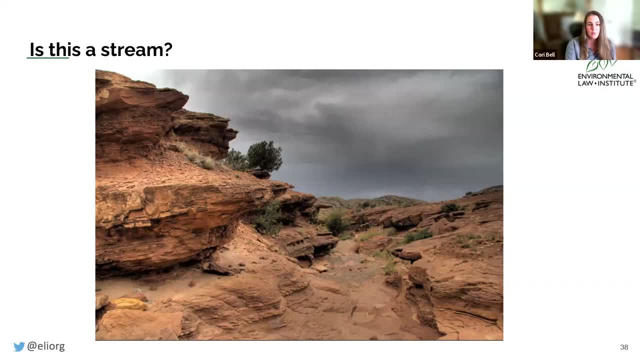 envisioned by the clean water act, with the goals that peggy mentioned before, including ceasing water pollution. the us already loses vital wetlands at a scary clip, and now we can only assume that it will get worse because of this decision, but there are some remaining options to protect. 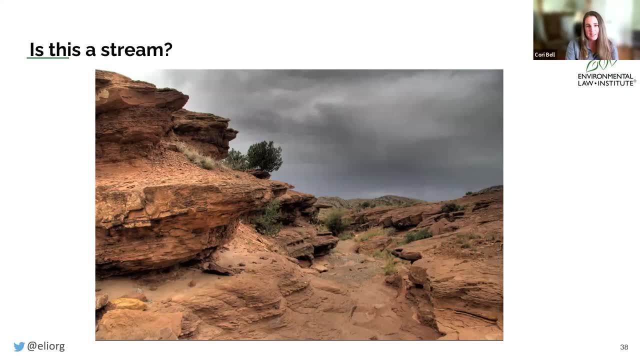 wetlands. i don't want to be um totally pessimistic here. those include, first and foremost, fixing the clean water act, and obviously that will take time, given the current makeup of congress and how slow everything is moving at the congressional level at the moment. it also includes 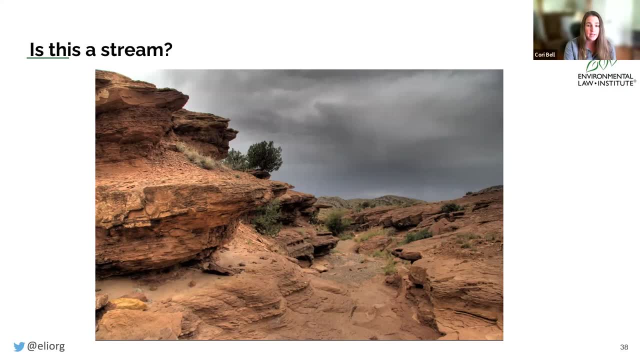 advocating for increased federal funding to conserve wetlands and protect them. you can, for example, pay landowners not to develop these areas um. also, you can enforce existing state, tribal and local water protections and increase funding for enforcement. and, of course, you can adopt new local requirements for the clean water act and, of course, you can adopt new local requirements for the clean 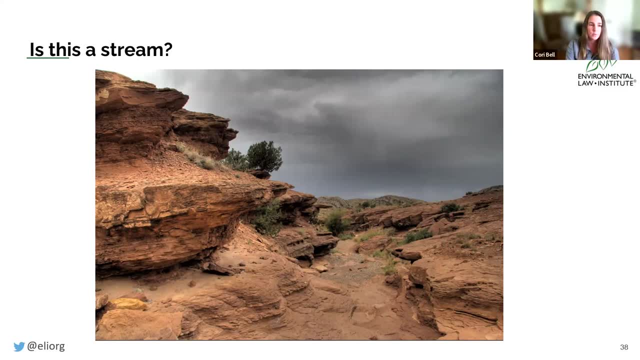 water act and, of course, you can adopt new local requirements that prevent and clean up water pollution in wetlands in the first place. so these last two options are pretty interesting because, like camille mentioned, there are around 19 or so states that do have additional protections. but 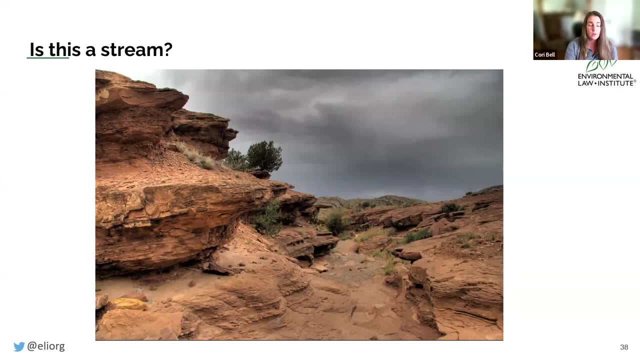 there are also 20 states that have passed what we call no stricter than laws, which essentially prohibit the state environmental agencies from being more protective than the federal epa. so it'll be a problem in those states to pass additional protections if you're interested in morning learning more about socket eli put. 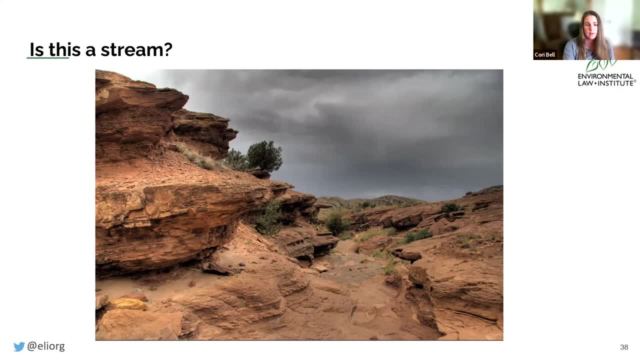 together a great webinar. i think it was last week and that's available online. also, the uh national association of wetland managers held an in-depth webinar on the decision. so you should check out those two resources, and now i'm going to hand it back over to peggy so she can give you some. 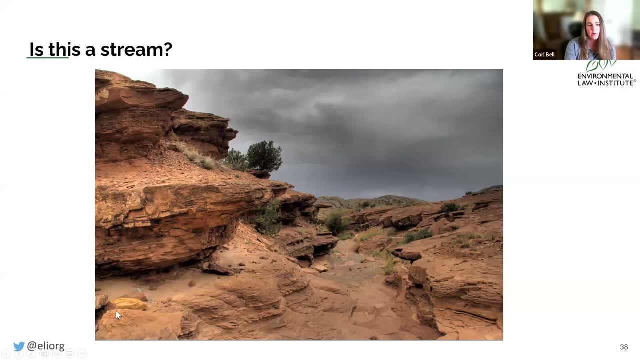 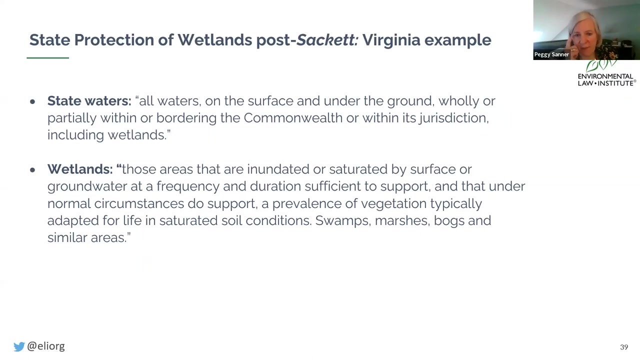 real world examples of how she expects this decision to play out in virginia. thank you everyone. um, we will just advance this slide. there we go. um, i would just note a number of the folks in chat had uh wondered about whether the slides were to advance. uh, cory was uh speaking without slides. so uh, if you're with us, 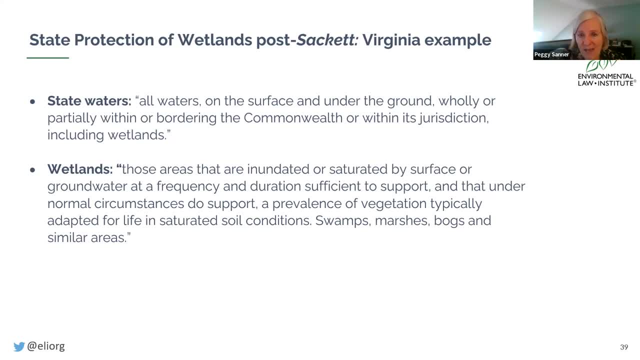 with a slide titled state protection wetlands post sackett, virginia example. you are with us, um. i would note again that, uh, all of the uh comments made by camille and corey about the seriousness of sackett and its effect on the protection of our wetlands, uh are, um, are are speaking the truth. uh, and while 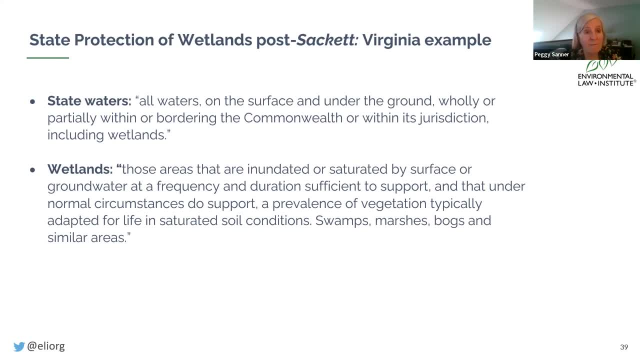 there are some examples, virginia being one where we have a very comprehensive state program. the majority of states do not, and even in states like virginia we have a significant concerns which i'll go through now. so, um, one way that the state program differs from the federal program is that there is no virginia state legislation. 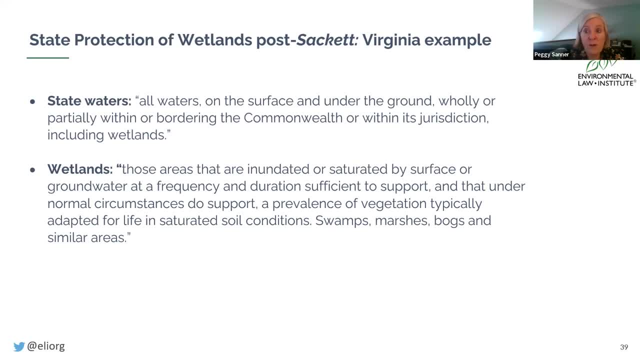 皆. that limits uh regulation of waters to navigable waters. instead, we have a definition of state waters which covers everything, all bodies on the surface and under the ground, wholly or partially within the commonwealth, including wetlands. those are state waters and they're within the jurisdiction. 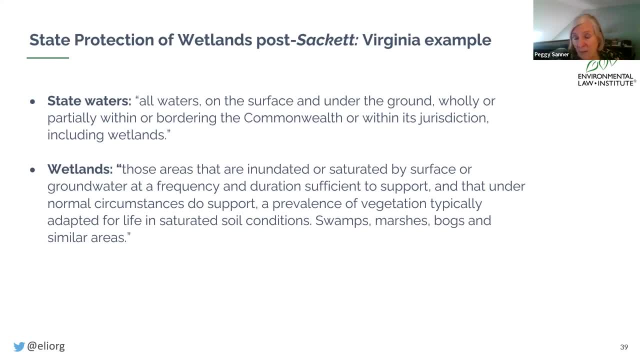 of our regulatory agencies to protect- they're subject to, frankly, an environmental unconstitutional protection of these waterways. There isn't a very expansive definition of wetlands themselves, which I'll let you read, but largely anything that is inundated or saturated by surface or 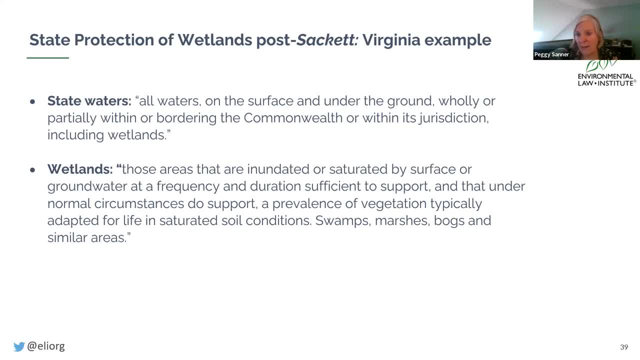 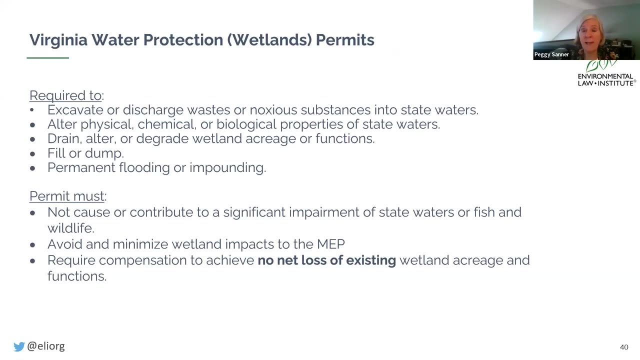 groundwater frequently and has the right kind of vegetation. Virginia's wetlands program, I will note, started in tidal areas in the late 70s and it was expanded in the early 2000s to address non-tidal wetlands. So at this point the entire commonwealth is covered by. 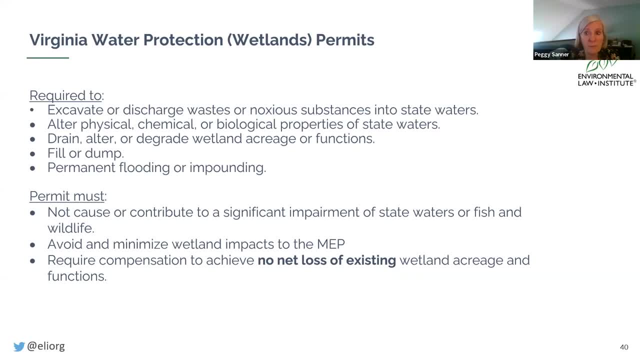 a wetlands program which is administered largely through state permits which had been issued in the 1970s conjunction with the US Army Corps of Engineers. That of course will change somewhat moving forward, But largely speaking, under Virginia's wetlands permitting program a permit is required. 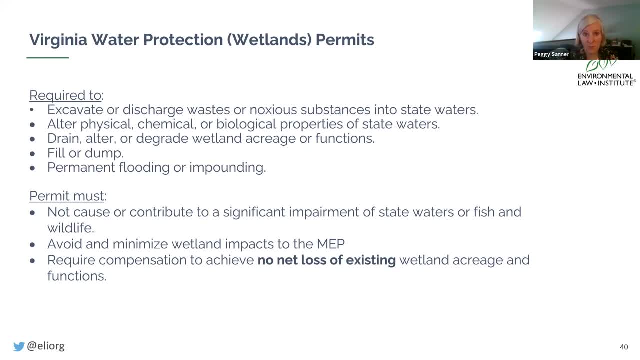 whenever anyone wants to excavate or discharge wastes or other noxious substances into the waters. whenever anyone wants to alter the physical, chemical or biological properties of state waters, drain, alter or degrade, fill or dump, permanently flooding or impounding All of. 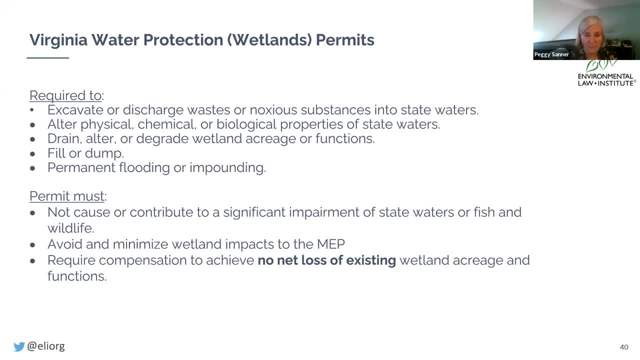 those activities require permits And, importantly, the permits as issued must ensure that the activity will not cause or even contribute to a significant impairment of state waters or fishing wildlife Permits must avoid, must require the person seeking a permit to avoid and minimize wetland impacts, And it also requires compensation. 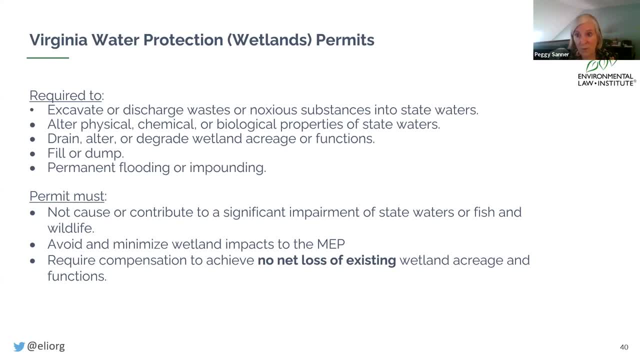 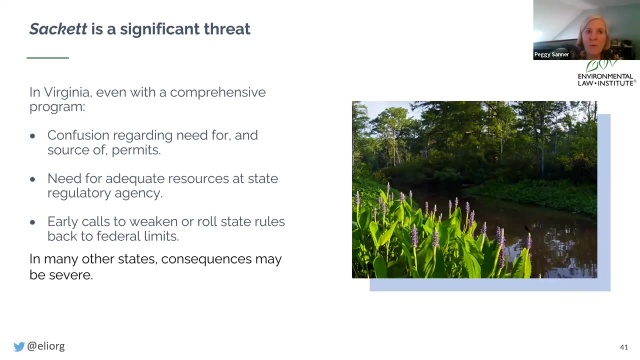 to achieve a standard which is quite important, and that is no net loss of existing wetland acreage and functions, A very important requirement, not always, in our view, attained in practice. But even with all of this statewide and comprehensive program, we recognize SACET as a threat. It is a threat because there already is confusion about 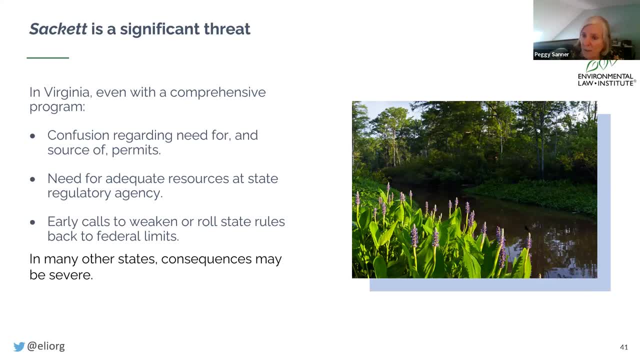 the need for and the source of permits. People who don't follow this work on a regular basis might have heard that you know the permitting program is over. They might not know. can we still go to the Corps for a permit, Or do we always have to go to the state? Does the state 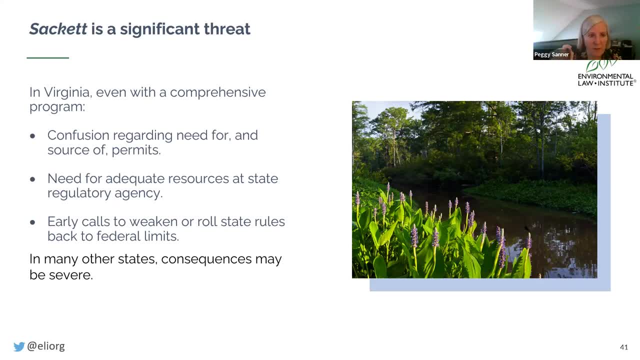 even have a permitting system, A lot of confusion which will have to be addressed. A grave problem which, in my view, will obtain not just in Virginia but across the nation, is the adequacy of resources to address areas which might have been covered by a federal permit under. 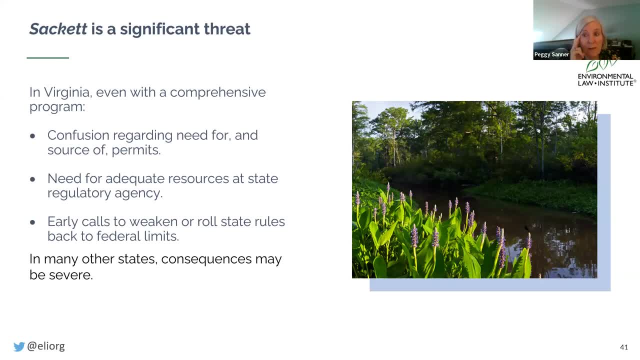 the 404 program but which will now be under the jurisdiction exclusively of the state, And I understand that estimates in our state are that 40 new people would be required to do the kinds of preparatory work that has been handled typically by the Army Corps of Engineers. 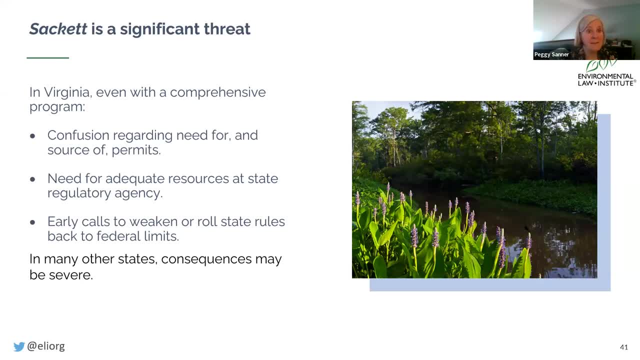 And in particular I'm referring to wetlands delineation, the need to inspect a property before any development activity and to determine what are the boundaries of wetlands, what are the kinds of wetlands. The Corps has done that, And in certain areas, of course. 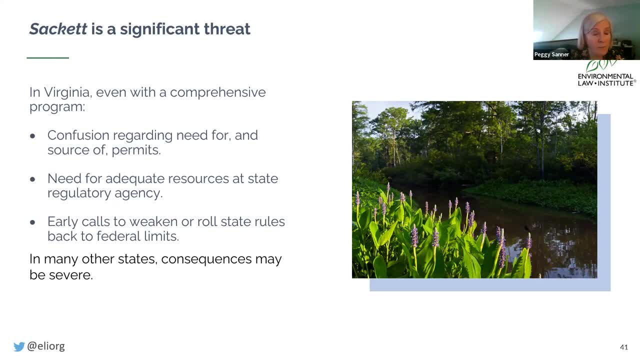 it will no longer be doing that, since there will be, even in Virginia, an end to some federal jurisdiction. Every year, since I've been involved in this work long before SACET, our politicians reexamine whether or not it's appropriate to have a state system that does more. 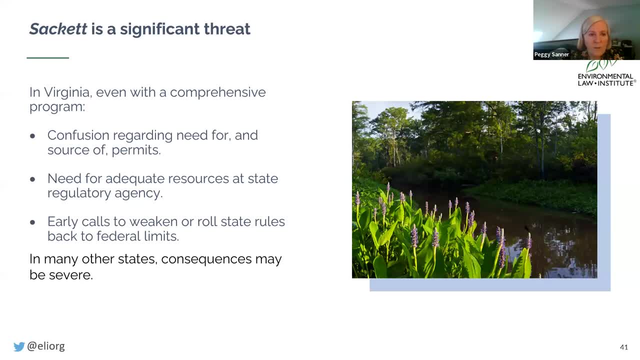 than required by federal law And we certainly would not be surprised to see some of those calls increase this year and to potentially find greater support- And that may be the gravest of all- And people who've been working in the environmental sphere for decades. 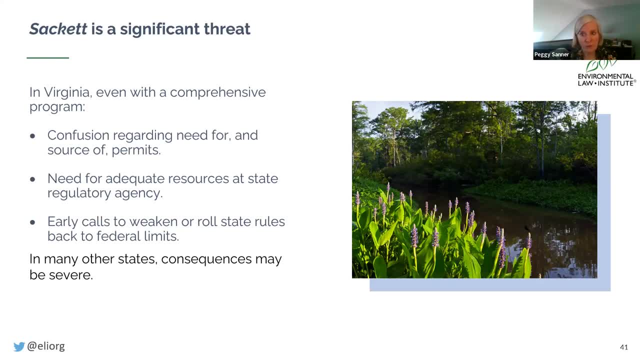 have been aware of the need not to allow for a race to the bottom- the lowest common denominator, but rather to allow states to experiment and, potentially, to do more, And so I think in all of the states where we currently have the greatest comprehensive programs, it will be important that we defend those programs. 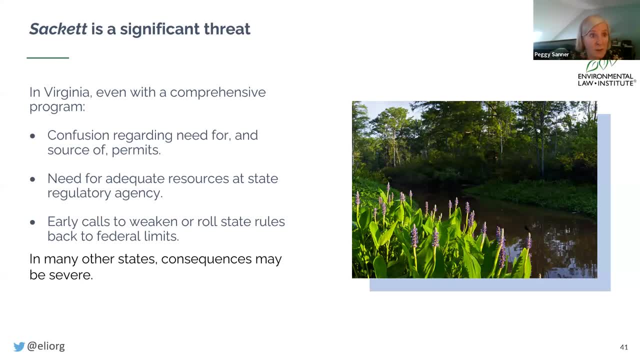 And in states where the programs are not currently comprehensive. certainly it would be a welcome development to see greater efforts made to expand state coverage. So the challenges that SACET has created will hit each state across the country, And I think that's something that we need to be doing in different ways, but in all cases in a significant way. 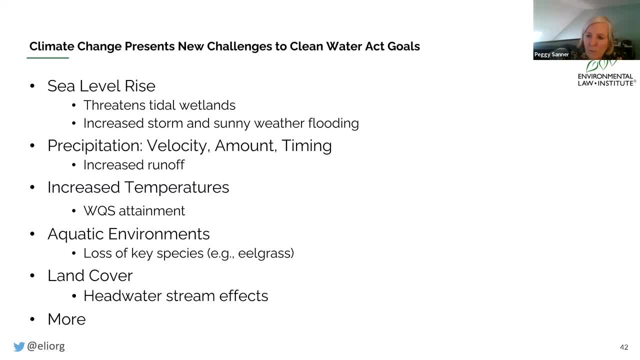 So that's all I'll say now for SACET in Virginia, But I did want to wrap this portion of the program up by highlighting something that many of you are probably already aware of, and that is potential effects of climate change in so many aspects of our lives. Climate change will present new and serious challenges to 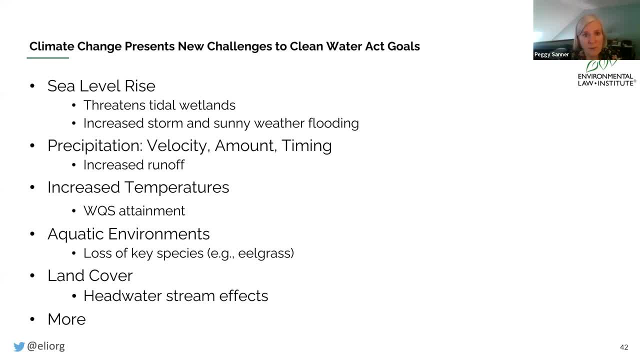 our ability to live up to the goals and practices of the Clean Water Act in a variety of ways. I'll just name a few, but it's not exclusive or comprehensive by any means. On our coastlines, sea level rise will indeed threaten tidal wetlands. It will drown many of them and it will try to create new wetlands in areas that are not. 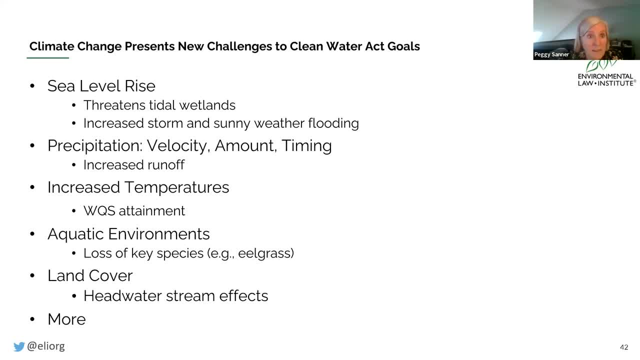 in the area that are now agricultural lands, cities, residences. A very significant effect on loss of wetlands, but also on increasing pollution to these waterways resulting from the flooding. and rise of the sea level Increases in storm and sunny weather. flooding increases in the velocity, the amount, the amount of water, the amount of. 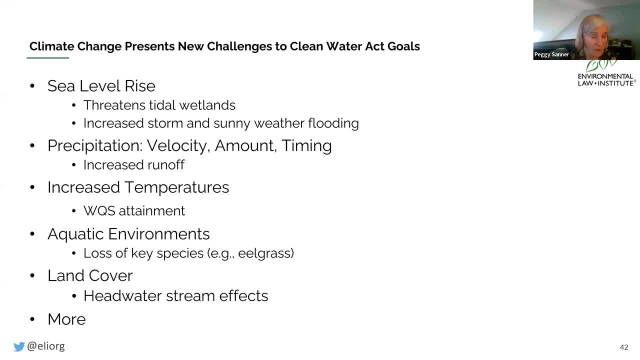 rain and the timing of precipitation. We've seen all the extremes across the nation in the last year and it certainly hits. these trends affect every part of the country: Rising temperatures. In the Chesapeake Bay we're already seeing warmer water. It's a very shallow water body and warmer water will have all kinds of effects on. 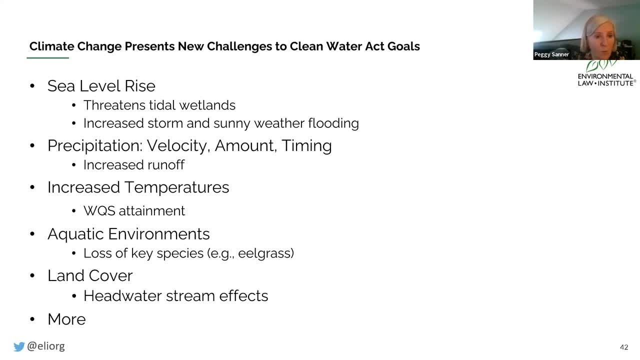 the habitat. Eelgrass, a really important under water grass for that environment, is giving out, giving way to other grasses or no grasses at all, because of, in part, increased temperatures, Land cover changes, The differences in rainfall. 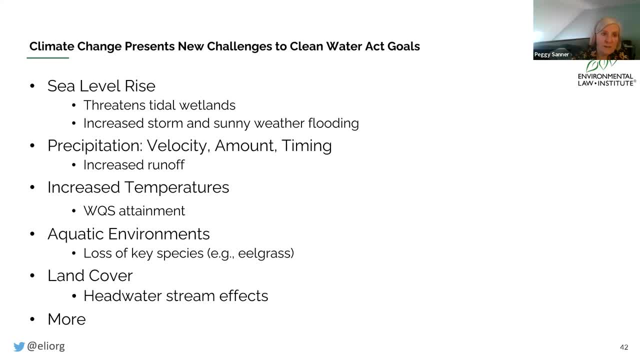 and unpredictable rainfall events. we see changes in land cover that have a lot of impact on the environment. Land cover changes, The differences in rainfall and unpredictable rainfall events. we see changes in land cover that have a lot of impact on the environment. added to development-caused changes in land cover will lead to changes to the temperature. 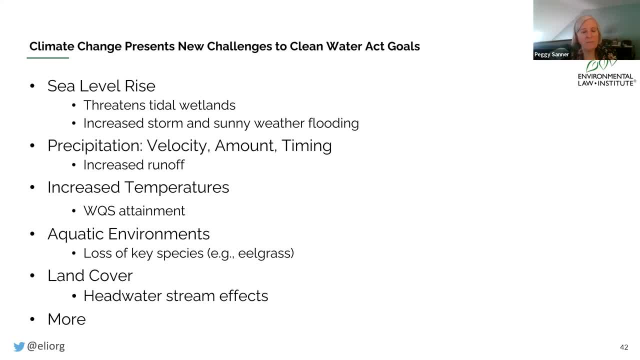 of water quality streams- excuse me, of headwater streams- and many other changes. This is just a sample. States will be working very hard along with the federal partner at EPA to ensure that we try to keep up with those changes so that the Clean Water Act maintains its position. 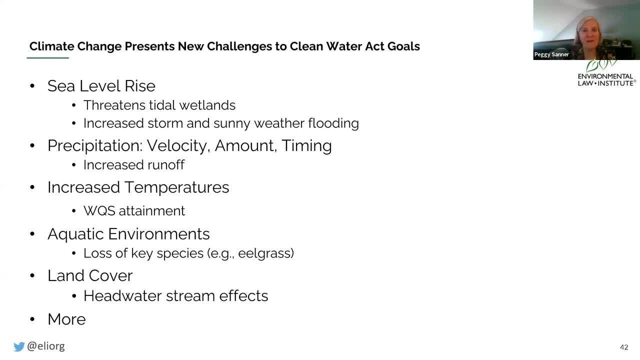 as the linchpin, the bulwark, the fundamental building block of our states, of our nation's ability to protect this clean water. So thank you all very much. Thank you, Peggy. So we are getting a lot of questions in the Q&A, quite a few relating to SAC-IT, but 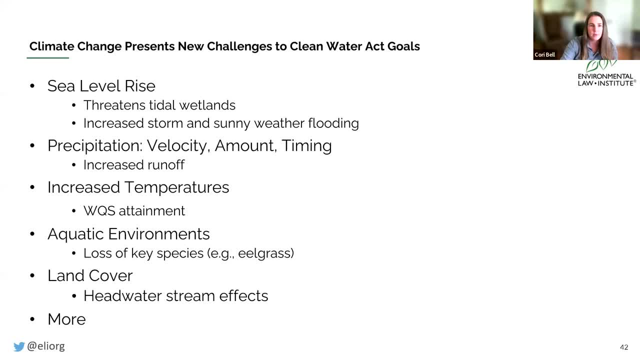 I want to start with… some of the more kind of basic Clean Water Act questions and I will direct those to an individual panelist and then if whoever doesn't answer wants to follow up, please, please, do feel free. So we have a couple questions asking about what I would consider emerging contaminants. 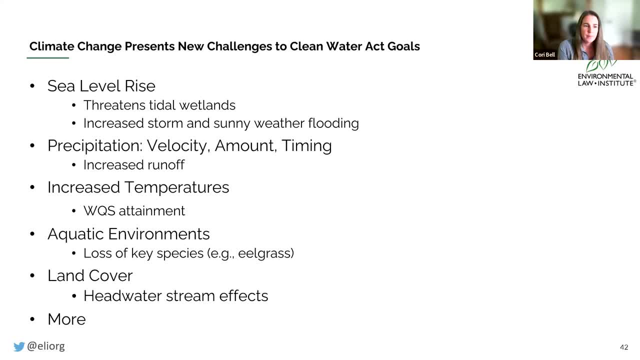 Camille, someone is asking whether EPA has the authority under Clean Water Act to… regulate microplastics and microfibers, and whether that could be done either at the wastewater treatment plant or if that could even be done at the washing machine level. 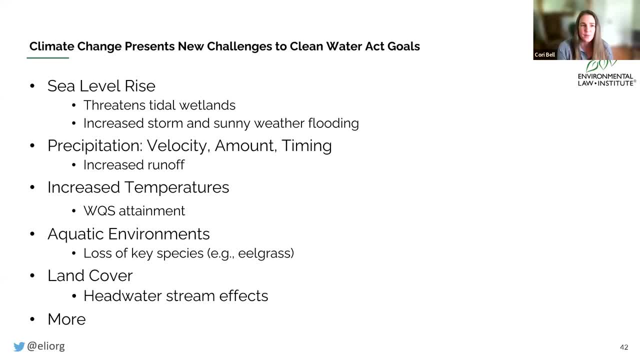 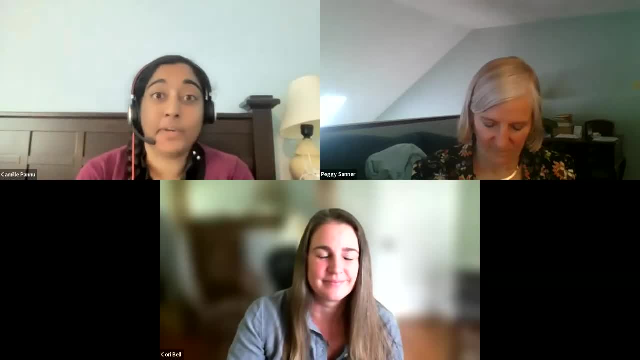 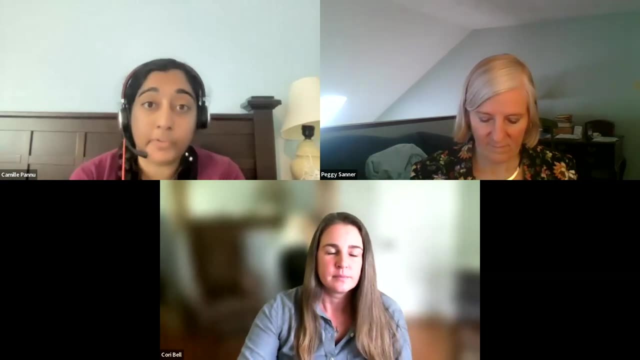 Could a washing machine be a point source? So could you discuss a little bit about that? I can try. So this is an area that the EPA has been monitoring and is concerned about. Microplastics are increasingly problematic and microfibers have been on their radar for. 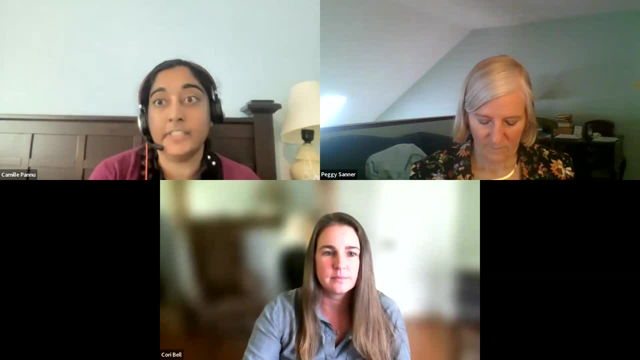 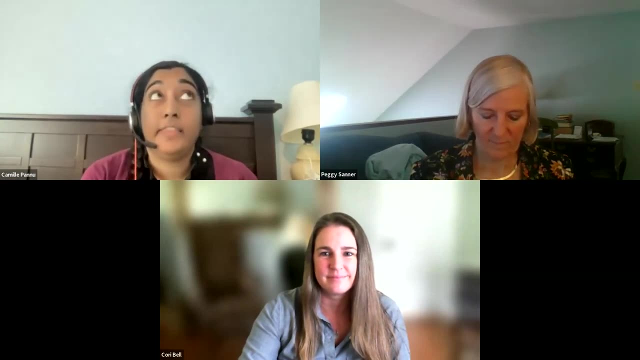 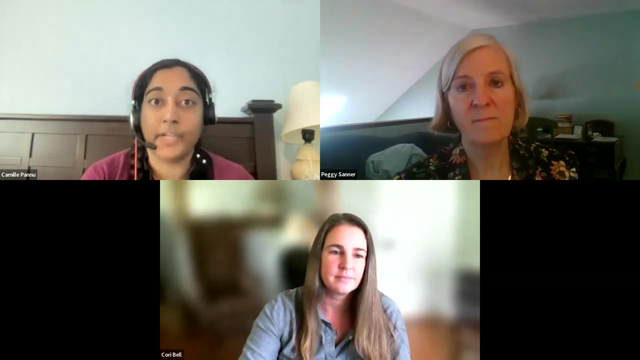 a while, Probably for as long as skinny jeans have existed as a modern creation. but so the short answer, I think, is yes. The long answer is that it's a process to get a pollutant listed or to get a category created and to go through the regulatory process, so that can take quite some time. 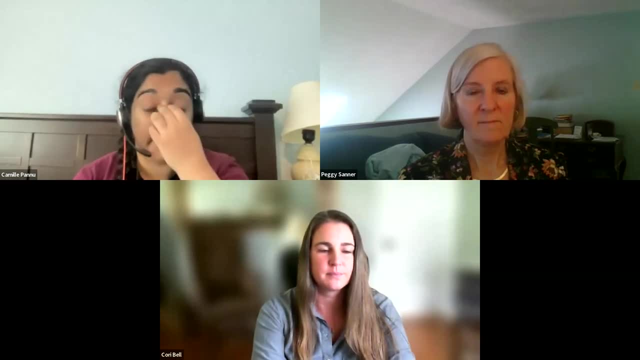 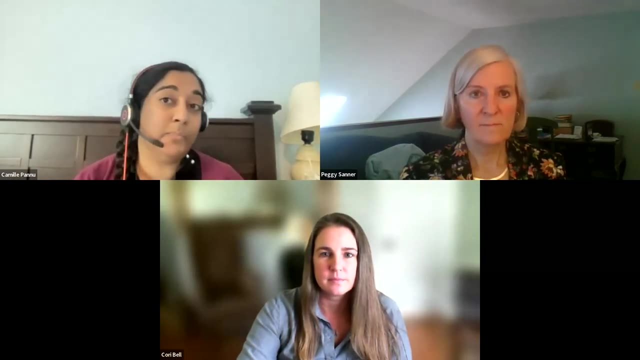 With respect to washing machines, I think the answer is no. I don't think they would be regulated as point sources, but what you would regulate is discharges into whatever the pipe is, And so whoever… And what can be done to make sure that there's a safe drinking water for any kind of use? 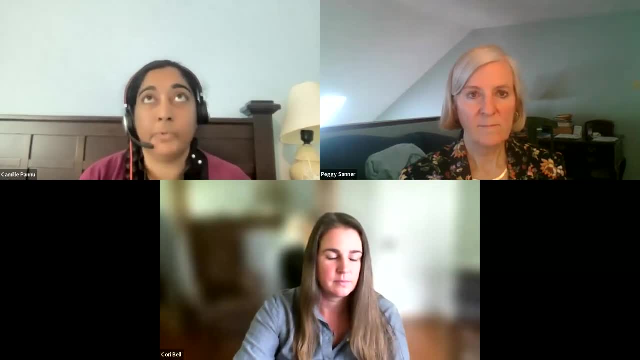 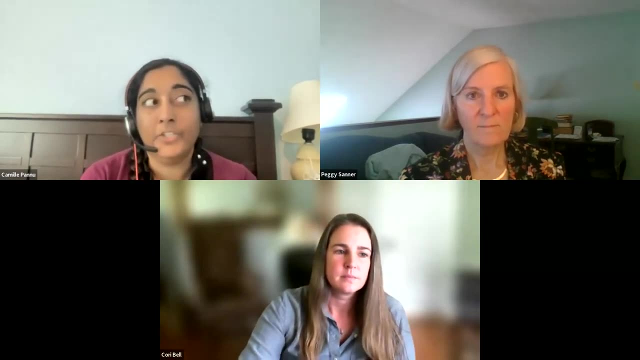 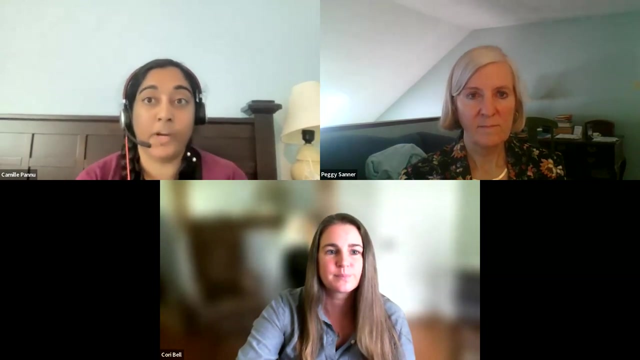 that normally wouldn't be a house. It would really usually be often regulation of the wastewater treatment plant level. But this is kind of a persistent tension in both the Drinking Water Act, the Safe Drinking Water Act and the Clean Water Act, which is that do we impose the cost of treating water? after it's already been polluted, Or do we require stricter requirements to protect water from getting polluted to begin begin with, so that we can prevent any of the cleanup costs from kind of coming down the line, and certainly for wastewater treatment plants? this is true also for drinking water distribution. 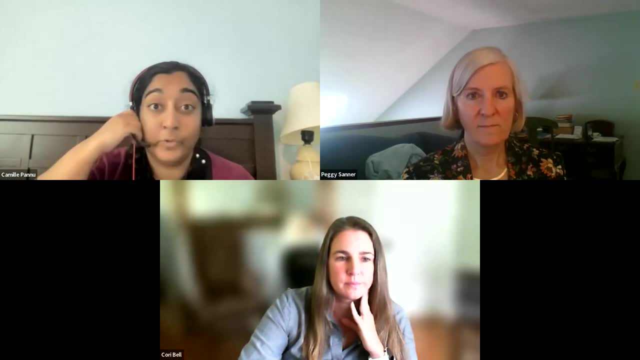 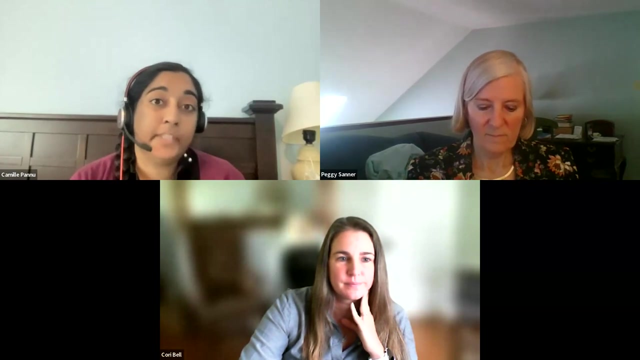 those tend to be publicly owned, meaning like owned by government, local governments- and so you're also kind of taxing taxpayers for a problem created often by industry. so, in terms, one of the things to think about, though, would be whether or not there's separate agencies that have authority to regulate washing machines. they do, so another way to kind of get at 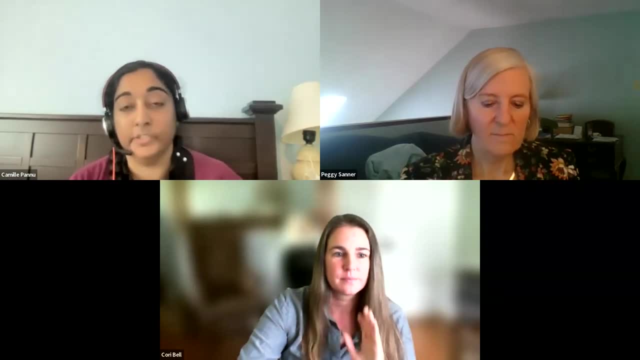 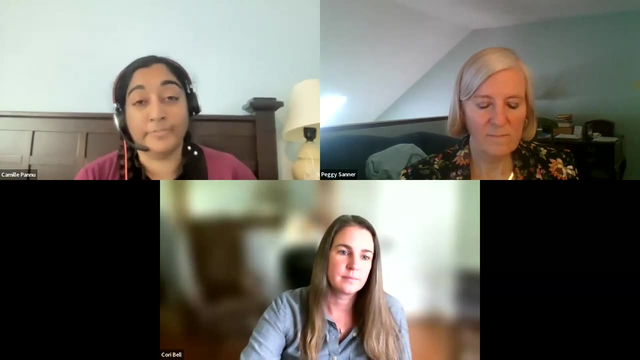 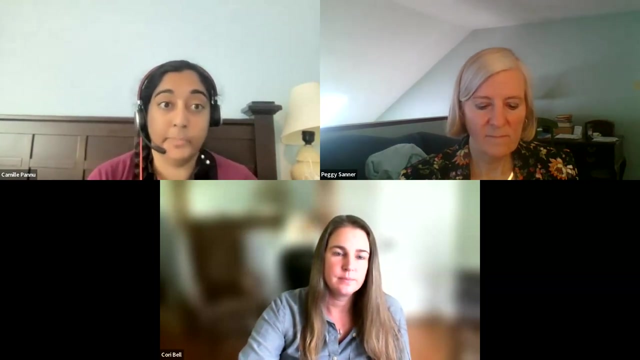 this is also to to advocate on the consumer protection level that there should be certain safeguards or environmental safeguards in the creation of certain technologies. there are micro plastic and microfiber filters available in washing machines. they're just relatively expensive and it's. they're not common, they're not mainstreamed on the market. so good questions. 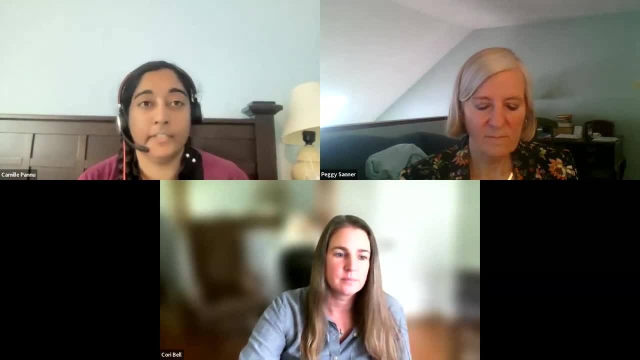 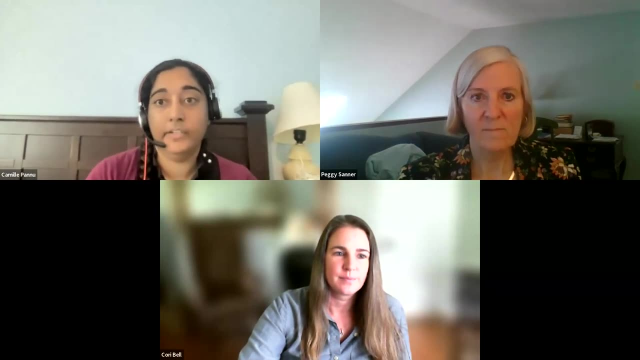 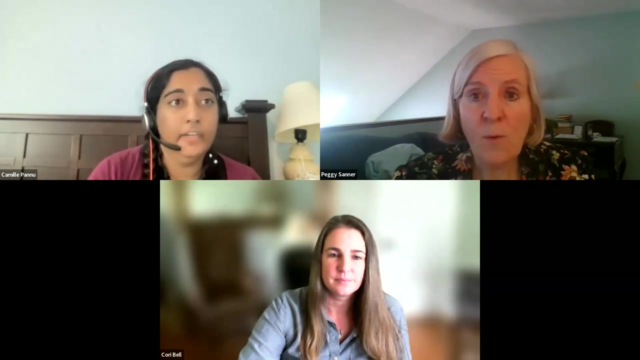 good questions, so i think they could regulate it. i think it could be difficult to regulate the sort, the actual washing machine sources of a lot of this pollution. thank you, peggy. do you want to follow up with anything? yeah, i will say that. um, we see, on a practical level, uh, some of our wastewater treatment plant. 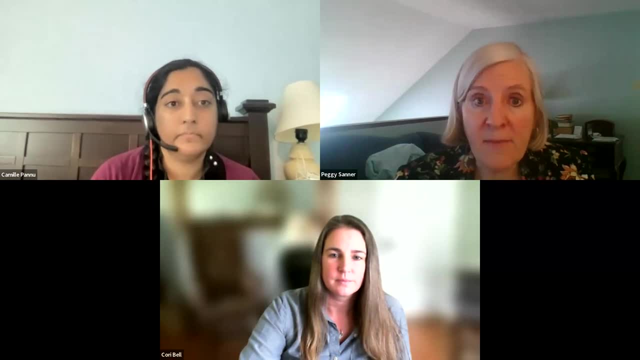 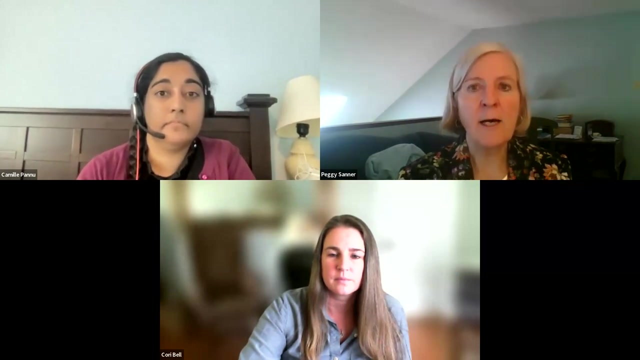 operators already working on methods to detect and remove some of these contaminants. microplastics certainly is one from the stream that they discharged. obviously, uh, much more needs to be done and corey mentioned um pfos, which is, she said, an emerging contaminant, um really big issue. 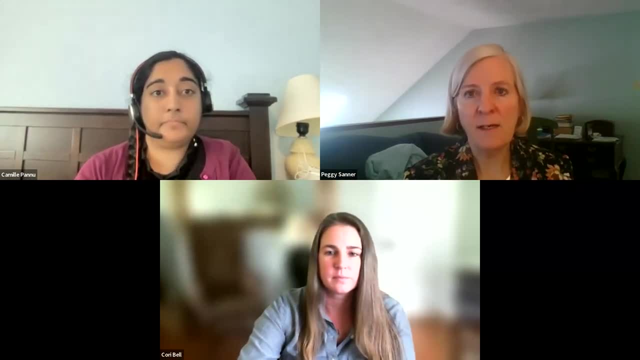 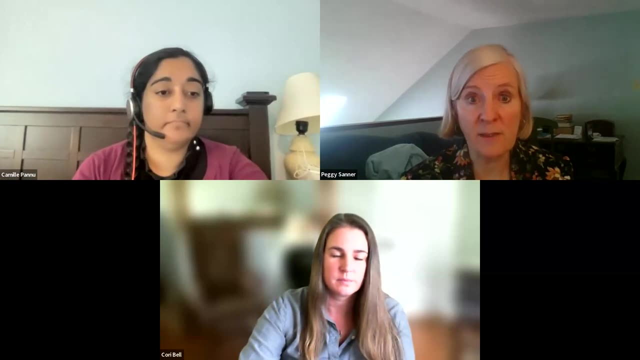 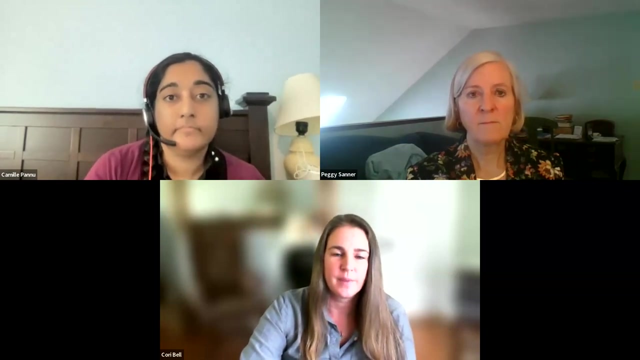 uh, and because so pervasive in part, um, that, uh, we'll see a lot more of that going forward and it will be done. yes, i agree, uh, to some extent under the clean water act, but through these other systems that Camille mentioned. Thank you, I'm going to direct the next emerging contaminant question to you, Peggy. 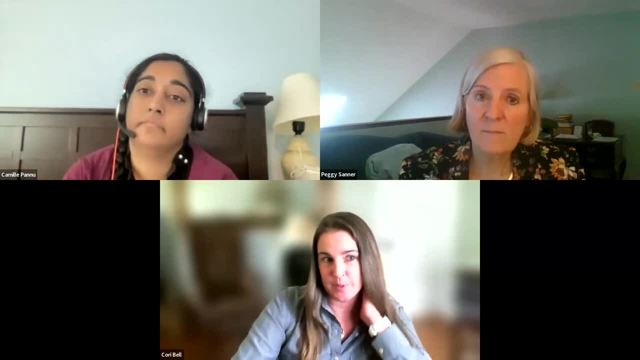 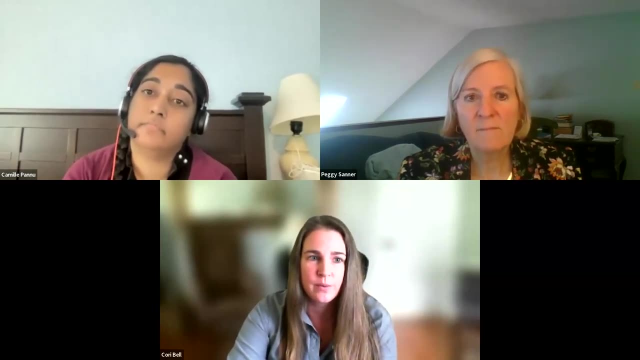 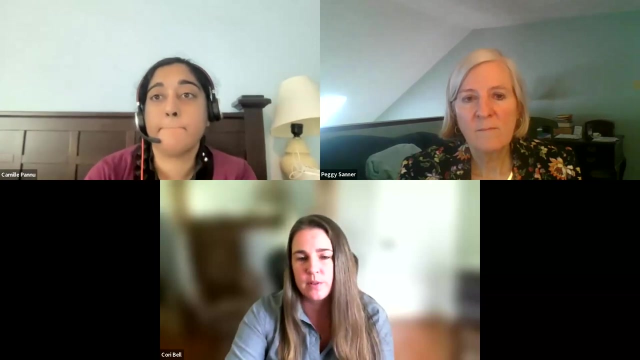 I'm not sure which of you might have experience with regulating aquaculture, but could you talk about how- whether it's fish or shellfish aquaculture- how they might be considered a point source and whether they're regulated under the Clean Water Act because of the pollution? 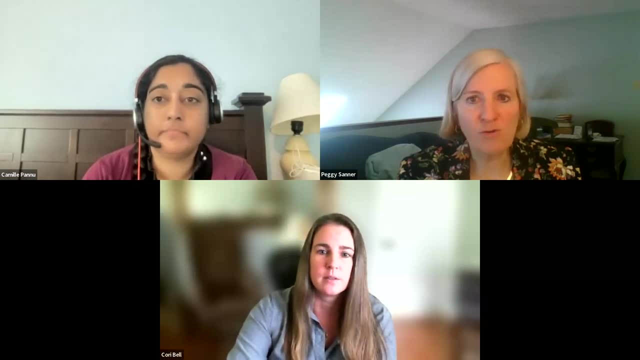 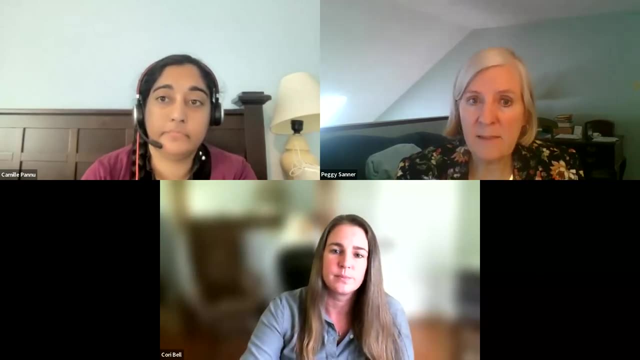 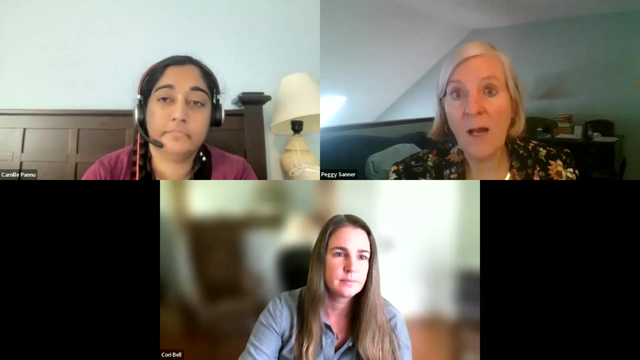 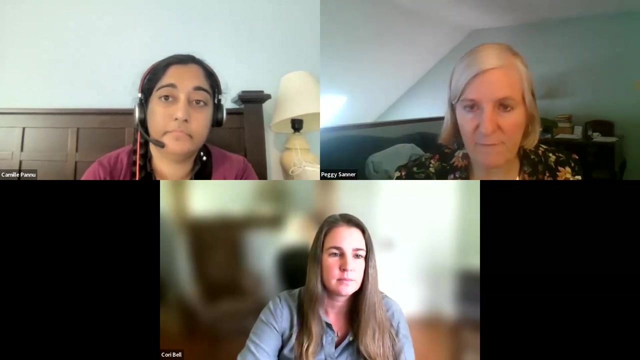 that they cause to marine environments. That's a great question. They are indeed regulated. They are of a certain size as a point source under the Clean Water Act. The concept, in a very general way, is: the fish are right- now I'm talking about fish maintain. 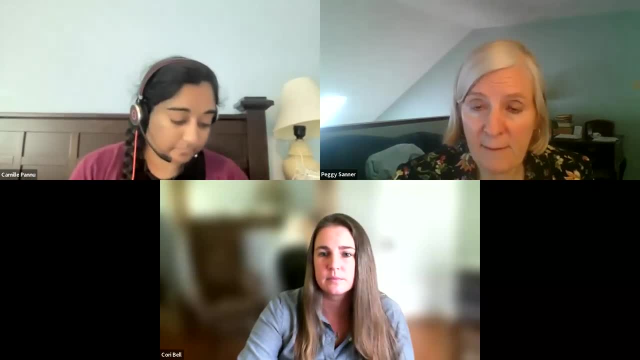 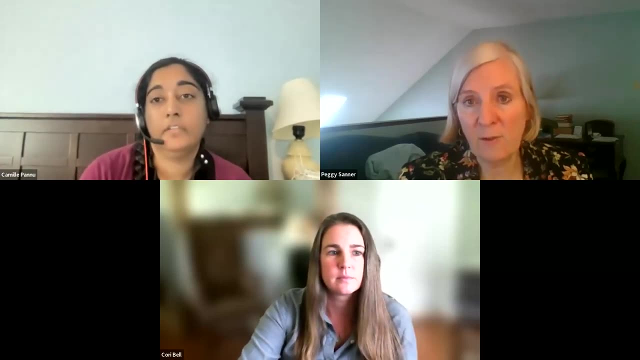 in a particular area, They are fed in a particular area and, of course, they, like any other living organism, discharge their feces in a particular area. Because it's so concentrated, it changes the water quality in that area and in the surrounding water. 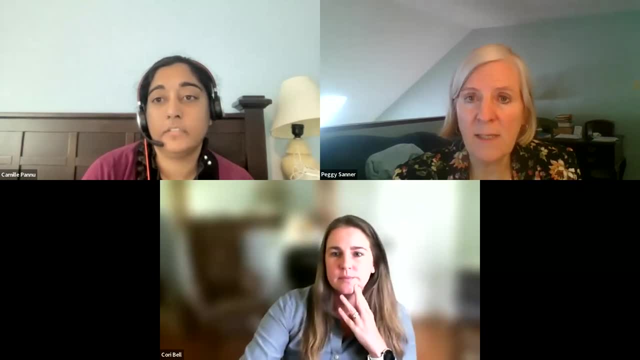 It does so to an extent that it becomes an issue that should be certainly, in my view and the view of many others, a regulated antithesis. Okay, So there's a lot of uncertainty and it is Not all aquaculture is depends a part on size. 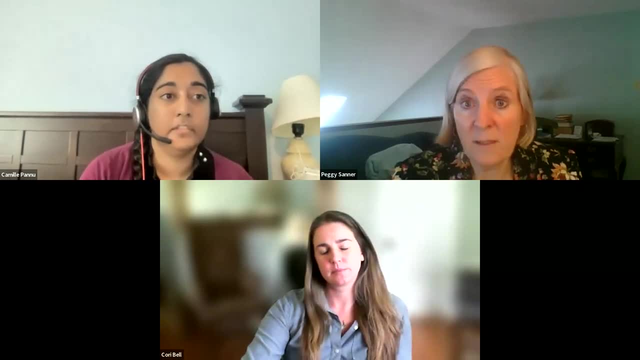 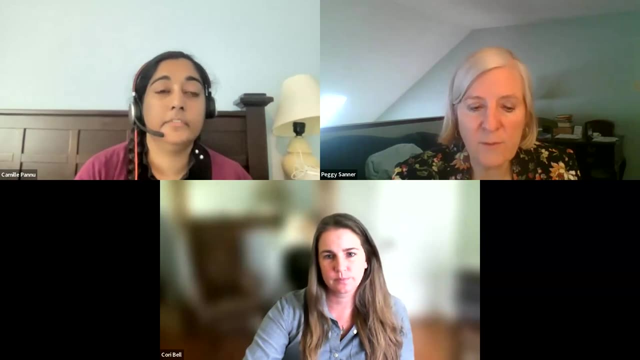 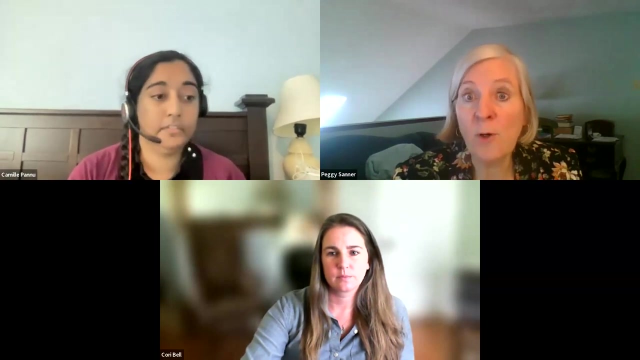 In our part of the world we are seeing a lot of, and certainly in support of a lot of, shellfish aquaculture, whether it's clams or whether it's oysters. Again, a lot of it depends on the size of the operation, but many of them are outside. 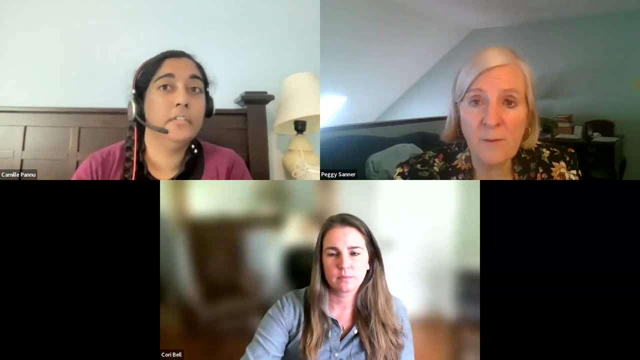 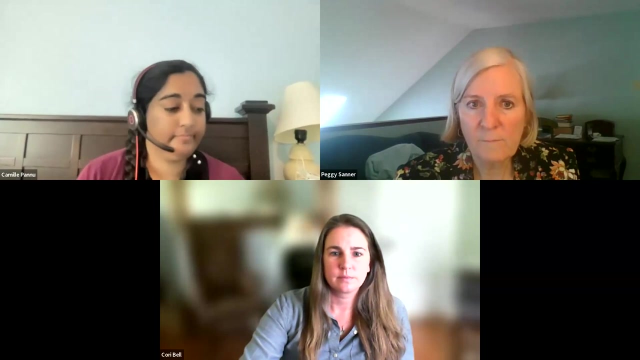 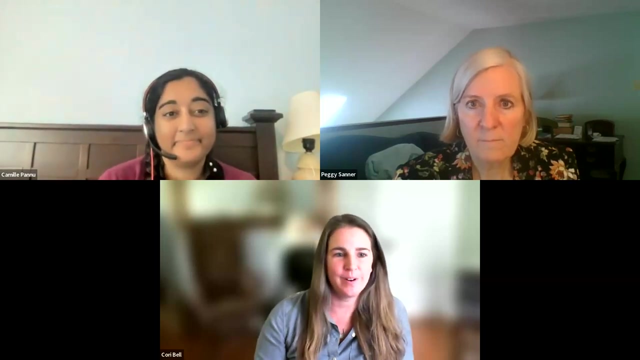 the size that would require of permitting under the Clean Water Act. But again, it has to do with the effect of the concentration of animals in a particular water body. Thanks, Peggy. Camille, do you have anything to follow up on? All right, 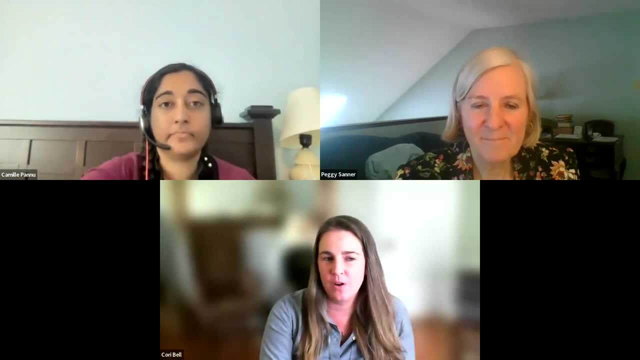 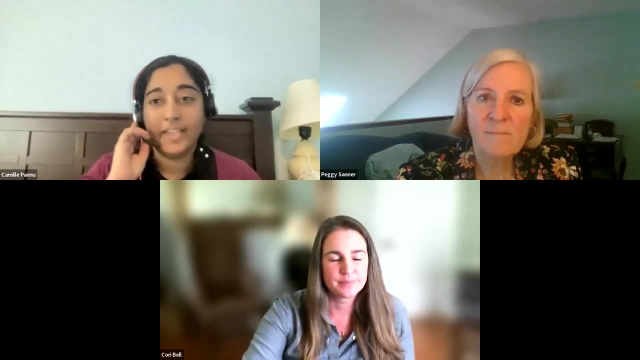 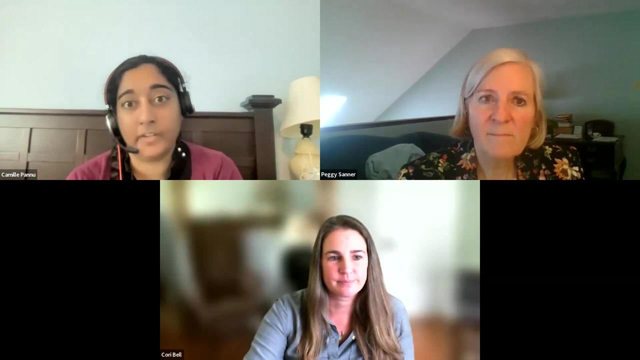 So I do have a question for you now, Camille. How, if at all, does the Clean Water Act regulate atmospheric deposition of pollutants? It generally doesn't. There are certain moments in time where you could make an argument that a specific atmospheric deposition of a pollutant could qualify. 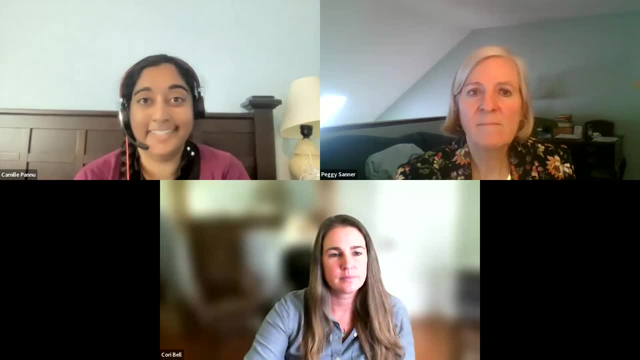 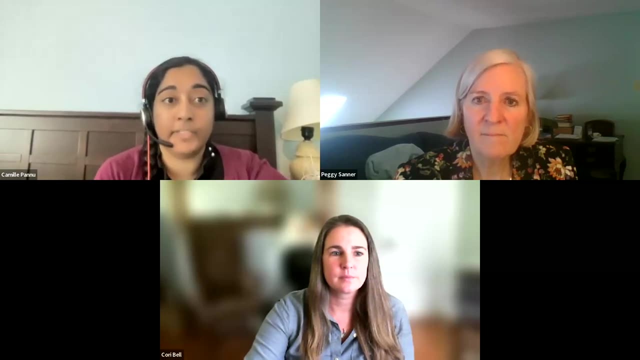 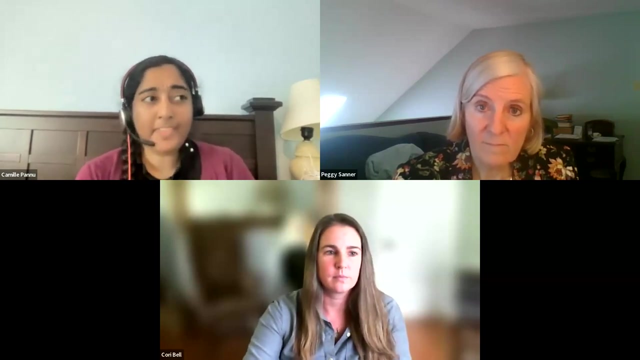 I'll give you two examples of things that don't qualify but are common. So when I lived in California, I worked primarily in the San Joaquin Valley, which is the most polluted air basin in the country. What? Because a lot of the air is polluted and so the energy costs that we spend on our air 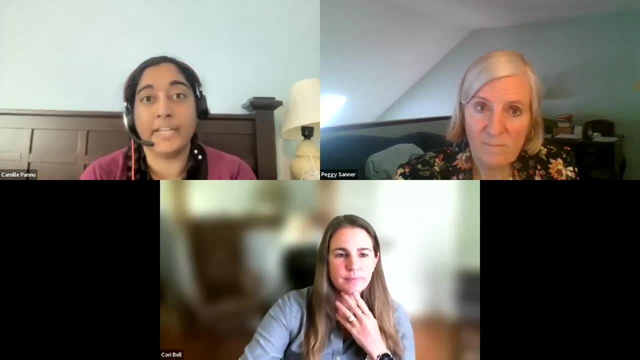 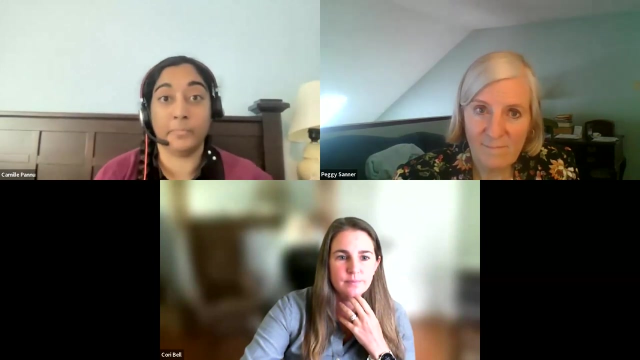 thousands and thousands of dollars, and so when we were asked about why we were so out of control compared to historic levels, the executive director for the Air District said that it was because it hadn't rained. And I was like what? And so what he was basically arguing is that all this air pollution would be not air pollution. if it rained and bonded with water particles and then became basically water pollution instead, which would be totally unregulated by the Clean Water Act. Another good example of this is if you live on the East Coast or in the Midwest and were affected by the smoke from the fires in Quebec and then got thunderstorms, which happened. 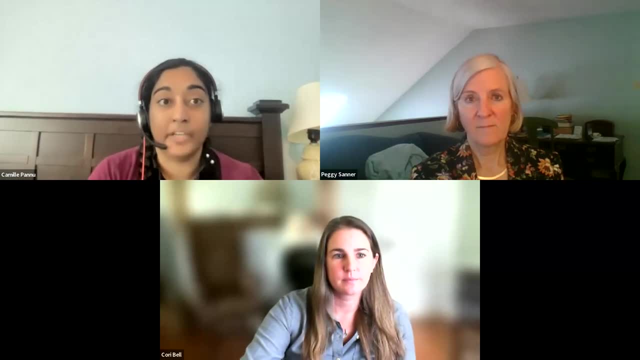 where I lived. it cleaned up the air. but it cleaned up the air because it took all of that ash and soot and particulate matter and basically washed it into storm drains. So atmospheric deposition is very rarely covered by the Clean Water Act. 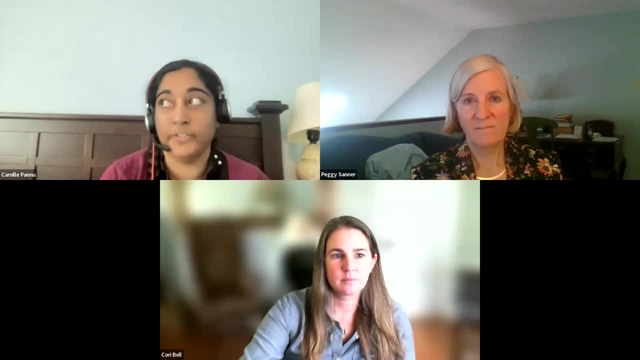 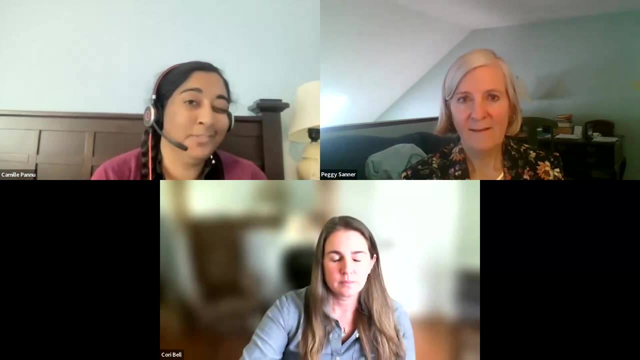 I can't think of a single time off the top of my head, but I'm sure there's been at least one instance where there was something more concentrated and something was put together. But yeah, for the most part it's not really covered. 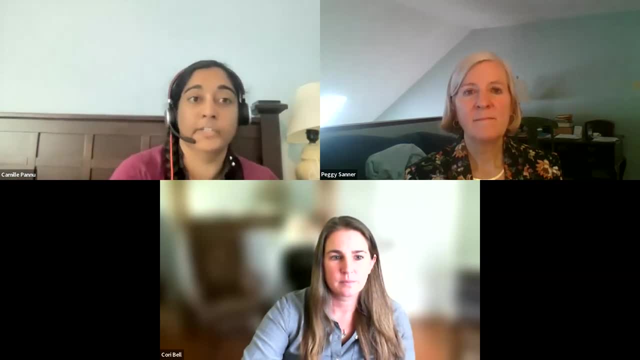 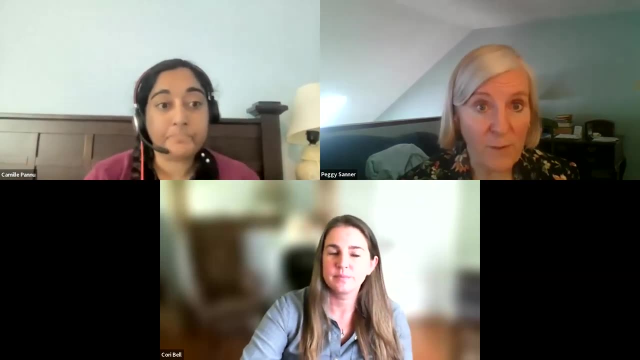 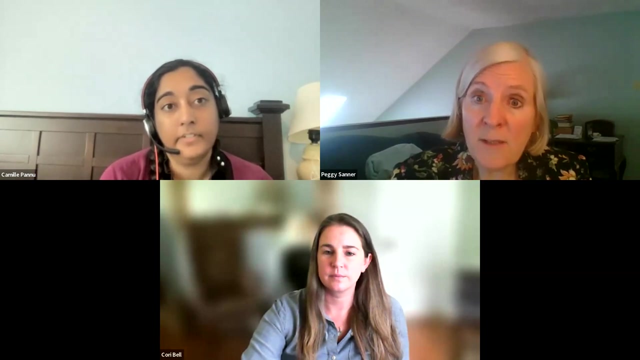 It's really thinking about things in terms of stream flows, like water into water, instead of thinking about air into water or rain into water. I'll just build on that. I agree with your comments, but I will say that in constructing the Chesapeake Bay, TMDL. 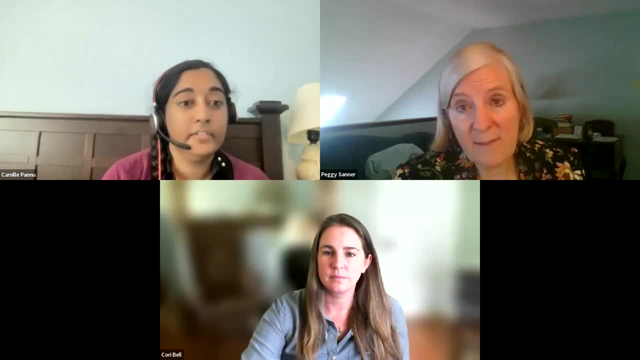 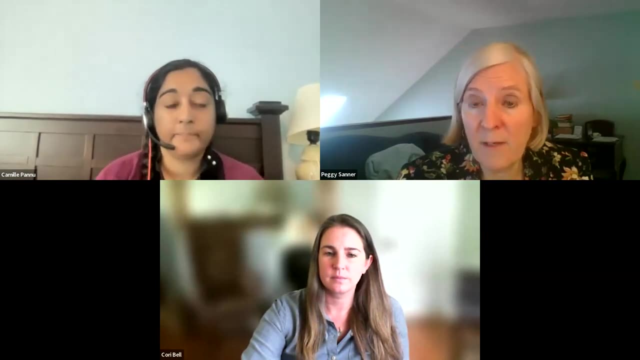 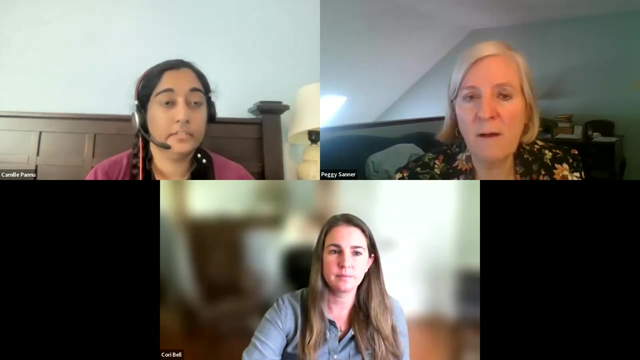 we've learned that. We've learned that about 30% of the nitrogen that is a pollutant to the bay comes from air deposition, and some of that's direct It comes from the air and deposits, if you will, directly on the surface of the water. But the other piece that Camille mentioned is that when it rains, a lot of that nitrogen compounds- nitrogen oxide is Captured by the raindrops onto the land and it becomes, as Camille said, nitrogen that's added to the bay. 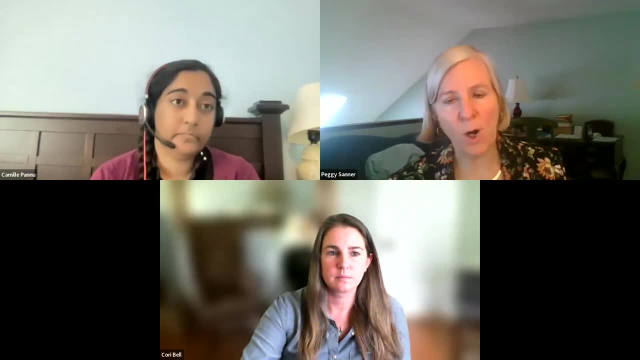 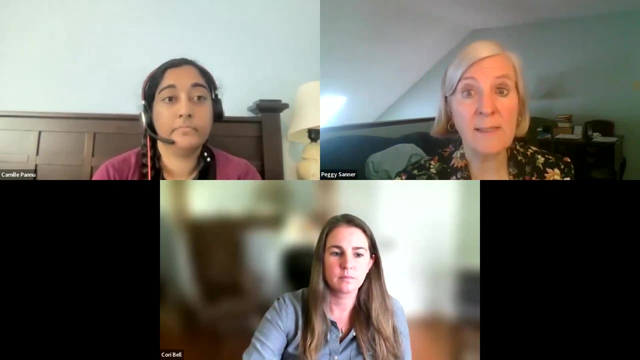 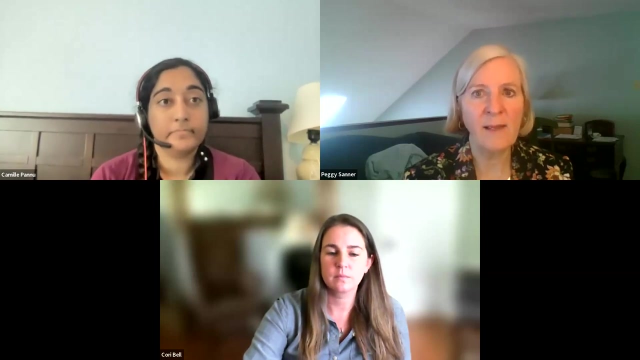 And so in those indirect senses they become part of the mix that are part of TMDLs. They are part of what constitutes the pollution load that a TMDL is designed to address- So only indirectly, to my knowledge as well, but that's an example of how they can be part. 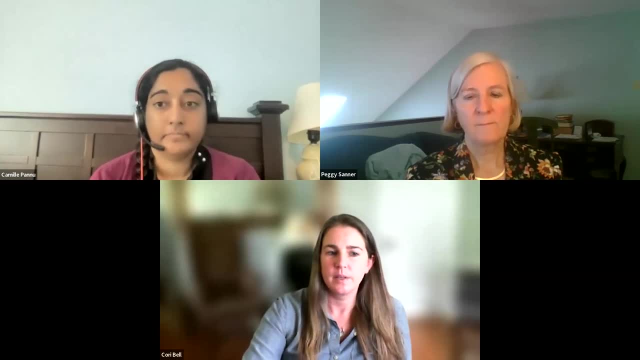 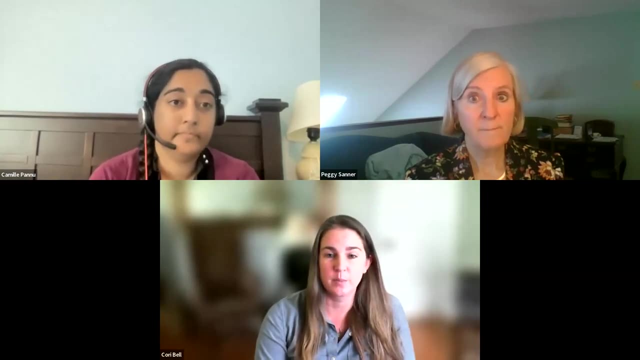 of the mix. Yeah, I know that this comes up quite a bit in the microplastic and in the PFAS context too, with air deposition of these pollutants. That's right, It's something you have to consider with a lot of these. 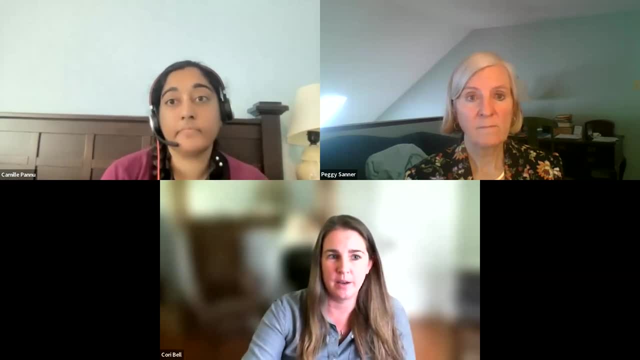 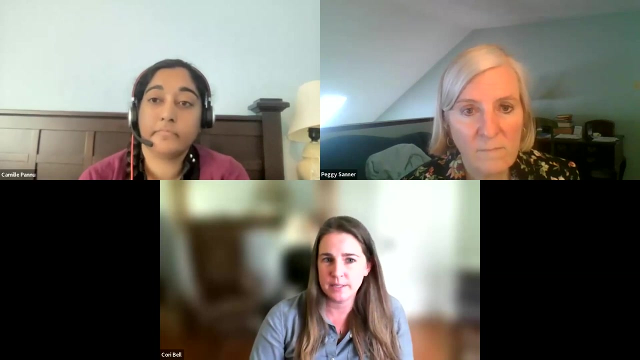 Moving on, there is a question for you, Peggy, about the interplay of pretreatment programs and exceeding TMDLs. So this person is asking whether, through the 303D program, Are pretreatment programs mandated where discharges have been identified as exceeding the TMDL. 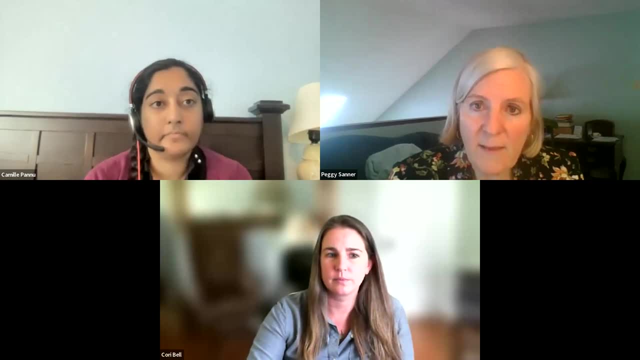 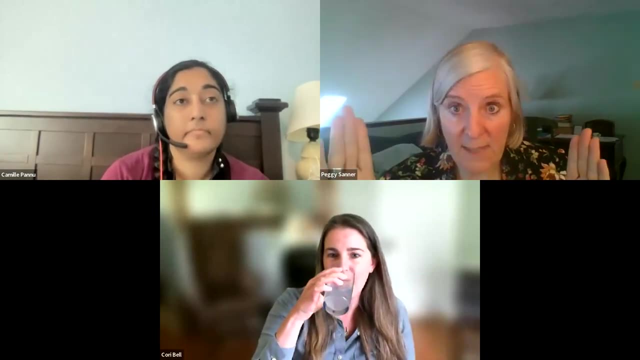 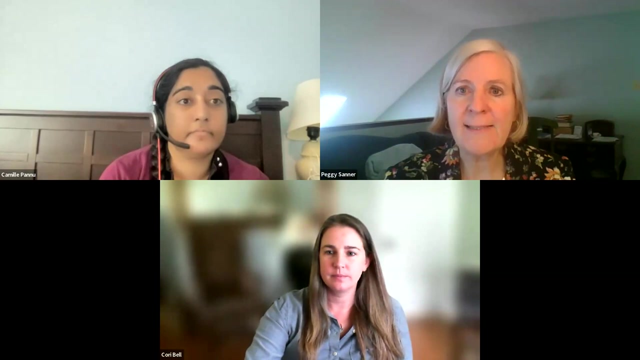 So that's a really interesting question And I will say that this is kind of the way it's conceived of, and I'm not saying it always follows this pattern, but in a TMDL context the idea is: you know, you have an impaired. 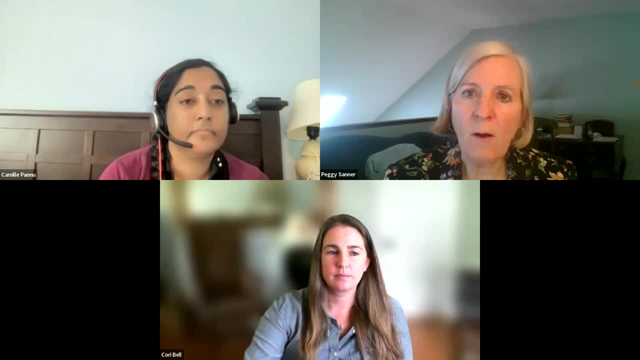 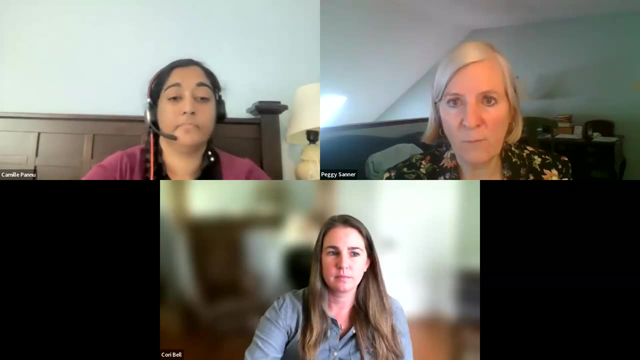 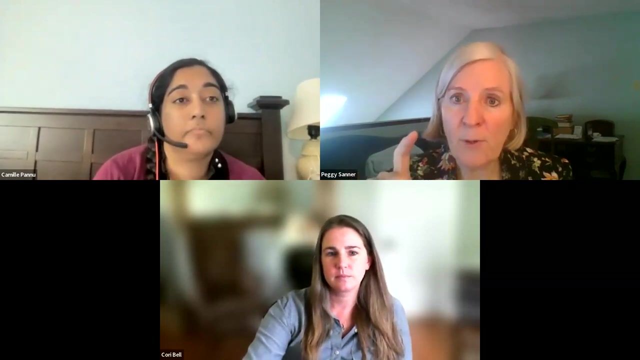 stream, an impaired waterway, All the pollutant sources are identified and added up and in a theoretic way- and hopefully in a real way, the point sources are each given a permit and that permit sets the level of the pollutant that that facility is allowed to discharge. 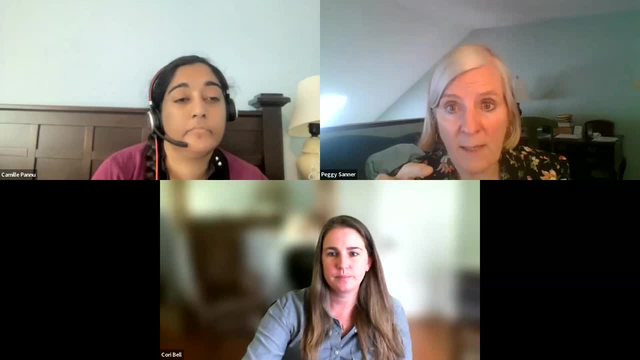 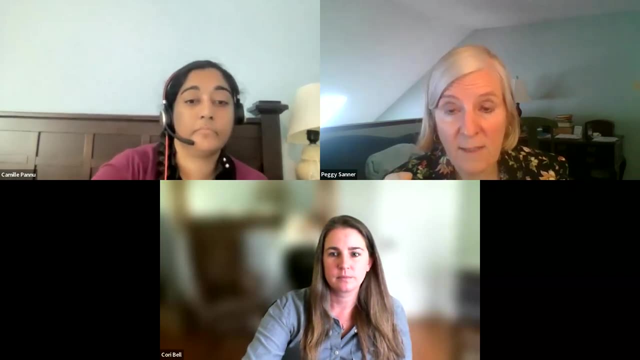 And in a TMDL context that should mean that the level of the pollutant that is allowed to discharge is the level that requires pretreatment. In other words, the facility has got to treat its effluent so that the pollutant is eliminated. 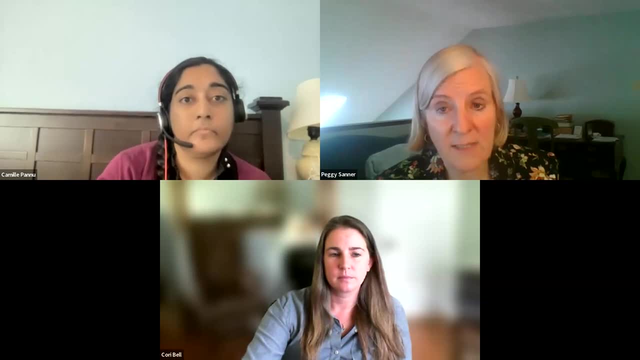 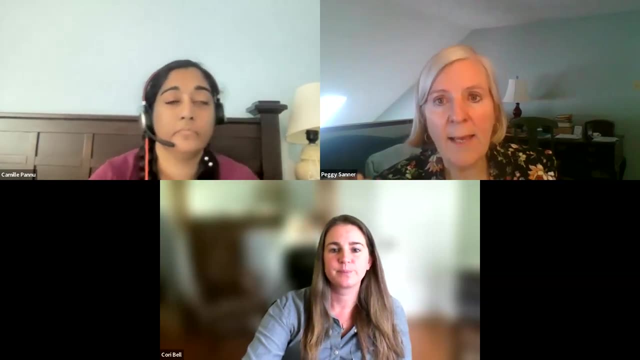 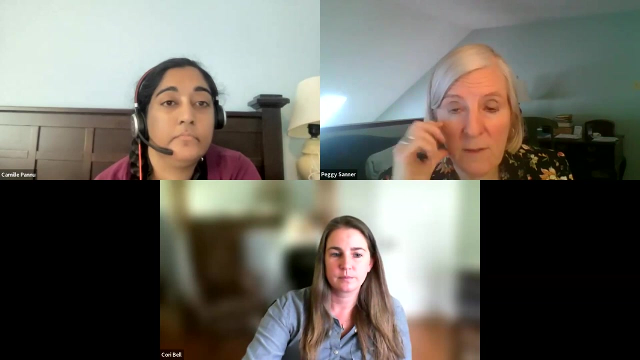 or at least reduced to the level that's acceptable to the TMDL. So that's the theoretic model. doesn't always work that way, and so just again to talk about the Bay TMDL, which is on a larger frame. 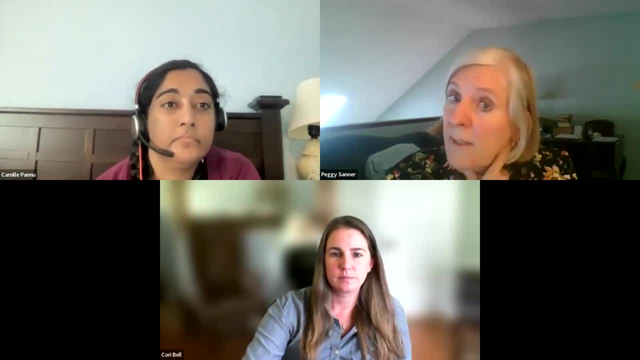 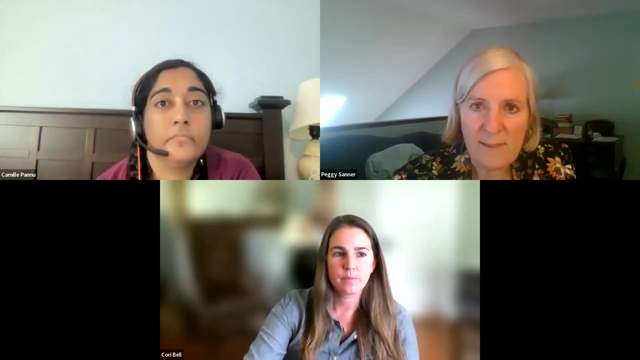 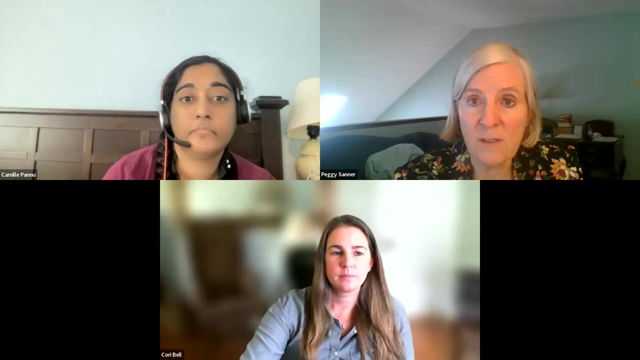 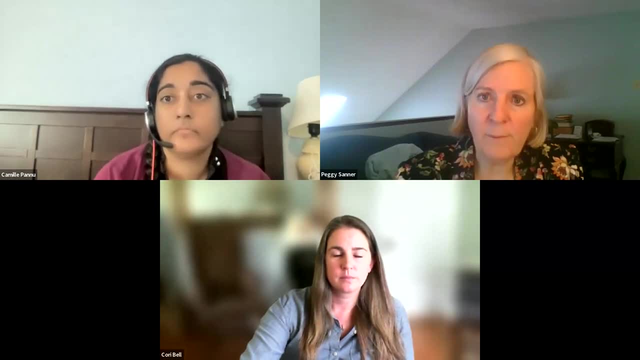 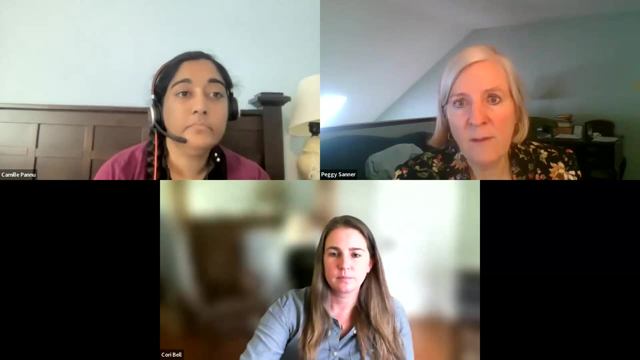 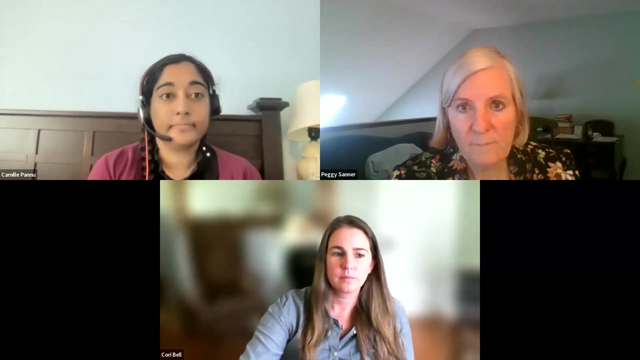 source. so they know whereysz all the pollution pipes are. Right, It didn't fit into that전에. nobody's going to be completely dwell upon that product until they do it. unfortunately, So formally this would be a temporary treatment for a point source. 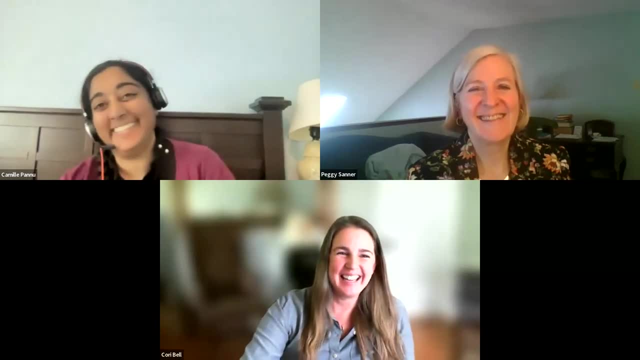 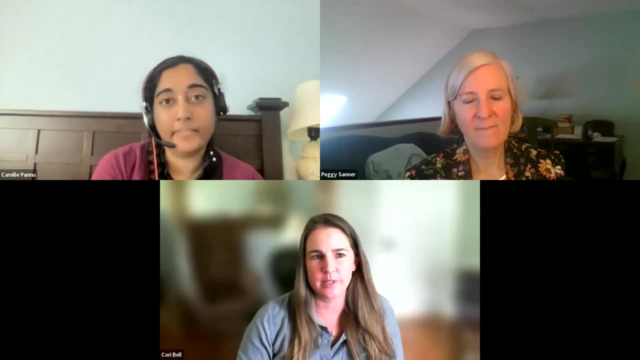 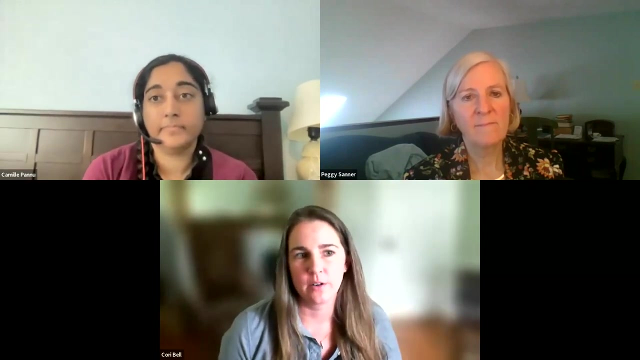 Does that make sense? I'm not sure. exactly Great So, Peggy, there is another question that I think you covered in your presentation, but I want to ask it just in case, And this is whether agricultural stormwater runoff is considered a point source. 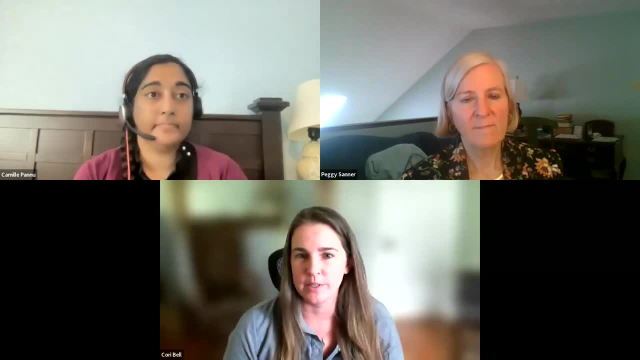 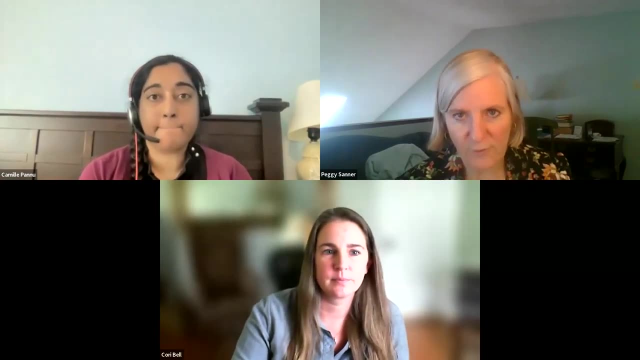 And I believe you answered this as being no, unless it's a CAFO. Is that correct? That's generally correct. That's right. CAFOs are definitely. at a certain number of animal units, they are definitely CAFOs. 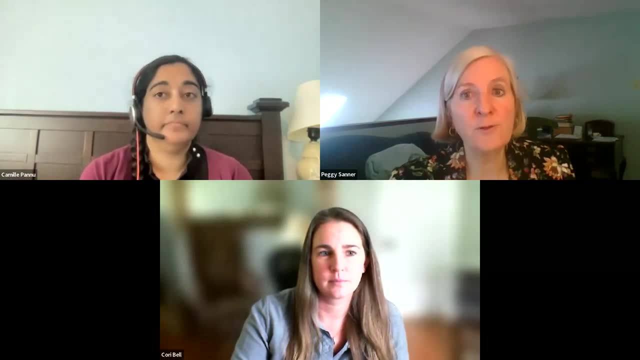 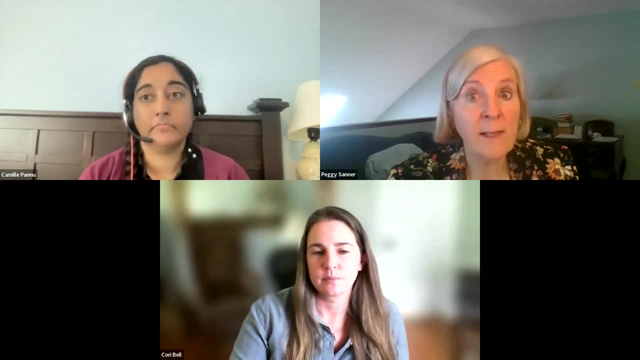 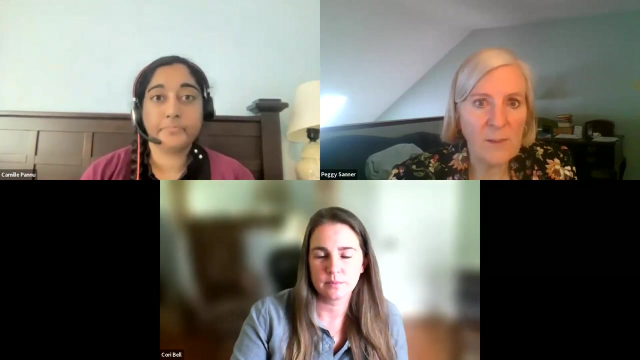 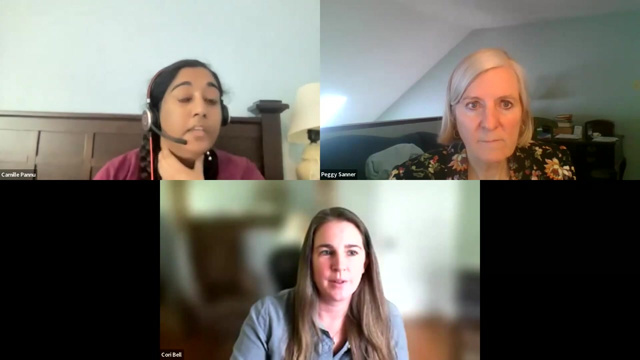 But apart from that, agricultural runoff is not a point source, It is a non-point source, And so it is subject, if at all, to programs that the state may impose, And not under the Clean Water Act. Thank you, I have a pretty specific question for you now. 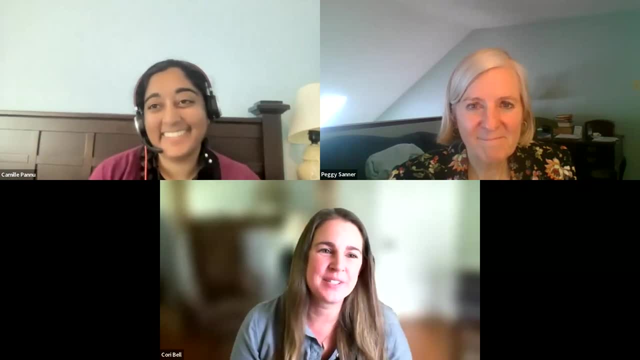 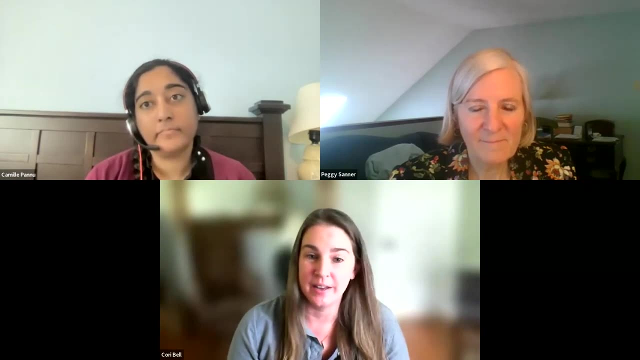 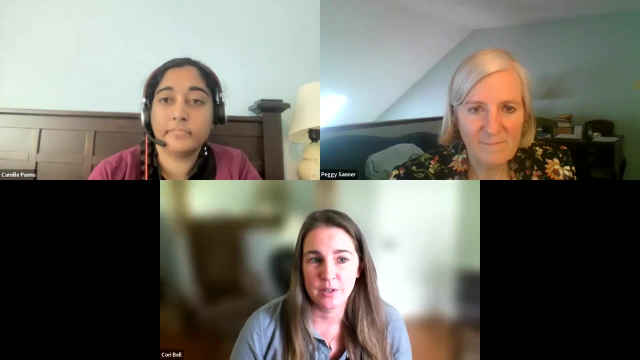 Uh-oh. So this is someone's asking whether there, if there is an administrative order of consent with EPA and in this case with the State Department of Health- I'm guessing it is State DOH- would this agreement an administrative order of consent? would it protect against a third-party lawsuit? 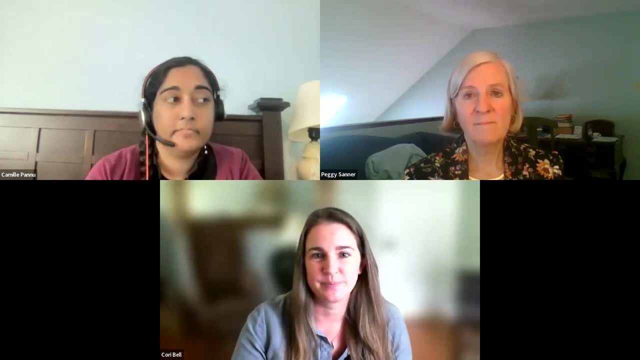 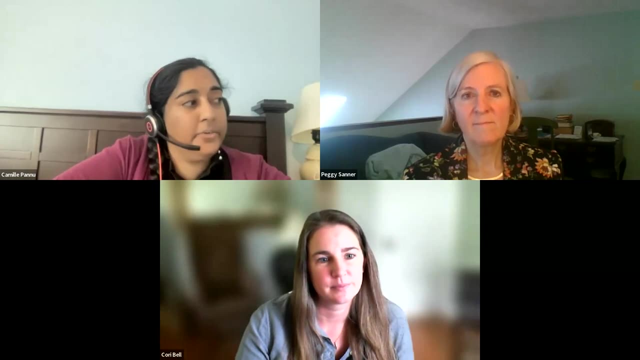 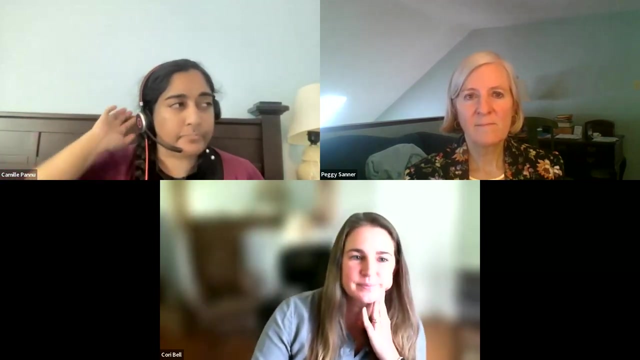 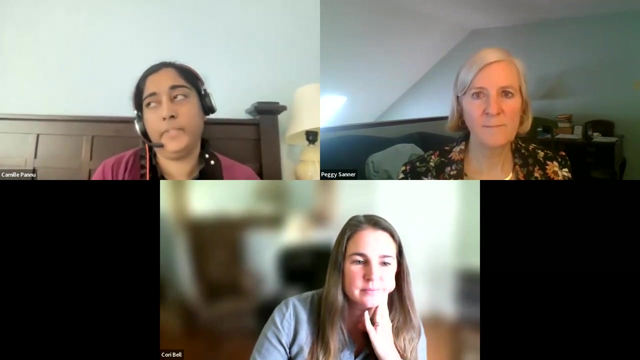 Would it protect against a citizen suit? Oh, that's a good question. I'm not sure. I'm not sure because I'm so where I'm stuck on, this one is standing. I don't know what you think, Corey, but um, and the reason I'm stuck there is because I don't think it necessarily would preempt a citizen suit, but you would have had to have protested the administrative order in some way. 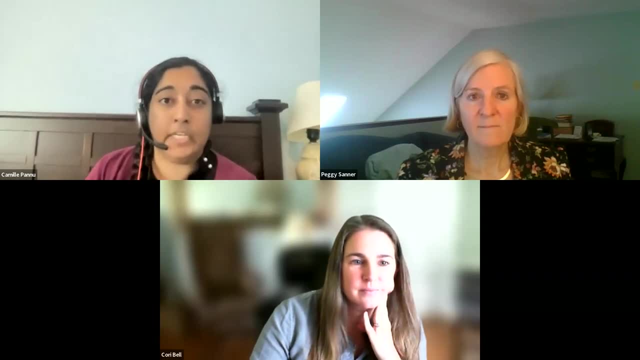 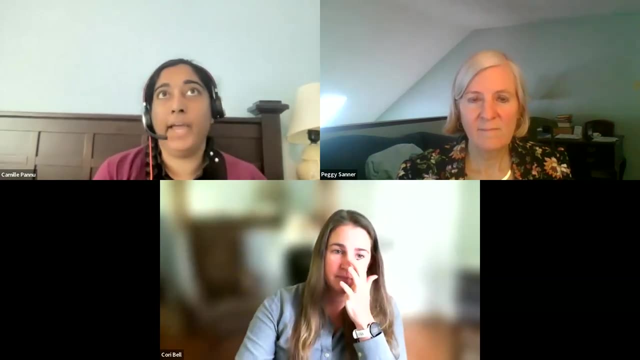 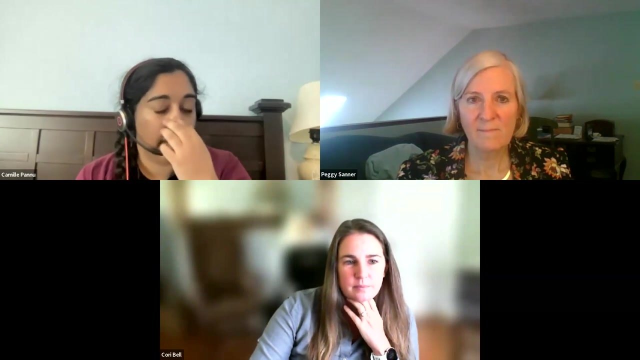 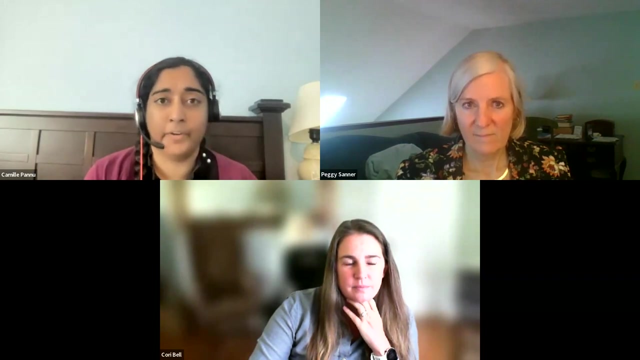 And I think it's really hard as a third party- like generally speaking third parties- can't intervene in an administrative order process in that way, And so I'm just I'm not sure there's a legal path, I'm not sure there's a legal pathway or a hook, but I'm also not a Clean Water Act litigator specifically. so, um, I'd be happy to come back, to like to ask around and follow up with um, with folks, but I I think the answer is it shouldn't, but as a practical matter it might, because there might not really be an avenue to challenge it if you didn't challenge it early on and if there's not a public process for challenging the administrative order. 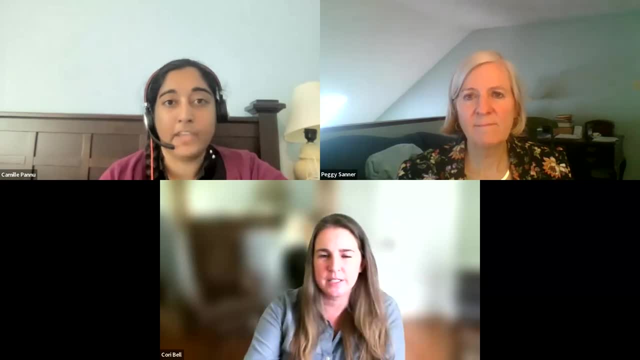 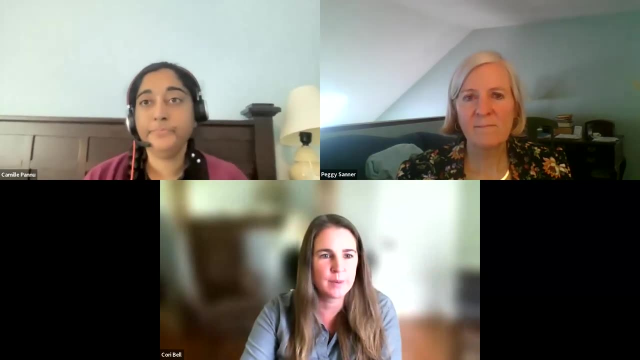 Yeah, I think we might need a little more detail to answer this. Peggy, do you have any? Yeah, I think we just need more information, so feel free to drop more information in the Q&A section and I can follow up. 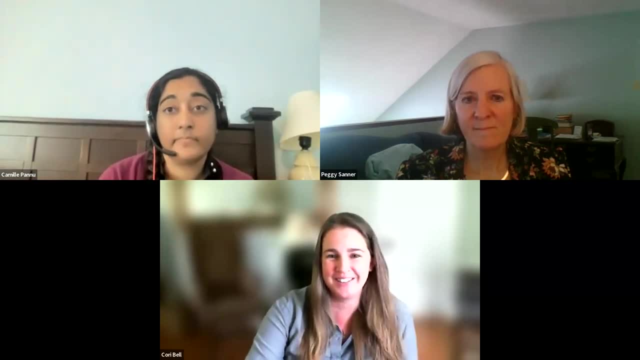 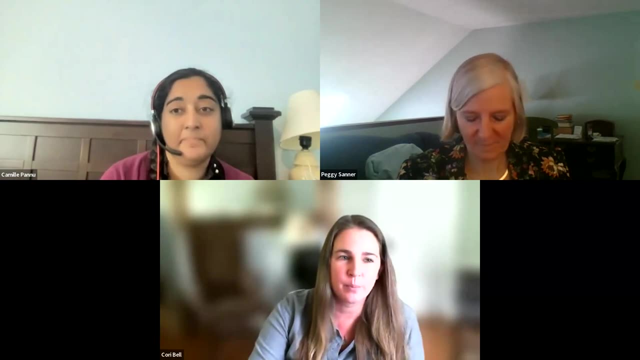 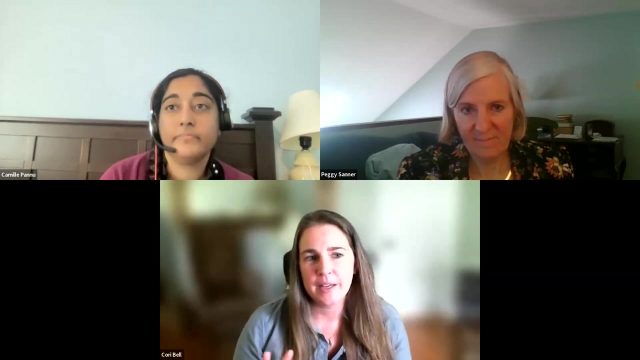 So there's a lot, of, a lot of questions on SACET, which is not surprising, probably half of what we've received so far. but there's a pretty broad question that has come up in a different, in different questions, and it's about the 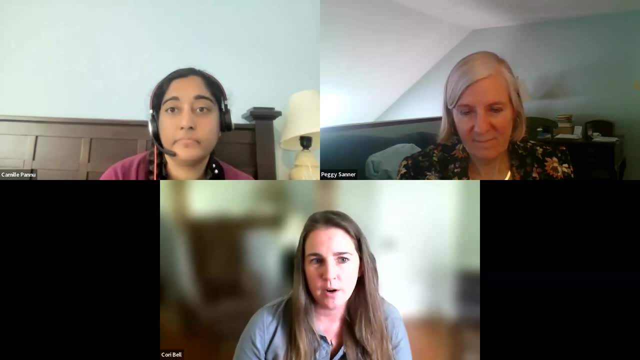 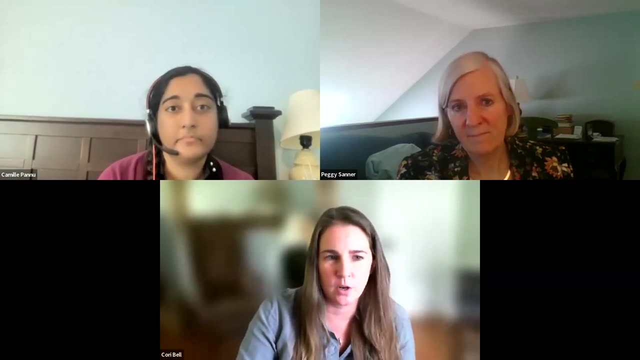 interplay of the definition of a navigable water and waters of the United States and how that's tied to commerce and the Commerce Clause. and I think, Camille, you had talked about that in your presentation, so could you just give a quick overview of that again? 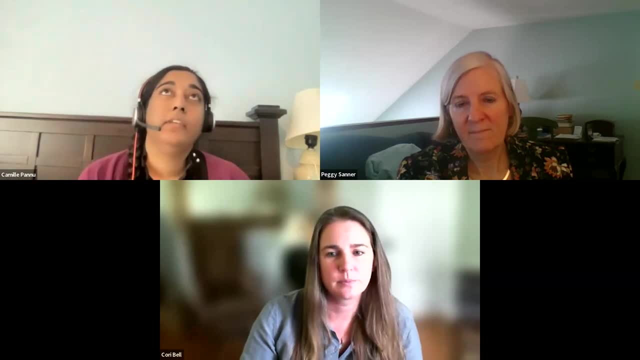 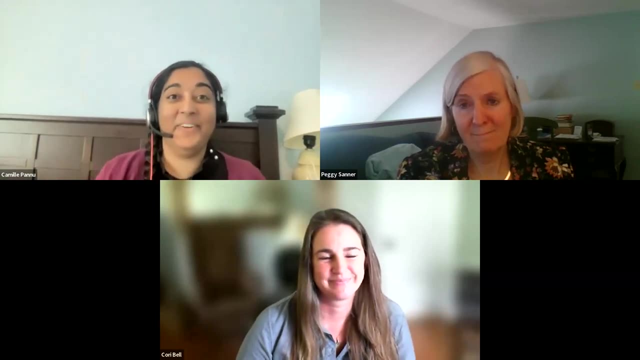 Sure, so I think, um, so the Commerce Clause is about one-third of what you study in a constitutional law course when you're a law student. so, and then it'll come up again and again and again, including an administrative law. 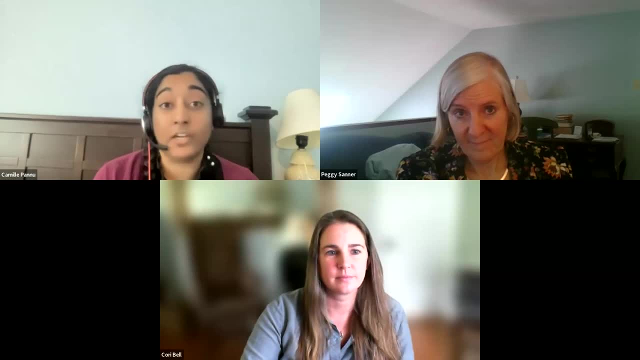 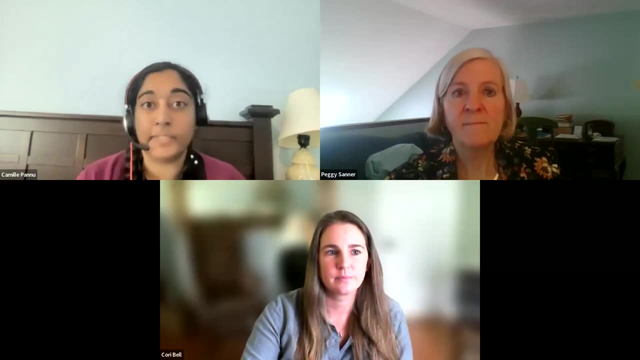 So my caveat is that the like the Commerce Clause is even how we have criminal federal crimes, for example. So I want to caveat this by saying that a lot of things are lumped under commerce that are not what you and I would traditionally think of as business or commerce. 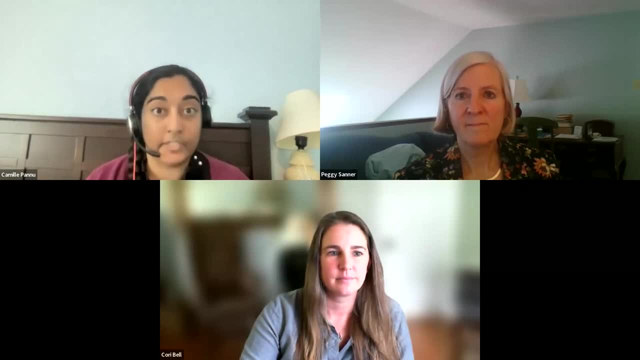 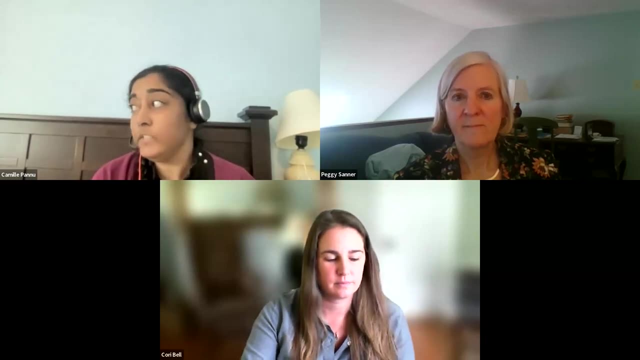 So commerce is kind of broadly construed. it is related to the movement of goods or people- I think that's like a fair way to think about it- or the provision of services. So so I would hold that as kind of your background about how we're doing this. 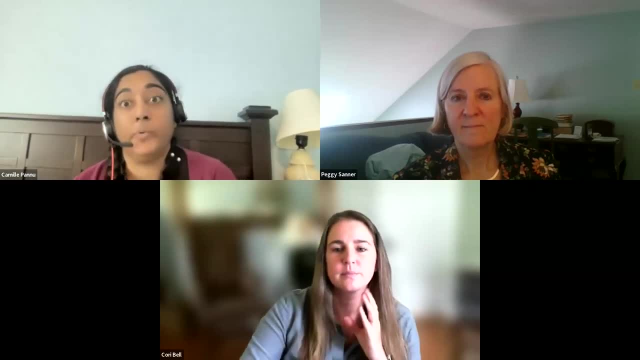 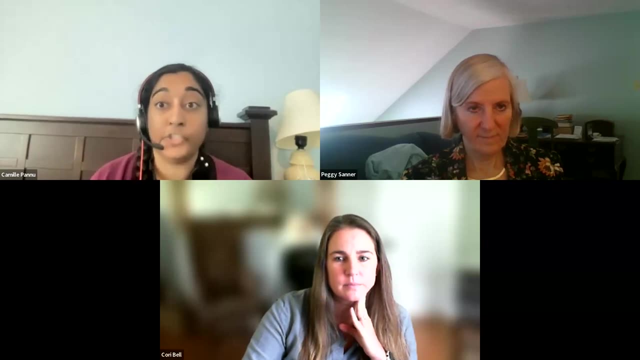 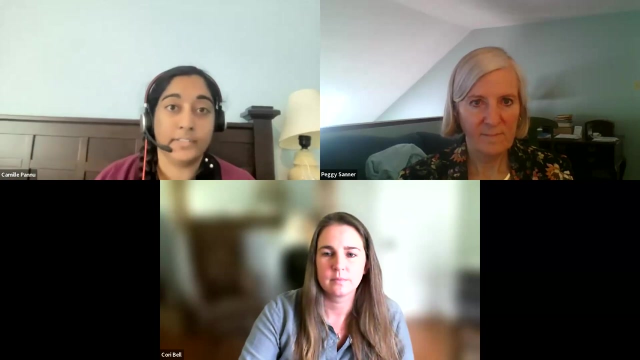 So the concept of a navigable water and its interface with the Commerce Clause and the idea of commerce, um, it exists, because way back in the day, when we shipped goods, we shipped them on boats, basically. um, you know, ground transportation didn't really exist, we weren't trucking things. if we were moving stuff over land, it was like in a caravan style, with horses or oxen depending on where you were going, so, and we didn't have railroads. 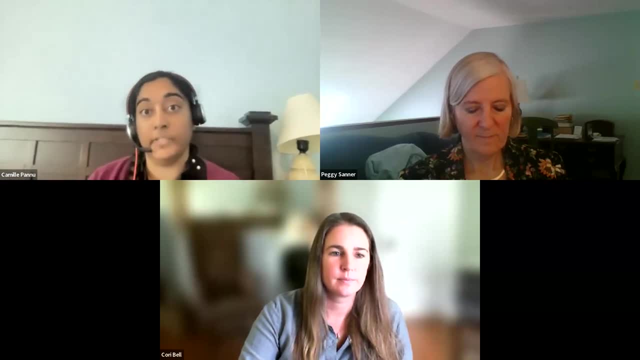 So most of what we were shipping at the time. So most of what we were shipping at the time that the Constitution was written and when they were thinking about the Commerce Clause was, you know, we were making canals, we were moving goods through shipping. 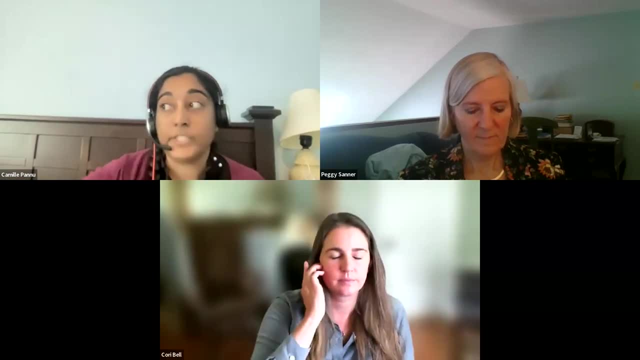 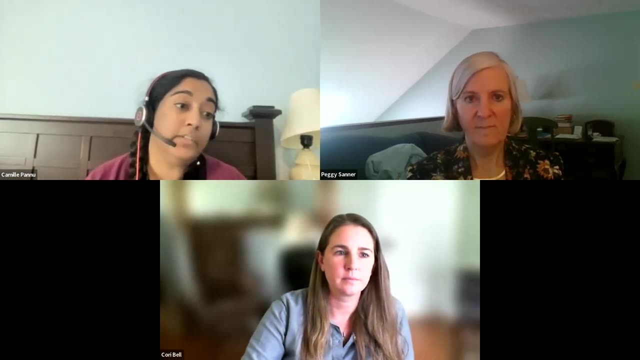 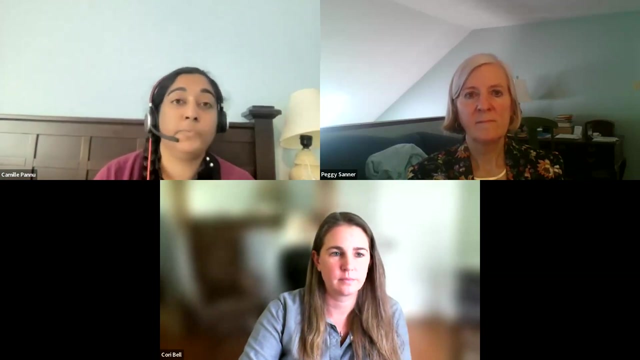 So that's where the idea of a navigable water comes from. Over time, Congress and the court, the federal courts, have upheld this or expanded this, including the Supreme Court. there's been this idea that there are certain other non like business related, but commerce and the idea of, like folks, being able to move and enjoy resources and transfer from one area to another. 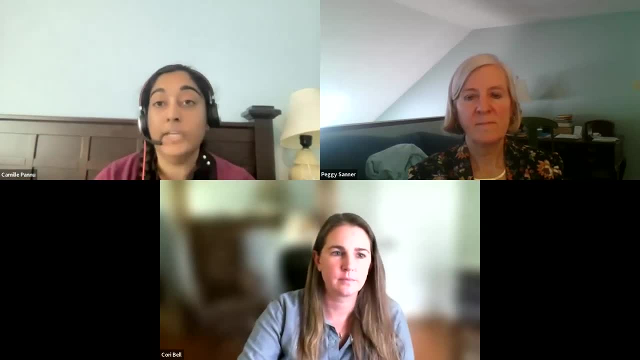 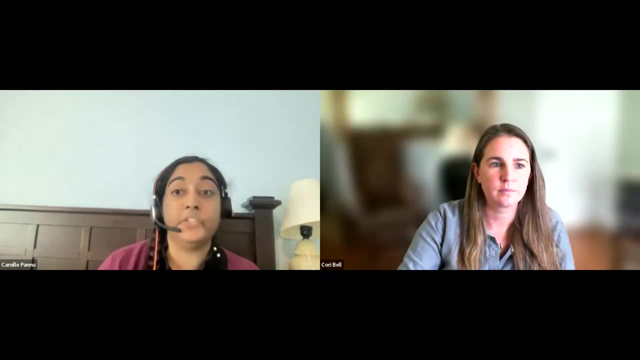 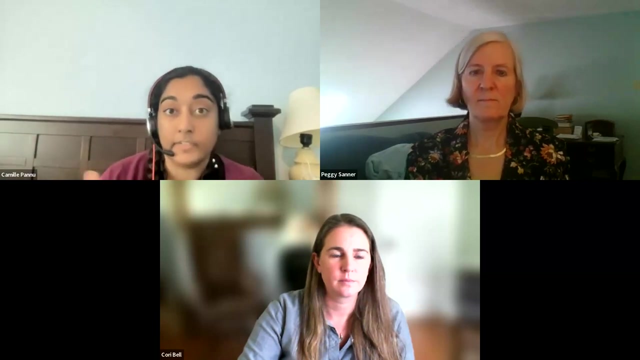 from one state to another, like just humans like you and me- That some of that comes under the Commerce Clause as well. some of it comes under certain amendments, but a lot of that comes under the Commerce Clause. So the idea of a navigable water is historically rooted in the idea of you could be shipping things, but over time has developed and certainly since the 1970s there's been a lot of case law that has expanded it so that it includes water systems instead of thinking solely about you know, can I put a boat down a stream? 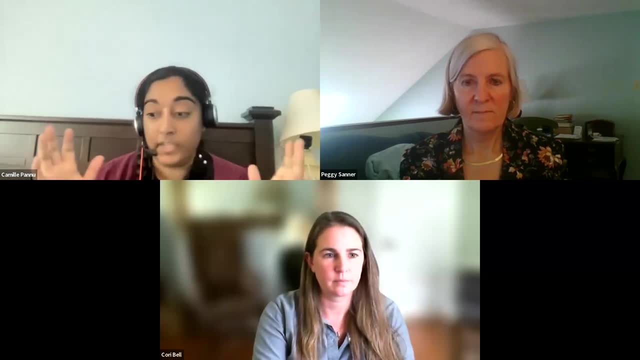 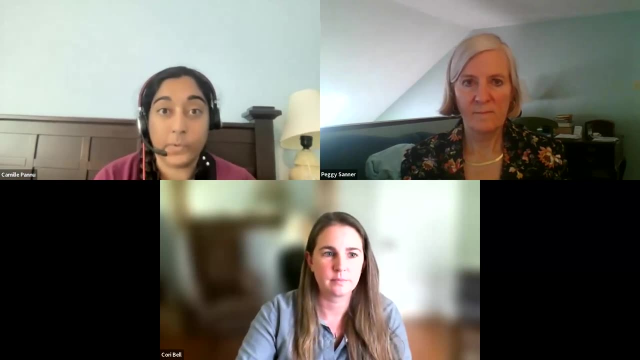 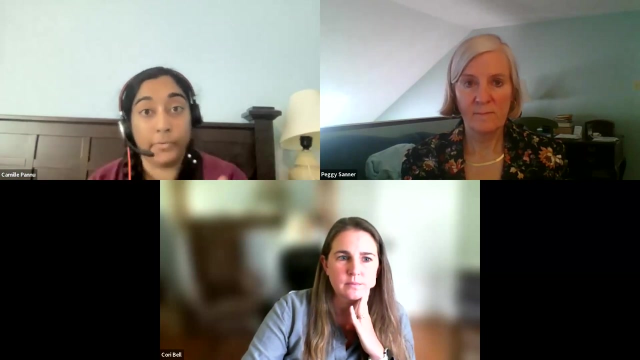 And so at the end of the Clean Water Act analysis, you do have to be able to put something into a navigable space, meaning, like you know, one day it gets to a water source that is involved perhaps in things going across states, but it doesn't have to be limited to like putting a boat in that space. 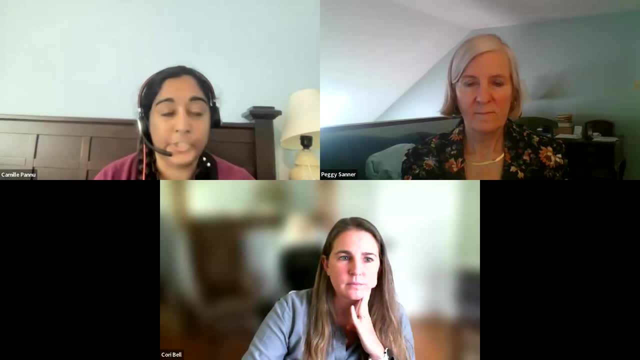 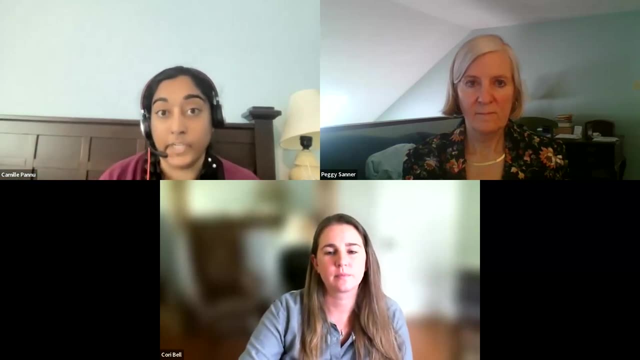 So, for example, the Colorado River. We don't see a lot of shipping on the Colorado River, but the Colorado River is really critical for energy production, particularly hydroelectric production, for several years, several states, And it's critical as a source of drinking water and irrigation water for. 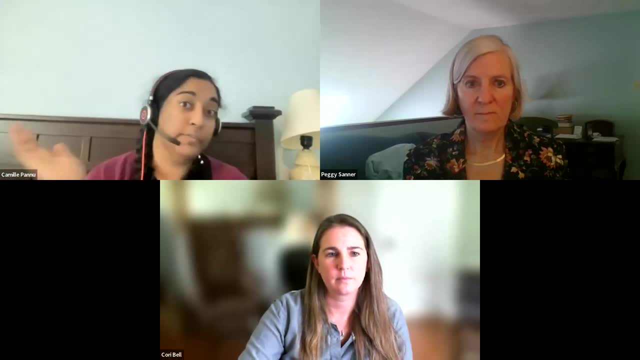 most of the Southwest, from Texas all the way over to California, All of the coordination that happens under that is a combination of the Commerce Clause power from the federal government and the states literally contracting with each other at like a sub-federal level to manage this. 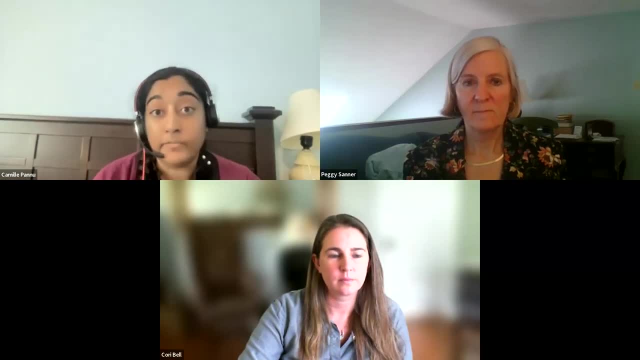 shared resource that's known as a water of the United States. So it's not involved in necessarily business commerce, but it is involved in activities that are related to the commercial process writ large and that are really critical for the health, safety and success of these. 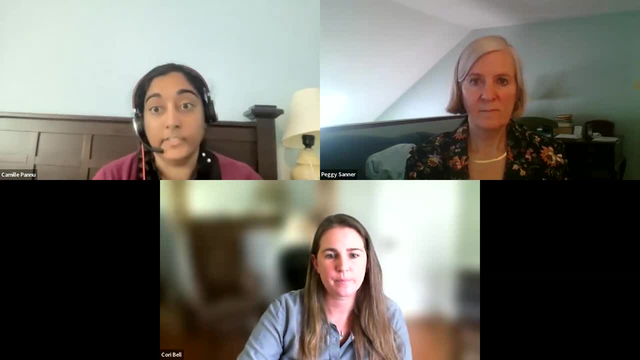 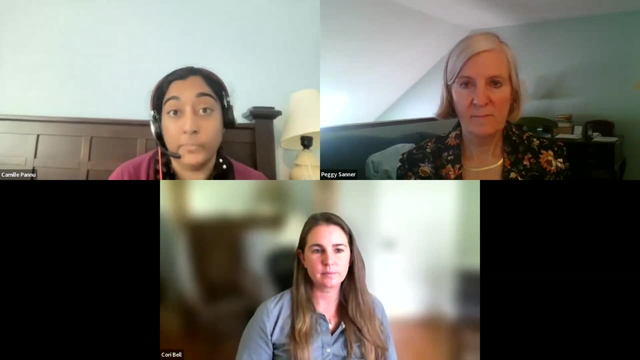 different communities at the local and state levels, And so I think it's important not to get too confined in how we think of commerce. but I think the question is intuitive and is a good one, because that's certainly how Justice Alito sees commerce. He wants to, like, narrow the scope. 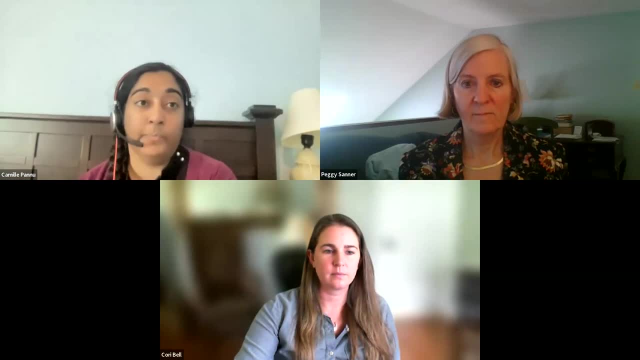 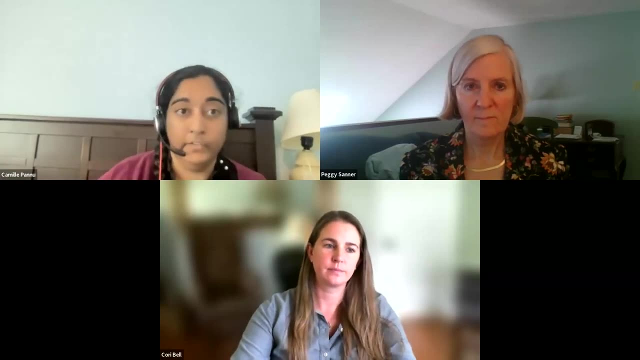 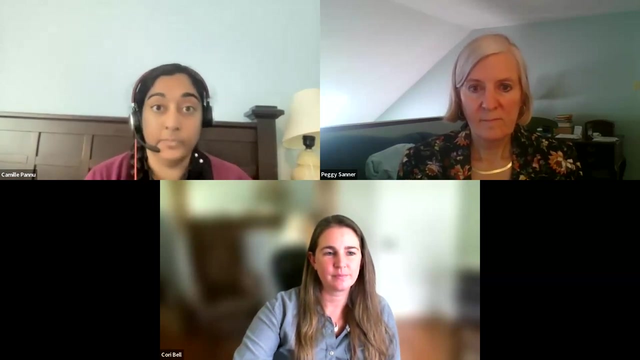 of the Clean Water Act to literally bodies of water that you can put a boat on that are probably crossing state lines And that's not consistent with the development of law around environmental protection and water. but it's certainly consistent with his prior opinions where he just thinks the federal 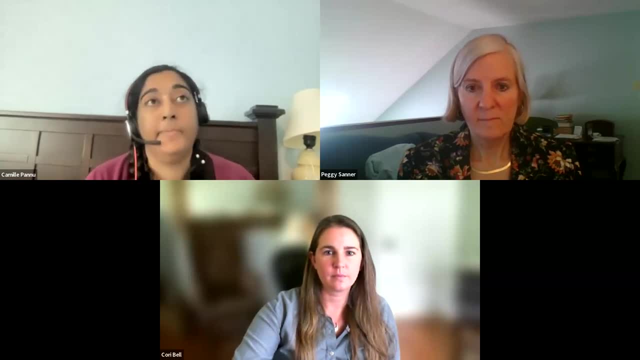 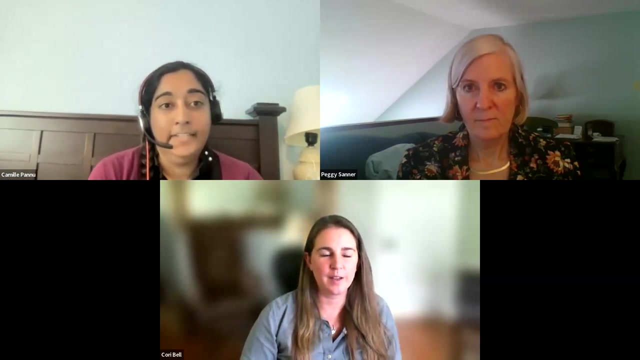 government should not be involved in. That's maybe an overstatement, but I feel like he feels like the federal government should not be heavily involved or not have as broad of a scope to be involved in environmental protection. Thank you for that. Yeah, I don't know if that is helpful. It might be an unsatisfying answer, but 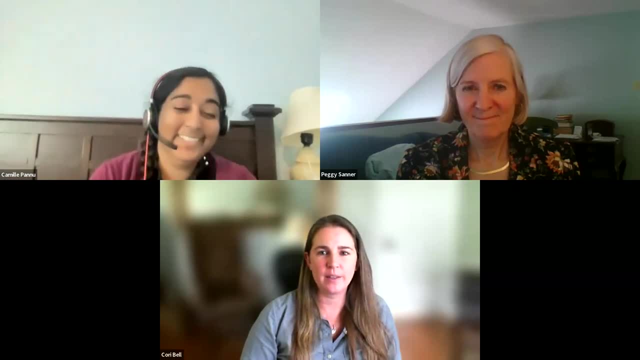 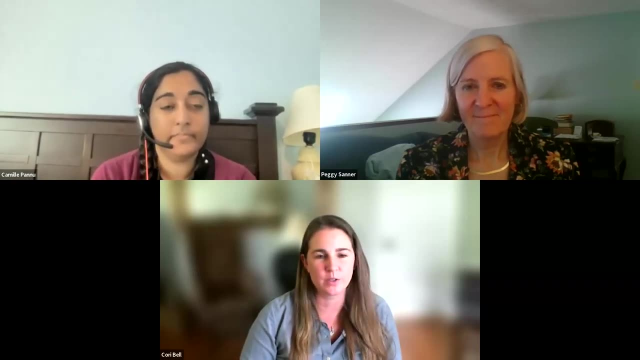 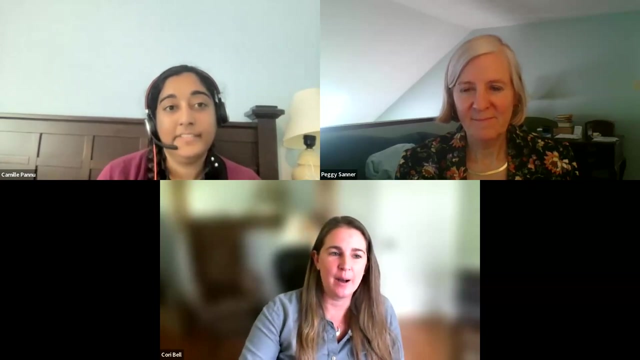 No, I think, I think that it was really helpful. And yeah, especially if you're a non-lawyer, when you hear commerce clause, you do not. you do not think about how broad that actually applies. Peggy, I'm going to turn to you now about questions about SACIT and how SACIT might help this. 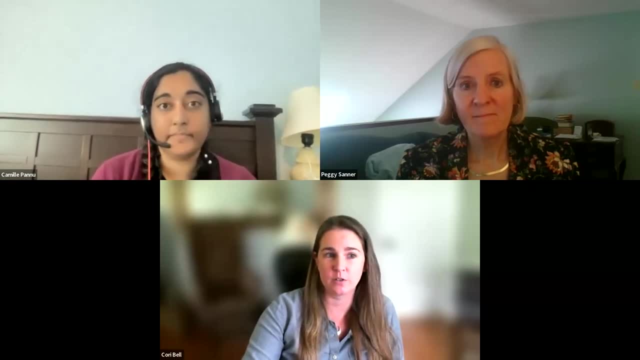 Okay. So, Peggy, I'm going to turn to you now about question about SACIT and how SACIT might help. this, Okay, might affect restored wetlands- Whether or not restored wetlands might be protected or not protected now under Sackett, and what factors might be considered when you're trying to determine. 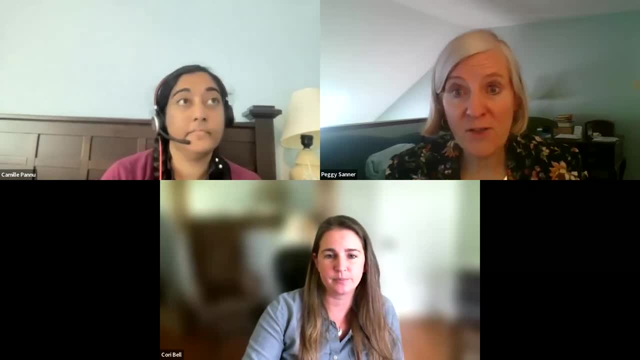 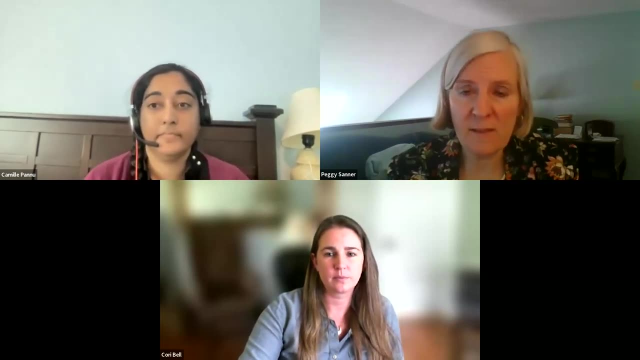 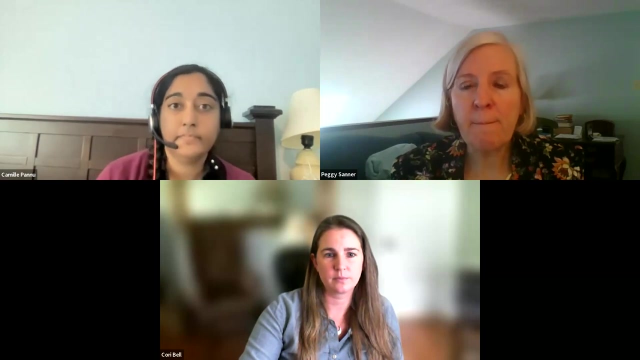 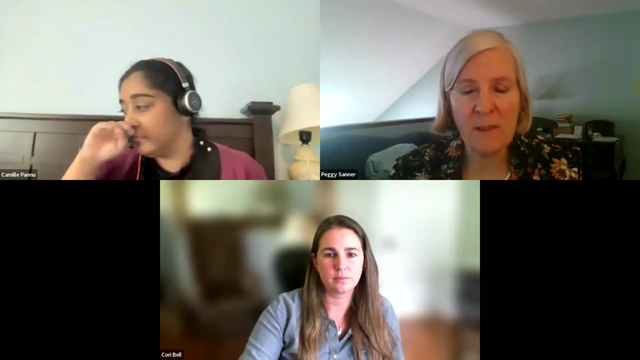 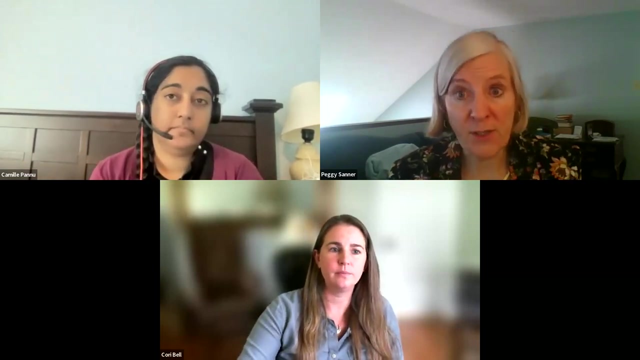 whether they are protected. Great question. As we see on the landscape now, restored wetlands are probably gaining more and more importance historically. for those who don't know, I mentioned where you have a project that could impact in existing wetlands. There's a requirement under Virginia and, frankly, federal law that the project to the extent 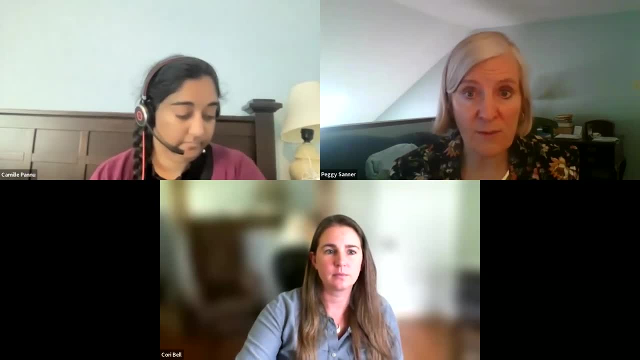 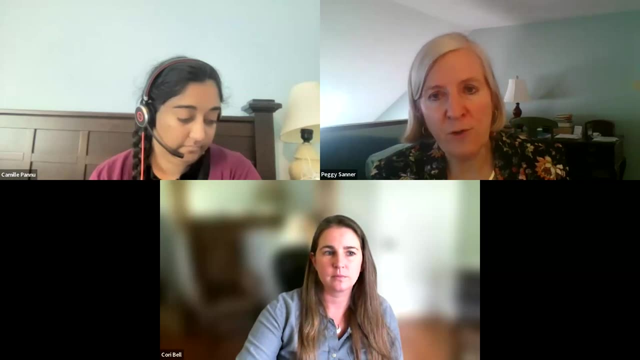 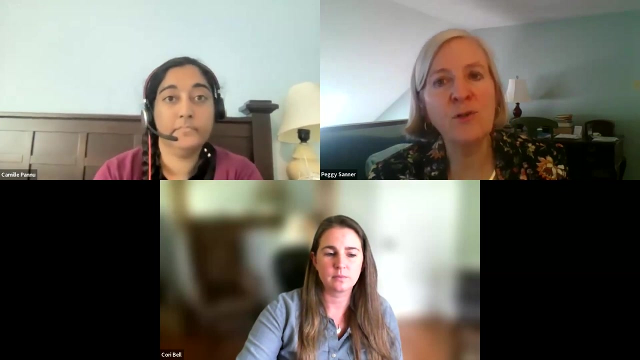 possible avoids making those impacts, minimizes those impacts and compensates for those impacts. The compensation can take a number of forms. One of the forms is to build or restore a wetland, In other words, to add to, if you will, the wetland stock in a region. 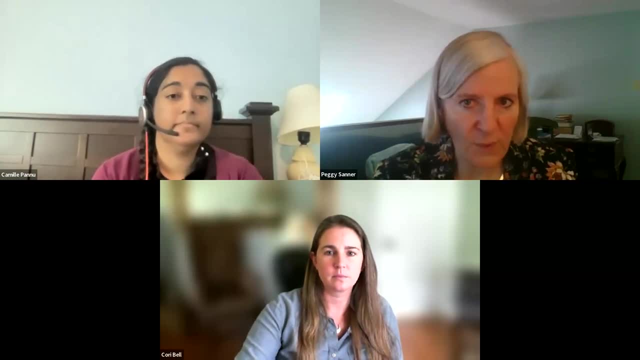 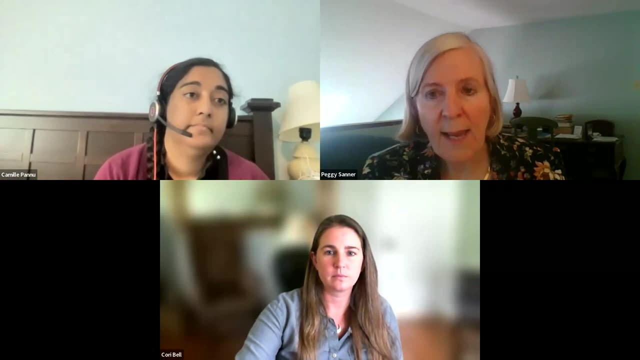 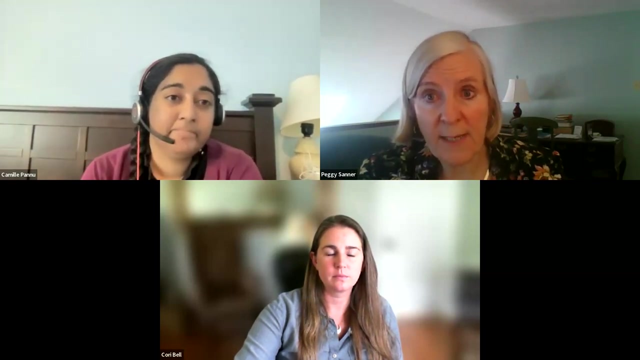 and then typically protect it by putting it in what is, in essence, a conservation easement. That's one way that you get restored wetlands. As development grows, the demand for restored or newly created wetlands also grows. We will see more of that. How are they affected by? 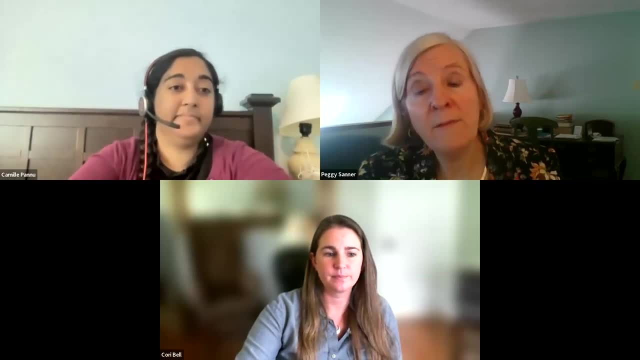 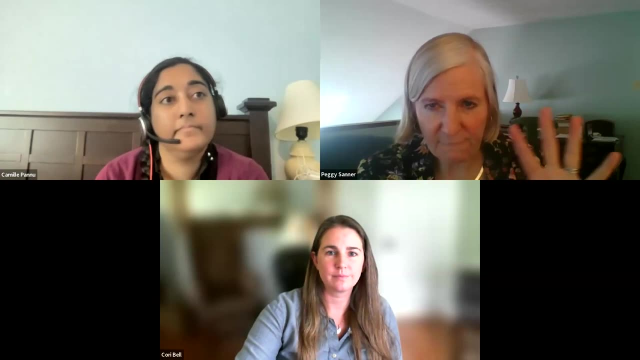 Sackett. Much of this will depend on where they are located, because the Sackett test- again, many of us are all trying to figure out how all this is going to happen, but the Sackett test, generally speaking, is that a water body, wetlands or otherwise must be connected. 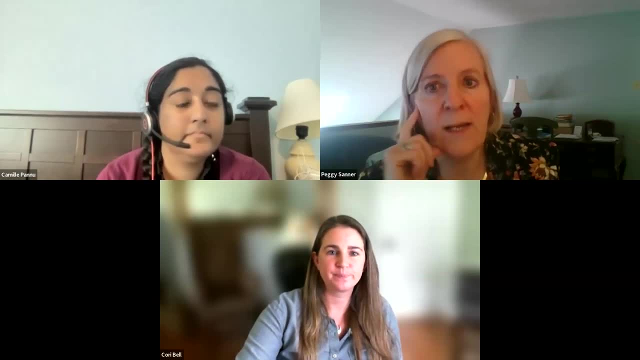 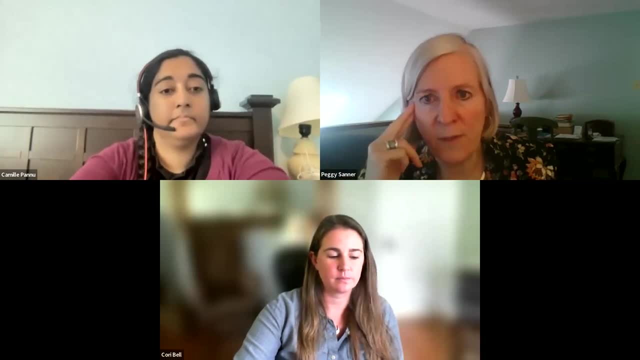 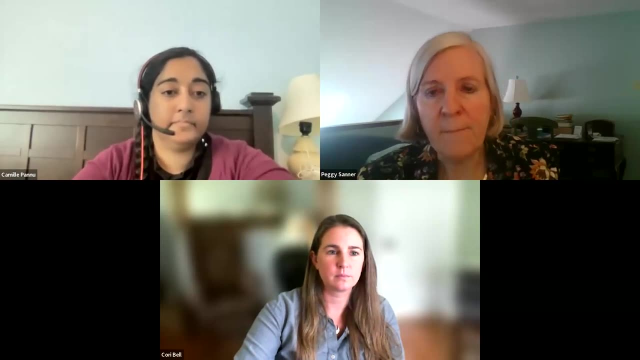 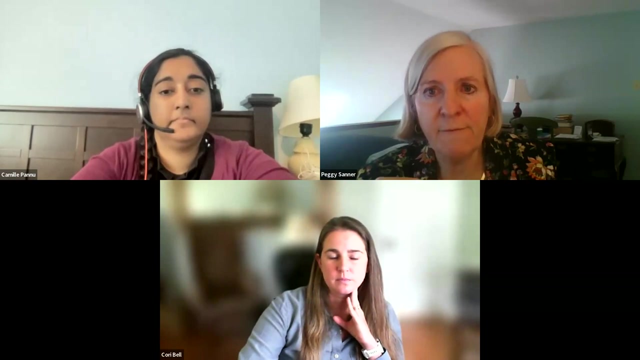 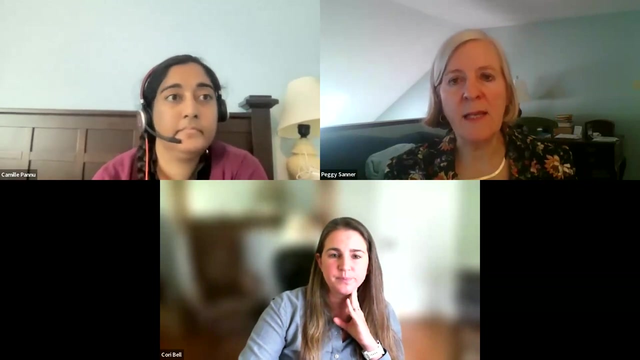 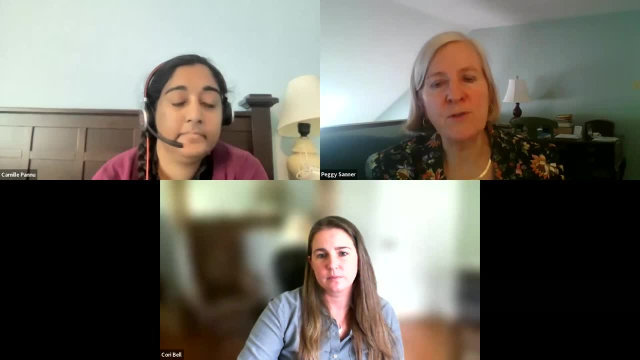 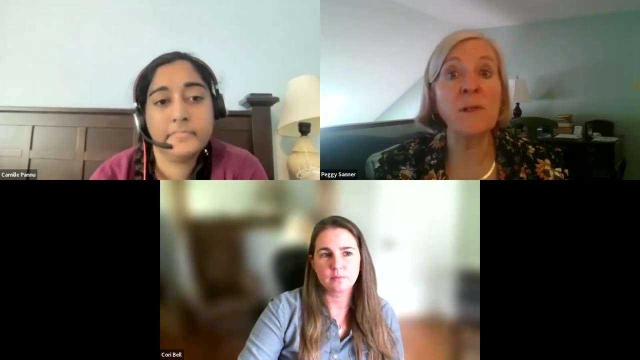 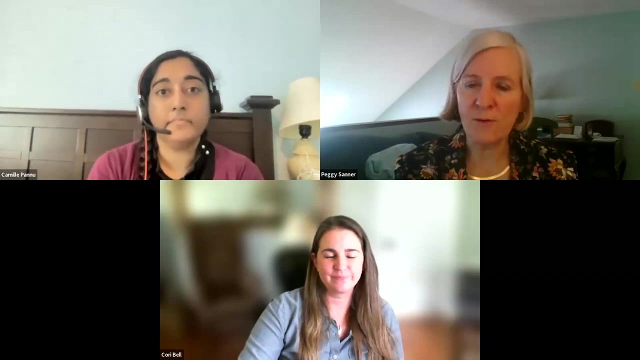 So I think they are not the area of most concern in terms of what SACET can do to our loss of wetlands broadly, but I think it's a really thoughtful question and I think we'll see that it's likely to require some more thinking about and also to see how that plays out in different landscapes with different climates. 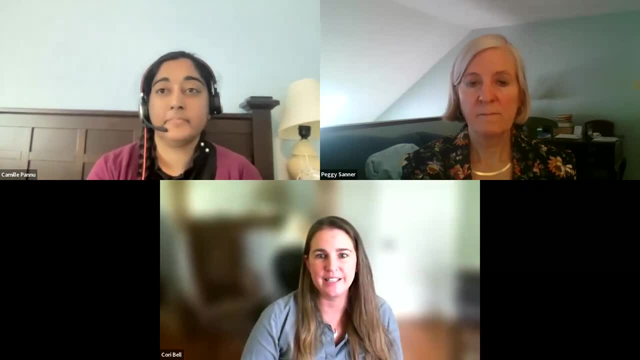 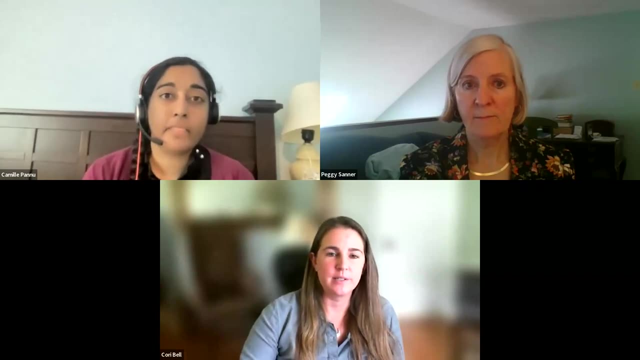 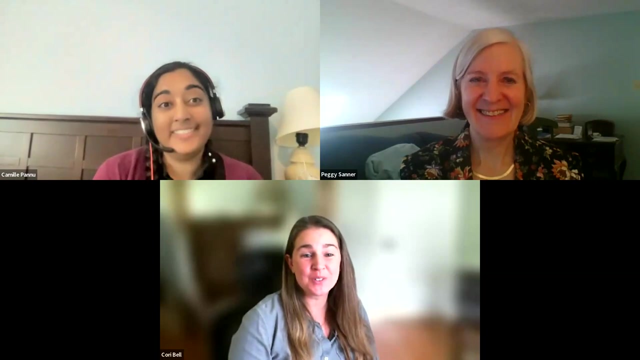 Yeah, I think a lot of this is just going to be wait and see, And a question that is related to that for you, Camille, is how might the term relatively permanent be applied to a lot of- yeah, exactly a lot of- those that you were showing, you know, the wet, the arroyos, the intermittent stream? 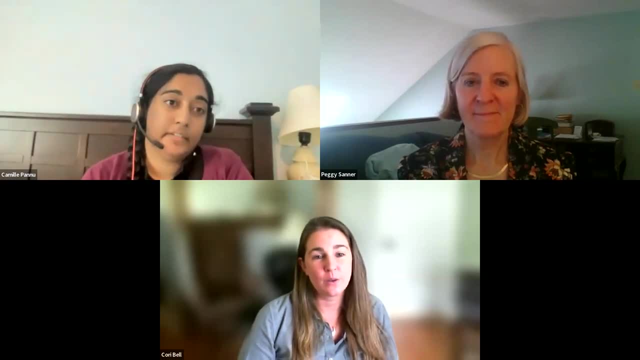 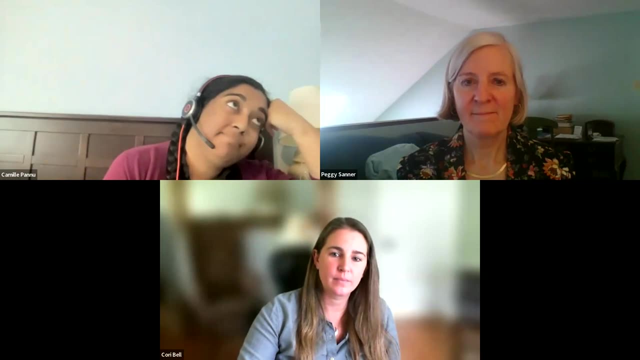 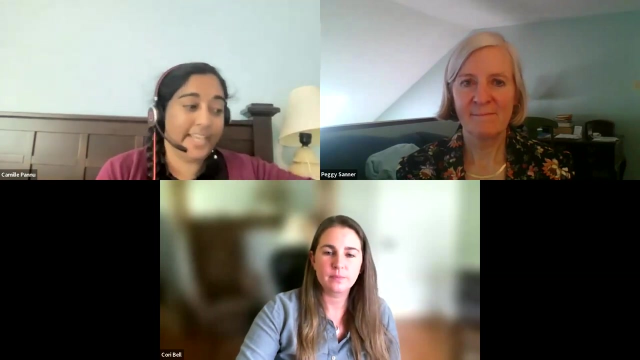 how do you think those might fare under SACET? Yeah, I mean, I think there is a way in which they could fare not badly. and here's how I think that Congress or EPA could ask states to designate which waterways are relatively permanent and, for example, set like Waters of the United States, kind of through a more collaborative process. 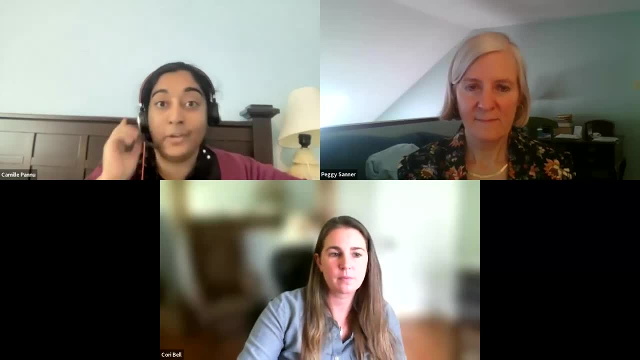 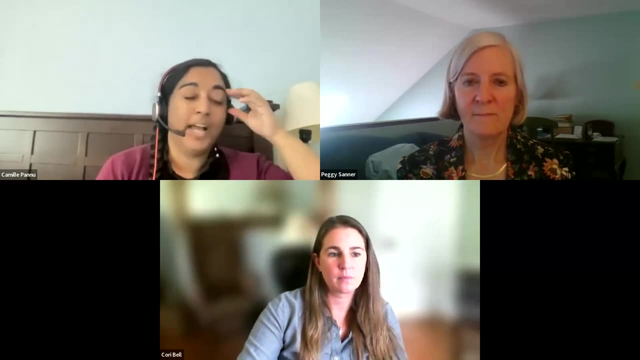 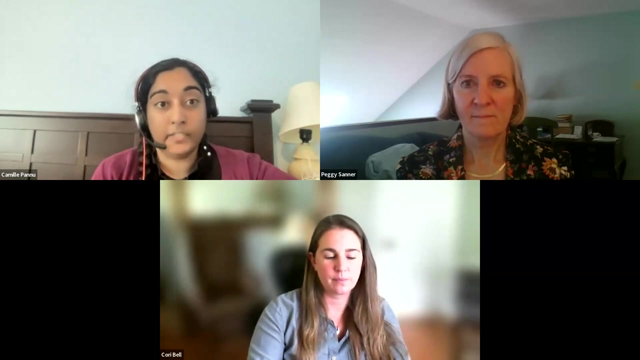 I actually think that might work in conservative southwestern states like Arizona will tell you what an arroyo is and they won't build in it. and it's interesting because I think a lot of people. I think one of the things that's going to be confusing is that SACET is based on Section 404, which is about filling in land. 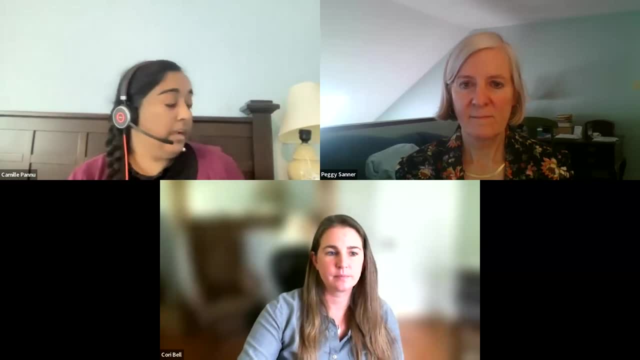 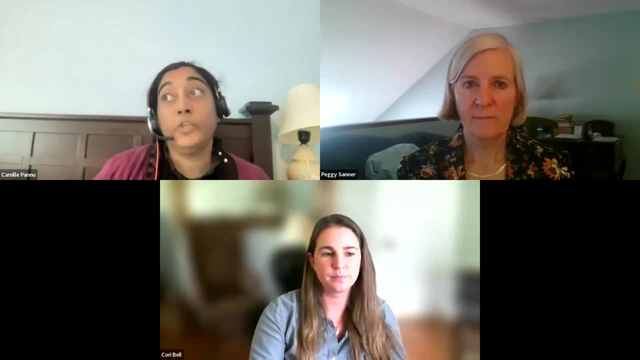 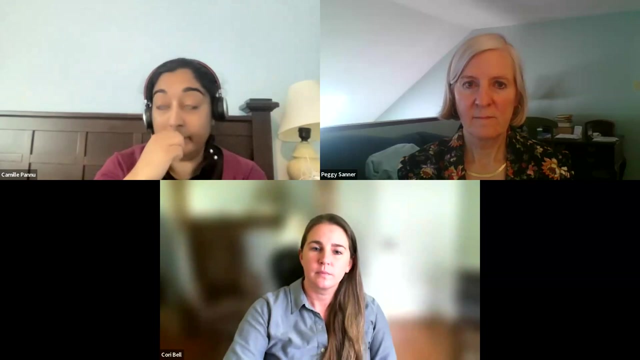 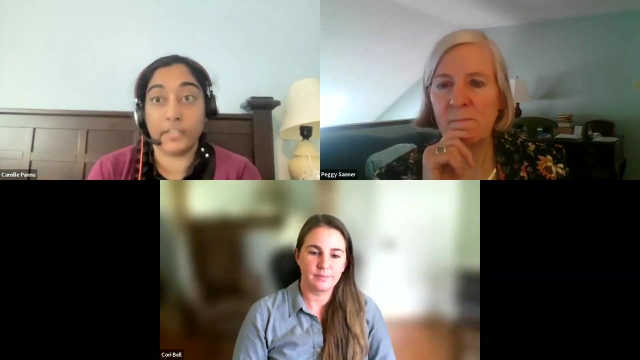 It's not based on like this permitting system, but the fear is that, because navigable waters is used throughout the act, that a definition of one section will be applied to the other sections as well. So so another good example of like something that I have never seen have water in it in my entire lifetime as a Californian is Tulare Lake, which used to be the largest inland freshwater lake in the in the country- literally the country- and 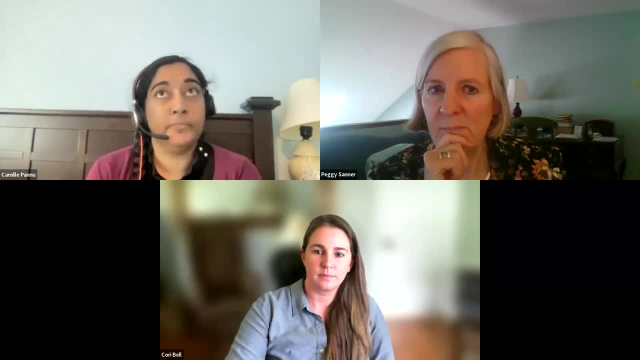 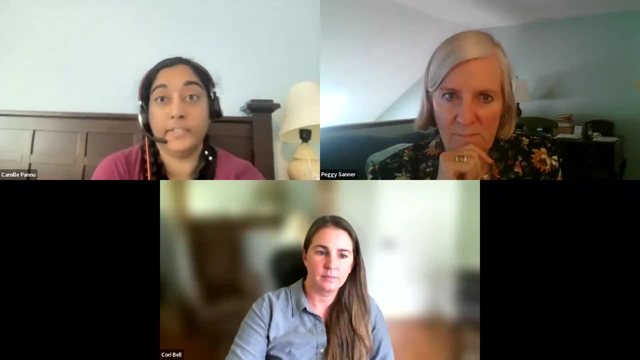 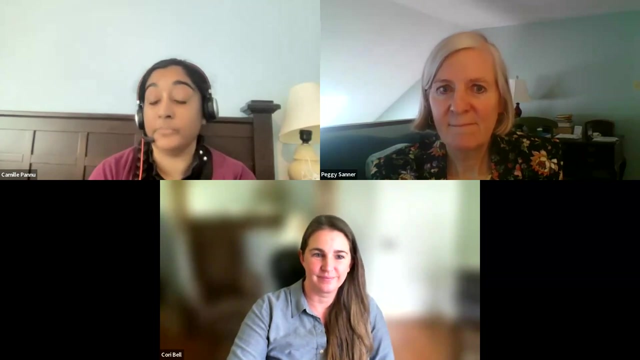 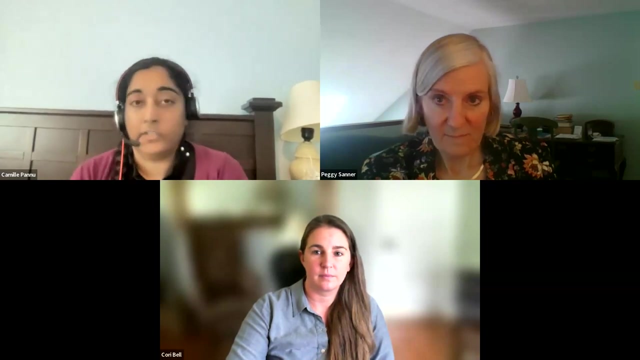 went dry, shoot, like decades ago before I was born, in 1983.. Tulare Lake was dry before then and it went dry mostly because it was siphoned off for agricultural purposes. This year Tulare Lake had water in it and it became an issue because people had built into part of the lake bed. but the original lake bed has been preserved as a wildlife area and that became. that, I think, is really interesting, because there's a lake that hasn't had water for decades, mostly because of manmade reasons. it would have naturally had water but we've diverted the rivers, we've got massive irrigation projects. we've sucked all of the water out of surface water in California. 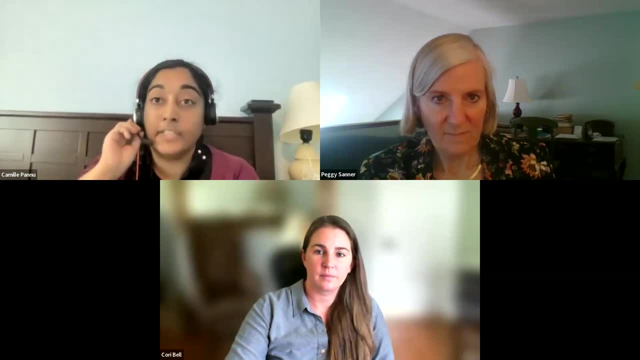 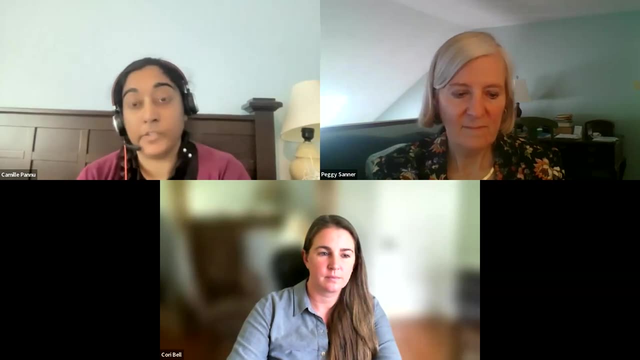 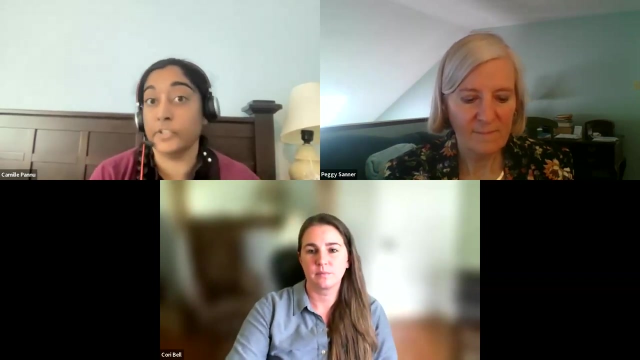 And you know, if you talk to people from the region, they would tell you Tulare Lake is a lake, even when it's dry, And so I think that's a really good example of what we're going to be contending with. If you look in Arizona and New Mexico, they call their rivers that are arroyo, like they have dry rivers, and they call them rivers. The arroyos are arroyos and it's a term of art. 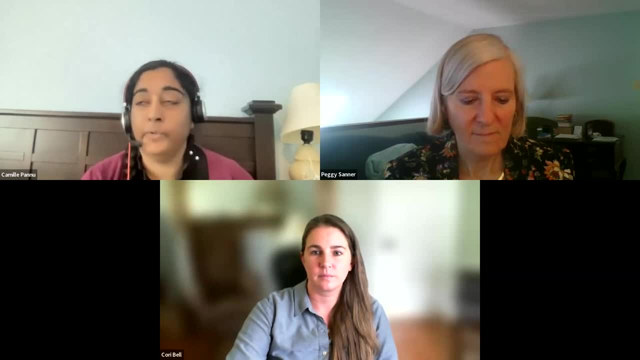 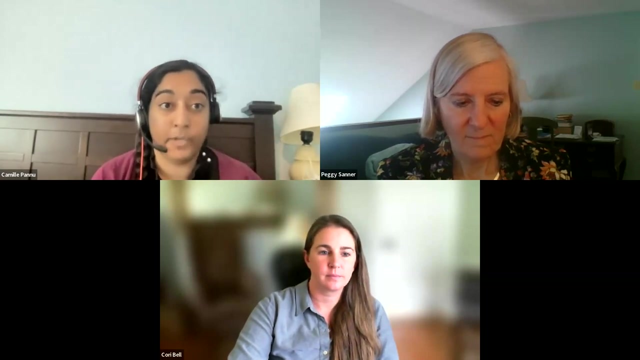 California has some building in, like Arroyo Seco, for example, or Seco in the Pasadena Los Angeles area is quite large and actually does have a lot of housing built into it. but if you look in Arizona, Arizona, Utah, Colorado, parts of New Mexico, for the most part they don't build in the arroyos because they know that if there's a rain, a flash rain or flash flood, it would be catastrophic for people to be there. 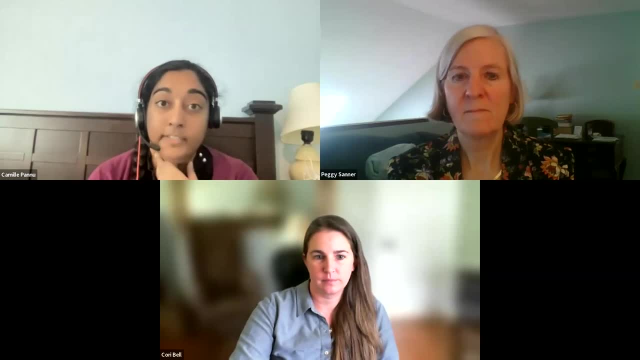 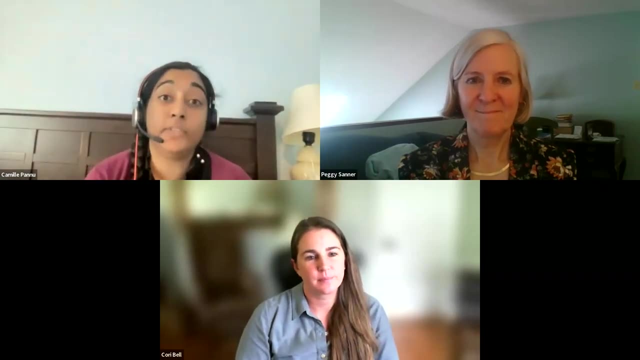 So instead, what they've done is they've converted a lot of their arroyos into parks. so this is kind of a meandering non-answer, But I think what I was trying to get at is I do think that there is room for stewardship and I do think that 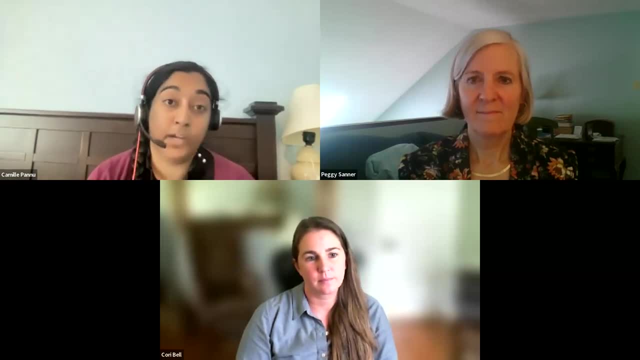 if folks can collaboratively kind of keep stuff out of the Supreme Court, I think it's going to be a really good thing. I think that would be a good thing, and perhaps one of those ways is to leverage the cooperative federalism between the federal government. 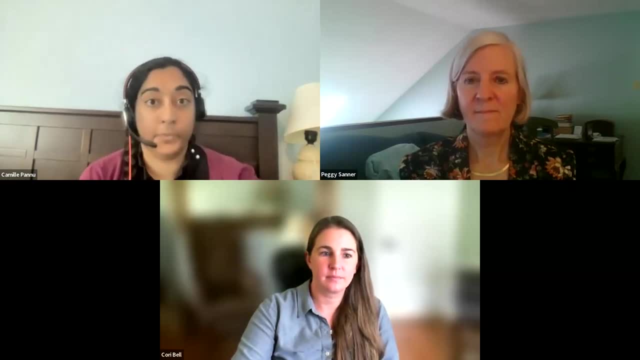 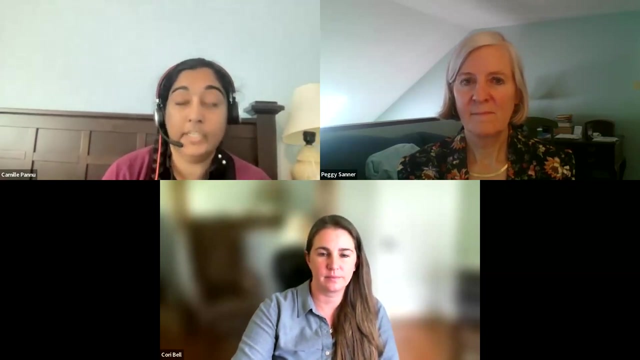 Given that we have a system of prioritizing waterways, perhaps there's a way to work collaboratively with states, particularly states that have these intermittent streams. I think it's going to be more controversial in areas that are experiencing climate change that is now making their streams intermittent that haven't been historically intermittent. 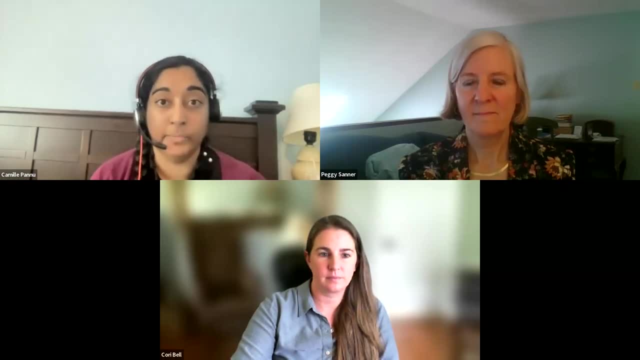 And that also do not have a history of very strong environmental change. So I think there's a lot of work to be done. There are certain red states that do environmental protection at the state level. there are certain red states that do environmental protection. 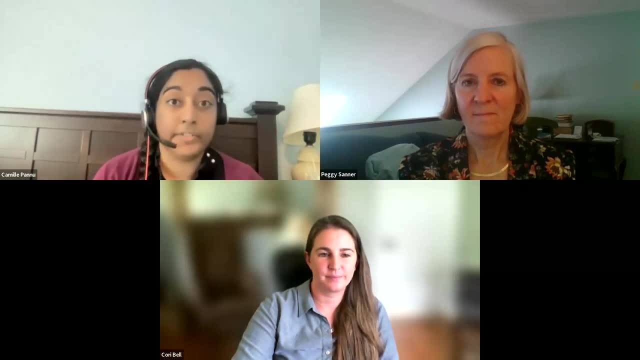 Not a lot of them anymore, but you know, historically this was a bipartisan issue, because destroying the environment has a bipartisan effect on everyone involved, and so there are still states that still kind of had that ethos, and perhaps not on all waterways or on all water issues. but there are certain critical issues on which they will unite and I think there may be some room for advocacy there. 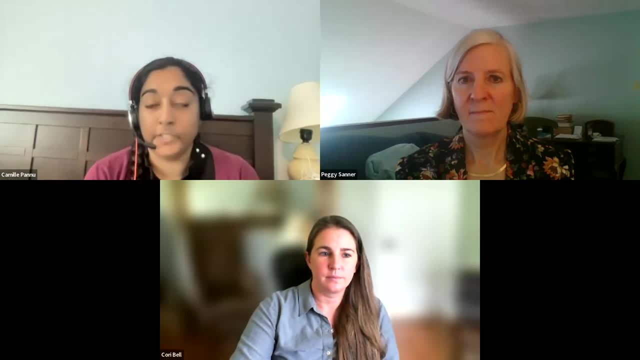 But I think that you know, if you ask Justice Alito, he will tell you the LA River is not a river. Tulare Lake is not a lake. Arroyos are not Arroyos, like they're not waterways. they're not. they don't have water. 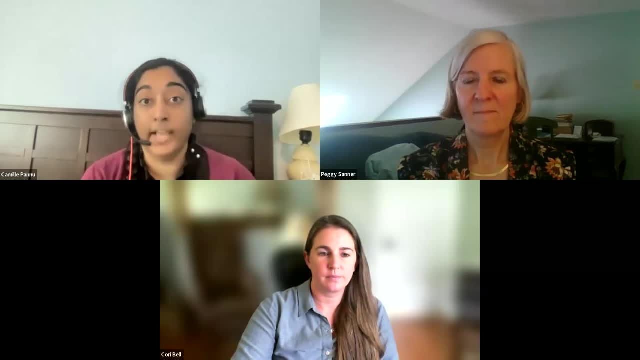 I think he would say it needs to have water more often than not or more than half the year. That was kind of what he hints at in his in this decision and in his prior opinions that are on the Clean Water Act. he tends to hint at the idea that dry means like periodic because of drought. it doesn't mean. 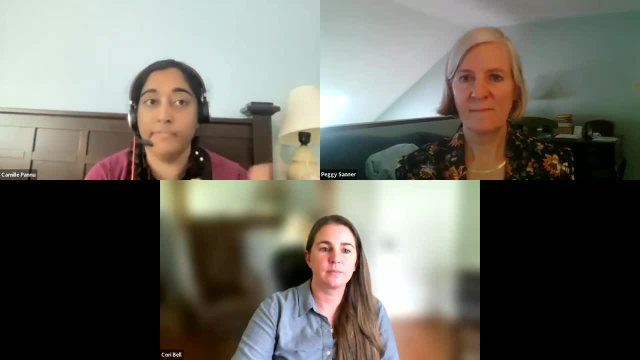 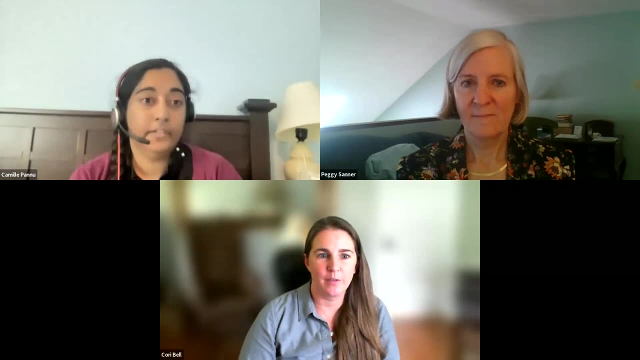 that it's dry more often than it's not, And in the Southwest things are dry more often than they're not, Right? I think there are some Southwestern states that that would be the vast majority of the water bodies, right? So it's a lot of-. 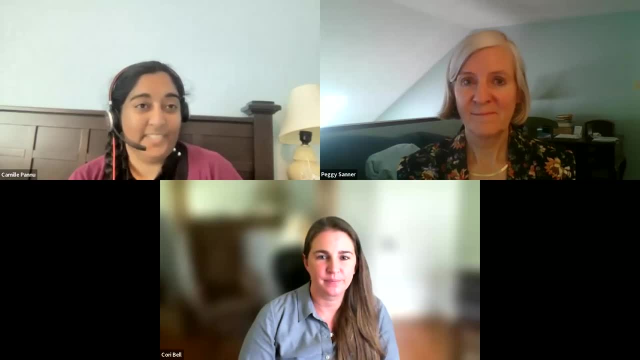 Yeah, Peggy had good statistics on this. It was: what was it, Peggy? was it 97% of, or was it you, Cori, that it was 97% of Arizona and 100% of New Mexico? Yes, I think that that's right. Yeah, it's, it's a lot. 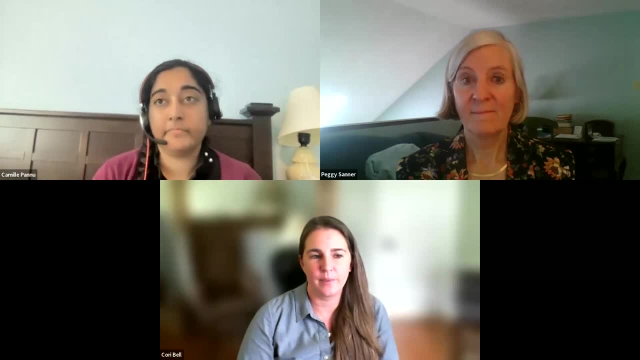 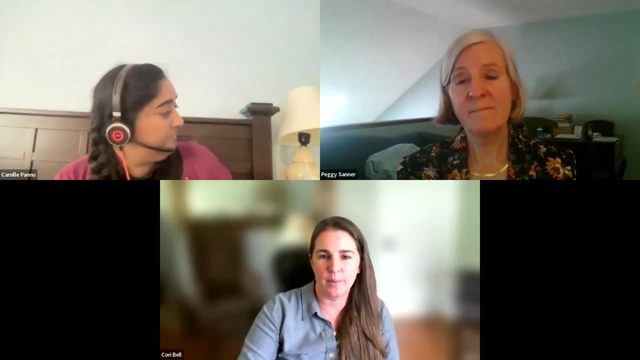 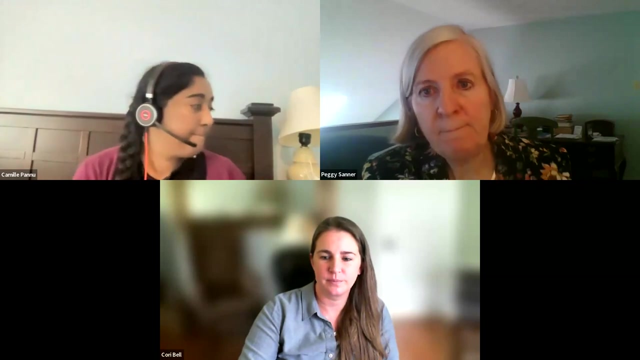 So we'll see. Peggy, There's a question about how SACET might impact the creation of TMDLs. if you want to talk about that a little bit, That's another really interesting question On a very high level approach, I would say. 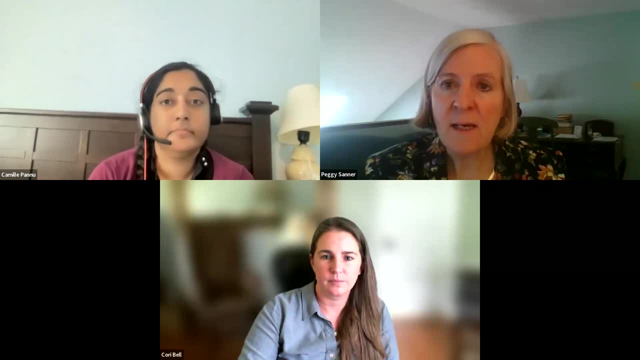 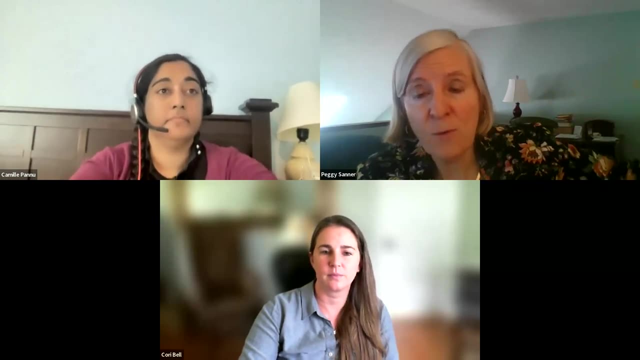 as others have mentioned, wetlands, whether they are in the uplands, the far end, the far highlands, the, you know, the source of our rivers or the tidal areas play a really important role in cleaning up the water. The ecosystem services provided by wetlands are very rich. They specifically, among those services, help to reduce the nutrients in waters, to get them down to, to ensure they are at levels that maintains a healthy environment, at levels that are consistent with water quality standards. 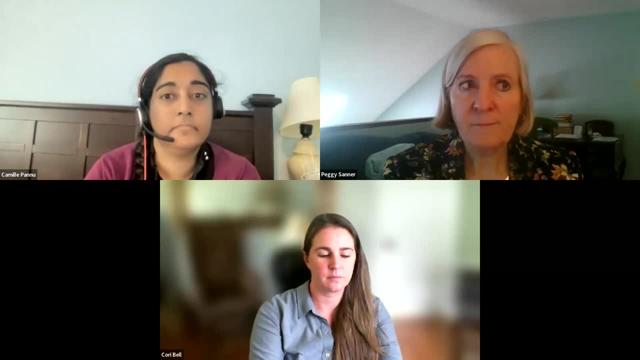 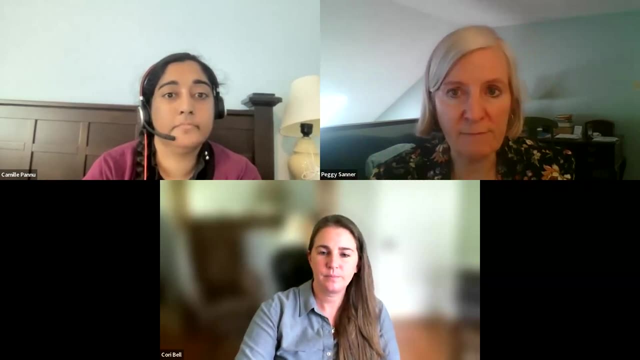 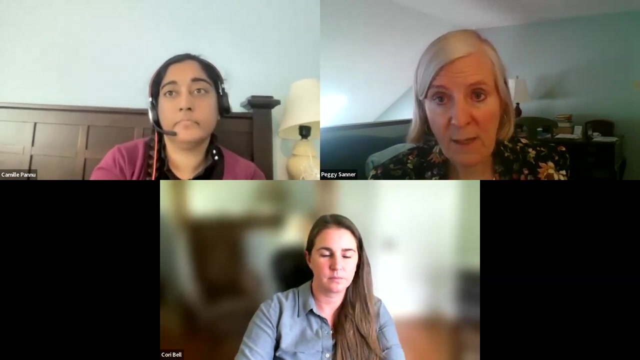 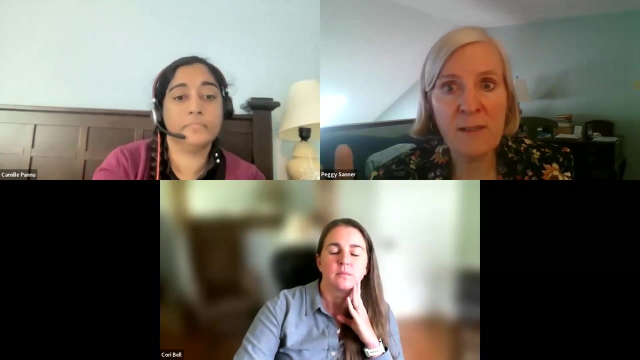 So in that general sense, to the extent we focus on non-tidal wetlands, which I think is where we're going to see most of SACET's effect, the elimination of federal protection could lead to greater impacts to non-tidal wetlands, loss of those non-tidal wetlands. 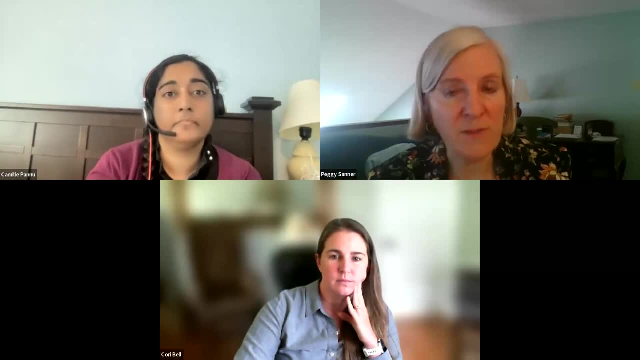 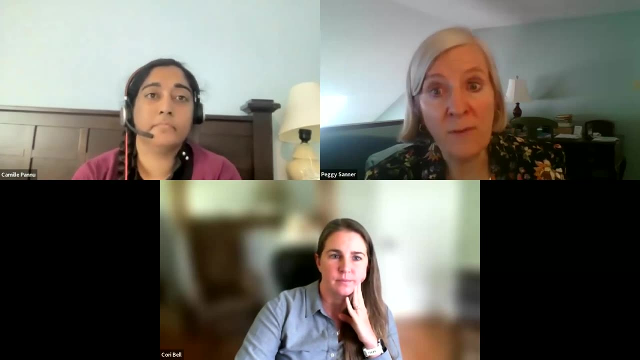 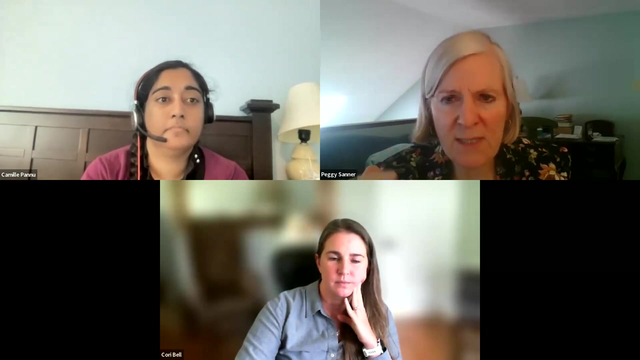 and loss of those ecosystem services, including reduction of nutrients and other pollutions, other pollution, And that would then allow for the downstream waters potentially to to be more polluted. but it will be a very complicated study that would be required to address that, because 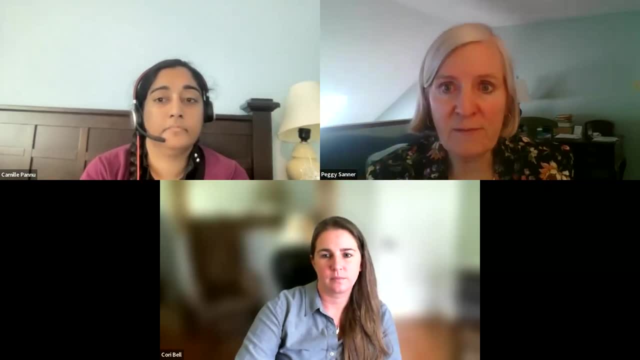 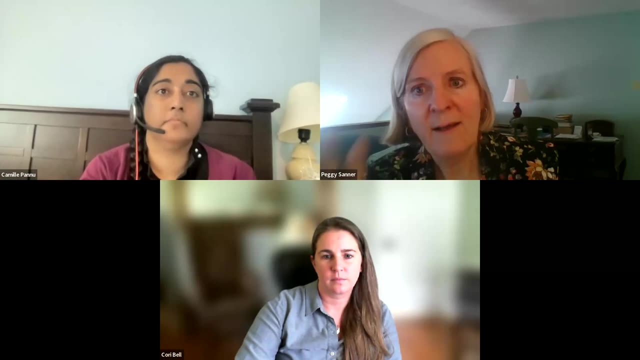 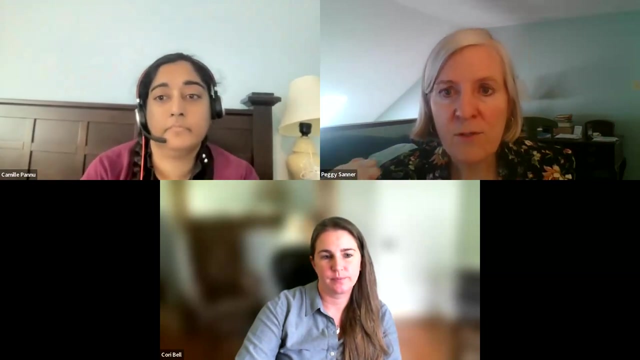 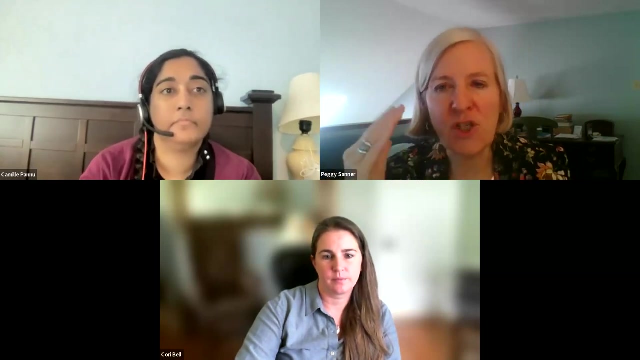 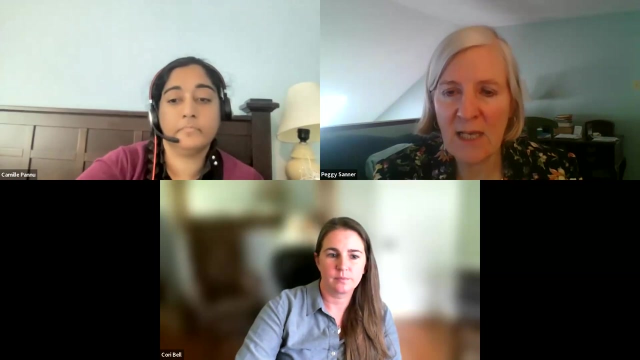 it would entail having a conclusive answer, which I don't have today, on you know which non-tidal wetlands are outside the new waters of the US, arising from SACET, and which are not. So again, I think it's very context specific, but I- but that's the general area that I see that wetlands help to through all the services they provide to keep our 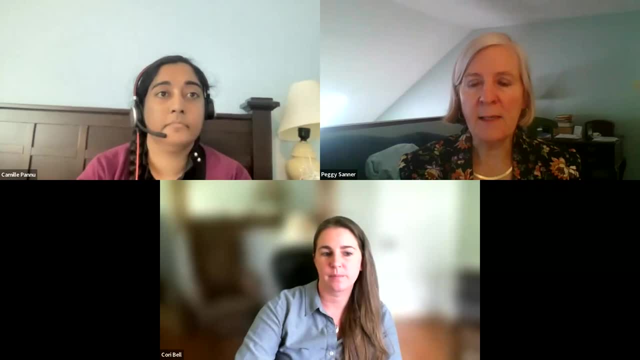 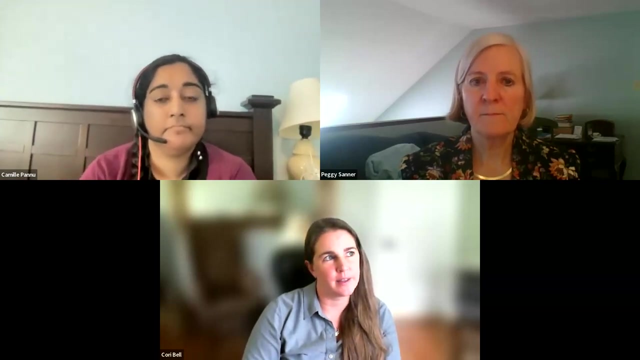 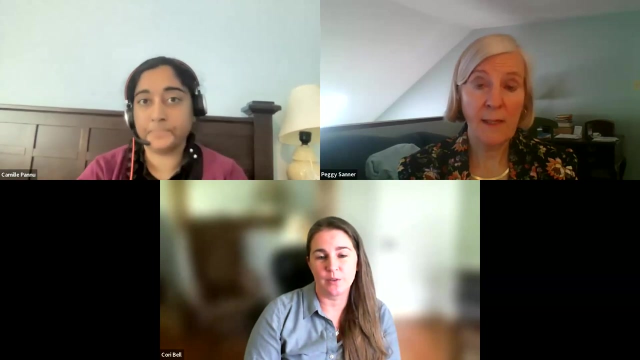 to keep our waterways unpolluted and and, and those, those are essentially irreplaceable services. So we'll have to see how that plays out in the land. Yeah, it seems like it would be safe to say that we'll probably need more TMDLs without the protection of those wetlands, right, Because we're going to lose all those ecosystem services. 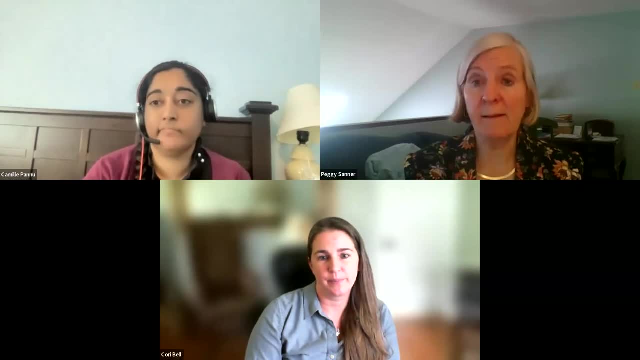 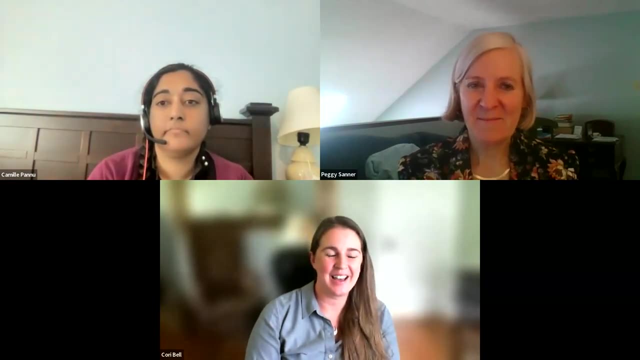 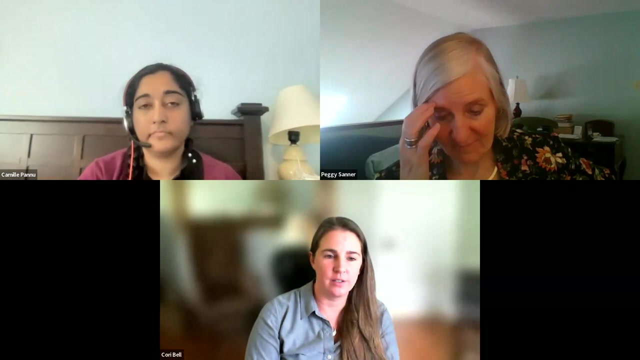 Yeah, More TMDLs that are actually implanted in the system. Yeah, more TMDLs that are actually implemented and, you know, carried to, carried to their term, But, yeah, sorry. Yes, Camille, a similar question for you: How might SACET impact groundwater regulation and the decision in County of Maui? 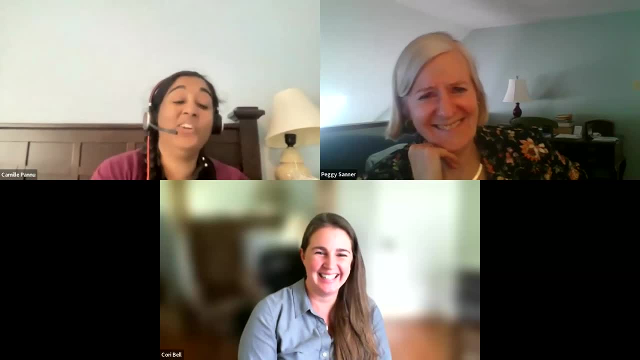 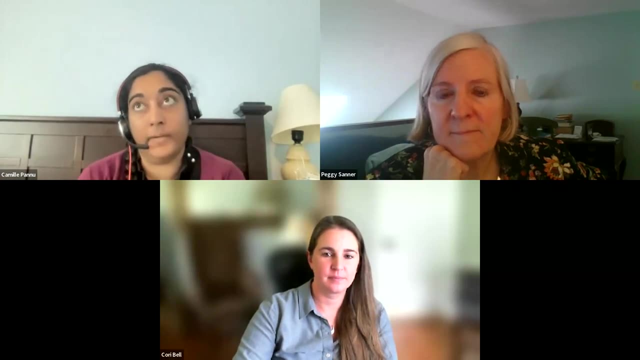 I don't want to think about it. Well, you know, County of Maui is relatively recent and comes from a conservative court. I think it's a really good example of- I mean I don't think the court is is on board with the Alito position- that groundwater in the context of County of Maui. 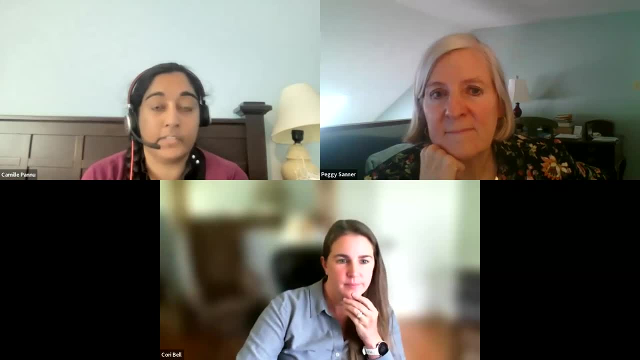 should not be considered under the Clean Water Act when it has a nexus to surface water. That's long been the law of several states in the West. So so I guess maybe I'm I'm a bit of a Pollyanna, but I'm optimistic that because I work in the state 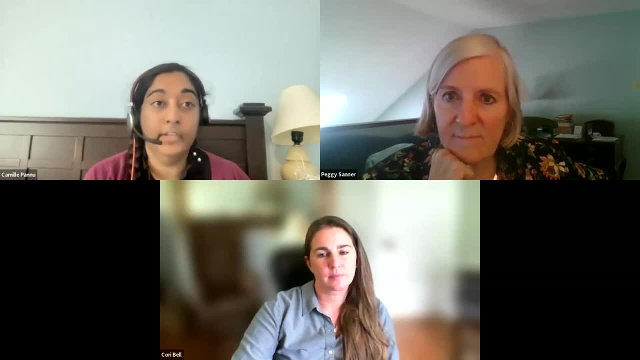 came from a conservative court. there's not enough votes to overturn it, So I'm hopeful that County of Maui remains good law. The hardest part about cases like County of Maui is proving that the groundwater has a nexus, So a lot of money goes into the hydrological and engineering studies. 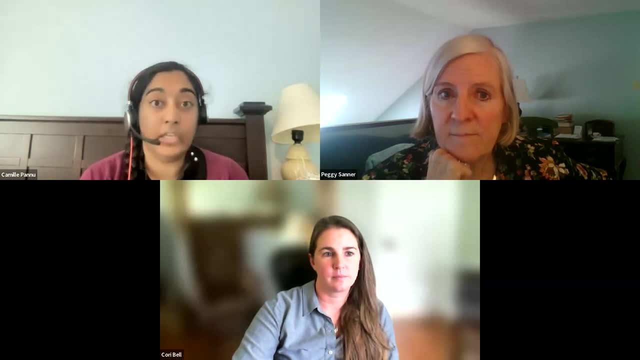 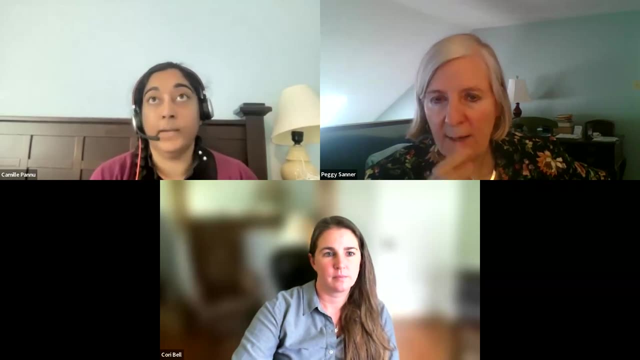 to establish that the nexus is sufficient and significant enough to bring it under the Clean Water Act. So it's actually kind of difficult to prove a groundwater pollution case, even under County of Maui as it stands. So I'm hopeful that SACET will not actually roll that. 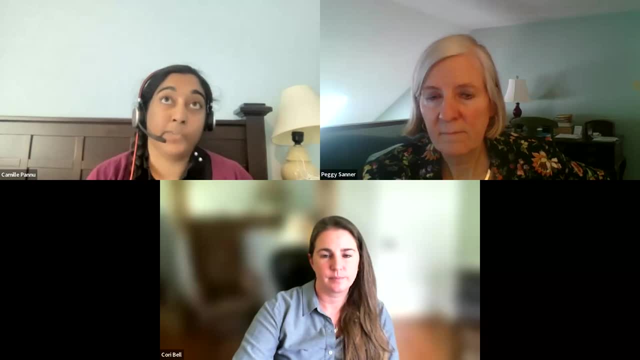 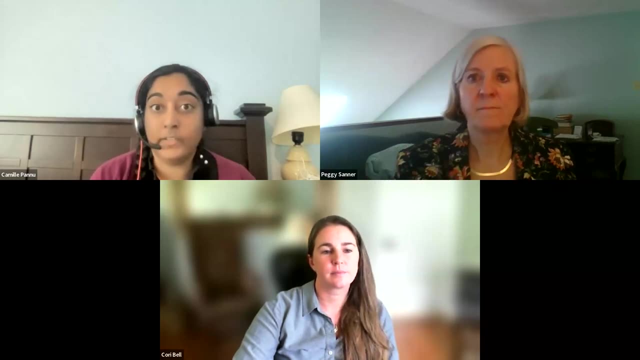 back, even though I think the County of Maui was kind of brave or not brave of the court. but it was a little bit of a departure from the way that the court had dealt with groundwater in the past, which is that they said: like we're not going to deal with groundwater because you 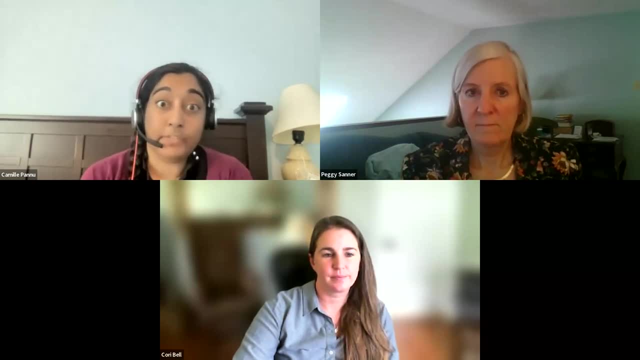 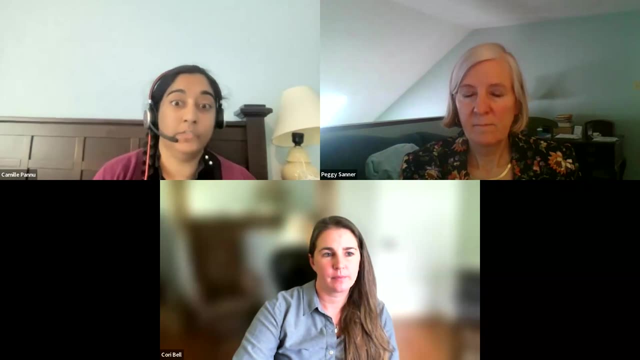 can't put a boat on groundwater Like it's definitely not navigable and it's historically not regulated the same way as surface water. And so I think, because a conservative court put its neck out a little bit on County of Maui, I don't think that. 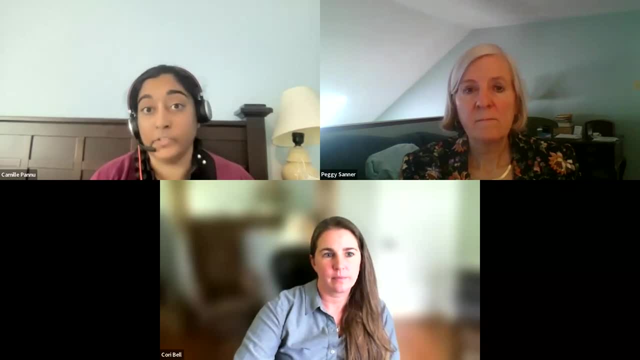 the current court has the appetite to roll it back. You still have several justices that were in the majority on County of Maui who are on the court, So I'm hopeful that they won't want to. I don't know, it doesn't come up often enough, to be frankly honest, for them to go. 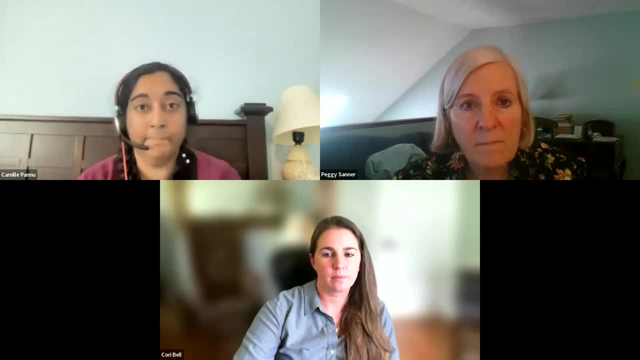 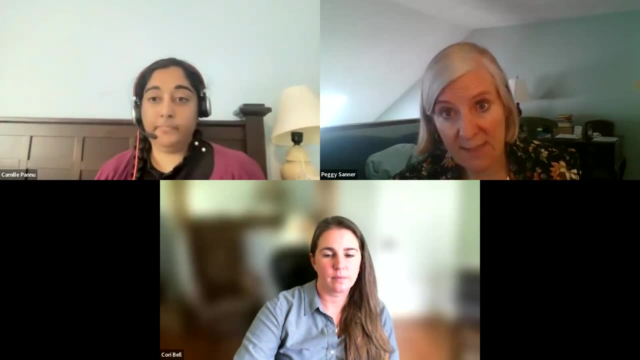 after it, the way they went after wetlands and SACET. in my opinion- And I'll just add one specific instance that I'm aware of- that actually was not successful. I'm not sure if it's true, but I think it's true. I think it's true. I think it's. 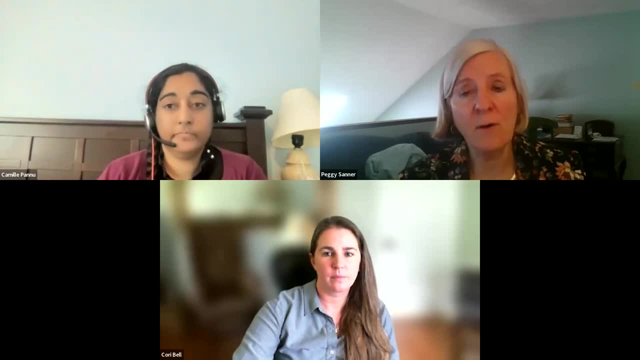 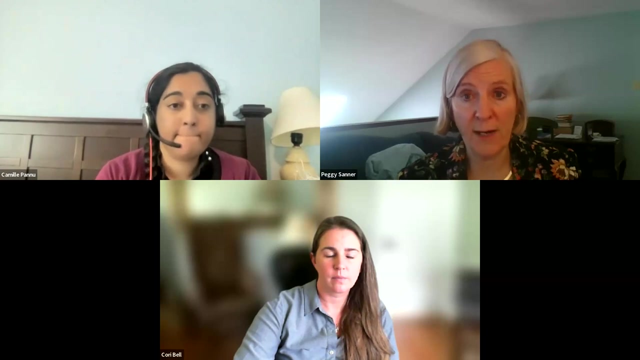 successful. It preceded County of Maui but involved a coal ash pond in our tidal areas, where the discharge of the effluent from the coal ash was proven by a trial court, after a full trial, to have originated in the coal ash ponds and to have gone through groundwater to reach the. 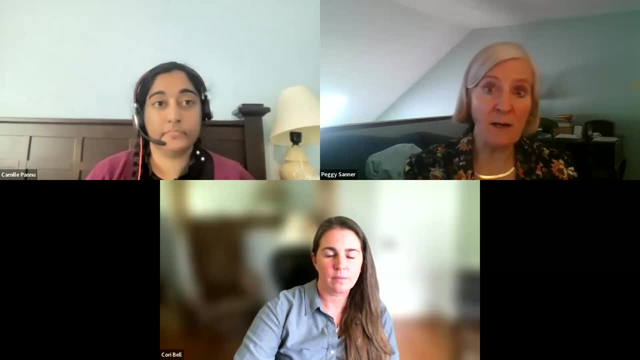 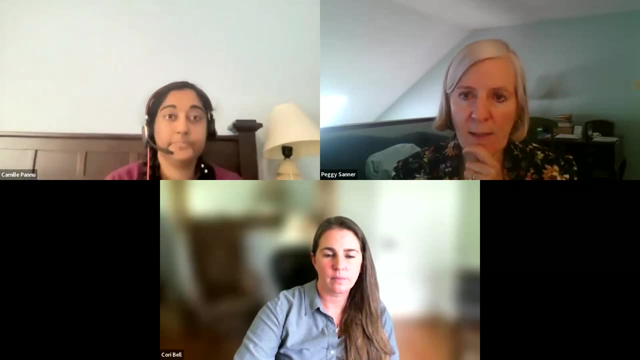 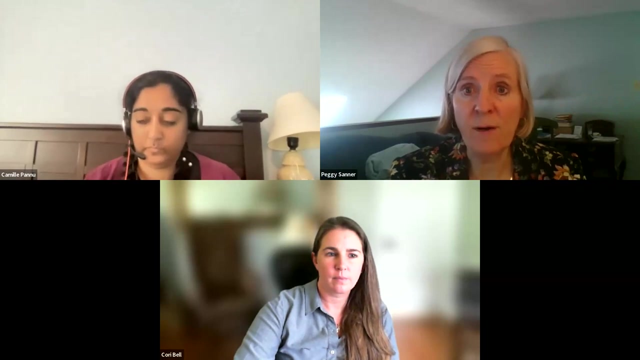 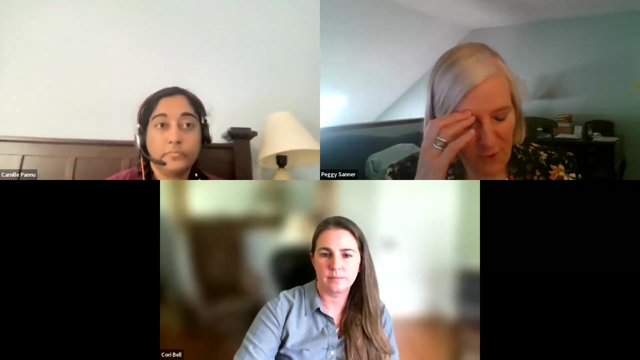 adjacent stream And the stream itself is plainly Clean Water Act governed, So the case ultimately died on other grounds later on, but we will see the cases where that functional equivalence will come up in lots of different contexts. So it should be really interesting and, frankly, very important. 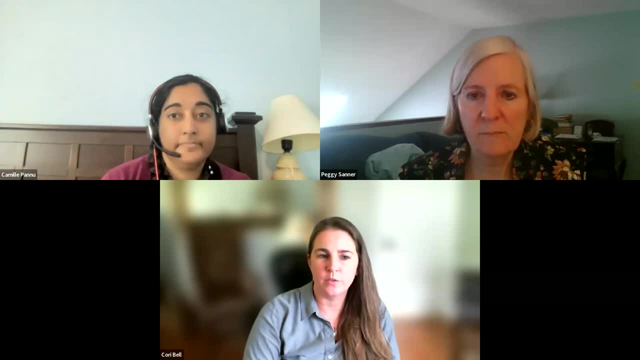 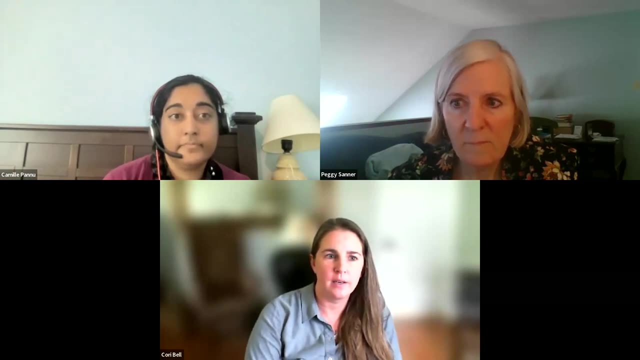 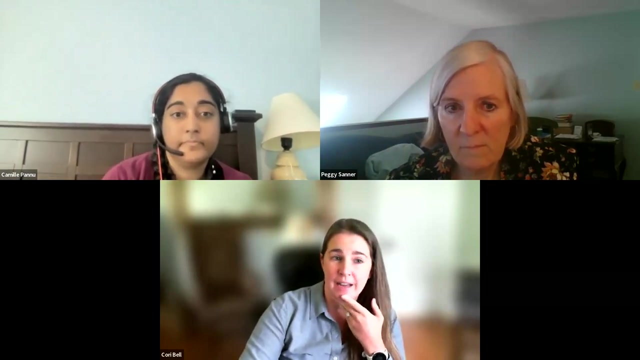 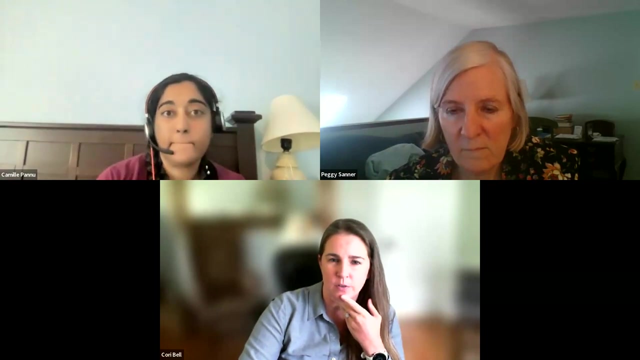 I think we have time just for one or two more questions, And I'll direct this one to you, Peggy. So there's a question about how SACET might affect Executive Order 11990, which is an executive order that protects wetlands. It was issued in 1977.. I'm not sure if you're familiar with that. 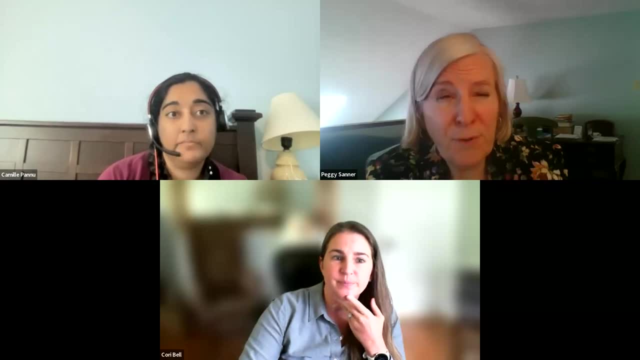 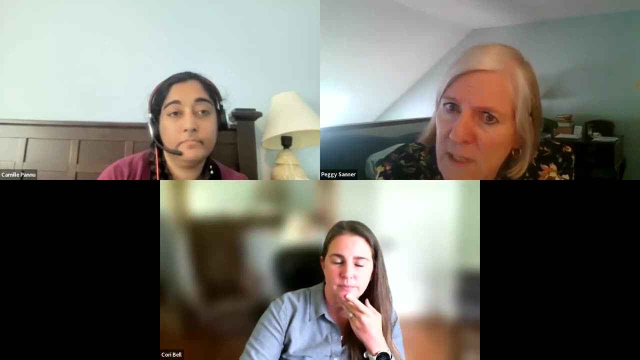 Actually, I'm not familiar with it, 1977.. 1977 would have put it, if I'm right about this, in the conservative administration. right, This was the Jerry Ford administration. Am I thinking correctly? I think, Carter. 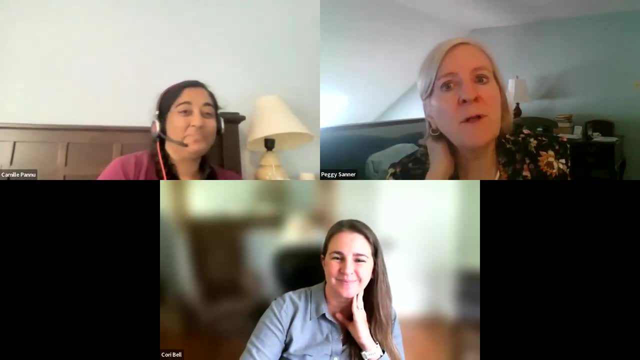 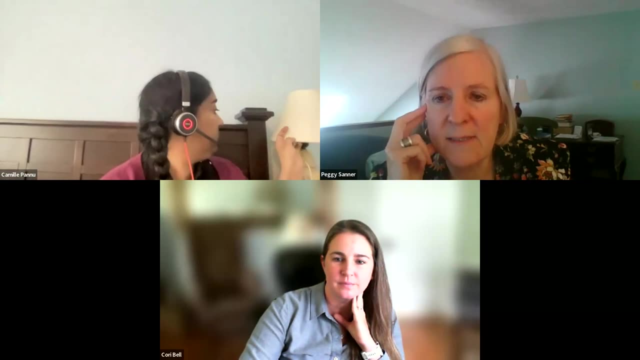 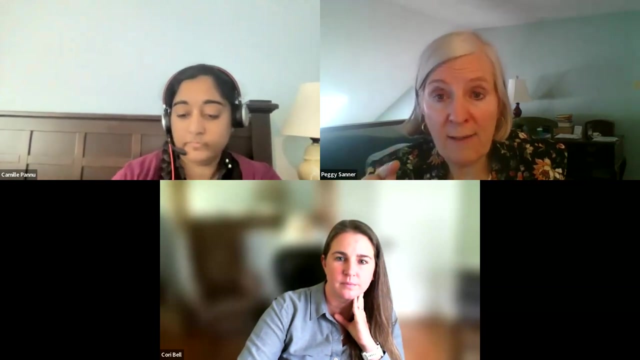 Oh Carter, Absolutely, And I ask that question because, of course, an executive order is issued by, in this case, the president, And so it matters in that sense to sort of think about who was the executive. So, Working on generalities and assumptions here- my own and that may be wrong- my guess is it was a. 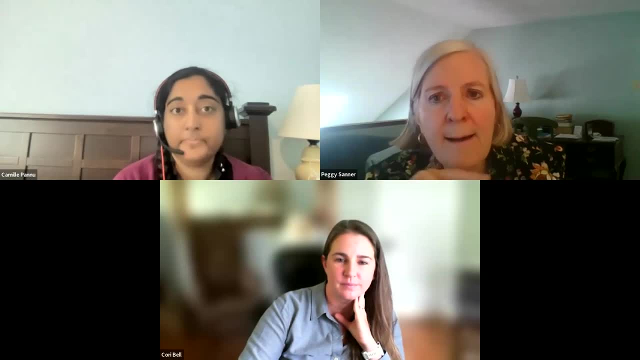 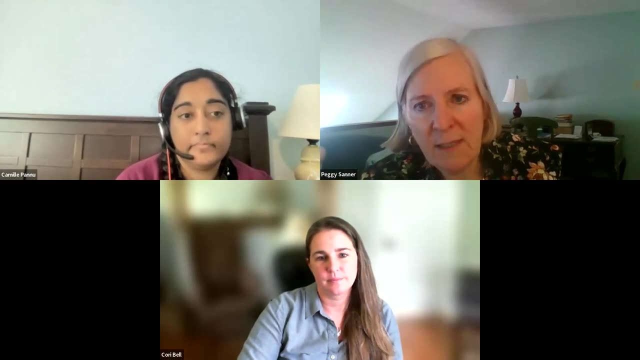 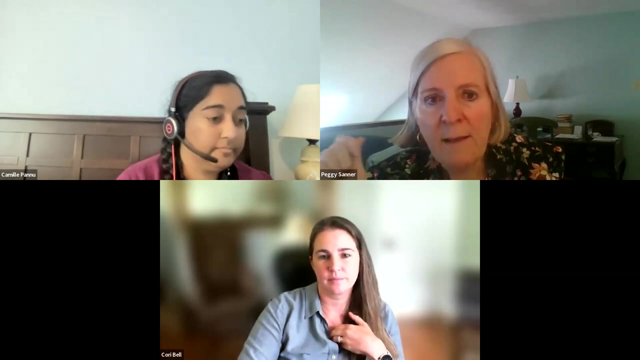 really important executive order for protecting wetlands. That's all I know. Executive orders have an interesting history. They are definitely the law that governs federal agencies during the term of a president. Their effect thereafter, you know, is kind of questionable. 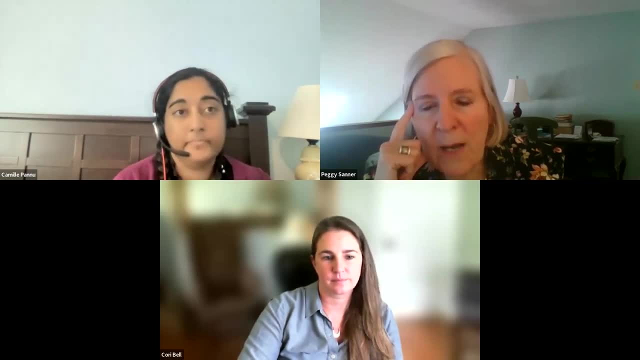 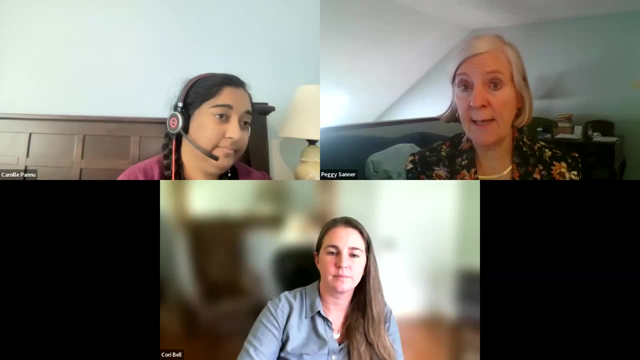 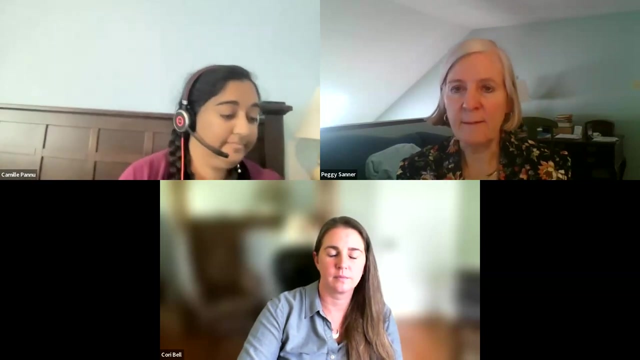 It sort of dissipates pretty quickly. So I would say it would be hard to make a credible case that it would stand in some way to help us hold back against the force of Sackett. I think we'll have to recognize that that was a great moment in history. 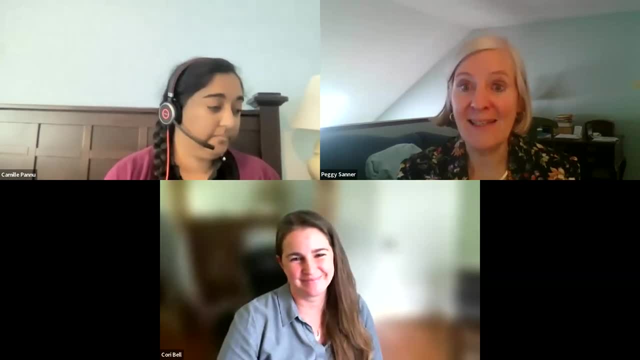 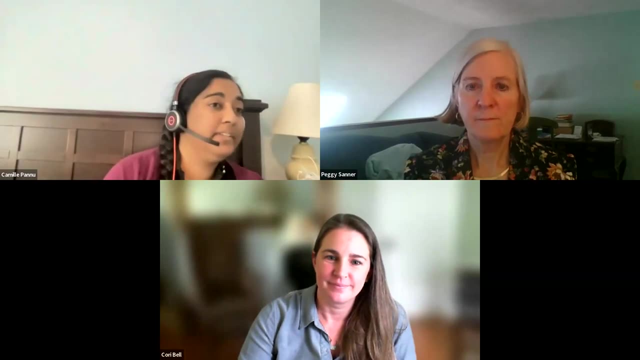 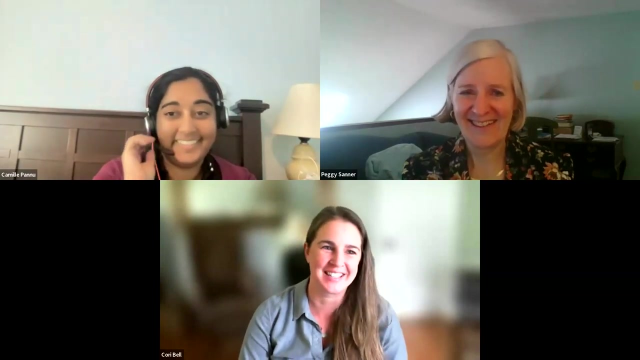 and that we could go back to it for ideas for what we can try to do in the future, but it wouldn't be considered governing law, Yes, or one. maybe we're just feeling depressed about the current situation. We can go back and revisit that executive order. 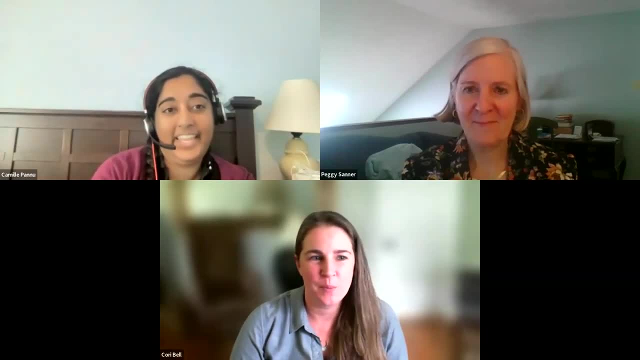 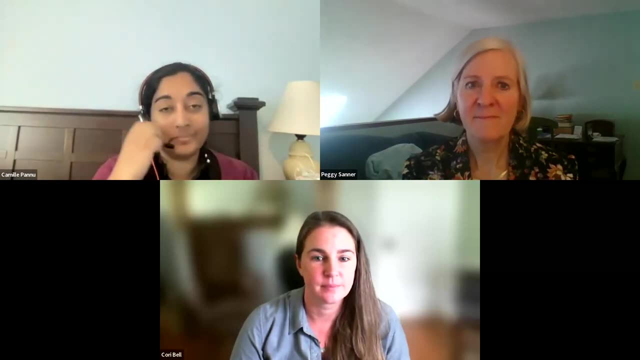 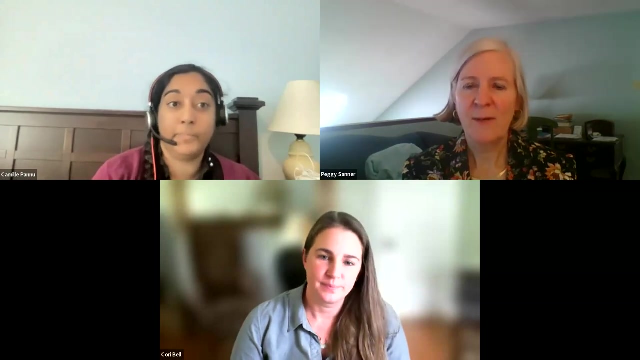 Right, Yeah, I have one more. Yeah, and it might- sorry, I was gonna say it might help also to understand kind of the order of authority. we call it among lawyers. So an executive order is kind of at the bottom of the list of things that are controlling. So, like Peggy was saying, an executive order can inform what federal agencies do. It certainly isn't in effect until it's repealed, But if you're in an administration that doesn't want to repeal it but also it doesn't have a policy priority, it might not get much traction As a functional matter like Sackett. 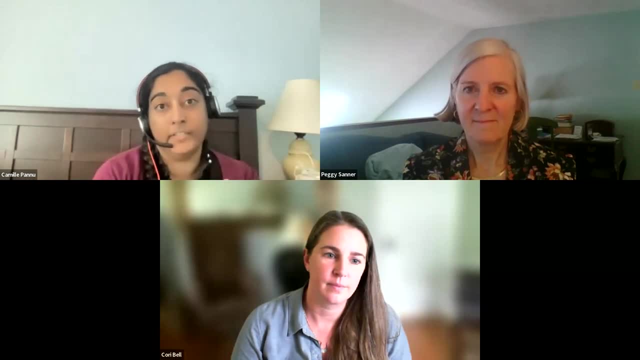 will trump. the interpretation of the Clean Water Act under Sackett trumps an executive order to a certain extent, And the Clean Water Act trumps an executive order as well. What typically happens is you try to harmonize the two, And I think that's what, historically, the argument is. 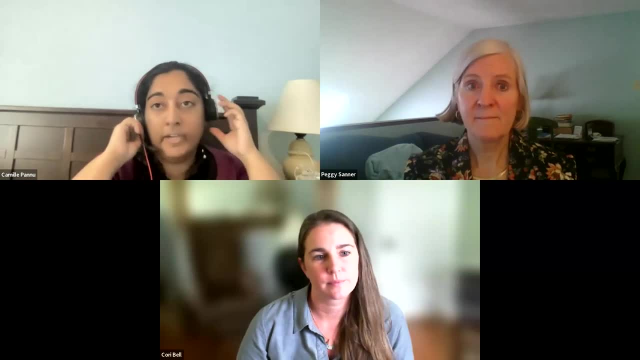 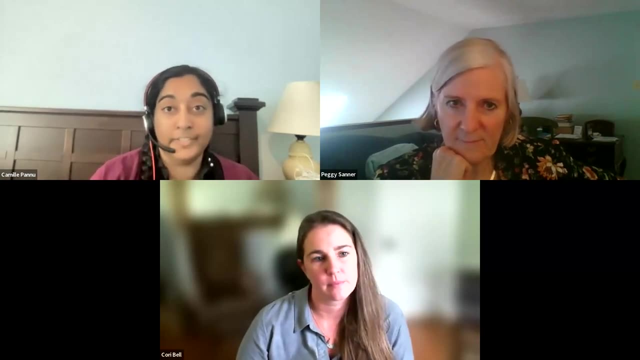 The Army Corps of Engineers in particular has done with executive order- the executive order that's being cited- But I think it's important to know that you can functionally overturn an executive order without having to actually litigate and vacate it. The legal regime can change if it's. 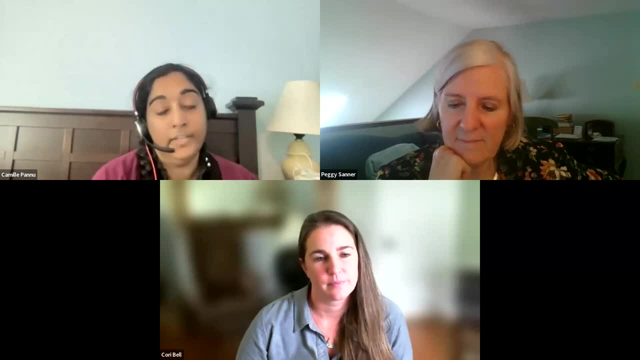 higher level court cases and statutes and that those can deprive an executive order of its power, even if the executive order is technically in force. It's kind of the lowest in terms of power: Right, Right, Right, Right Right. 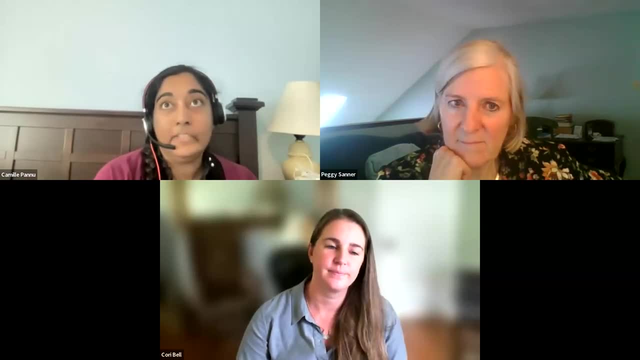 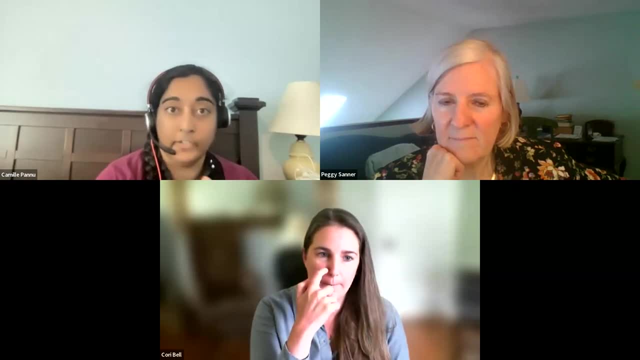 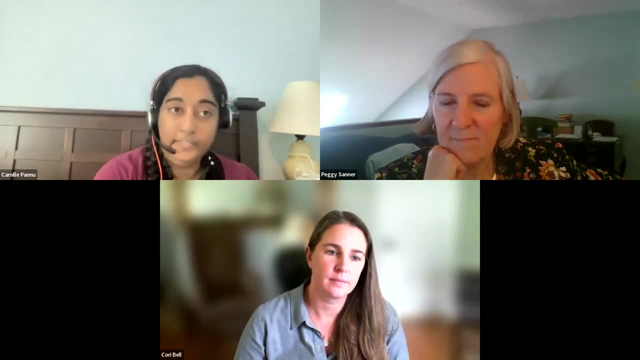 have a lot of process because they go through Congress and we elect our Congress people and regulations and rules have a lot of process and so they get less deference than a statute. But you know we think about them. So an executive order has no process for the most. 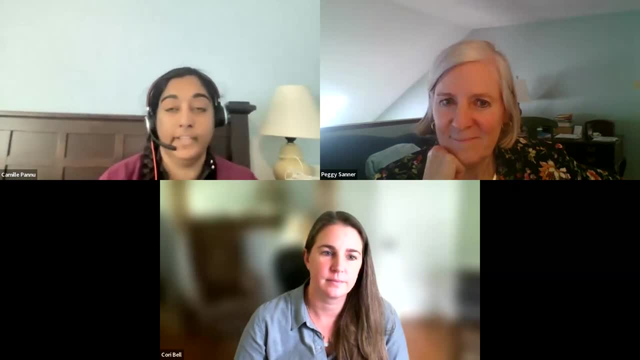 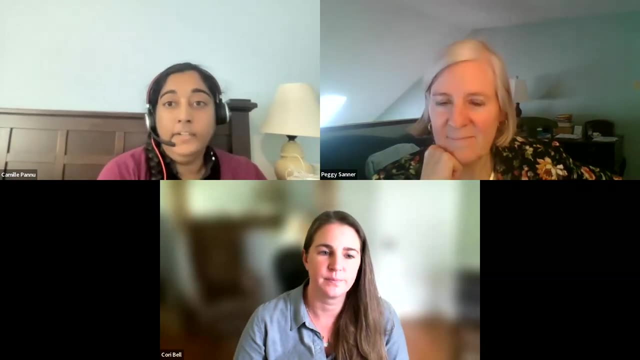 part, And so it has very- it's very- weak. all things considered, It can be used effectively, but within the boundaries already set through case law statutes. Thanks for that, Camille. I think that that is probably a good place for us to. 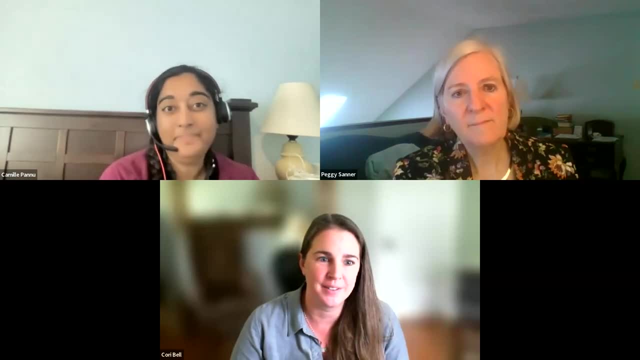 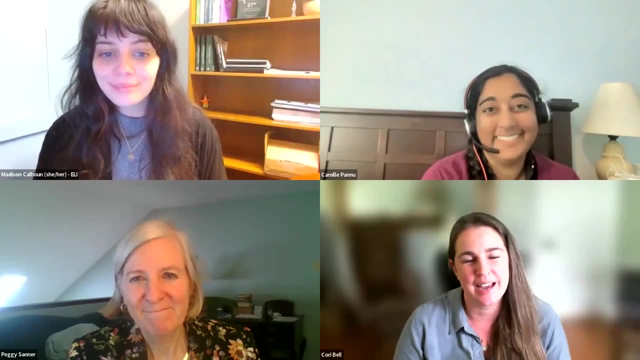 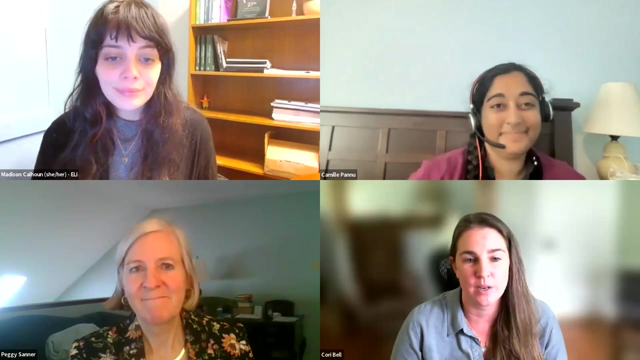 wrap up here. Thank you to both of our panelists and for entertaining a very hot bench, I'd say, of questions, especially with Sackett, And thanks to the audience for attending and asking a lot of these really interesting questions. Like I said, I think that we're going to be playing wait and 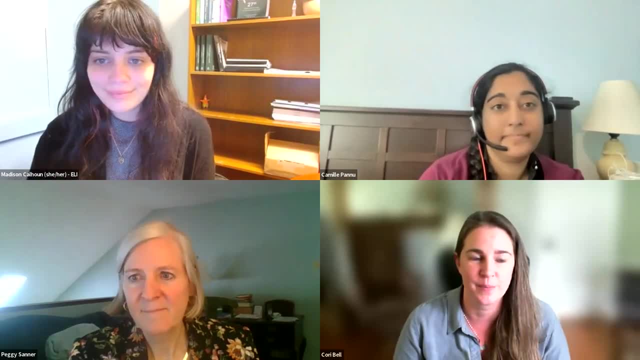 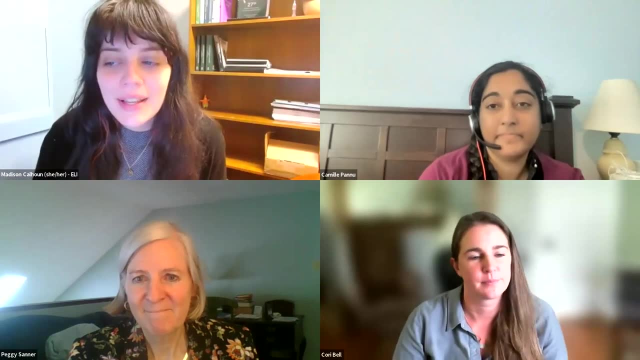 see when it comes to Sackett, at least for the next several years, And I will pass it over to Madison now. Thank you all so much for speaking at today's webinar. We so appreciate your time and your efforts to educate our audience on environmental law. We appreciate. 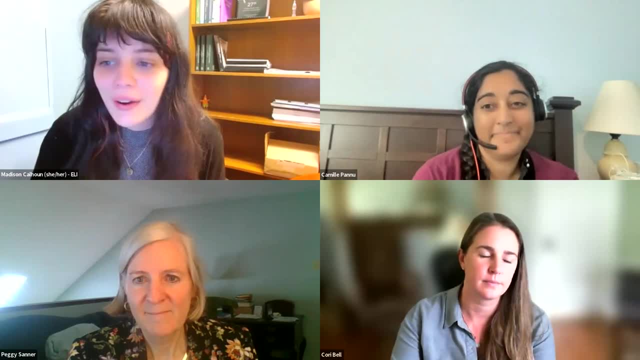 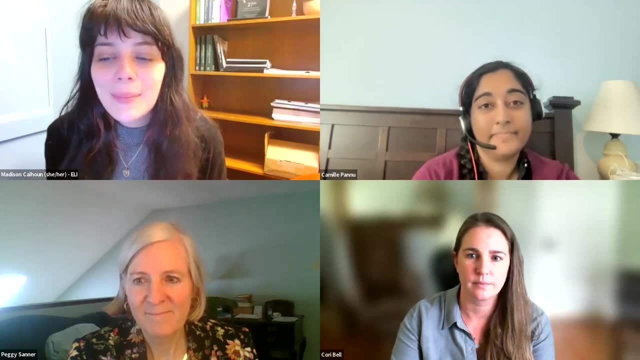 you diving into the Clean Water Act and also spending so much time answering our audience's questions today, And thank you to those in the audience. Thanks for tuning in. We really appreciate your engagement. Please join us back at 12 pm Eastern on Thursdays throughout June and July for the rest of summer school Coming up next. 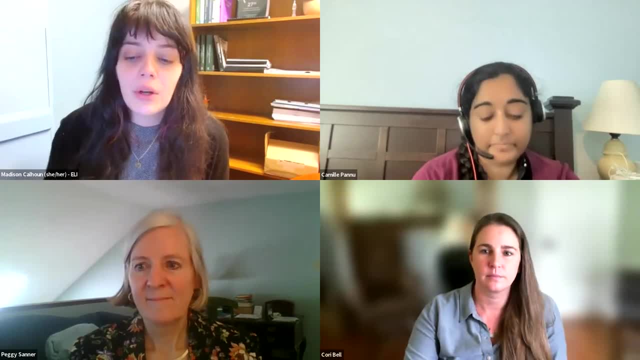 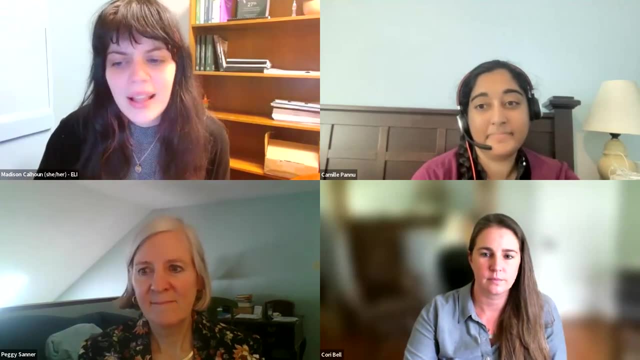 we have our land use and energy law session taking place at ELI's office in Washington DC next Thursday. That will also be recorded, So if you're not in DC, please look for it online. probably at the end of next week or the beginning of the following week, But Thursday after that. 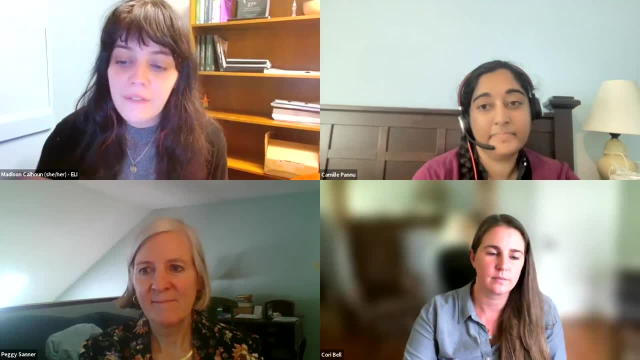 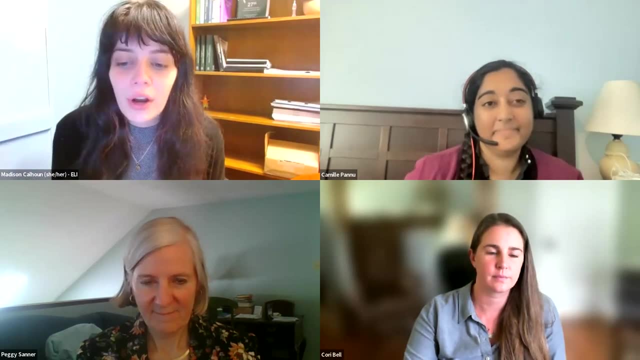 we will be taking a break, taking one week off, And then after that, three weeks from today, we'll be here again for our virtual summer school webinar on the Clean Air Act. Please remember to register on ELIorg if you'd like to attend future summer school sessions. Thank you again to our audience for attending and 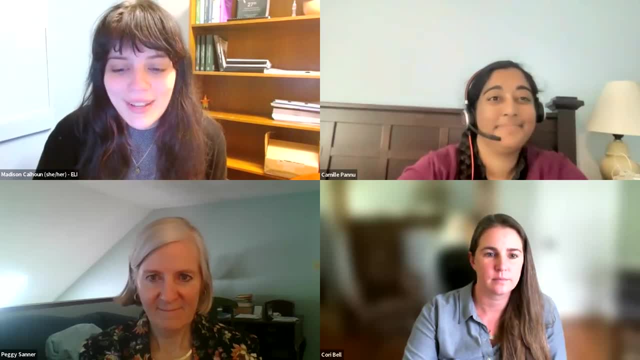 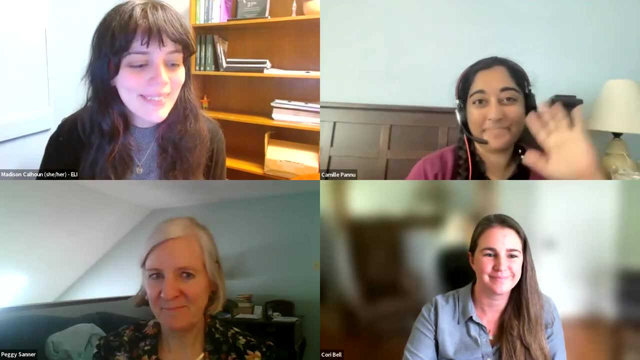 to our wonderful speakers, Corey, Peggy and Camille for their presentations. We so appreciate your time and we hope everyone has a great day. Thank you so much. Thank you, Thank you.